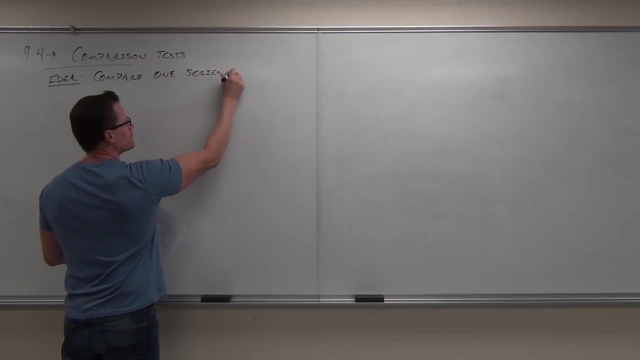 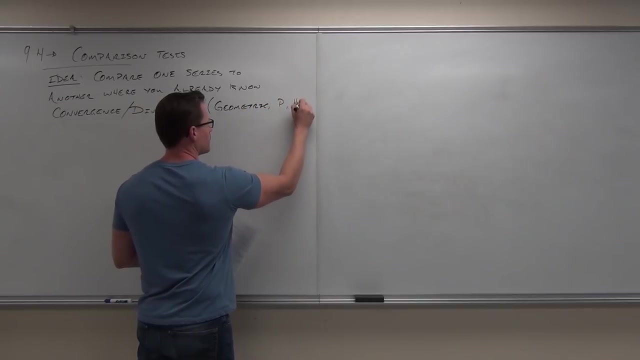 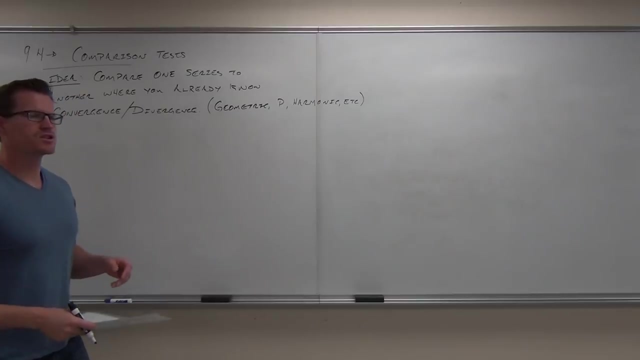 Compare one series to another where you already know the convergence or divergence. Typically, this is the series that we've already talked about in this class, like a geometric series or a piece series or a harmonic series, something like that. Do I need to write that down? Okay, I better write that down. So here's the idea. 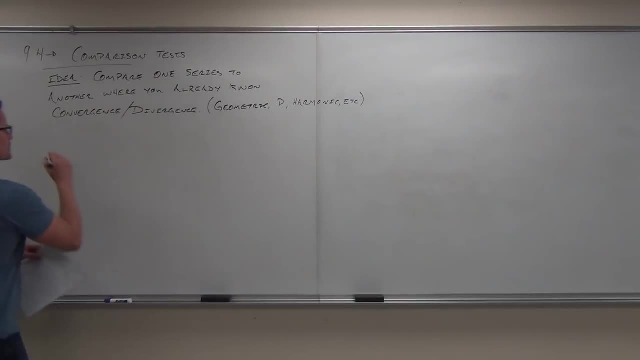 Do I need to write that down? Okay, I better write that down. So here's the idea. So here's where the comparison test comes in. It says: all right, so suppose we have two series. We have a series of a sub n, and we have a series of b sub n. 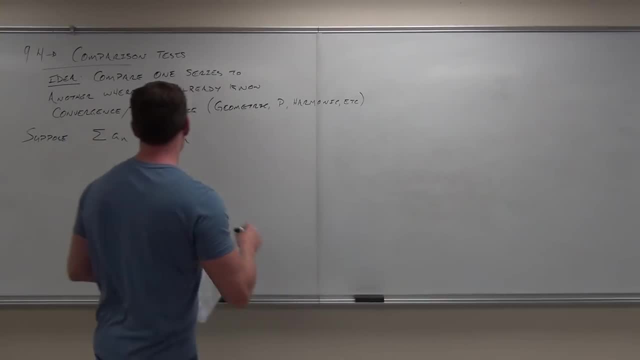 And both of these are series with positive terms. So suppose a series of a sub n and a series of b sub n are series with positive terms. Well, there's going to be two cases and I'm hoping that you see the similarity between. 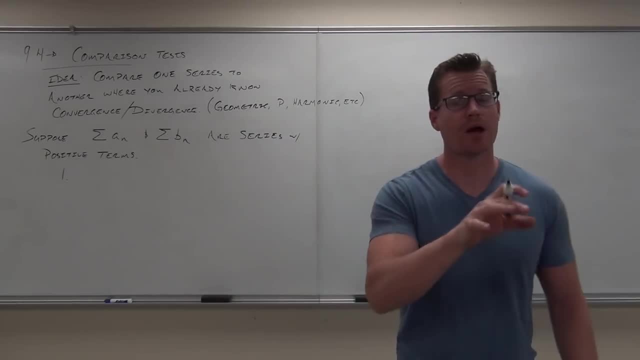 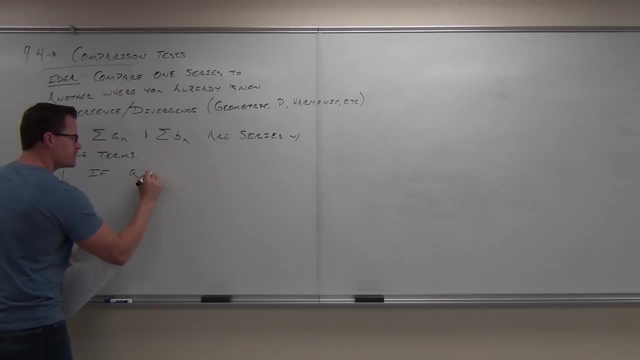 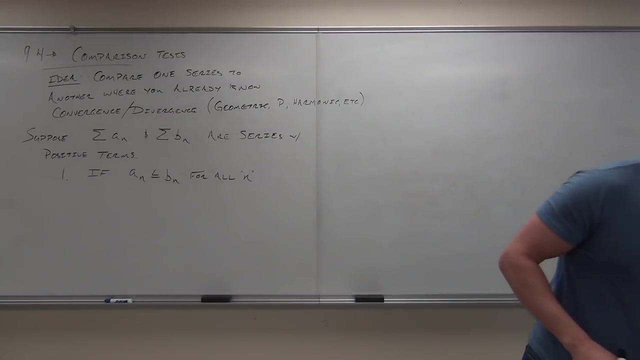 this comparison test for series and the comparison test that we had for sequences. So here's the idea. Let's suppose or let's say if let's say, a sub n is less than or equal to b sub n for every term. So basically, here's what we got. 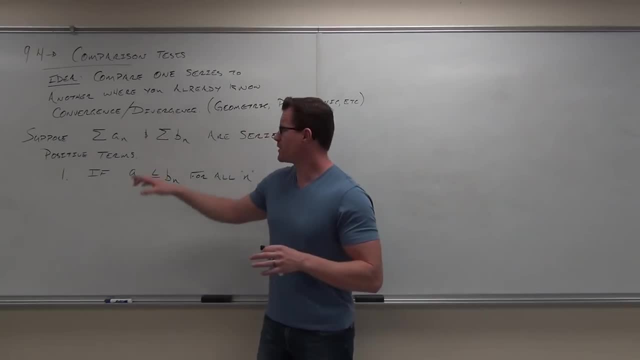 We got these two series. They both got positive terms. but here's what we know. We know that the series of a sub n, every term, the sequence of that, basically every term, Every term, a sub n is less than b sub n. 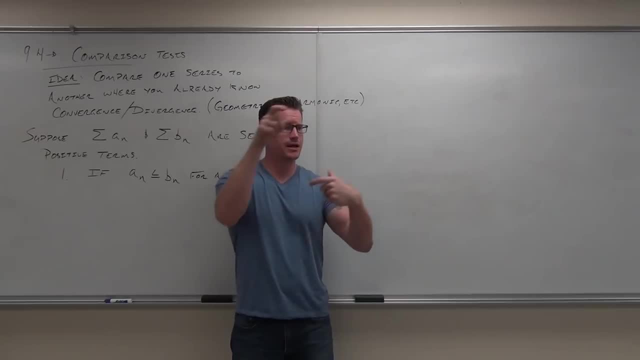 So, for the first term, a sub n is less than or maybe equal to b sub n. Next one, a sub n is less than or maybe equal to b sub n, And so forth and so forth and so forth. So basically, if I have my b sub n like this, my a sub n is right below it or maybe equal. 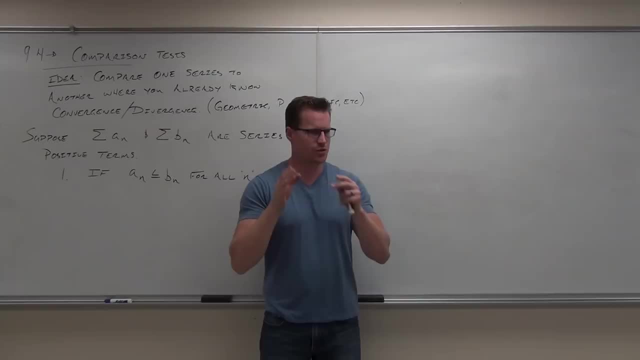 with it, But it's never above it. Do you guys understand that idea? So, term by term, a sub n is less than b sub n. Quick hint on: if you're right with that, Let's further suppose that b sub n, that series converges. 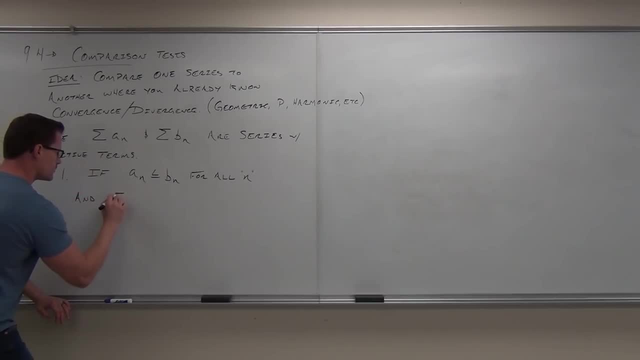 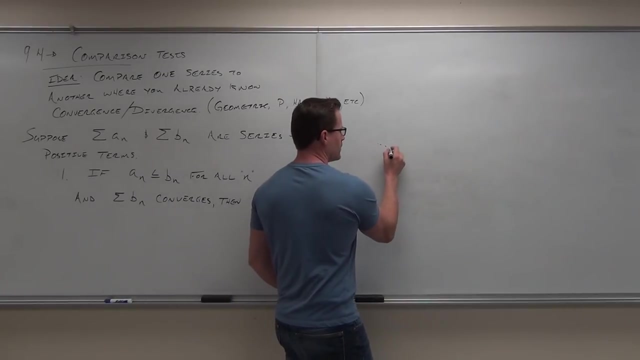 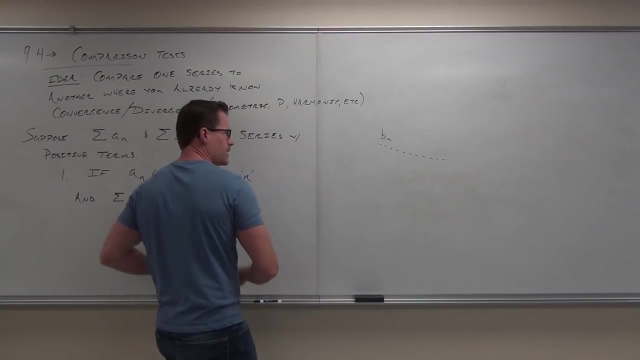 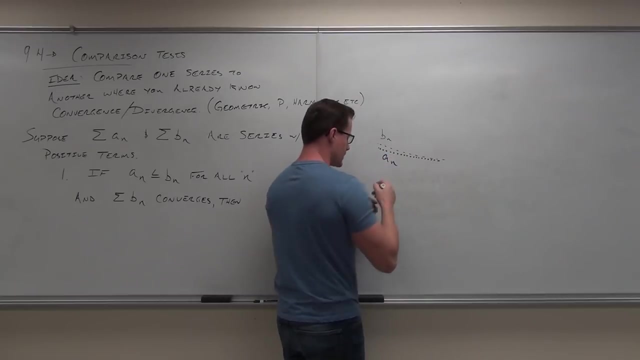 What's going to happen? What's going to happen if I have my b sub n's and I have my a sub n's? Okay, Okay, Okay, Okay, Okay, Okay. And I say, hey, tell you what. They're both positive terms. 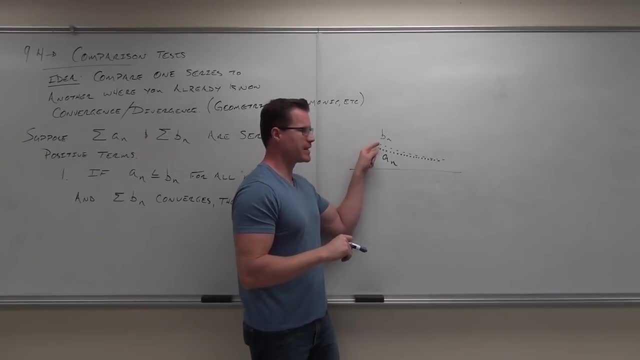 So they're both above zero. And I say for every single one of these terms: a sub n is less than, or maybe equal to, b sub n. It could be right on top of it, Who cares? It's just not greater than that. 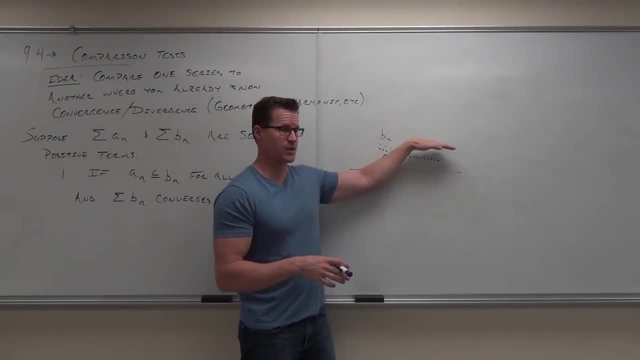 I say. furthermore, what I know is that this series, when I add all these terms together for b sub n, this series converges. So if the series of b sub n converges and a sub n is always less than that, but it's, 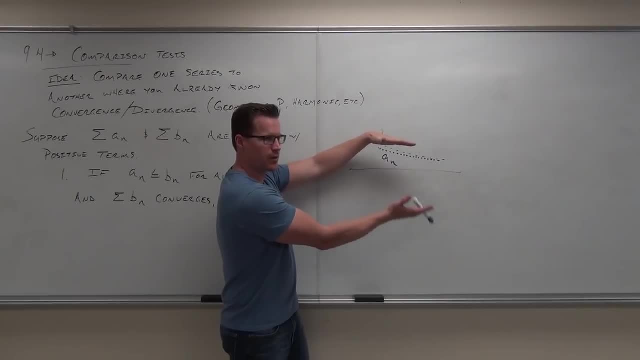 never negative, Right, It's always positive. So it's basically, it's bounded and it's less than the series that's convergent. What's going to tell you about this series of a sub n? What's going to happen to that? 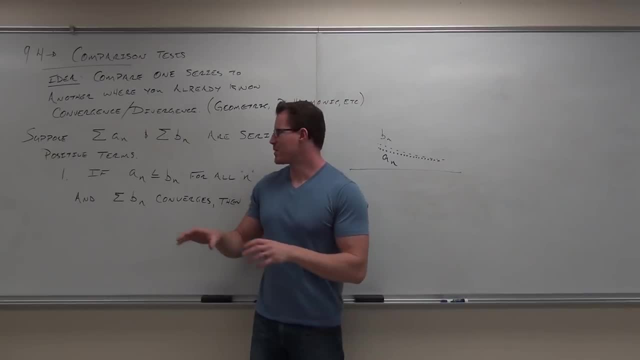 It has to be. So here's what the comparison test says. It says: compare one of your sequences to another one where you know the convergence, for There's going to be two scenarios. The scenario's going to be well if a sub n is always less than b sub n. 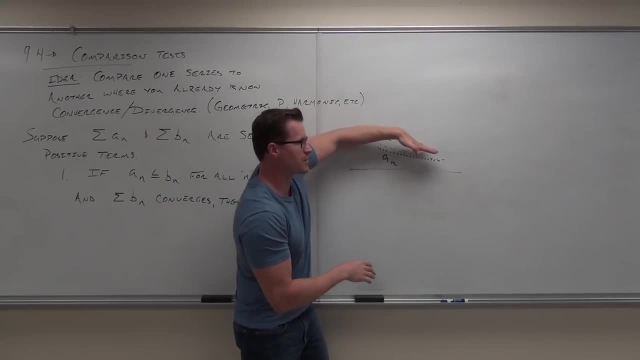 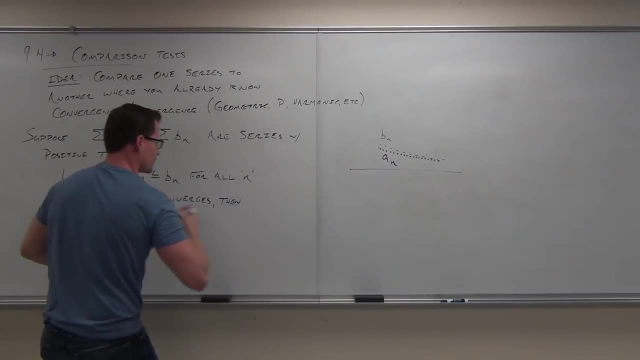 if b sub n converges, if the series of b sub n converges, where add all together goes to one number, then if a sub n's always less than that, it also has to converge. Okay, let's see if you're paying attention. 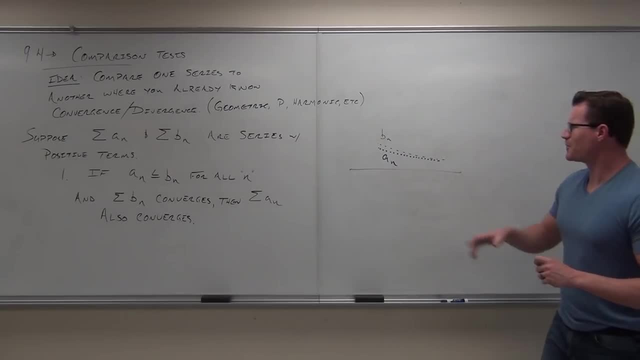 I know some of you guys look like you've got sleepy eyes, so let's focus right now. So now let's do this one. okay, Jacob here, eyes on the board. Now let's suppose that b sub n diverges If a sub n's always less than b sub n and b sub n diverges. 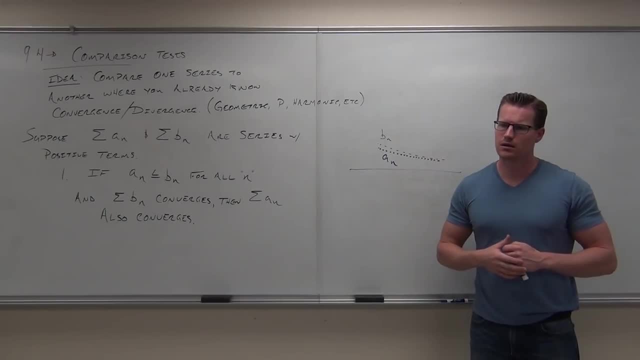 what does it tell you about? What does it tell you about a sub n? Why not? Because it's below it. It's below it. Oh well, a sub n is below the b sub n. So if b sub n converges, yeah, if a sub n's below it. 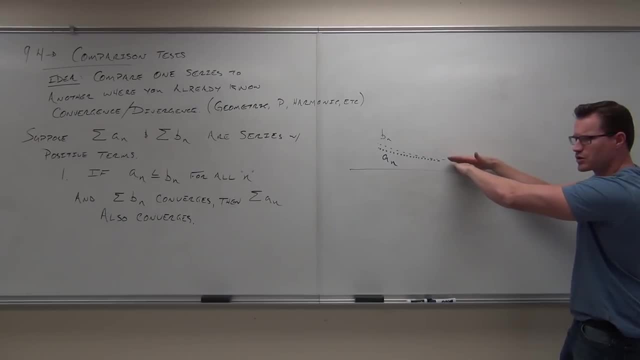 it's also going to converge. That makes sense, because it's kind of pushing it down here and getting closer and closer and closer to one number. If I add those together, we're talking about the series. now not just the sequence, but the series. 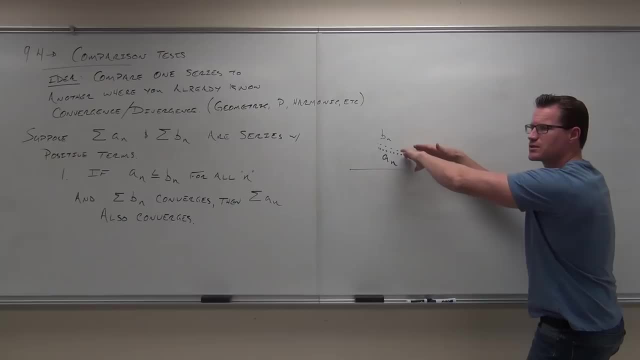 So if the series of b sub n converges and a sub n's always below it, then the series of a sub n also has to converge. But if the series of b sub n diverges and the series of a sub n is below it, 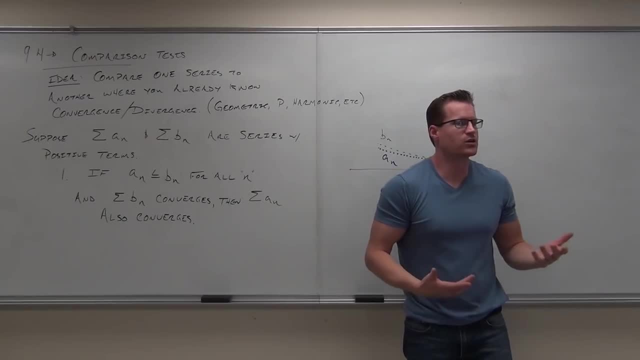 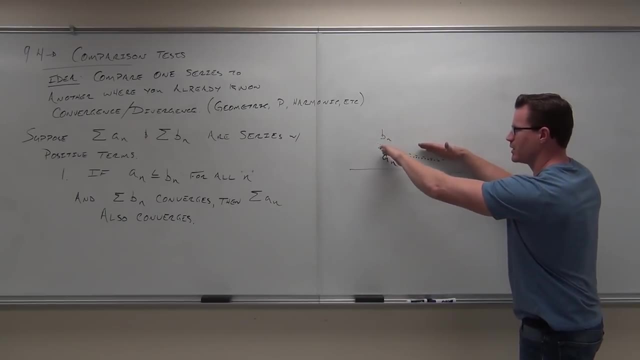 it tells us nothing. a sub n could diverge, It could converge, I don't know, because it's not being forced anywhere. This idea of the series of b sub n converges and a sub n's below it, the series of a sub n, is being forced somewhere. 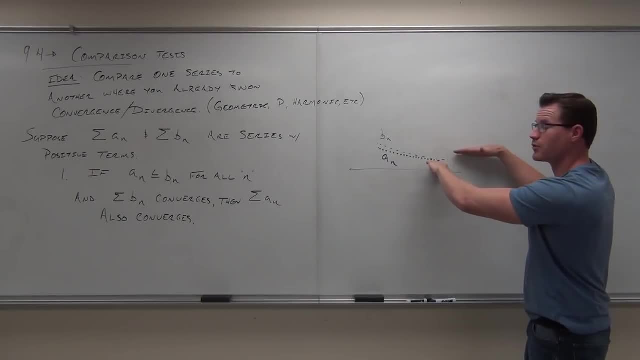 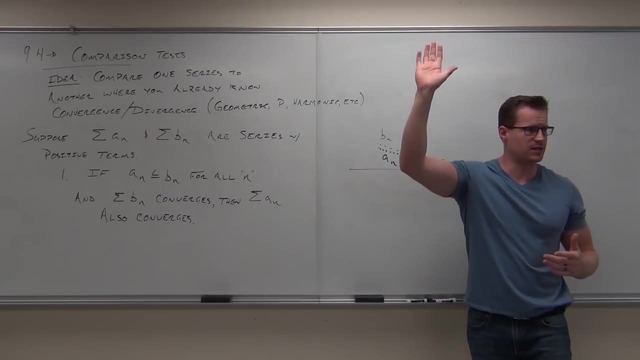 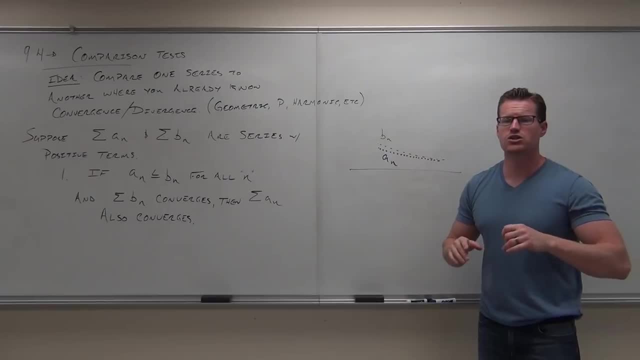 Okay, what's it going to take? What's it going to take to show that a series would be divergent? What would have to happen here to show divergence, b sub n has to be less than a sub n. Oh, hang on. 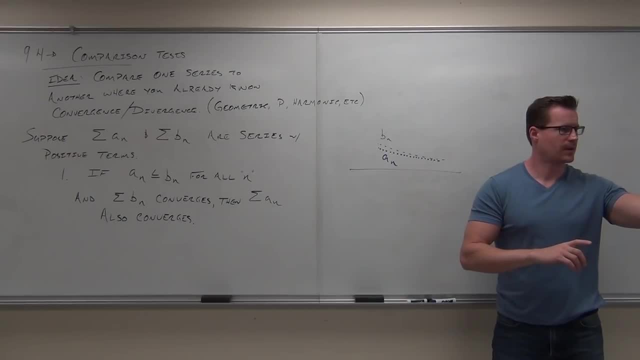 Two people thought: Go ahead, a sub n will have to diverge to show that b sub n is divergent. Okay, I'm going to state it as a sub n is being compared to b sub n. So let's say that right now, b sub n is going to converge. 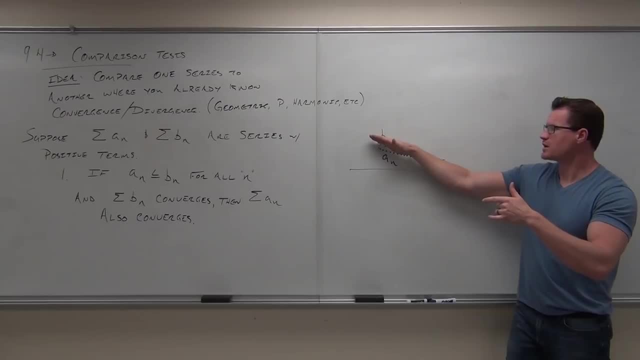 Sorry, we already did converge, didn't we? Let's talk about b sub n diverging. So let's say that b sub n is going to diverge, With a sub n being below it. does that show divergence? No, Where would a sub n have to be in order for b sub n to diverge? 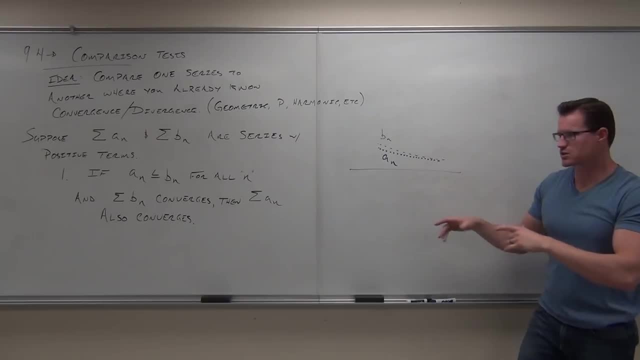 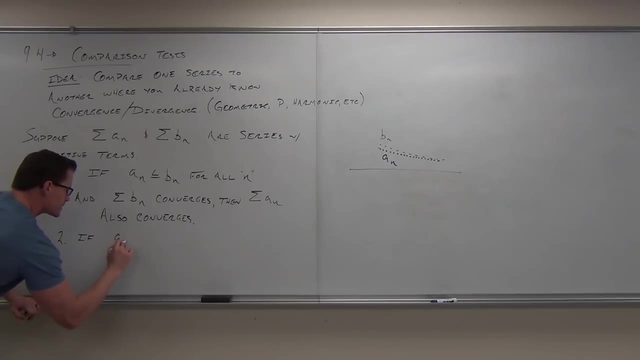 and a sub n must also follow suit and diverge Above n. It's got to be above it, So that's our next case. So if a sub n is always bigger than or possibly equal to b sub n, for all n and the series of b sub n diverges, 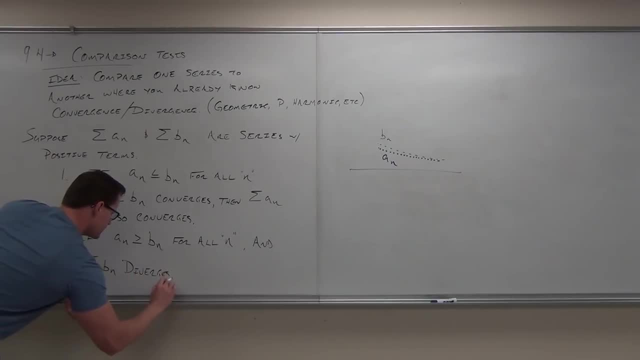 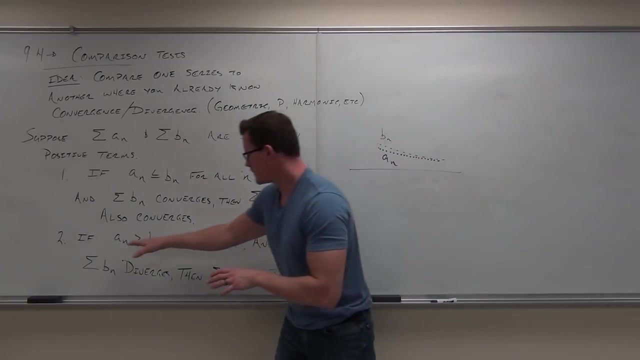 well then, the series of a sub n has to diverge. Here's this case. It says: all right, So start off For every single term. here's b sub n. a sub n is a little bit bigger. Here's b sub n. a sub n is a little bit bigger. 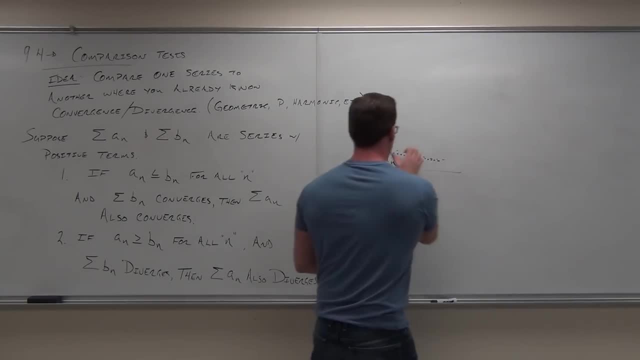 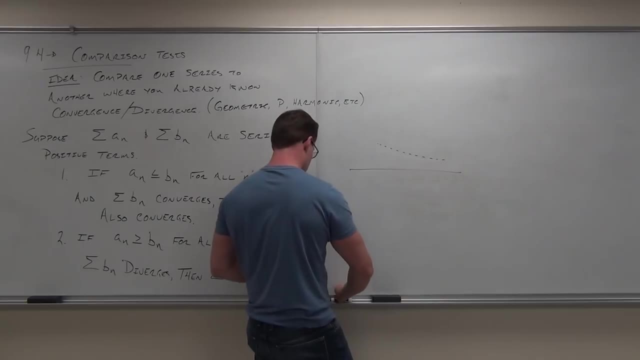 Here's b sub n. a sub n is a little bit bigger, So every single time, Well then, a sub n is not here anymore. a sub n says no, no, no, I'm always just a little bit bigger. 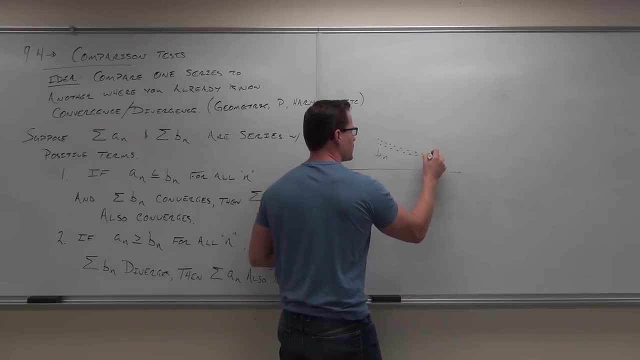 Now I'm up here Term by term. I'm a little bit bigger. Now suppose this Suppose that the series of b sub n is divergent, So this thing diverges, And a sub n is also a little bit bigger every single term. 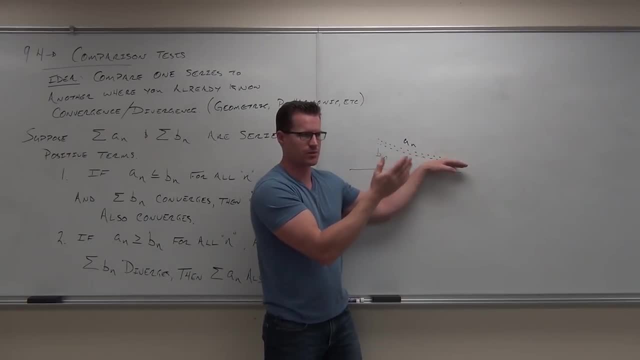 If this thing adds to infinity or diverges or something you know? the series adds to infinity, it's going to diverge And a sub n is a little bit bigger. Where's the series of a sub n going to go? It's going to be bigger than that. 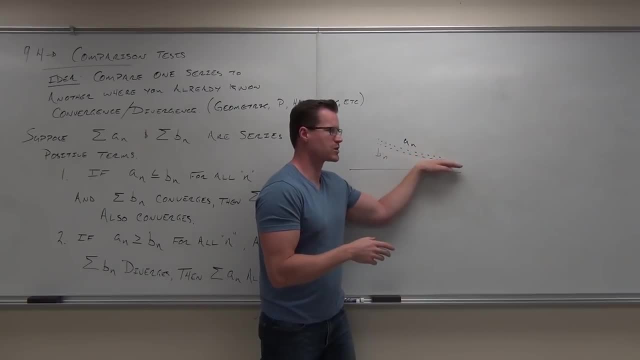 Since it's term by term, bigger. if I add up all these terms and it diverges, then if I add up terms which are slightly larger than that, it's also going to diverge. I hope you understand that idea. So now let's do this one. 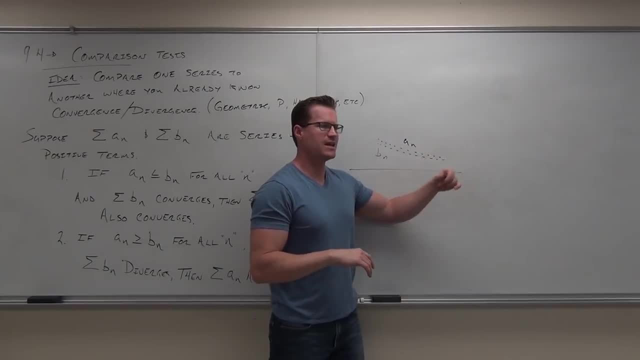 Let's say that b sub n converges. If a sub n is a little bit bigger and b sub n converges, what does it tell you about a sub n? Nothing. It says, hey, this one's bigger than that Great. 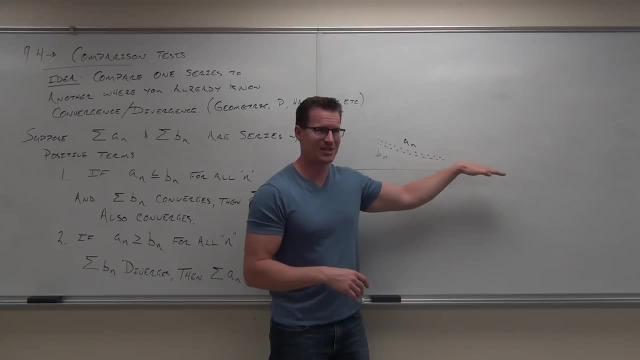 b sub n converges. OK, What's it? tell you about a sub n? Nothing, Because a sub n is bigger. It could converge, I don't know. It could diverge, I don't know. It's not being forced anywhere. 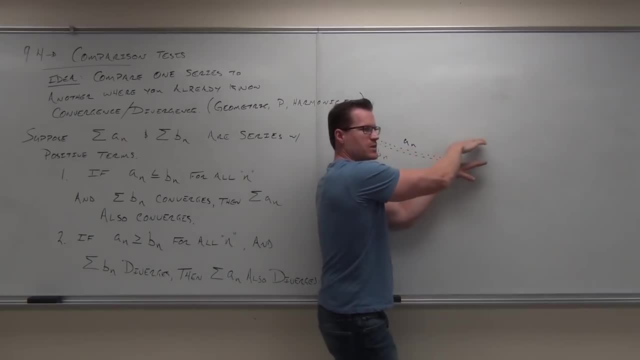 With b sub n diverging, it forces a sub n to also diverge because a sub n is larger than that Show of hands. if you feel OK with that, I like that idea. Would you like to try some examples? You can see the similarity in what we did between our sequences in this. 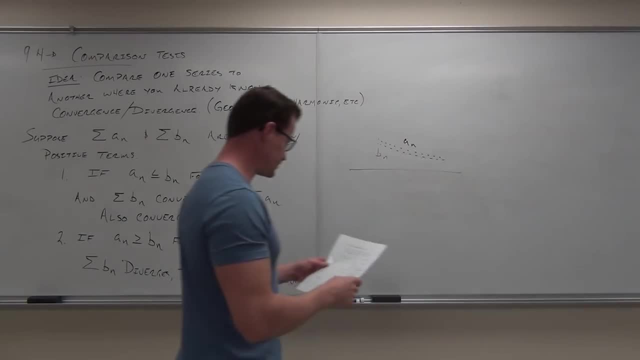 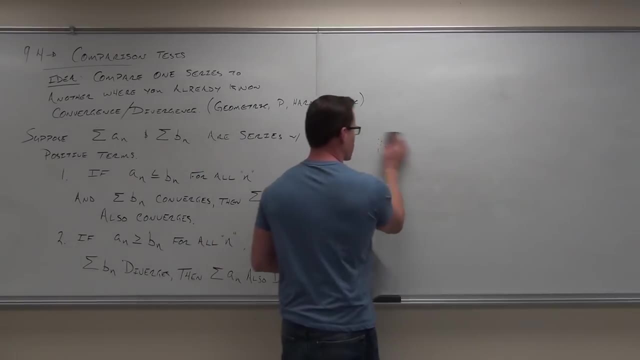 It's really similar. It's just a series. Just had to make a statement here, So let's try a few examples. Are there any questions before we get going on? Hopefully it's going to be pretty straightforward, So let's try one. 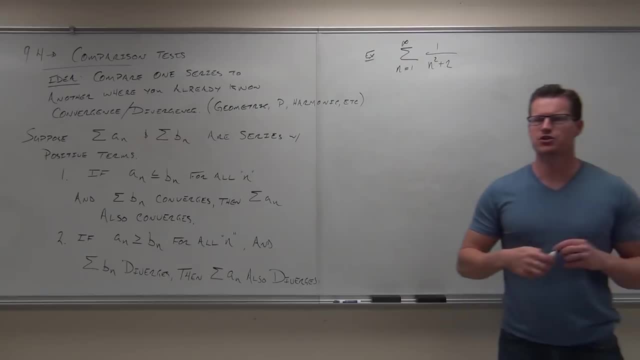 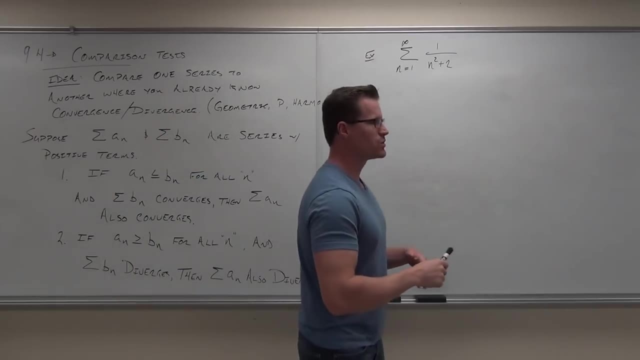 Let's really see if you're with it today. By the way, what's the first thing we should always check with series, No matter what. First thing: We should always check that because it can be really quick. So let's do the divergence test. 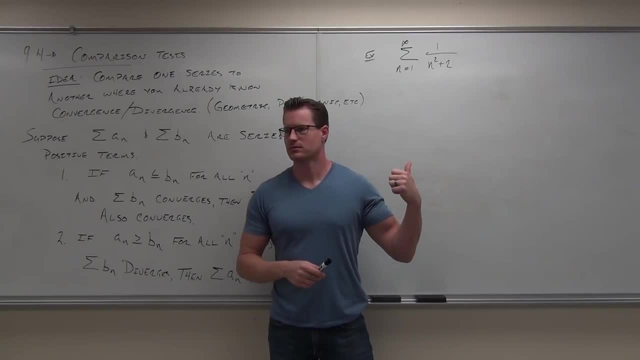 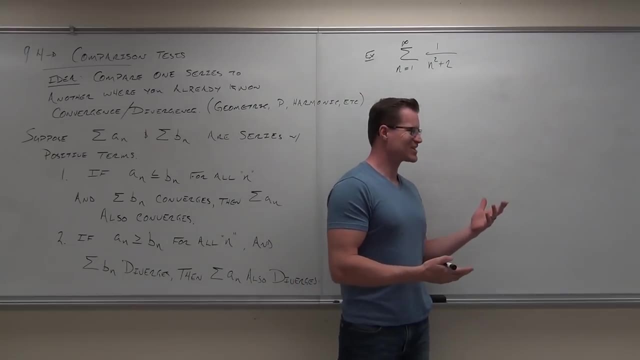 Does that diverge? OK, That's a horrible way to ask that question actually. Are you certain that it might not diverge? That's a weird way to ask it. Does it pass the divergence test? So, basically, is the limit equal to zero. 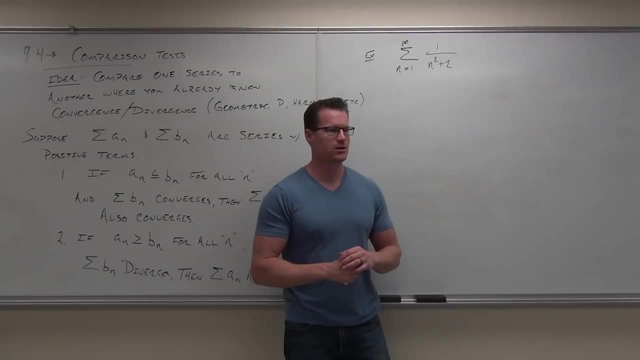 If it wasn't equal to zero, what would you know about this series? For sure, So it might not be divergent- is basically what you know. Do we know it's convergent yet? No, no, we don't know that. 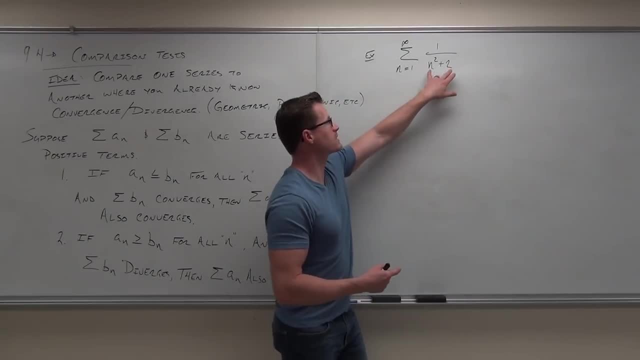 But we know it might not be divergent, because the limit of our sequence, from which our series is built, equals zero as n approaches infinity. You OK with that one? OK, so we check that first. Nextly, we go through a progression. 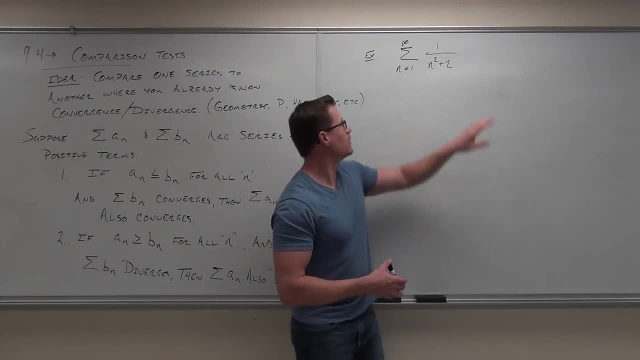 Is it a p-series? No, Would that be a p-series? Yes, OK, You sure Yes, Yes, OK. Say what now? When p is greater than 1? When p would be greater than 1.. So we know something about that, but this is not. 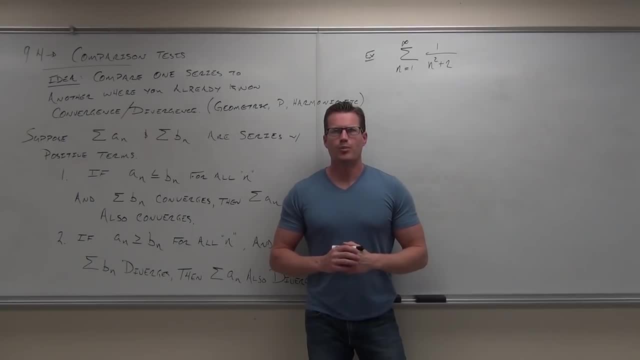 Now, later on, we're going to compare this to something very similar to that. How about integral tests? Could you do an integral test with this? You actually could. It'd be hard to do because that's not a perfect square, but you could still do it. 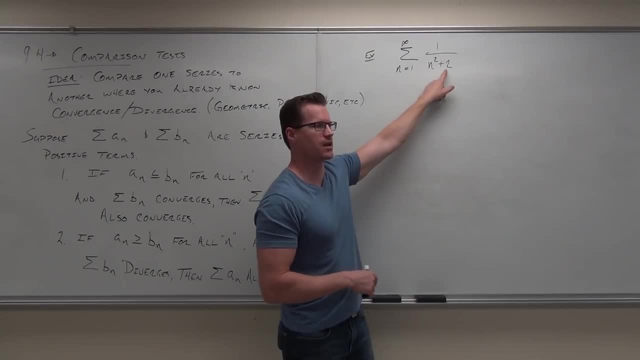 You could do an integral test with that. It's going to be some form of like a tan inverse. OK, if you were to do that- Not such a big deal- You could do that. Is there an easier way to go about it? 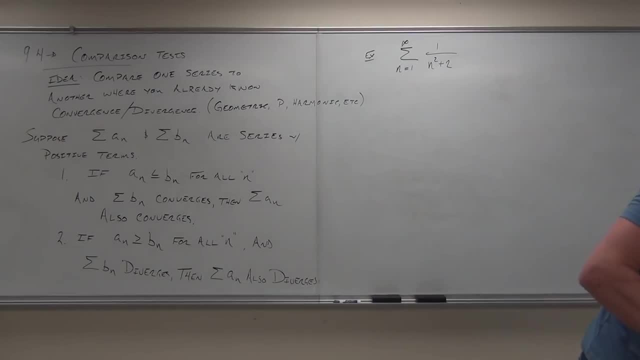 Yeah, Here's the easier way to go about it. Let's compare this to a series that we already know the convergence for. So, basically, here's what we need to know. Firstly, we need to say whether these terms are all positive. 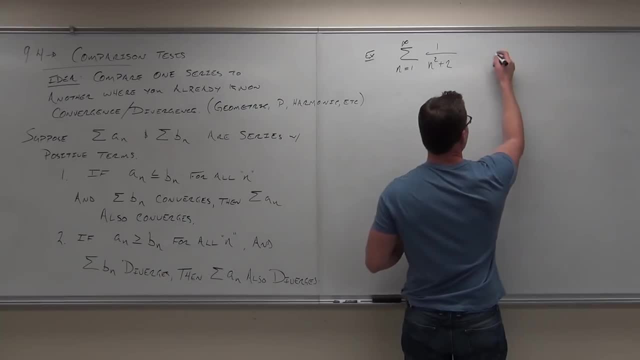 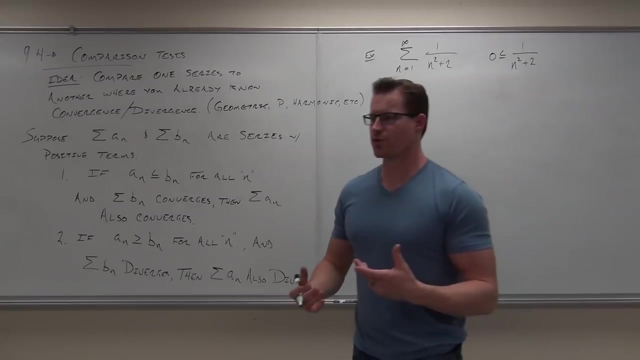 Are all these terms positive? Yeah, OK, So we know that, because all these terms are positive, this is greater than or equal to 0.. And now we're going to base this on something that we already know: the convergence. for If we're trying to show listen, if we're trying to show convergence. 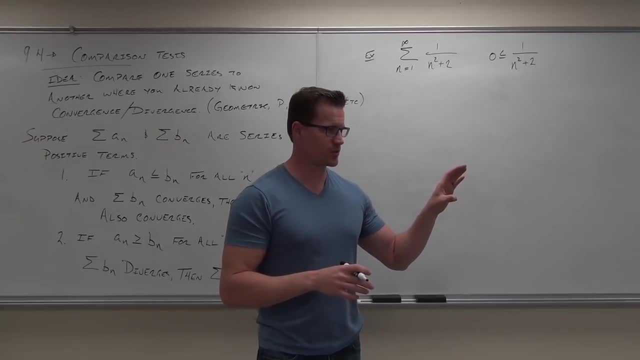 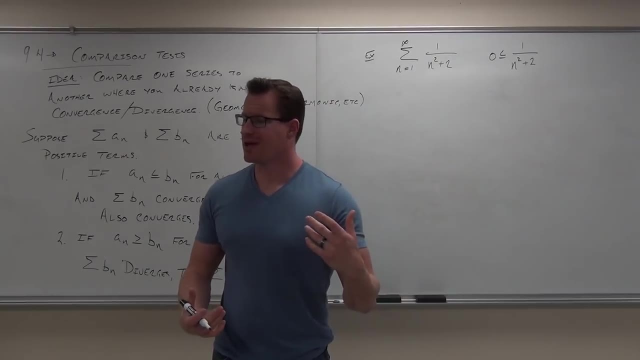 you need to have this as a less than something some series we know convergence, for If you want to show divergence, you need to have this bigger than some series you know divergence, for It's silly to have something less than something divergent or bigger than something convergent. 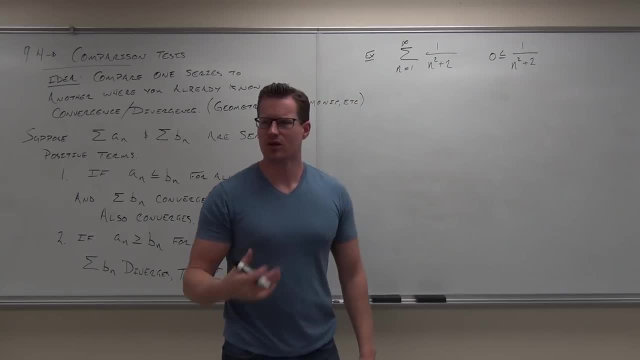 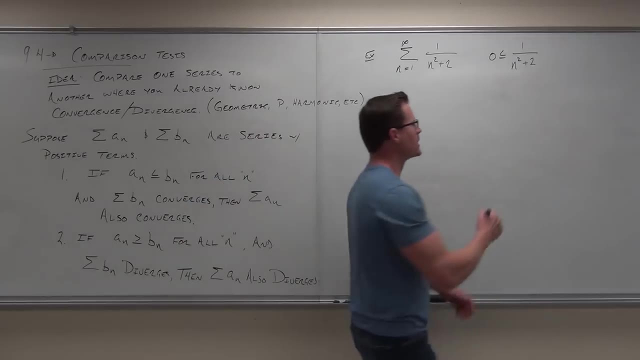 That doesn't show you anything. So what we're going to do is: OK, does that look like anything familiar? And you guys just said it. You said it looks like a p-series, doesn't it? Yeah, Let's make this less than the p-series. 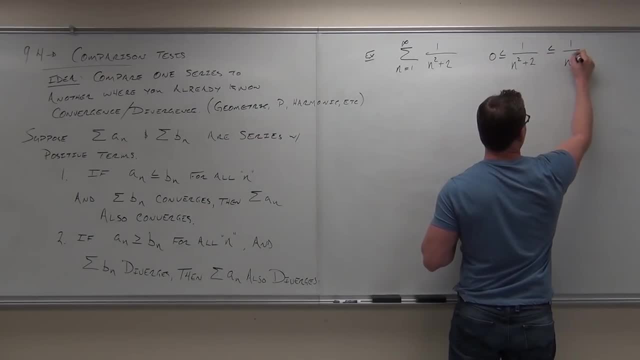 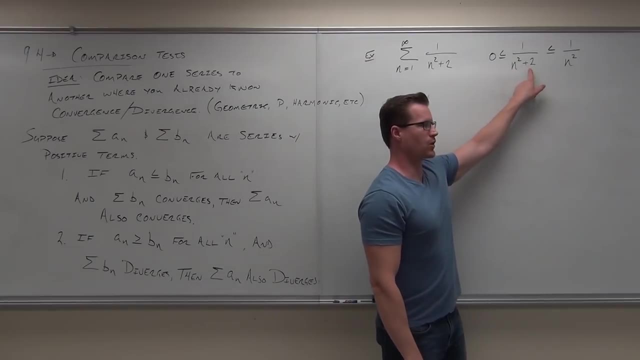 Is this true? Is that true for all n greater than 1?? Yes, Yeah. Well, we know that when a denominator gets larger, our fraction gets smaller, So this fraction would always have to be less than this fraction. You still OK with that one? 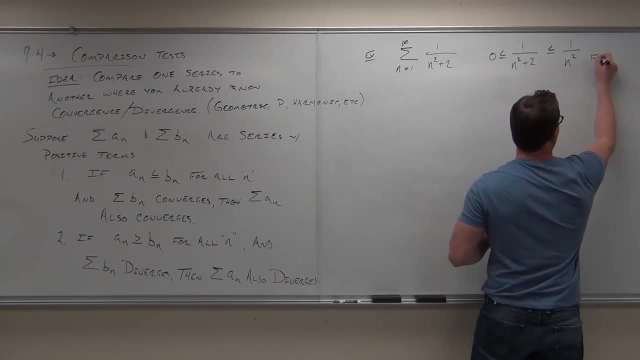 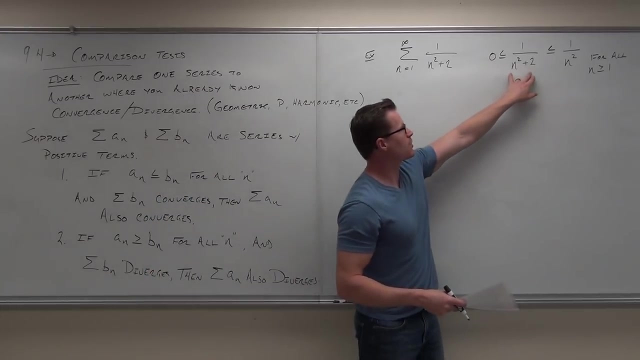 And this is true for All n. Yeah, As a matter of fact, it's true for all n, But we only need it greater than or equal to 1.. So let's go back and see what this says. This says: we're always going to have positive terms, no matter what. 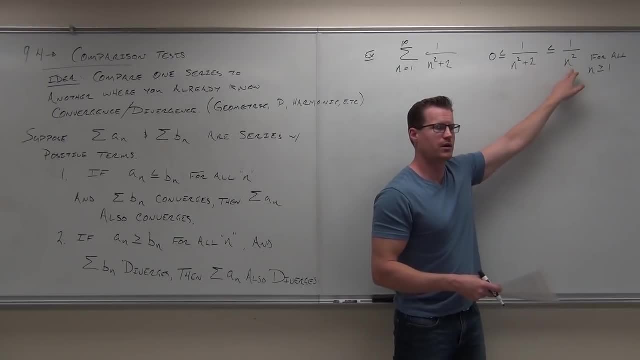 This says that. well, this is a true statement. We're basing this on something we all know: the convergence for right here. This is a p-series That's fantastic. Well, if that's a true statement, then here's what the comparison test says. 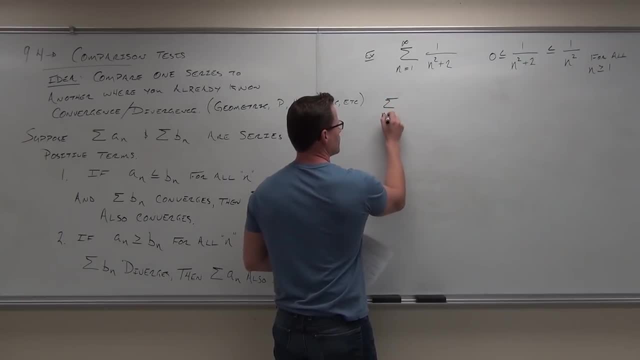 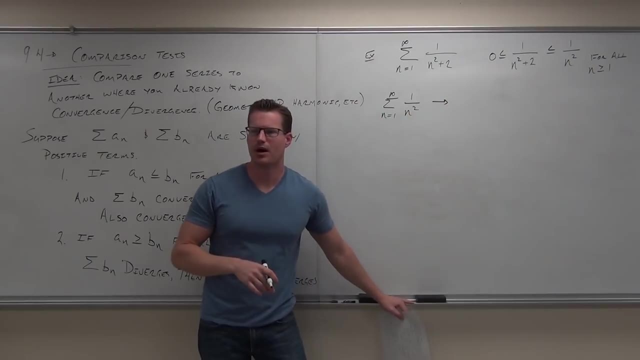 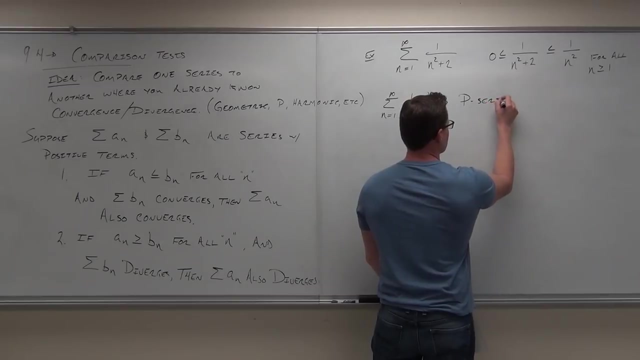 It says: well, do you know this convergence for this? OK, let's go through it one time. What's that called again P-series? What's the p here? 2. So we know that this is a p-series. 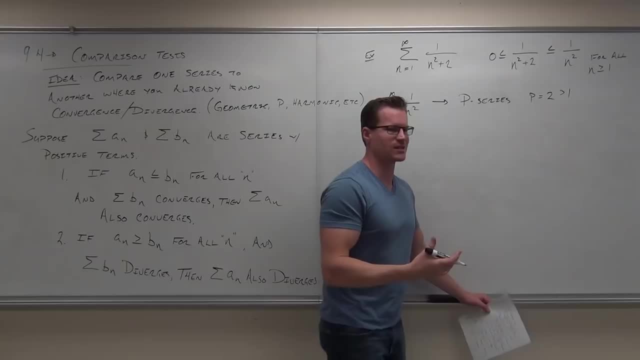 p equals 2.. Hey, that's greater than 1.. That's fantastic. We know that if p were less than or equal to 1, we'd get the harmonic series or something below that. That would be something that would be different. 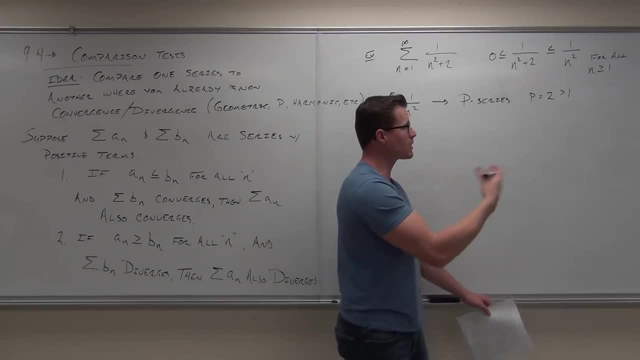 Actually, yeah, above that, as far as sequences go, We'd be divergent. So here we know: hey, it's a p-series, Not a problem. p equals 2. That's more than 1.. Therefore, this series is what. 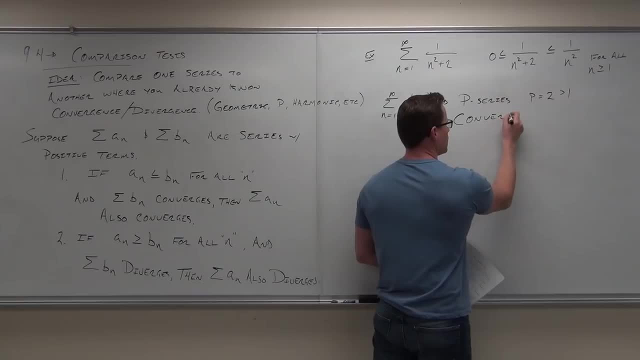 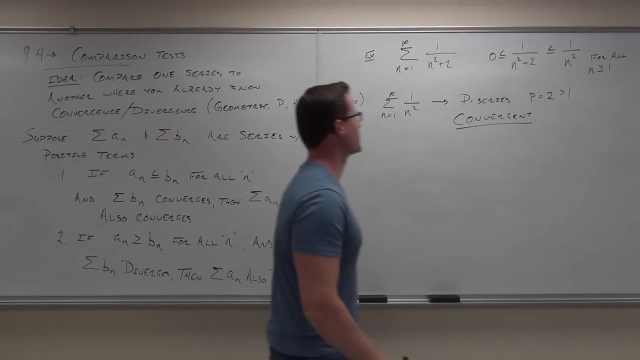 Convergent. Now we're going to put the whole thing together. Put the whole thing together. We start with some series. Yeah, you could do a couple other tests with this, Not a problem. Can we do a comparison test? Well, that depends. 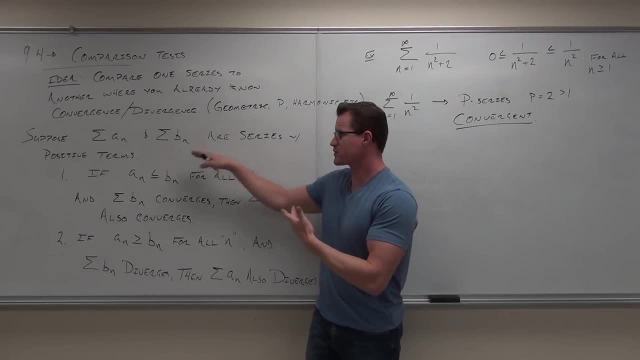 Are all your terms positive? Yes, Yeah, it says right here: you've got to have positive terms. So all our terms are positive, No problem, Is it less than a series that you know is convergent? That's what you ask now. 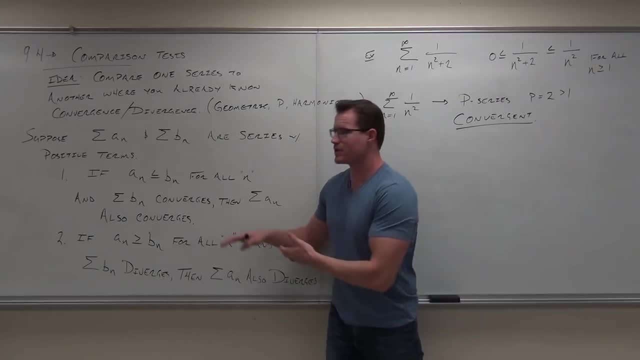 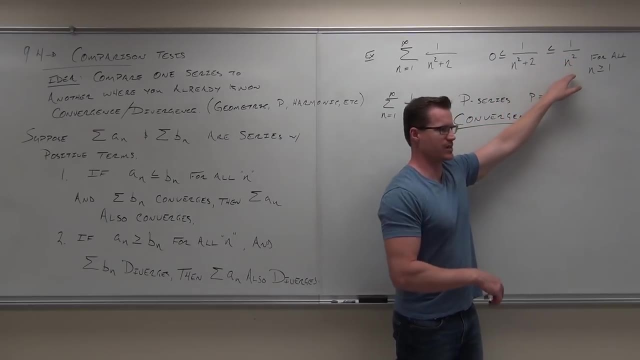 Is it less than a series you know is convergent, Or is it bigger than a series you know is divergent? In our case, I know that this thing is less than 1 over n squared. It has to be that way because I'm just taking my denominator and adding 2 between this fraction and this fraction. 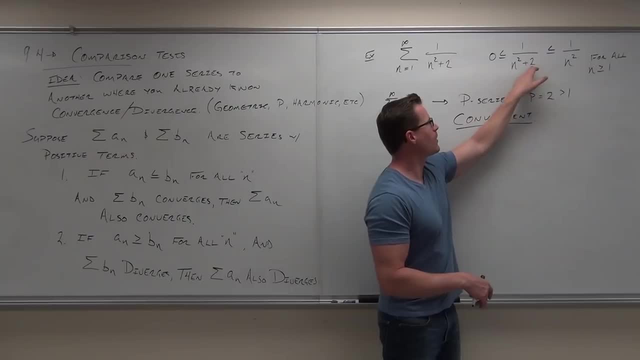 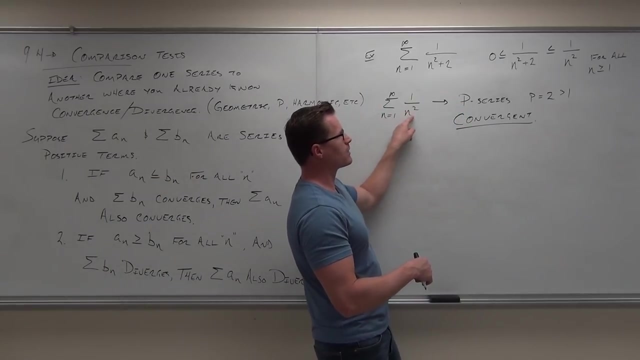 between this sequence and this sequence, or likewise our series and our series. So these are always going to be less than these terms For every single one: term 1, term 2, it's always less than that. If it's always less than our series we know is convergent, well then we've got to look at that thing. 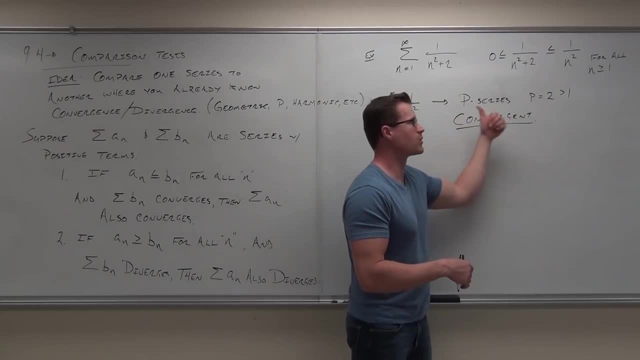 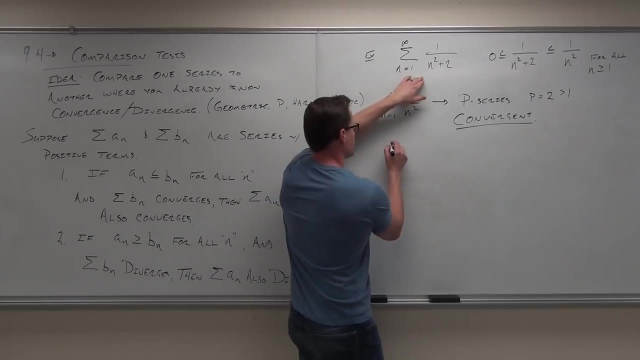 The series of 1 over n squared is a p-series. We know that p is equal to 2.. That's more than 1.. That shows convergence. So what do we know about this series as well? It also converges. It also converges. 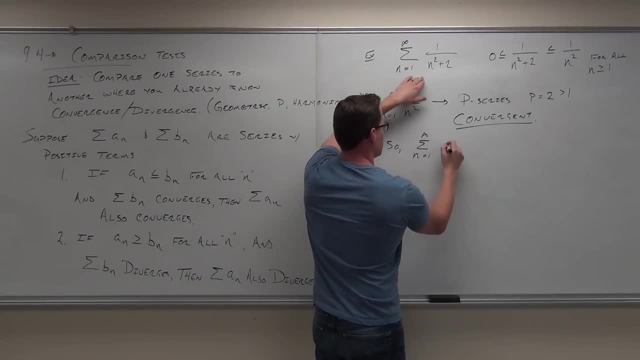 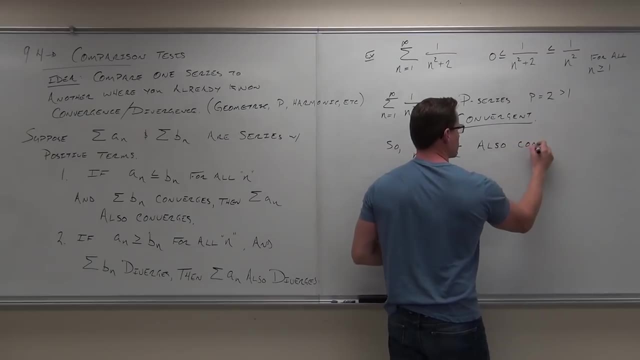 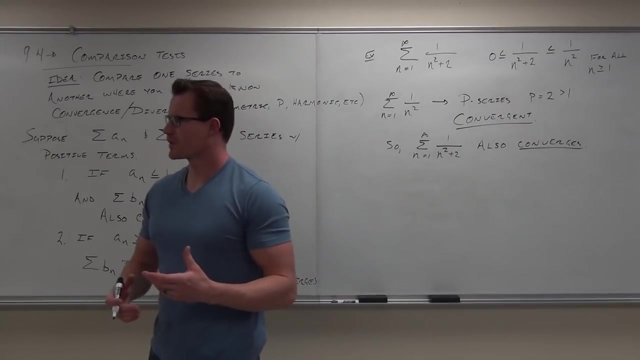 So Our series of 1 over n squared plus 2 also converges. I want to make sure you guys really understand this before we go any further. Did that make sense to you? Show of hands. if it did, I feel okay with that. 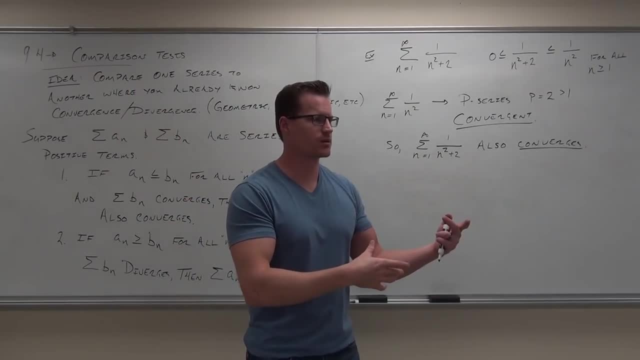 So, basically what we're doing, we're comparing one series to another. We're comparing it to make it to show whether it's convergent or divergent by saying: well, if it's below one series, that converges, our series converges. 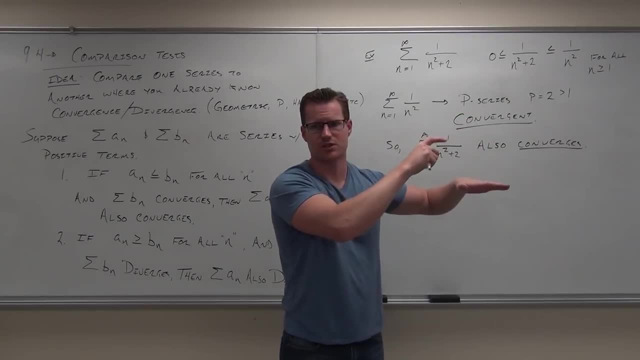 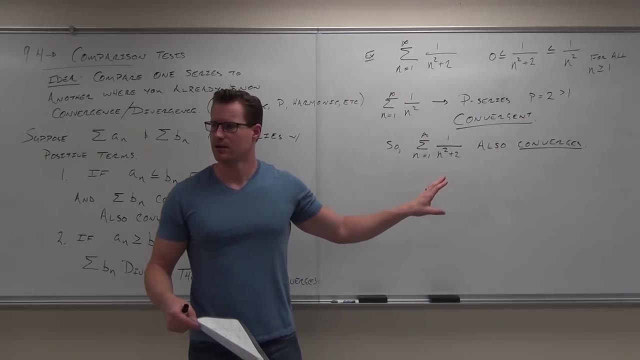 If our series is above one series that diverges, our series diverges as well. That's the only two scenarios that we can really have. There's only two cases. Have I explained this one well enough for you guys to get it? Can we move forward? 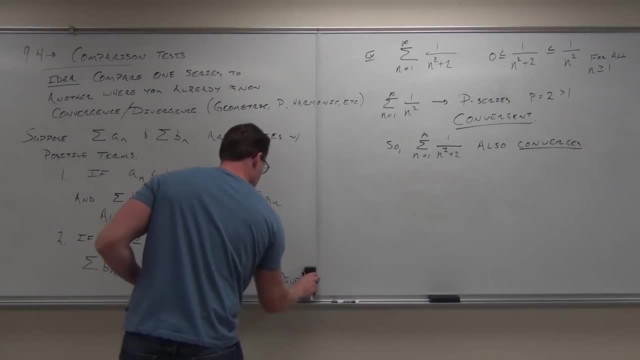 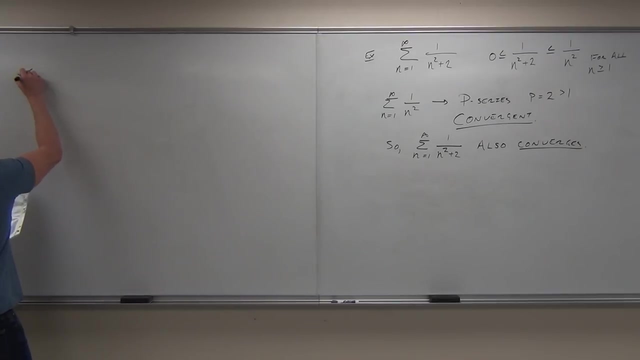 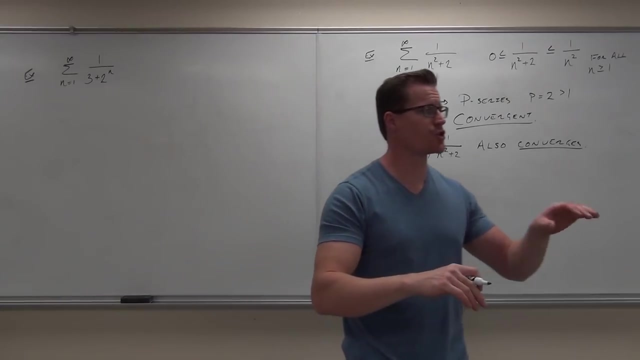 Let's try a couple more. Okay, Let's give this one a try. Let's start from the very beginning with all of these series. Really go through the progression. What's the first thing that we try any time we get a series and we're trying to show convergence or divergence? 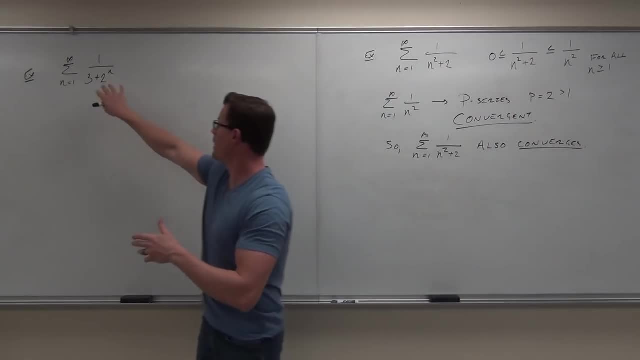 What do we test first? Convergence. Okay, So we're going to take a limit of this thing. Does the limit of this thing equal zero? Yes, If it didn't, we'd stop right there. If it does, hey, we're good to go. 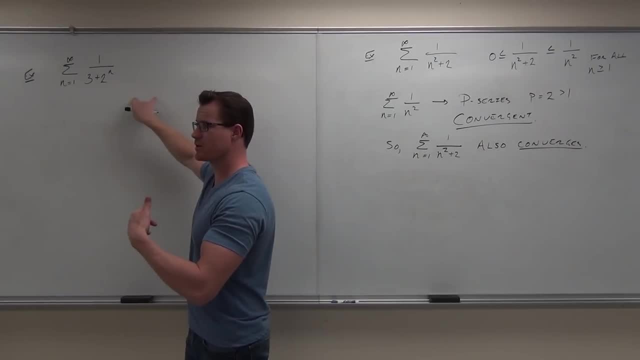 Let's continue with this thing. So it says, hey, the limit of the sequence goes to zero. That means that potentially, we could be possibly not divergent. We've got to show that, though. We can't just stop right there. 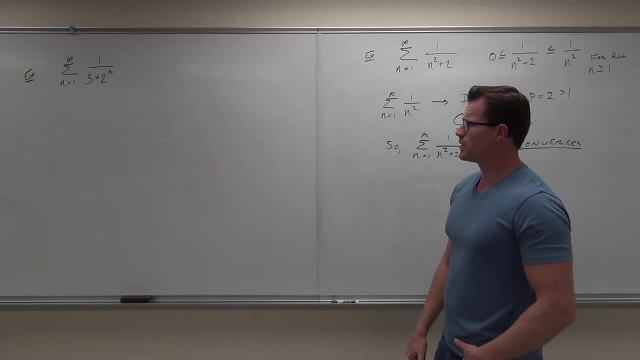 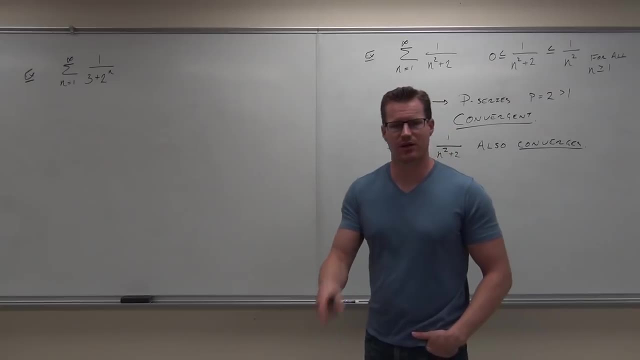 It doesn't show convergence. After that, man, we go through our list of things to do. Could we do integral tests? I don't know. Maybe, But it's probably a little bit easier to do a comparison test right now. Here's why I see that. 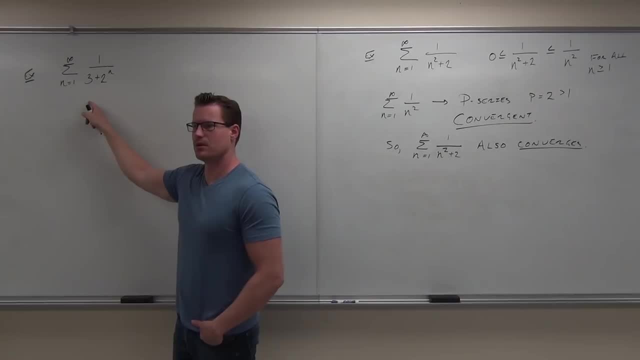 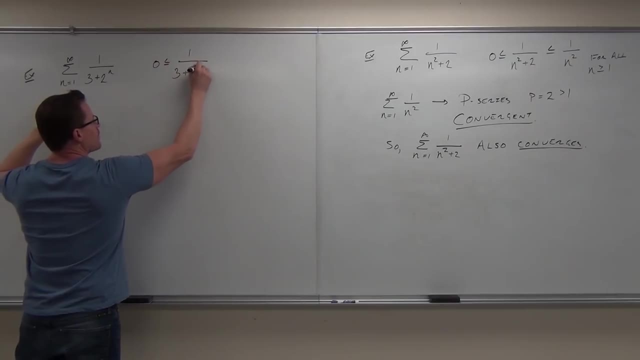 The first thing I see are my terms positive all the time. Okay, Well, that's one condition We've got to have that for a comparison test. So I know that we have. all my terms are positive. Second thing I'm thinking about is this: 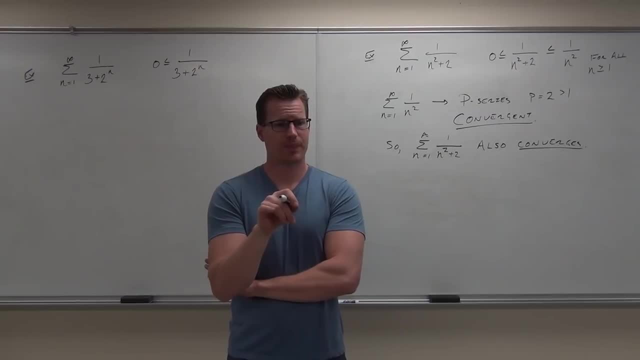 Can I show that this is either greater than some series which is divergent, or less than some series which is convergent? Can I show that I don't know? Can you show that I can show that I know how to do it? 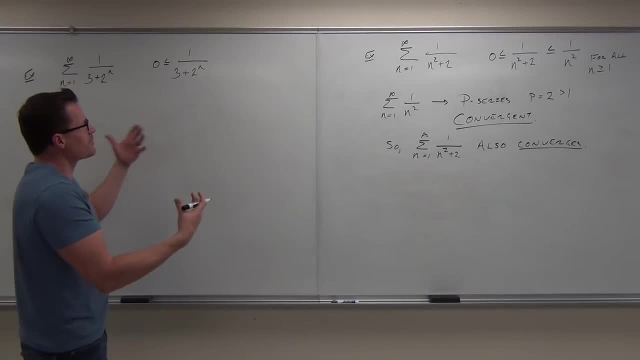 Here's what I'm thinking. I'm thinking that the one thing about this is that three is kind of holding me back here. Does that make sense to you? So the reason why the comparison test is so nice is that, if you haven't noticed, 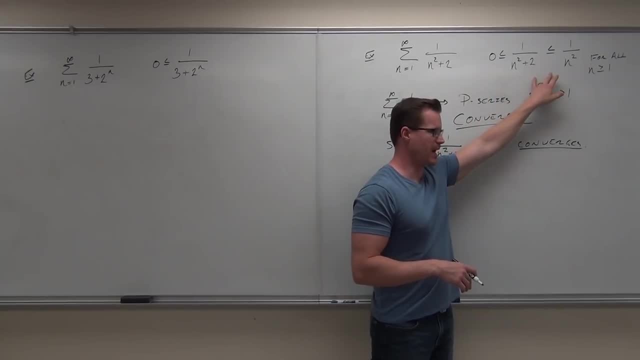 this already. it allows you to get rid of little pieces which are holding you back. So you go: hey, that plus two, that plus two is holding me back, man, Let's get rid of that. Well, if I have a plus two on my denominator, it's going to be less than one. 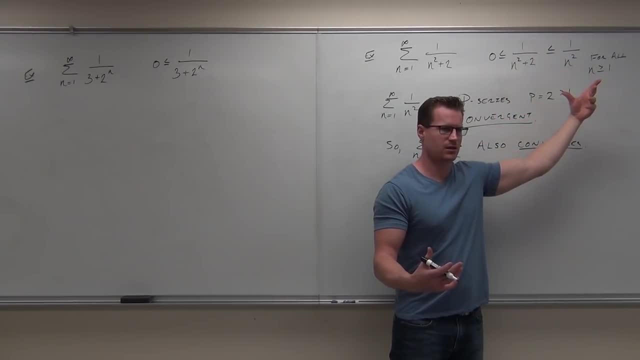 over whatever I have without that plus two, Does that make sense? Now here's the little kicker for you. What if it was a minus two? Yeah, that would be a problem, because here that would be a minus two, That would be a greater than. 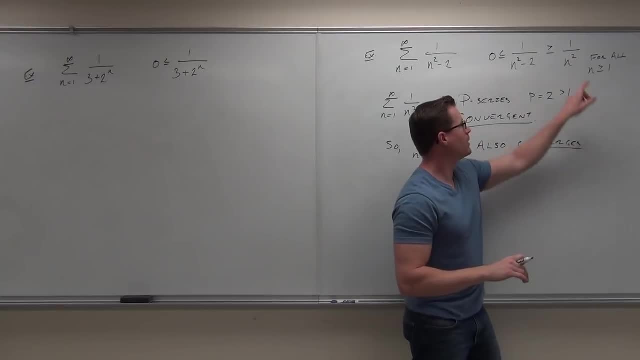 OK, stick with me here. I'm going back to this example. Now, look, we know that this series converges, don't we? But that series is bigger than this. This double inequality makes absolutely no sense. So this is bigger than zero. 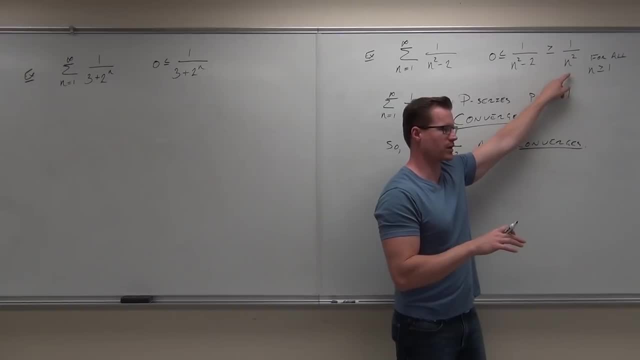 OK, this is bigger than that. So I can't use a squeeze theorem- if you're thinking squeeze theorem right here- because I don't have my double inequality set up the correct way. This is all right, Those are positive terms, Fantastic. But now this series is bigger. 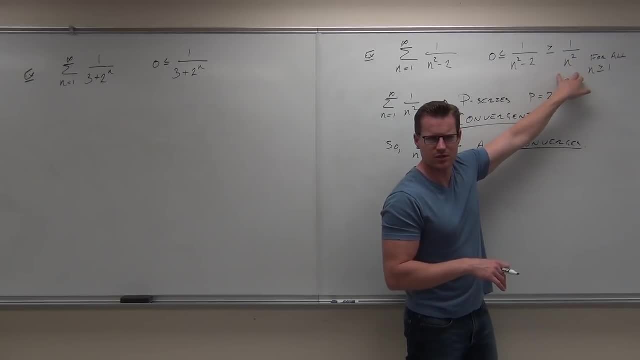 It's bigger than this one. This one- I'm sorry this one- converges or diverges. Tell me something about a series which is bigger than a convergent series. Does it tell us anything? That would be a problem. We'd have to do something different with that. 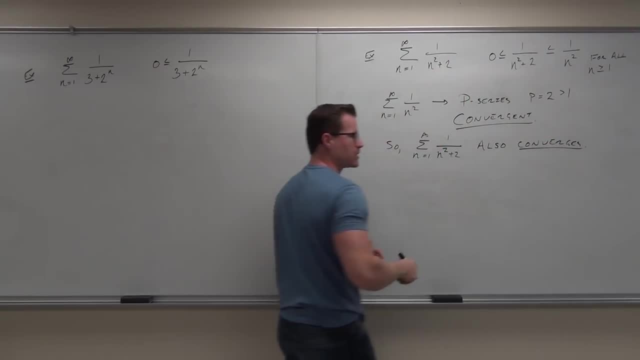 But if we have the plus man, we're all set up. We're good to go. In our case, do we know that this is less than or equal to some series? Less than what? One over two to the n? You know, I mentioned the squeeze theorem about five seconds ago. 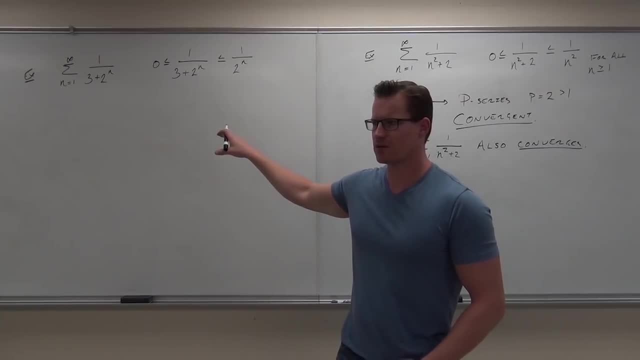 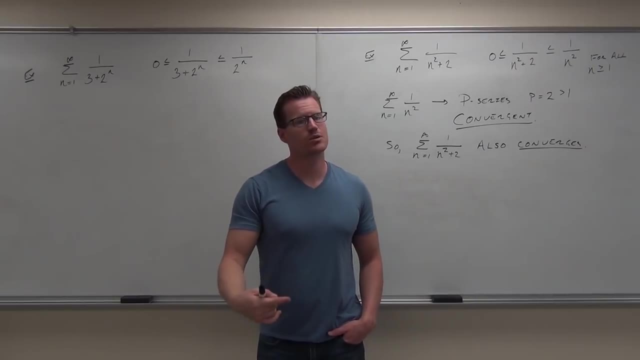 Do you see that essentially we can use a squeeze theorem here as well? Limit of zero is zero, Limit of this thing is zero, Limit of this goes to zero. We actually did use that for sequences. Now the series is a little bit different, but basically the idea is about the same. 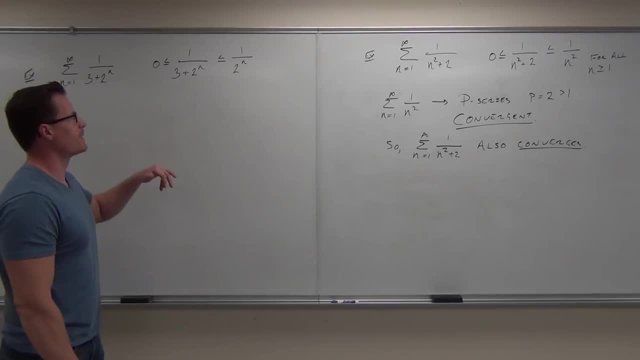 as far as comparing them. So with comparison tests, we set it up. All we have to do now is determine whether this thing converges or diverges. Let me make another point for you here. If this were divergent, would it tell you anything about this? 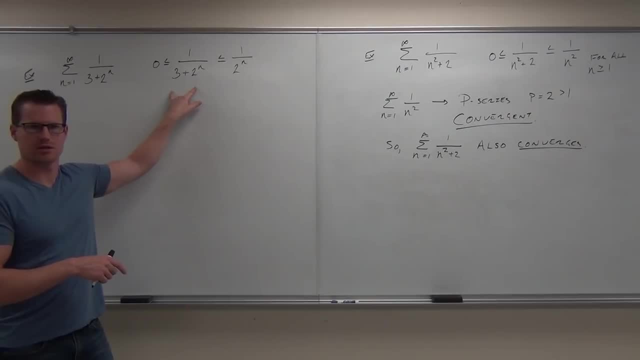 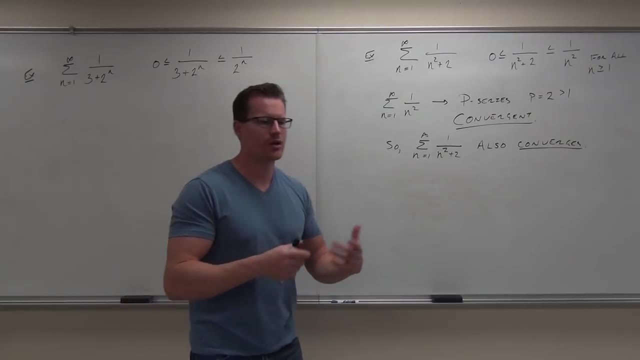 If this is convergent. would it tell you anything about this? So we want to see if this is convergent or not, Is it? You've got to show it to me, You've got to show me. So let's talk about the series of one over two to the n. 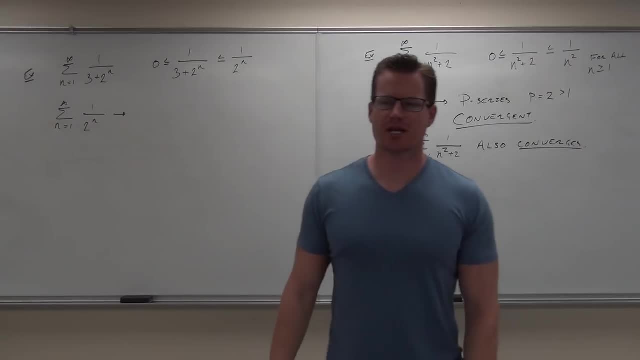 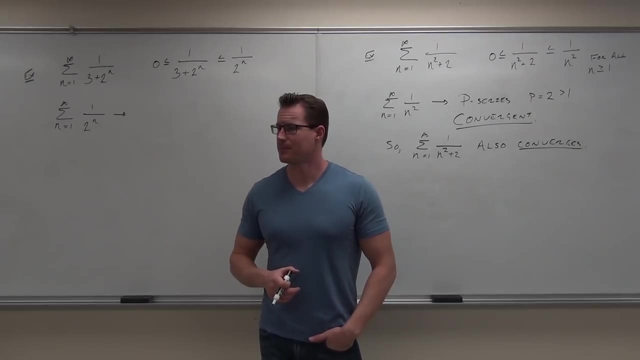 Tell me how that thing is convergent. Tell me why, And don't just say, well, if I take the limit, it's zero. You can't do that. Say what now. n is always increasing. That's true. Explain that. 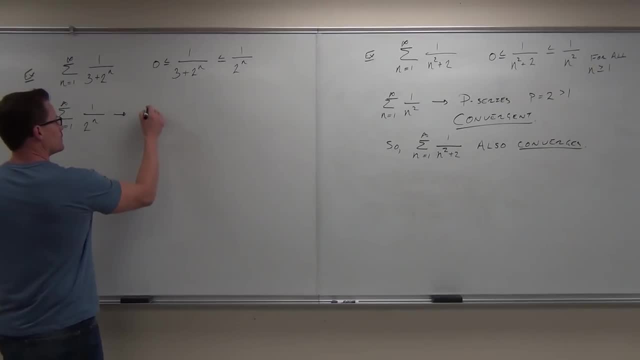 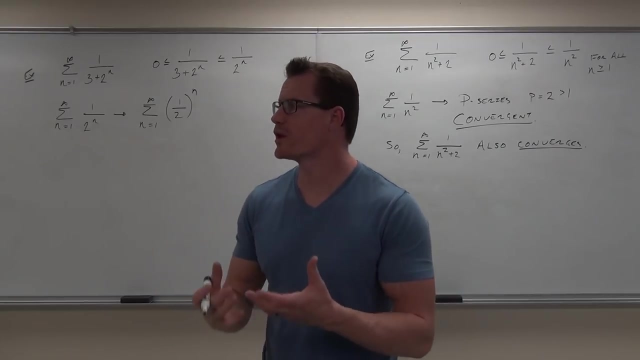 Well, you can make the whole thing to the n power and then take out one half, OK. So if I did this, is that still true? Guys? remember, you're not trying to read me at the wheel here, right? You're trying to base these on series that you already know. the convergence for 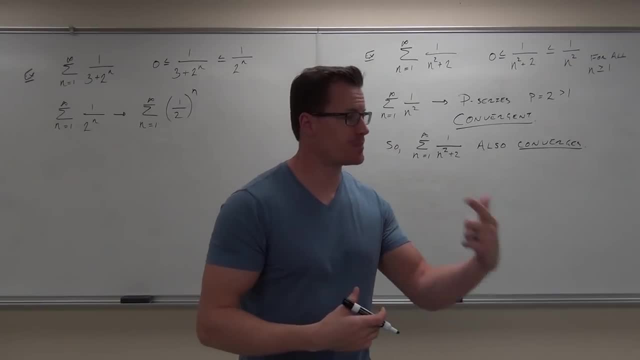 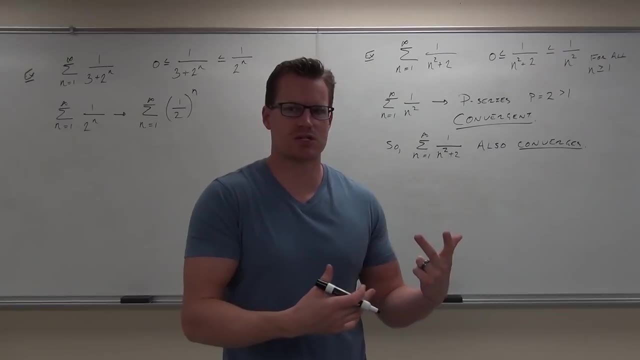 That's why I put it at the very beginning: Base it on a geometric. Base it on a p-series. Base it on harmonic series. Base it on one of those things. Does that make sense to you? You can do the integral test for some of these and that would work. 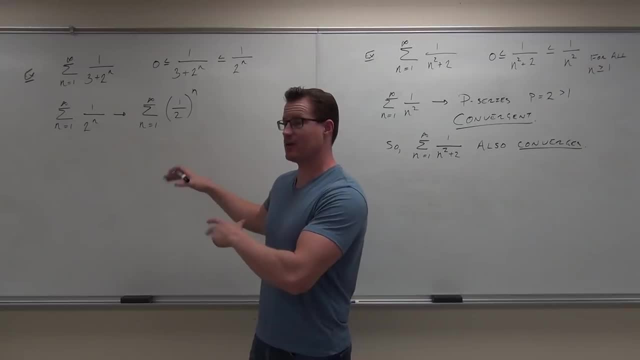 Sure, But it's easier if you base it on things that we already have. If you can do that, Quick head nod if you're OK with this, so far, OK, cool. Well, we know that our terms are positive. We know that our terms. 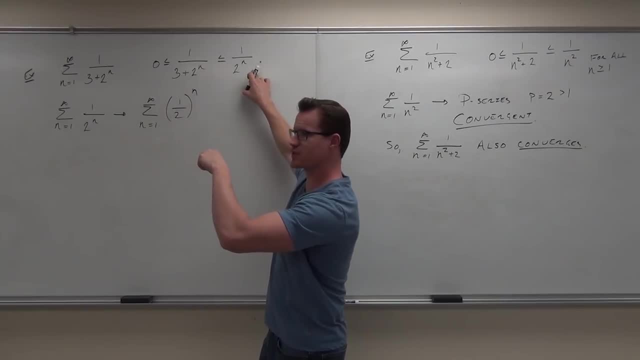 Term by term, this is going to be less than this one. Now, this is great news for us, because we know something about the series of 1 over 2 to the n. The series of 1 over 2 to the n is the same as the series of 1 half to the n. 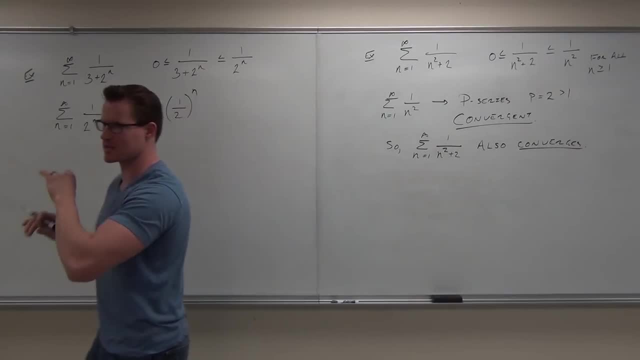 Oh, that's fantastic news. Why is that fantastic news? What type of series is that Geometric? Now, because it's geometric. we can immediately determine whether this thing converges or diverges. Now, what I told you a long time ago, a few lessons ago, 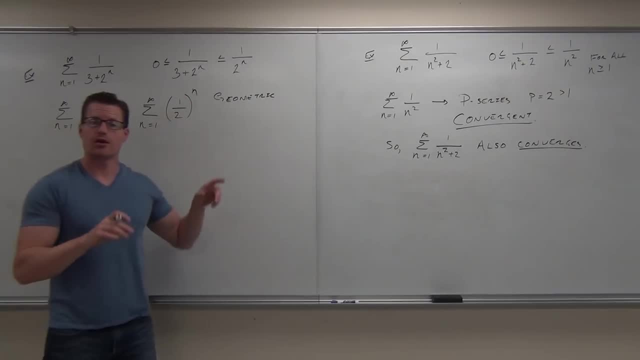 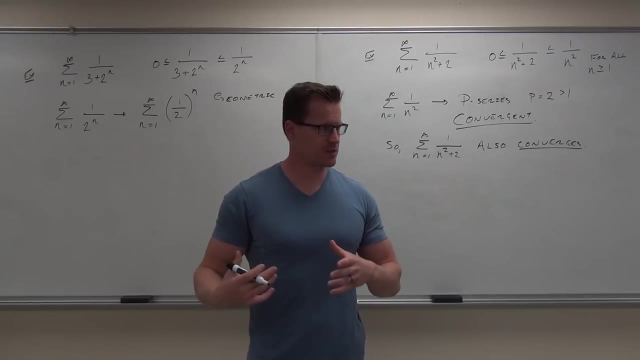 was that this and this have to match. Now, that's true. if you need to find the sum, Does that make sense? Are we finding the sum of these series? No, So do I care? Not really, I don't really care. 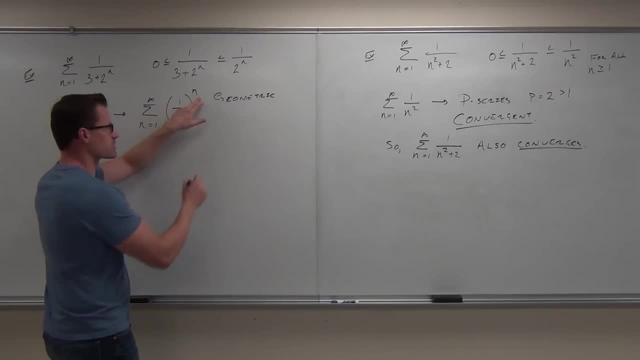 You can but notice that if I pull out a 1 half to match my powers, If I pull out a 1 half to match my powers, remember that, whatever this is, you have to match it: 1 minus 1,, 2 minus 2,, 3 minus 3.. 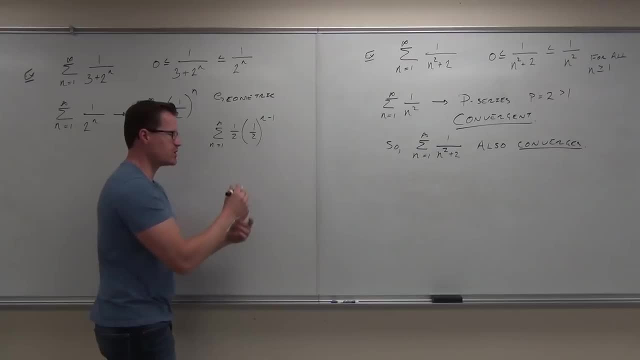 If you were to find the sum, because remember what the sum of a geometric is- it's a. that's your first term- over 1 minus r. I've already covered this. You can refresh your memory on that lesson as you want to. 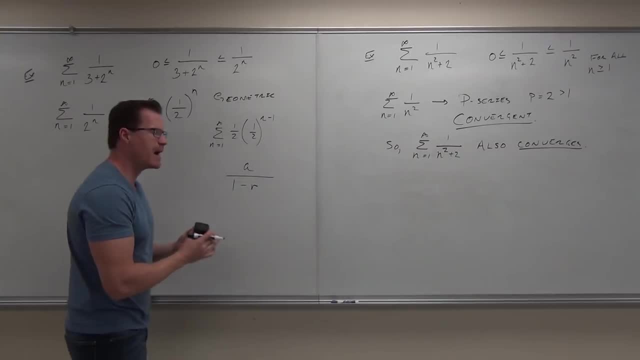 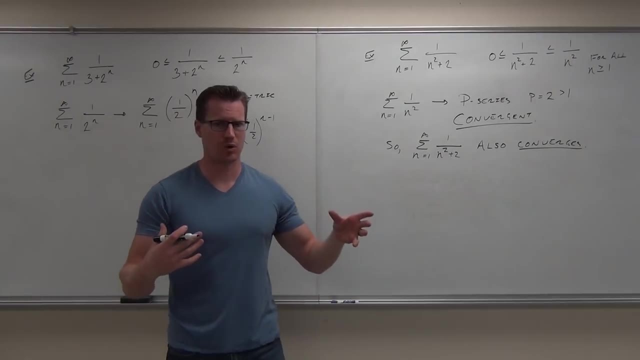 But since we're not finding the sum, it doesn't really matter as far as convergence goes. The reason why it doesn't matter: once you have this to a power, I don't care how many of those factors you pull out. That 1 half ain't changing. 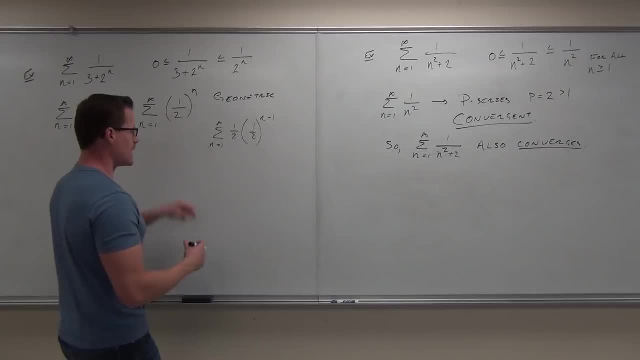 Does that make sense? So all we're really looking at now, not really the a, don't really care about it. What I'm worried about is the r. How much is the r? Absolute value of r is 1 half. 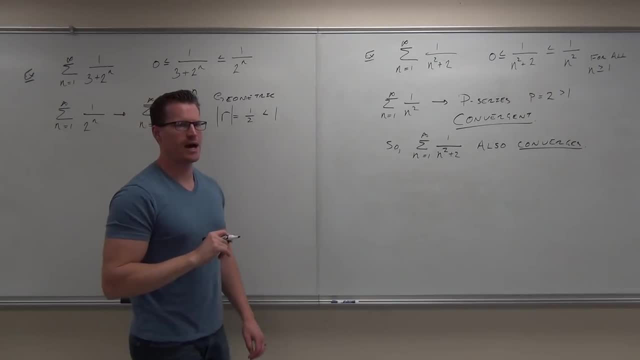 That is less than remember that if we have the r- absolute value of r less than 1, tell me something about that geometric series. That's perfect. So, because this is a geometric series with r is less than 1, absolute value of r is less than 1, this thing is convergent, or this converges? 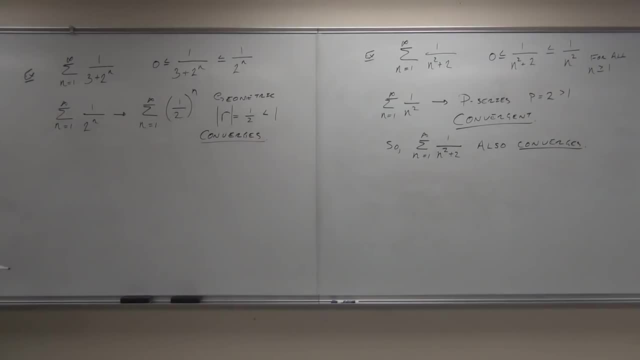 I'm hoping that you understand the reason why I'm not matching my powers. Do you understand why I'm not matching my powers? You're not trying to find the sum. Not trying to find the sum, Don't really care about it. Okay, so let's refresh, because on your test you are going to have to find the sum. okay, 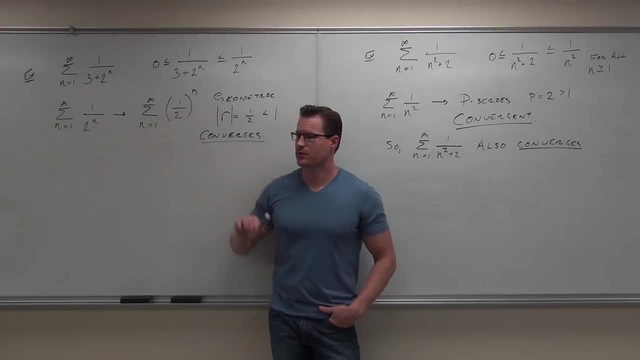 If you did have to find the sum, would this be good enough? No, Now you could do this. Remember, I gave you a shortcut. I said: if you had to find the sum, you just think about what your first term would be. 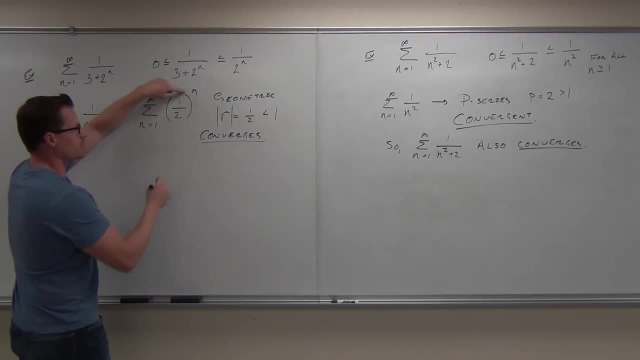 Your first term would actually be: if I click in 1, your first term would be 1 half over 1 minus 1 half. Does that make sense? That's how you do it really fast. No matter what that is, even if they don't match, it's your first term over 1 minus r. 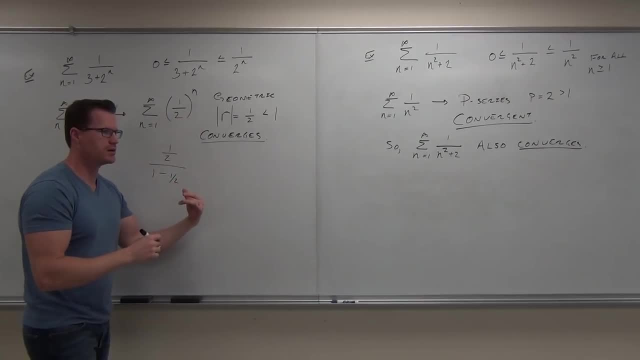 Not a big deal. If they do match well, you get to use your a. It's a over 1 minus a is your first term Always. you can take your first term over 1 minus r. It's not a big deal. 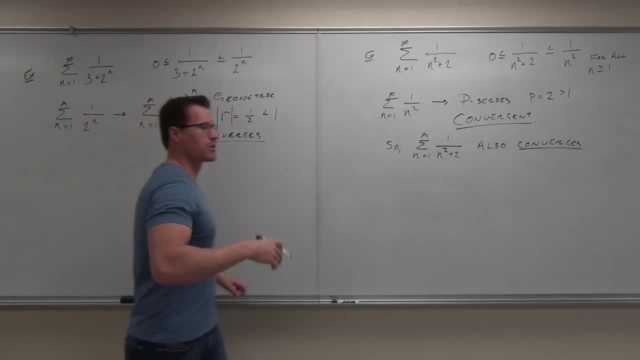 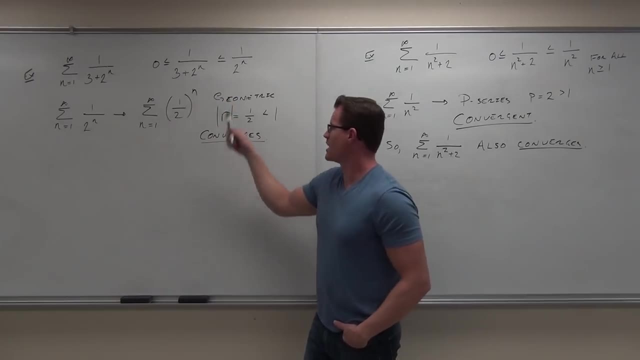 I covered it in a previous lesson. You can go back and check that. Now let's keep going with our current problem. So we start here We go. cool positive less than 1 over 2 to the n. That's a geometric series. 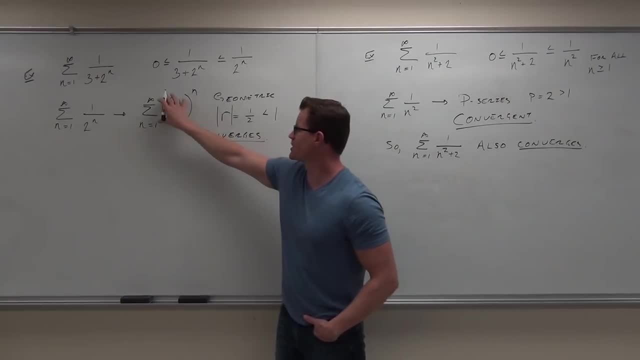 That thing has an r of 1 half, which is less than 1.. It says that this series converges. Tell me something about the series that I'm given. It also converges Why? Because it's less than 1 over 2.. 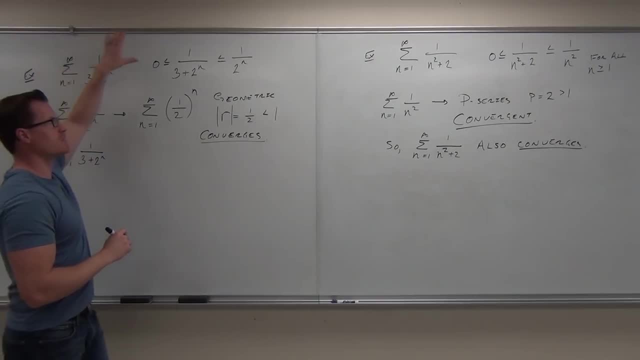 Very good. The series we're given is less than or equal to some series that converges. By the comparison test, that means that this series also converges. It's less than or equal to some series that converges. Is it still making sense to you? 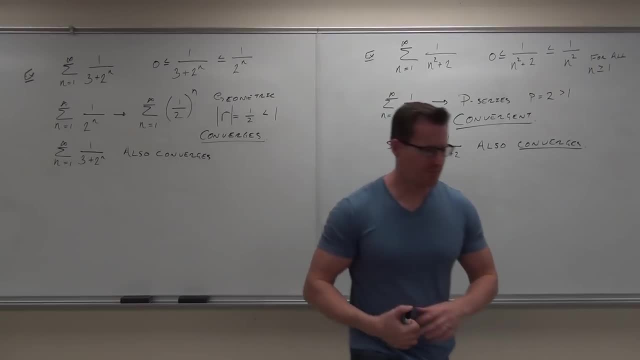 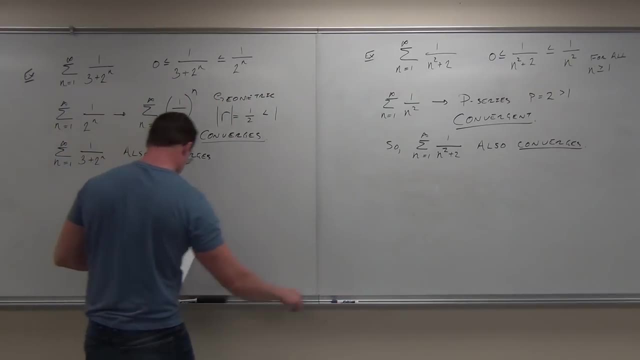 Is it interesting to you? It's similar to what we've done before. I think it's kind of interesting, kind of fun. Tell you what. we'll do one more and we'll talk about something slightly different. Would you like to try one? 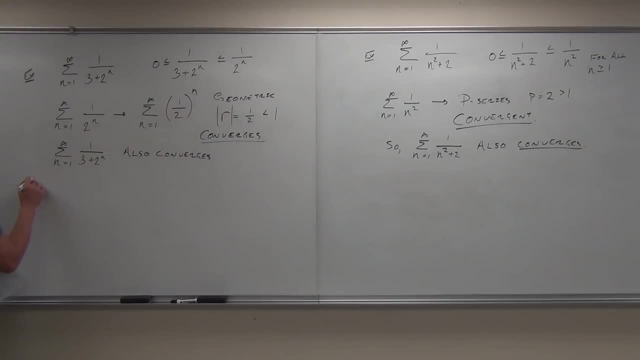 I'll give you about two minutes to see if you can manage to figure this one out. If not, no big deal. So here's what I'm asking you. I'm asking you to firstly determine whether these terms are all positive. You have to show that. 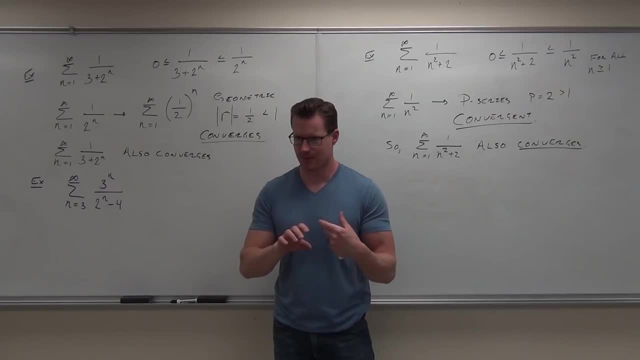 So the comparison test works when both of our series have positive terms. So show me like this that our terms are always positive and make sure that you're right. Notice that this does not start at 1,, it starts at 3.. 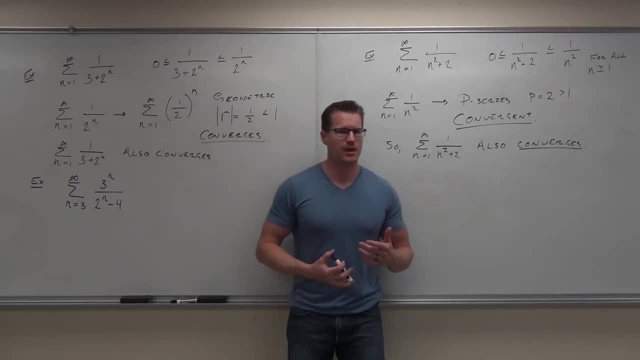 So show me that we have positive terms. Next thing: determine what is going to work here, whether this should be bigger than or smaller than a given series. Remember that if it's smaller than a given series, that series must be convergent. 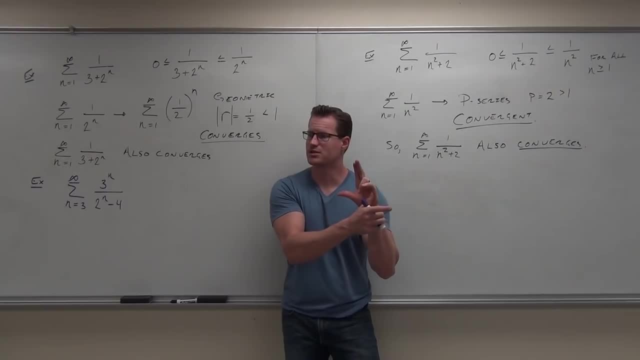 If it's bigger than another series, that series that you're basing this on has to be divergent, So pick the correct one. See if you can do it. Everything in this video is still going to be convergent, So you can find all the answers if you don't get everything right. 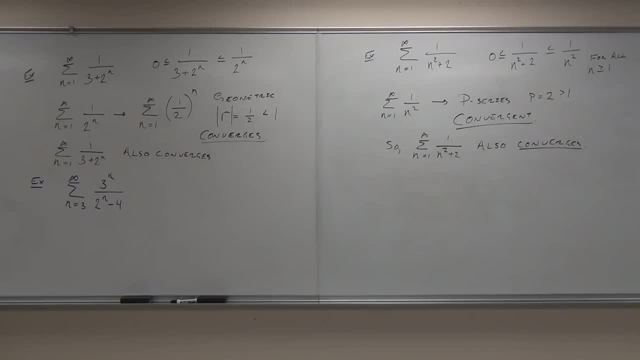 You know, the relationship is all about the result. It's not just the result. You can figure out the answer by looking at your own test results. But you have to try to figure out what you see in the final results And not just by looking at your sobie. 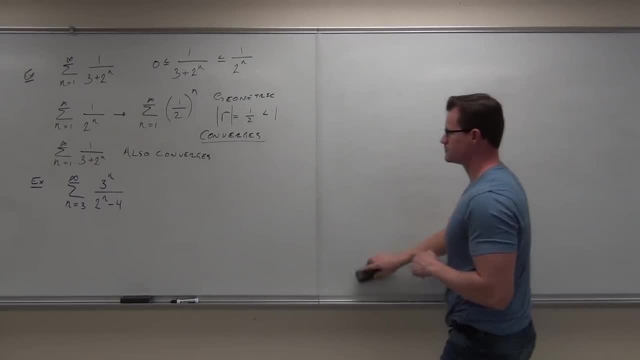 And we're here looking at the results, because we have no real results And we're all going to try and figure out what we actually get. We're going to see what we get after that. You're going to see what we get after that. 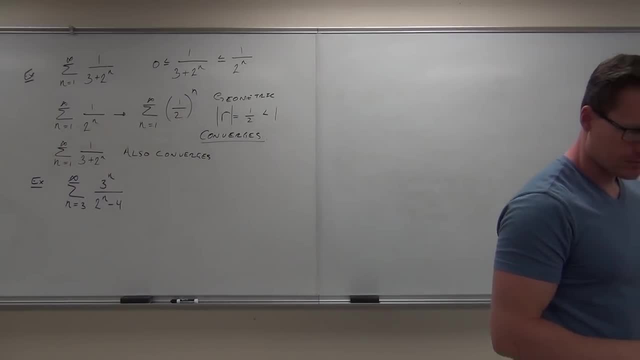 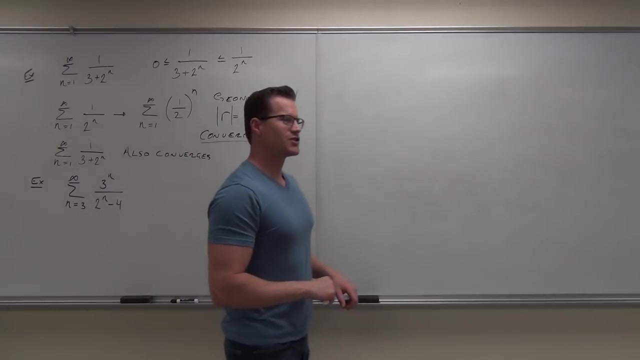 You're going to have to try and get to and from that. Tell me something: are all the terms here positive? Did you see why we had to do n starts at 3 and not n starts at 2 or something? If we said that n starts at 2,, we'd have something undefined. if we said n starts at 1,, we'd have 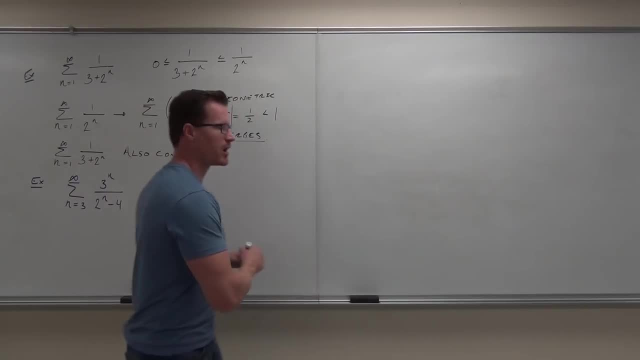 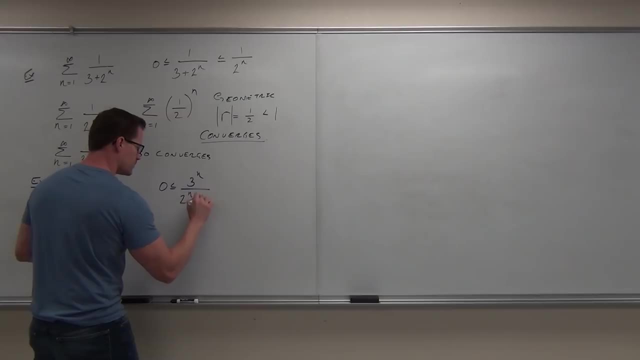 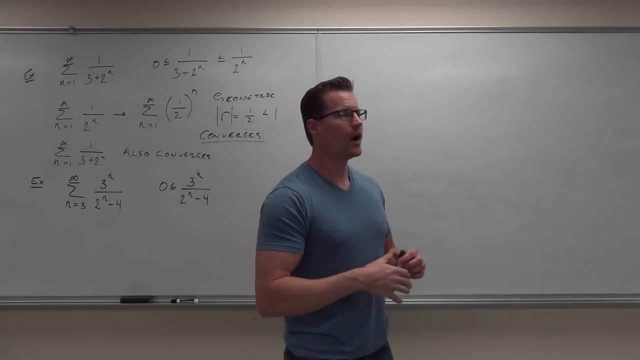 a negative and then something undefined. so we said 3, so we get something that is positive, So okay. so yeah, all the terms are positive. Now, next up. next up, what is this going to be based on? What's a good series for us to base this one on? 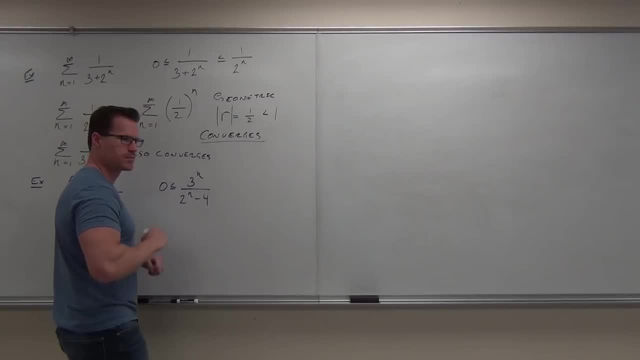 Try to figure out whether it's diversion or conversion. What is it? Do you remember? Do you remember me saying that when you have a constant like that, that's the thing that's holding us back? typically, This is what's holding us back right here. 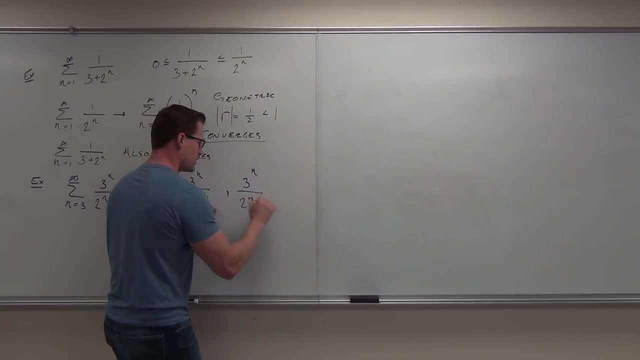 So we have 3 to the n over 2 to the n minus 4, and we have 3 to the n over 2 to the n. Check it out. here's how you figure this thing out. Would you be able to tell me conversions or diversions for this guy? 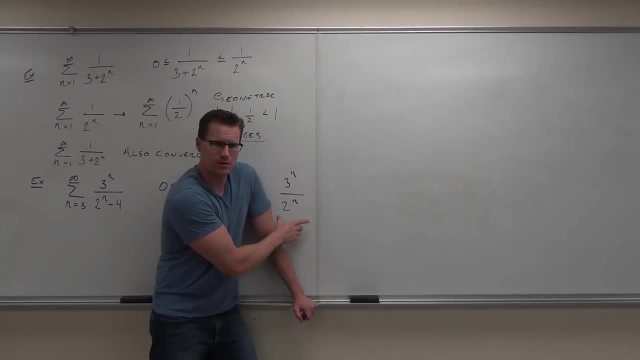 Yes, Okay, cool. Specifically, what would you be able to tell me? It's divergent, because it's divergent. Okay, so we're going to get to a divergent series right here Now. this one would have to be greater than or smaller than this one, to show also that: 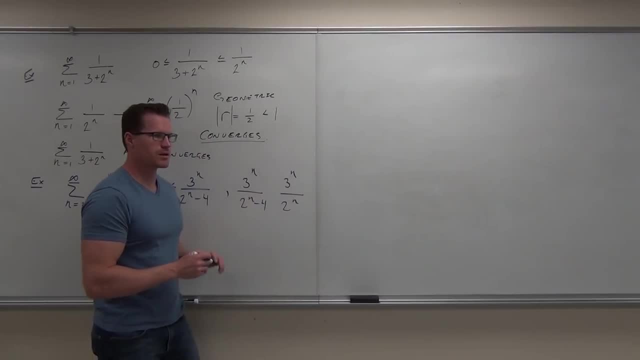 we're grazing, So we've got to figure it out. Is this bigger than this? This is this one. No, No, If I take a denominator and I subtract 4 from it, it's going to make it bigger than my starting. 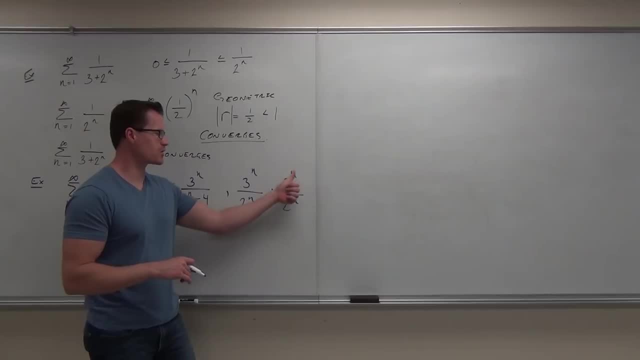 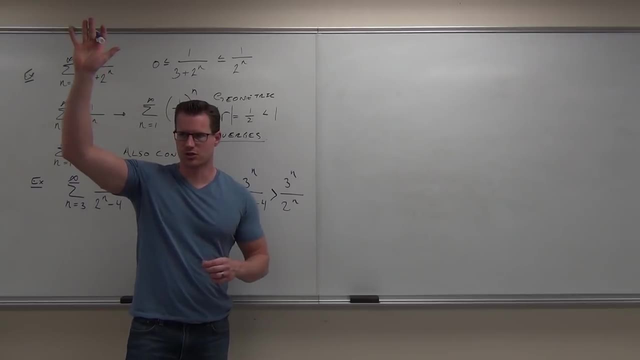 fraction. So basically it says: this fraction is always greater than this fraction. My denominator is smaller, therefore my fraction is larger, So I can actually be okay with that one, Are you sure? Mm-hmm, Okay, Do you guys see the point of trying to do this or saying, hey, you know what? 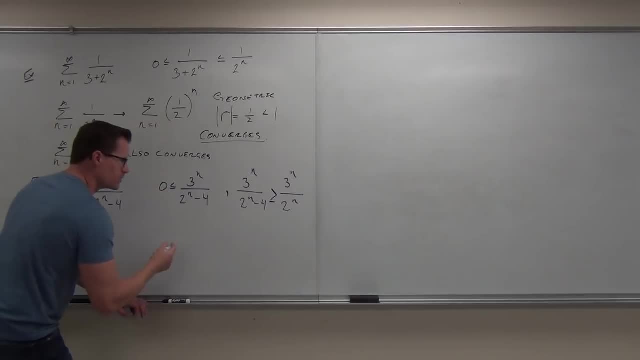 This is always bigger than this series. If I sometimes possibly equal, who cares? So if this series, if we can determine that this series diverges, then we can show that this series diverges as well. How about this? How am I supposed to write this series? 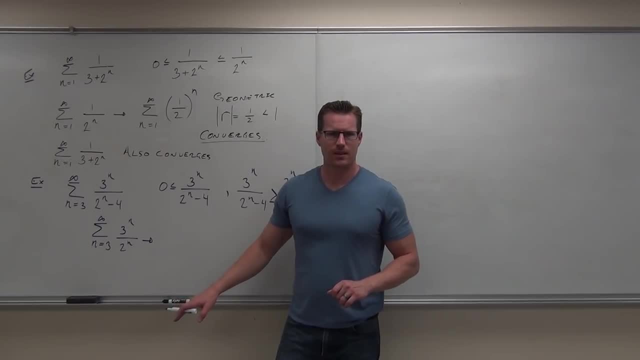 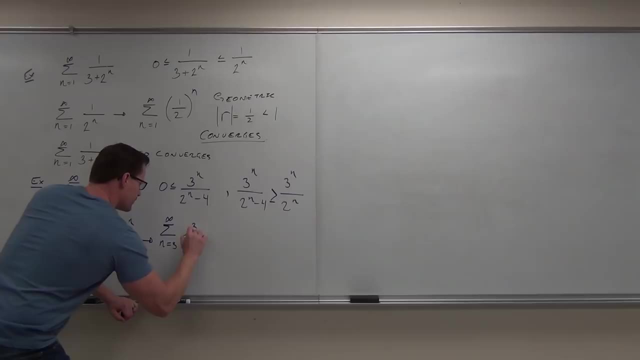 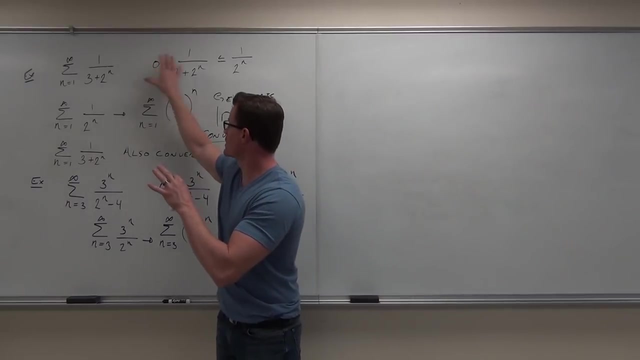 What should I do with it? Turn it into geometric? Yeah, It looks just like a geometric series. That's great. So we'd have 3 halves to the n power. Remember: the idea is base your given series on something that you already know: the convergence. 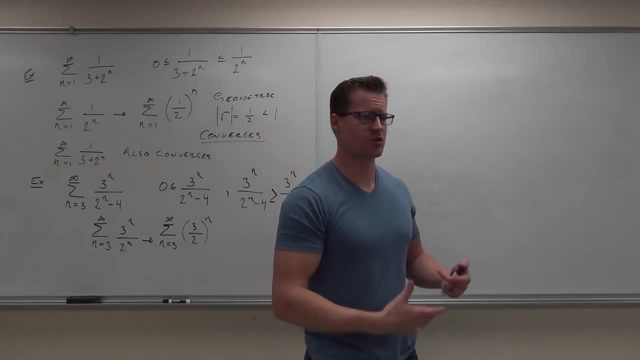 for, whether it's geometric, whether it's a p-series, whether it's a harmonic series, one of the ones that we already know. So for us, we're saying: man, you know what This thing looks, a whole lot better than this. 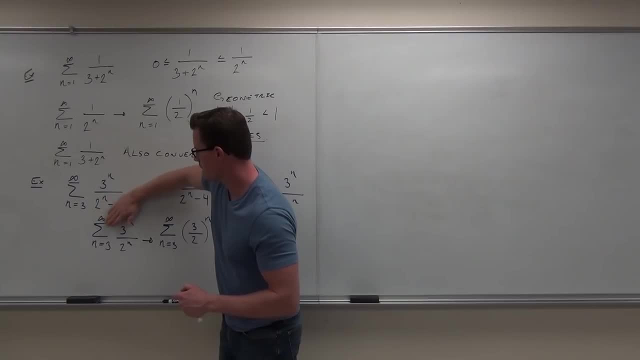 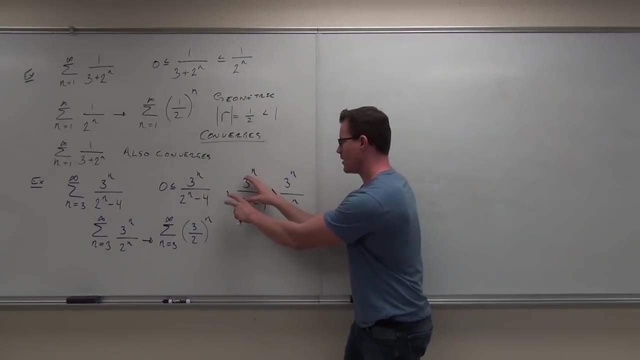 It looks a whole lot like if I got rid of that constant. it would look a whole lot like a geometric series. So let's get rid of the constant. So if I get rid of the constant, what that means is I'm basing that on something without. 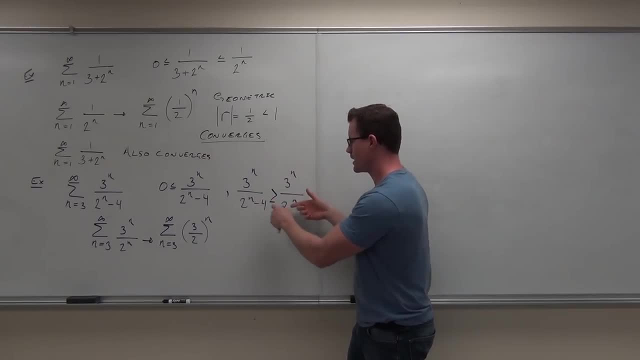 my minus 4.. Well, it's going to be bigger than 3 to the n over 2 to the n without that minus 4.. That's the idea. Since I know that this is geometric, that's why I chose that one, guys. 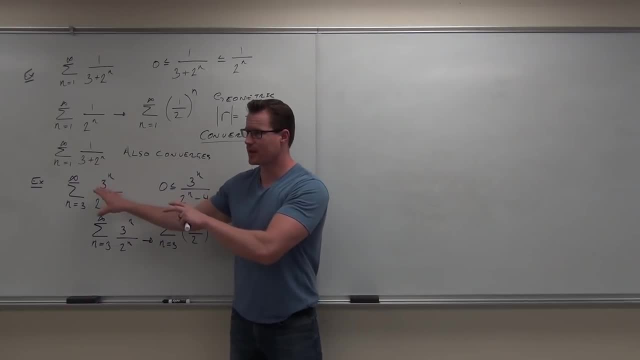 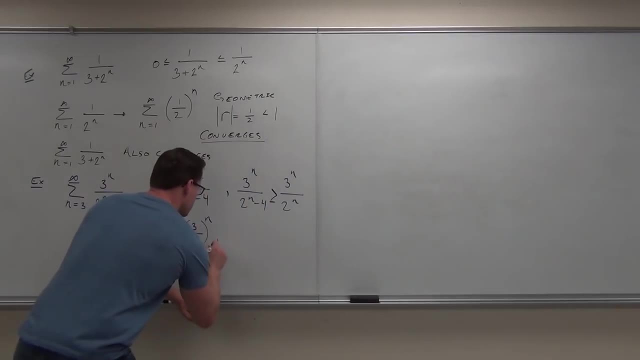 I'm not picking something out of a hat. I'm picking something that looks really similar, that I know the convergence for or divergence for. In other words, I know that that's a geometric series with r equals 3 halves, So we'd state this is geometric. 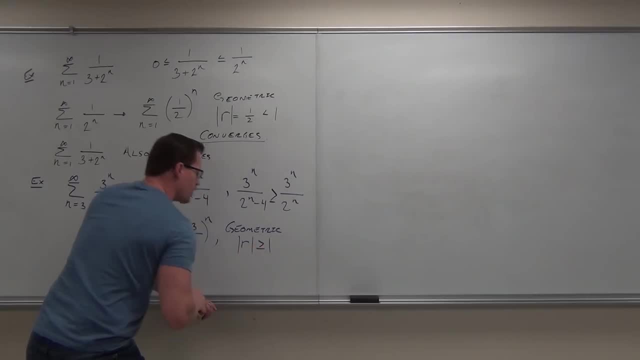 This has an r with an absolute value greater than 1.. Specifically, we'd probably write it this way: Absolute value of r equals 3 halves. That's greater than 1.. Tell me something about a geometric series when your r is greater than 1 in absolute. 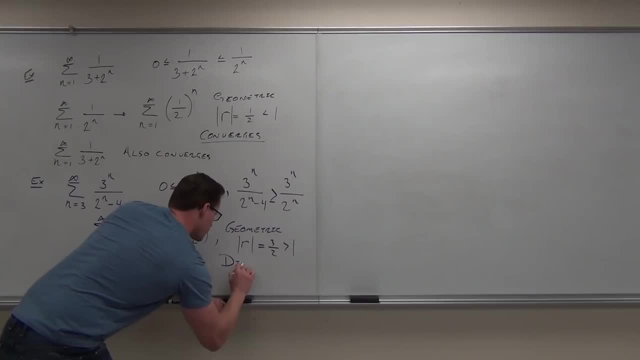 convergence. Notice: these are not arbitrary statements. You state it is geometric. You state that the r is 3 halves. Absolute value of r is 3 halves is bigger than 1.. Therefore, this geometric series diverges. Now is it going to be a problem that this doesn't match? 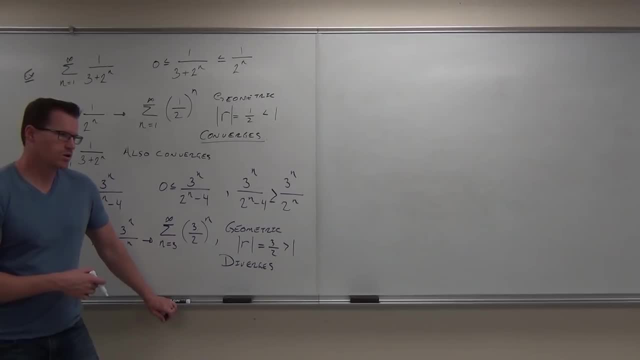 No, No. Could you make it match? Yes, You could. You just pull out 3 halves to the third and you'd have 3 halves to the n minus 3.. Not a problem. Why aren't we doing that? 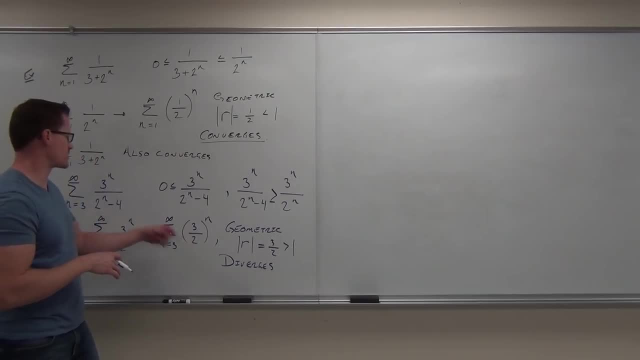 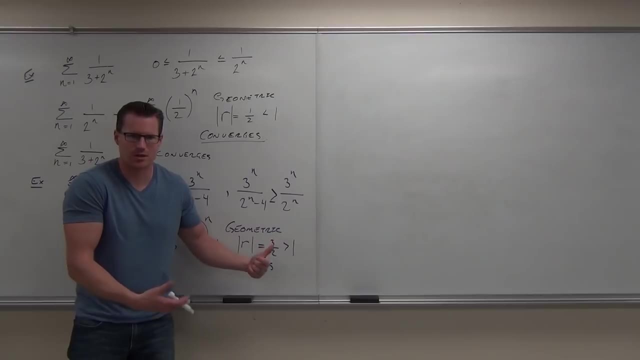 This sum is not going to be the same as the sum. It's saying that this is always bigger than that. So I don't even really care what the sum is. It's divergent anyway. I can't find the sum here. 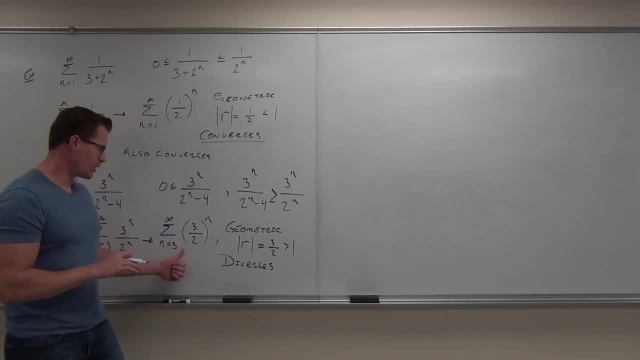 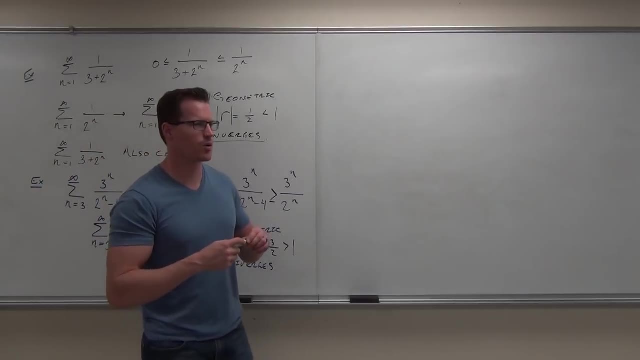 So I'm not really concerned about the sum. but if you're wondering why in the world are you not matching these up to an n minus 3, it's because the convergence or divergence will not change. I said this one time. This is kind of an important note that you have down somewhere in your memory banks. 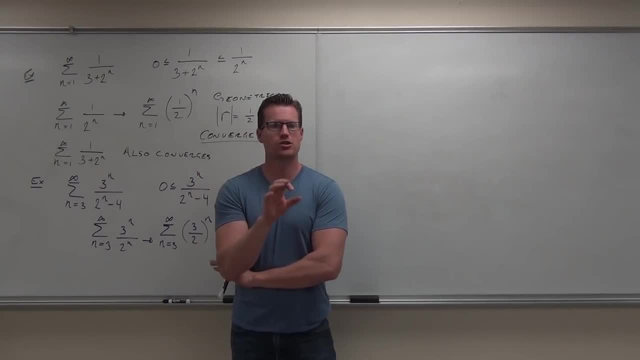 Remember that convergence or divergence will not change if I add or subtract a finite number of terms? Do you remember that The convergence or divergence will not change if I add or subtract a finite number of terms? The sum will change? Yes, the sum will change, but not the convergence or the divergence. 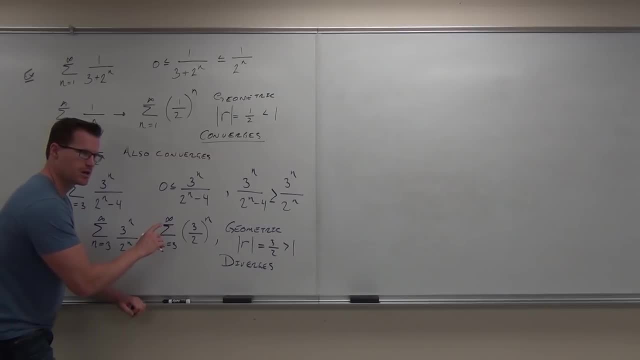 So, basically, this right here- look at the board please- This right here has the same convergence or divergence as this does. It has to, because all I'm doing is adding to it three terms Or four, Or from here to here. 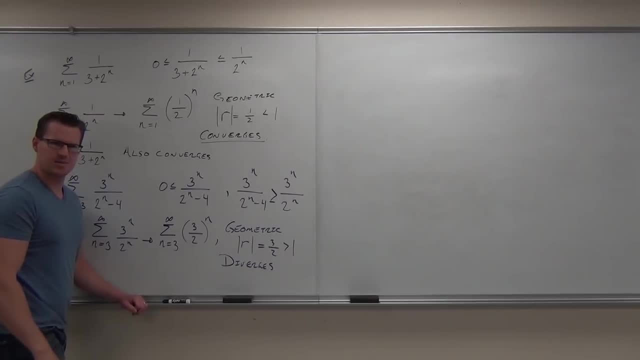 All I'm doing is subtracting from it three terms. Does that make sense? Therefore, if this one diverges, I'm subtracting three terms. This one also has to diverge. Don't care that I can't find the sum. 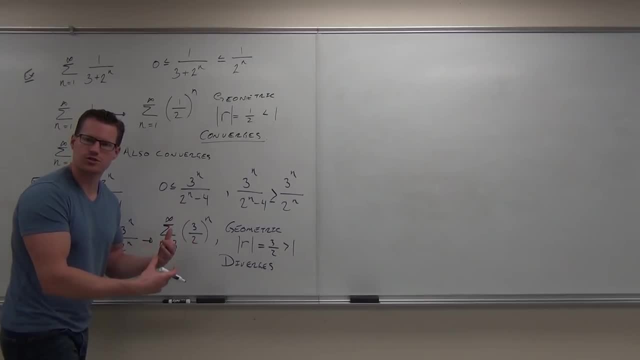 We're not worried about that anyway. We're not finding the sum here. What we're doing is finding out convergence or divergence. Now let's go one step further. So, because we know that my series is bigger than a given series for which I know divergence, 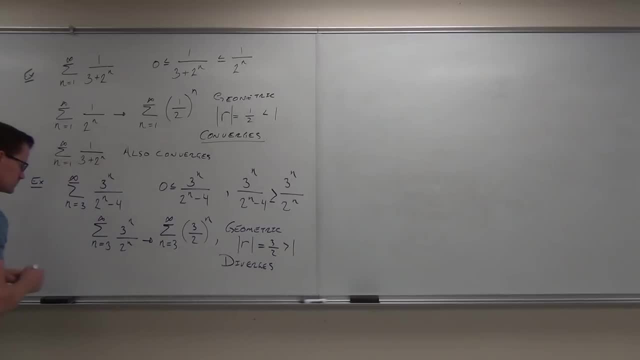 tell me something about my given series, And that's exactly how I want you to write it. I want you to start with a given series. I want you to base it on something you know- convergence or divergence- for Typically you kind of have an idea in your mind. hopefully you do. 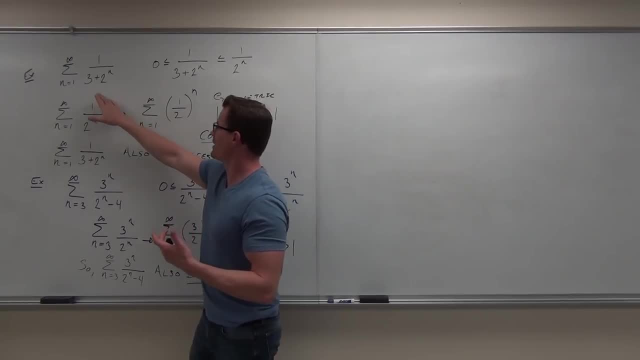 before you start this, Like for here, I'm thinking: you know what, if I cover that up, that's going to be. oh, that looks like a. that looks like a geometric to me, with r equals 1 half. If I cover this up, man, that looks like a geometric with r equals 3 halves. 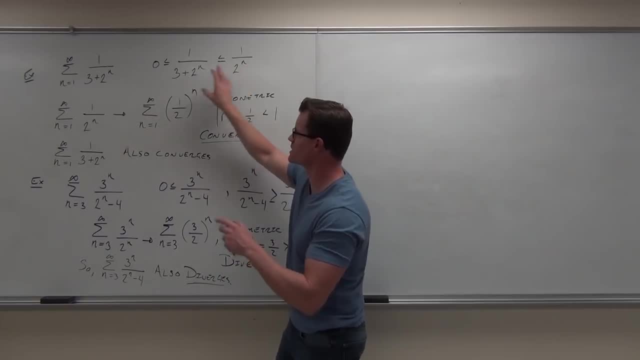 So I'm saying, okay, I'm going to try to make this smaller than a series that converges. I did it. It looks like a geometric. It's smaller than a geometric that converges, Therefore my series converges. Okay, this one is bigger than a geometric that diverges, therefore my series also has. 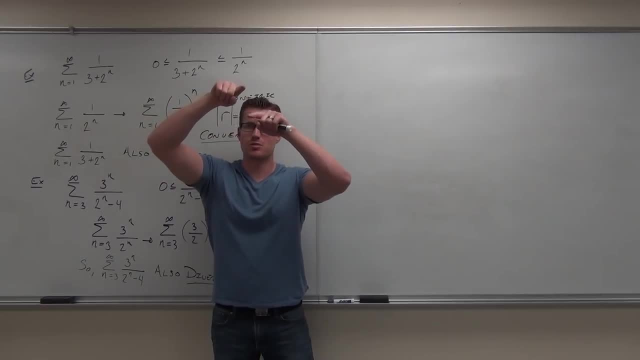 also has to diverge. This is the case where a sub n is smaller than b sub n, it's forcing it to converge. This is the case where a sub n is bigger than b sub n, it's forcing it to diverge. 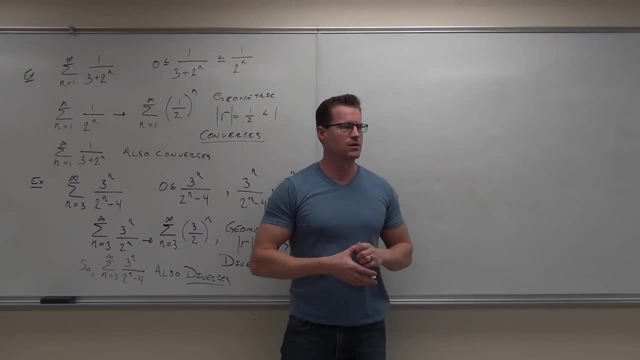 Show of hands. can I explain this well enough for you guys? Questions: Could we have just skipped all this work and we did the limit test, Limit comparison test? Yeah, We're going to in a minute. What do you mean? limit test? 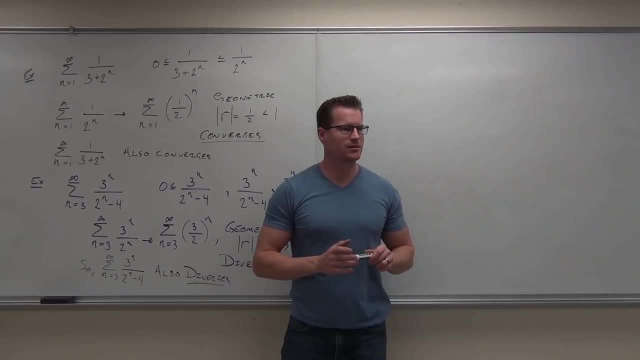 It's like the divergent test, Like take the limit and get that original thing and go to infinity. Yeah, You could have, but you didn't stop me. You should have, but you didn't. I thought you were trying to make a point. 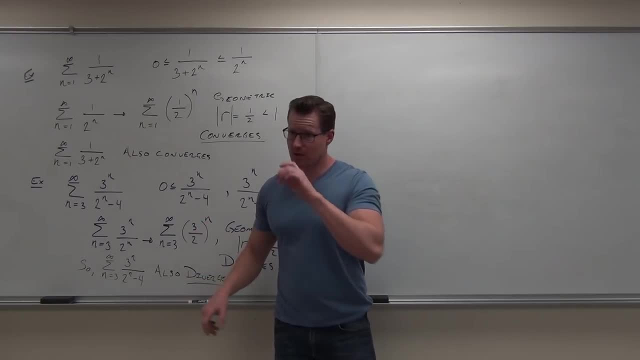 I am making a point. I did make a point, But if you do, if you do, the first thing you should always do is what I've said, that every problem except for this problem. right, Because I was making a point. 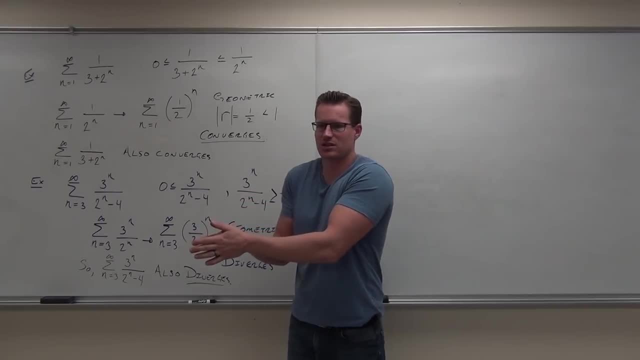 But if you did that well, you have a fraction that's bigger than 1 raised to infinity. It's going to go to infinity, It's not going to go to 0. This would fail. with that. It's going to be a divergent test. 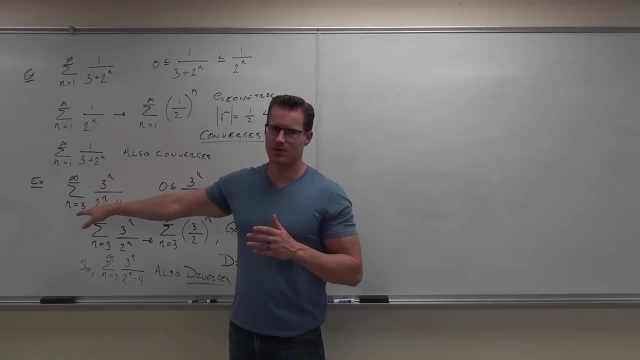 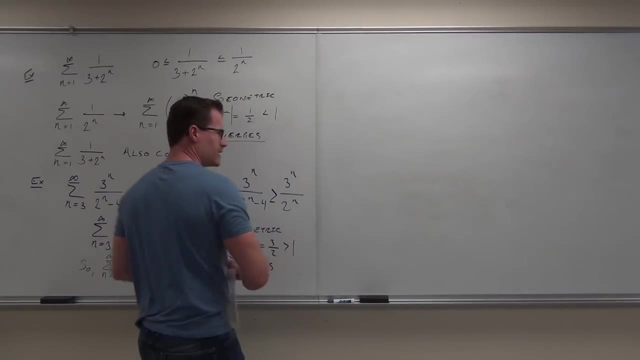 It would not equal 0. It would be divergent. Does that make sense? It stopped right there. Good catch, Let's try one more. Any other questions before we continue? You guys are awfully quiet today. That just blew my mind, honestly. 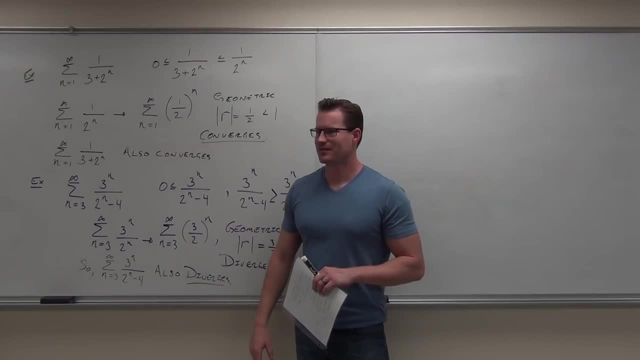 This one, The limit little comment, Divergent test. After I let it soak in: Oh yeah, Now doing this appropriately would take a little work, because you can't just start with 3 to the n over, 2 to the n minus or without the minus 4.. 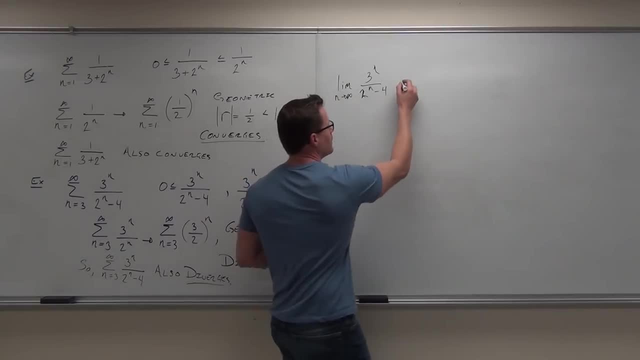 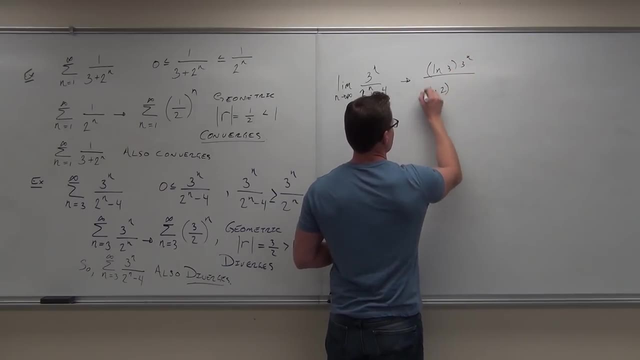 So you'd probably have to do the L'Hopital's and say this is infinity over infinity to get rid of that 4.. So you'd have ln 3, 3 to the n over ln 2 times 2 to the n. 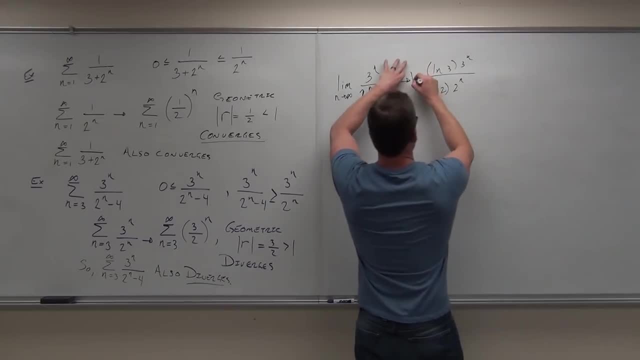 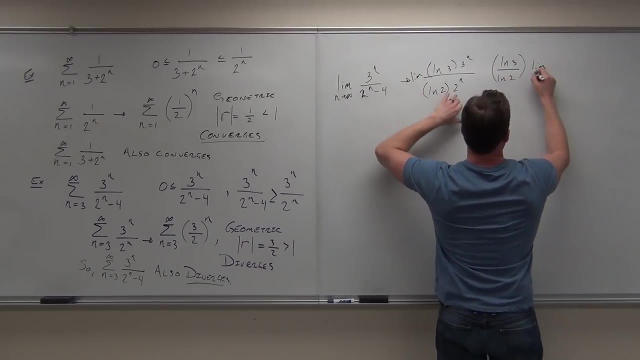 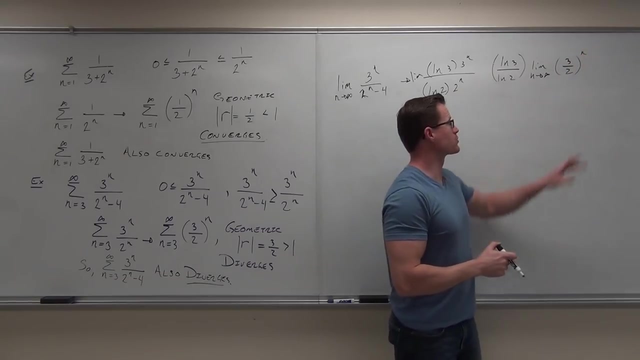 Then you'd do it. then you'd go ahead and say: that's a constant, So pull out the ln 3 over ln 2, have a limit, as n approaches infinity, of 3 halves to the n. And then we think, okay, this is a fraction that's greater than 1.. 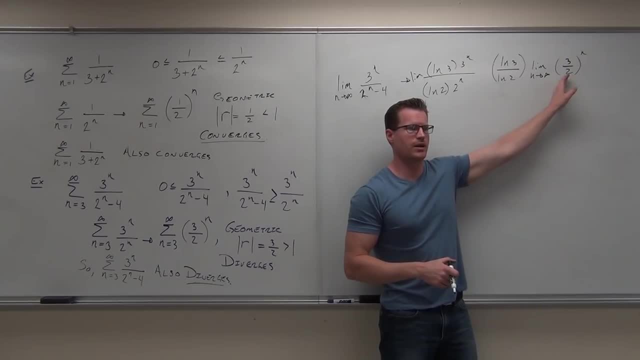 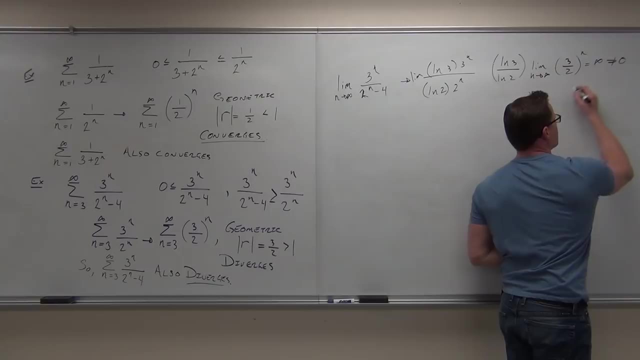 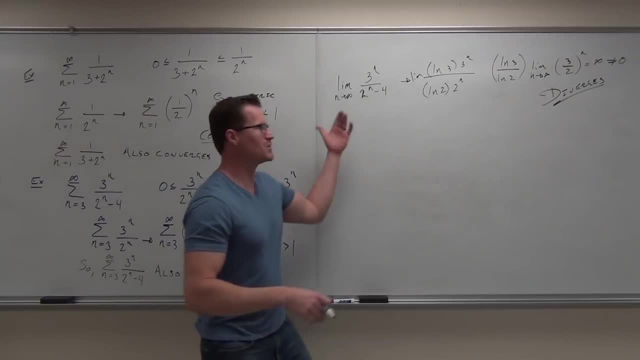 And you could also show it that way. So this is a twofer. We could do divergence test and it fails it. Hey cool, no problem, It's not equal to 0, therefore our series diverges. Or you could show it this way: 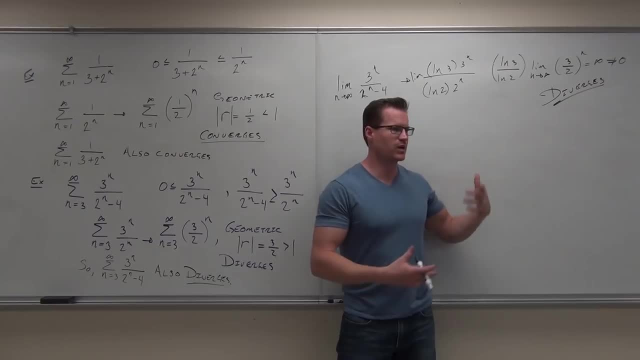 Honestly, for me they're about the same level of difficulty, but you should be checking the divergence test first. That was a great point. Show of hands. if you understood both of these, Good deal. Okay, now we'll do one more. 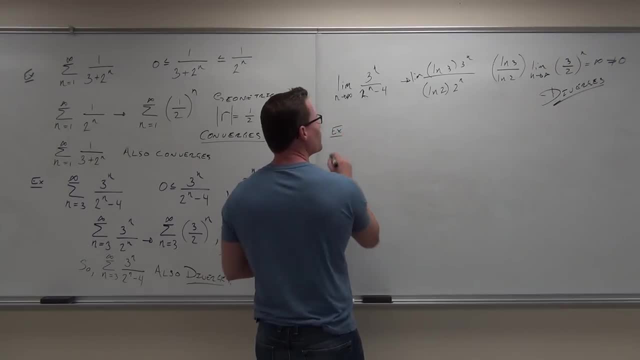 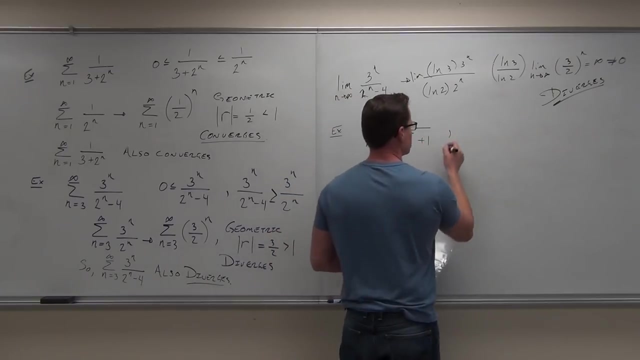 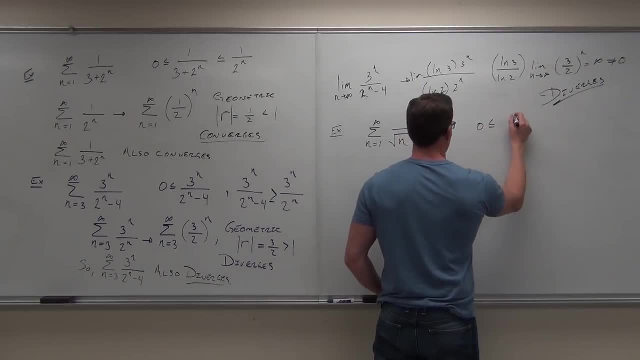 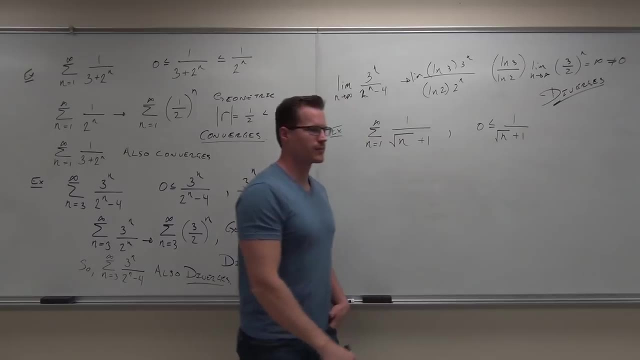 Yes, no, Yes, Okay, Cool now what's the problem on our series? that we can't do what we want to do. What's our problem? The plus 1.. The plus 1 is a problem, So let's base this on a series without the plus 1.. 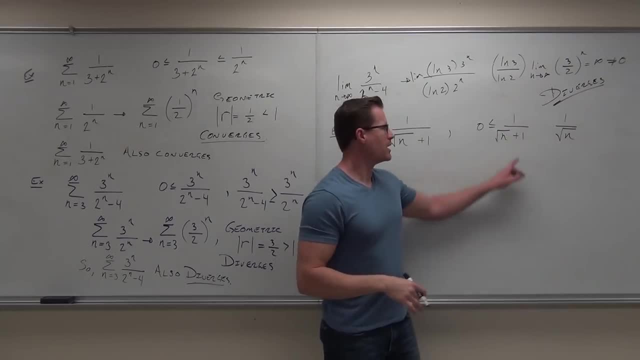 Because I don't want the plus 1.. The plus 1 is the problem. Is this series greater than this series, or is our given series greater than this series? Is our given series less than our series? that we just made Less than? 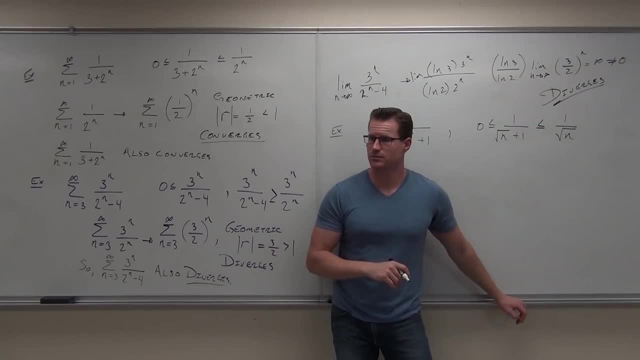 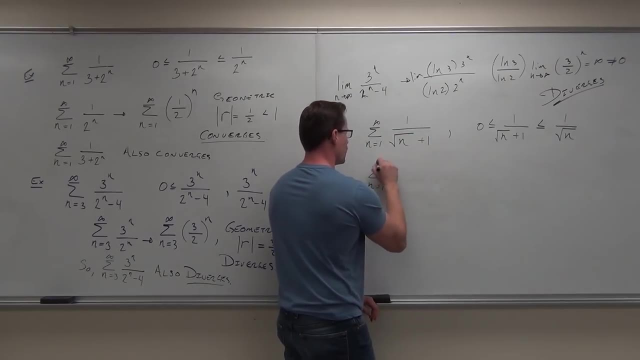 Less than For sure. less than So far, so good. Okay, now here's the issue. If I do the series of 1 to infinity of 1 over the square root of n, do you understand that that's the series from 1? 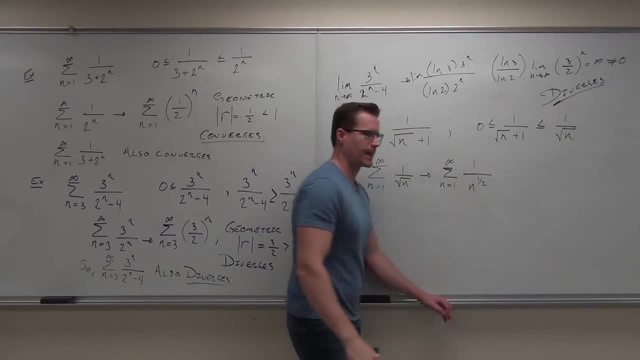 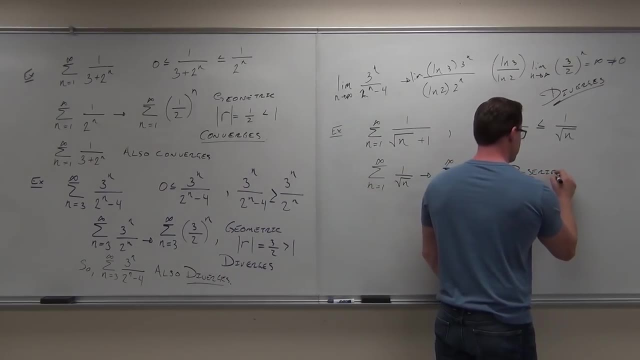 to infinity, of 1 over n to the 1 half power P series. Tell me something about that P series. P series, very good. What's the P 1 half? That's less than or equal to 1.. 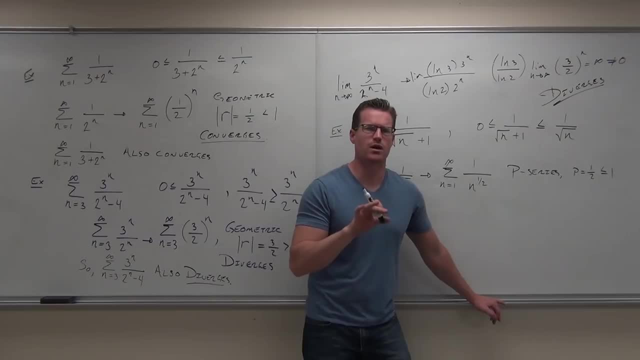 Tell me something about a P series where the P is less than or equal to 1. Divergent. Now let's go back to our original series. We have a P series right here where the P is less than or equal to 1.. 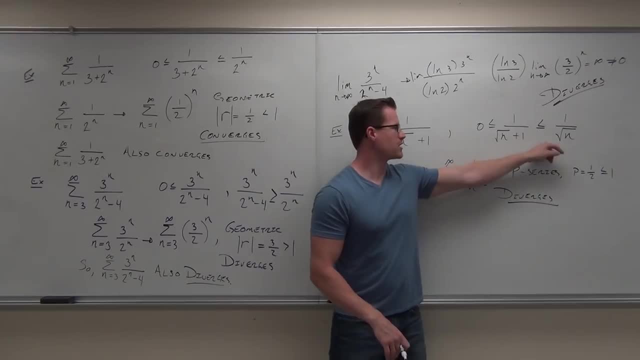 This series diverged right. Uh-huh. What's it tell you about my given series? It's not a P Crap, why not? It's greater than 1.. This is the time where you have B to the n and you have A to the n. 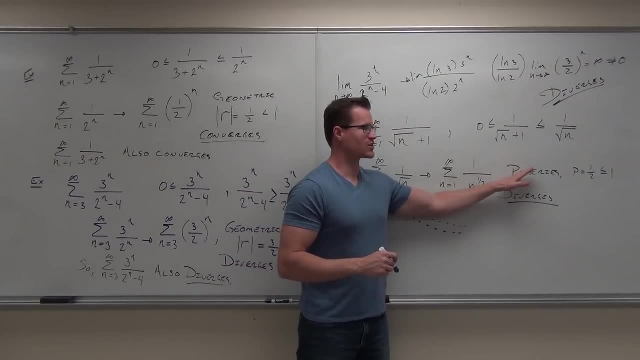 And I say, hey, look at this. B to the n diverges. What about this one? I don't know. It could converge, It could diverge. I don't know because I'm being forced anywhere. That's this guy, okay. 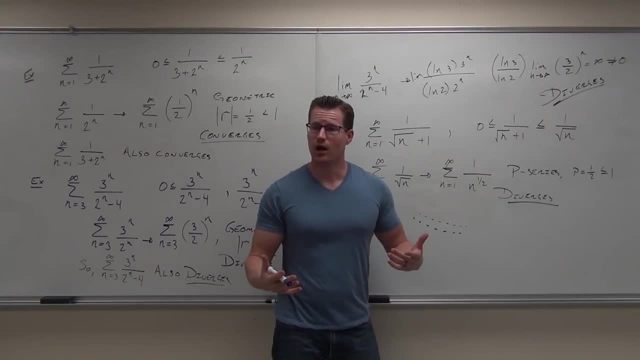 That's the don't be this guy. Well, this is the only thing that we could do. I mean, we can't make this. This is smaller than the series that converges, because we don't know what that is. We don't know what it's going to be. 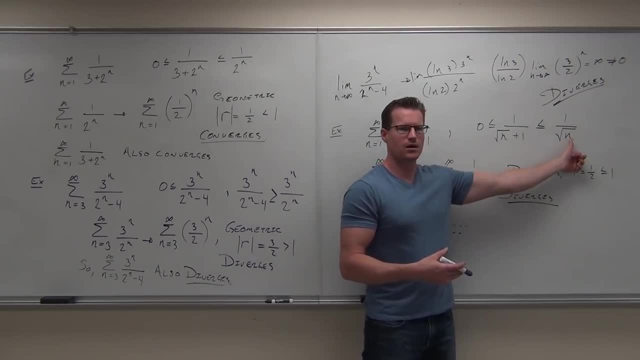 We don't know anything about this. The only thing that we could do is base it on this immediate one, This one that says: okay, we know for a fact that this is less than 1 over the square root of n. We know that for sure. 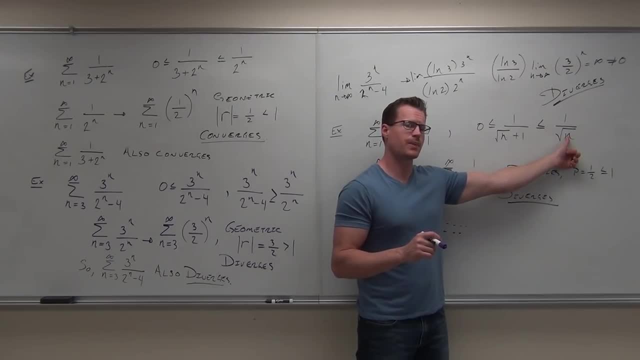 But we know that this thing diverges. If that diverges and our series is less than this one, it's inconclusive. It's not a good test for us. That's the only thing we could do, But it wasn't a good test. 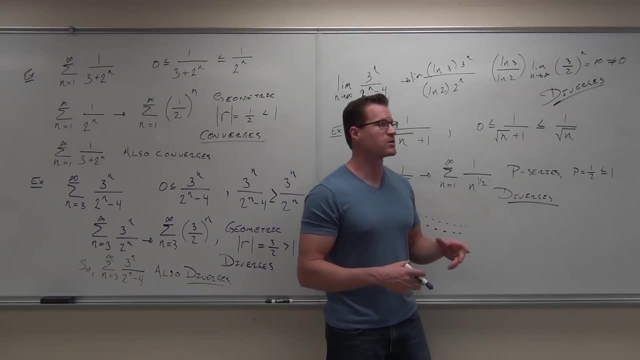 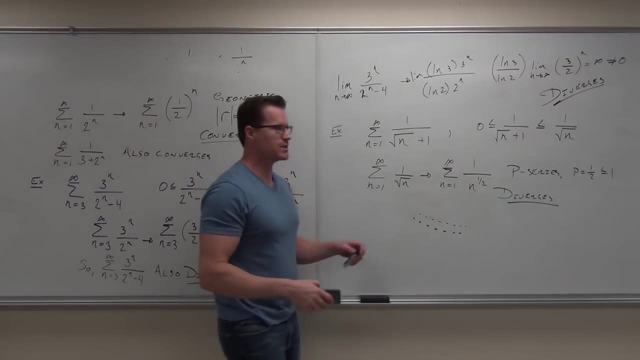 Now the point is, we don't just stop here, We have something else that we could do- The other type. by the way, we didn't test this, but hopefully you did this in your head. Could you do the divergence test with this? 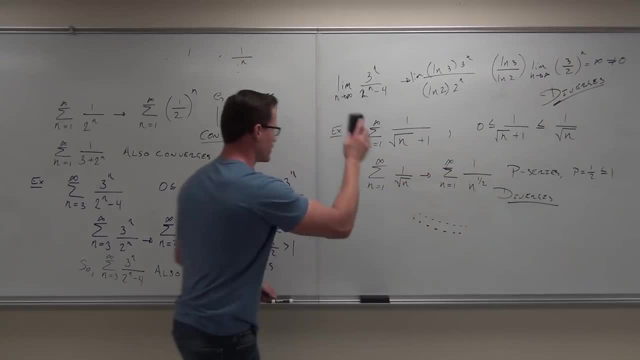 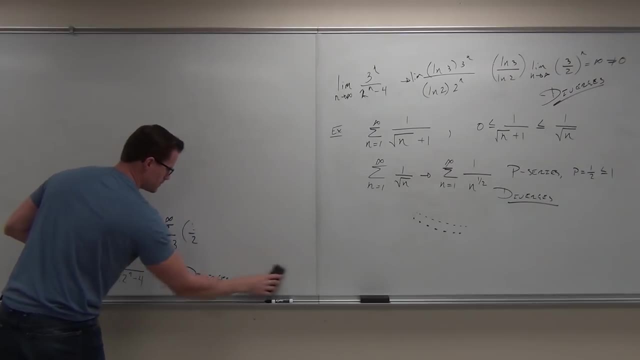 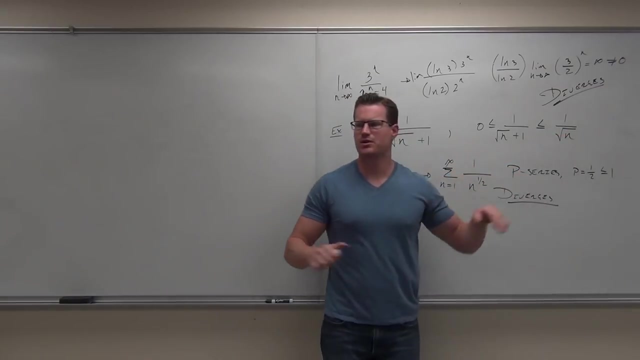 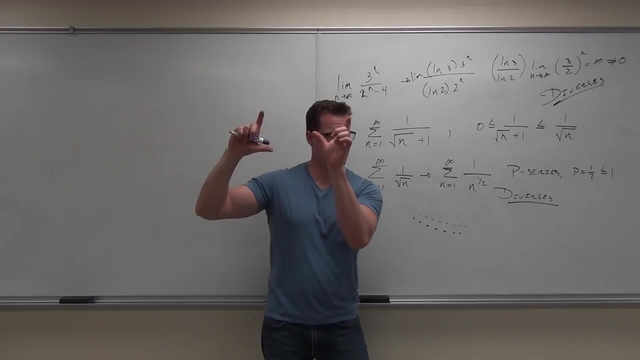 The limit of this guy is zero. so we know we should have moved forward, unlike the last example. So if ever we can't just use a Basic comparison test like the ones we had, What we had works great if your series is less than something convergent or more than something divergent. 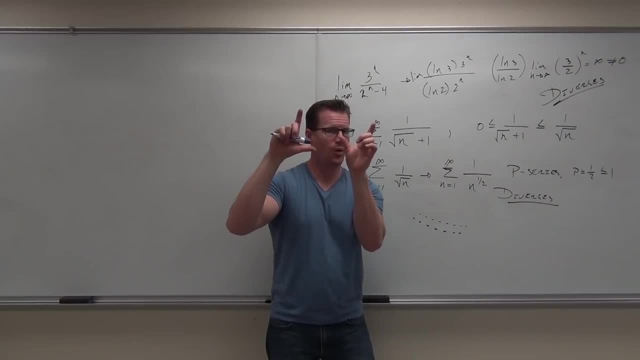 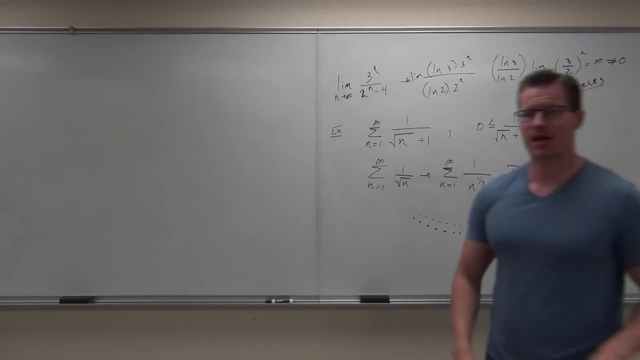 Does that make sense? If we're less than something divergent or more than something convergent? it doesn't make any sense to do that. We have another test for that. We're going to talk about what's called the limit comparison test. 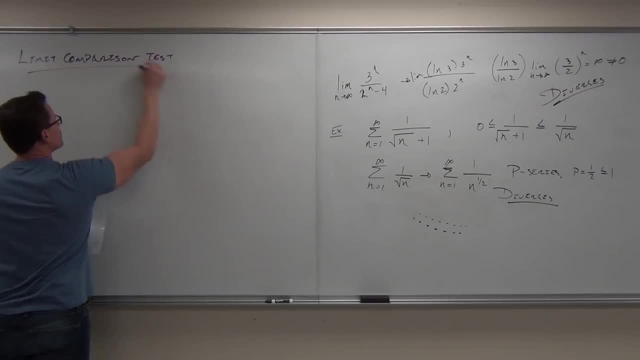 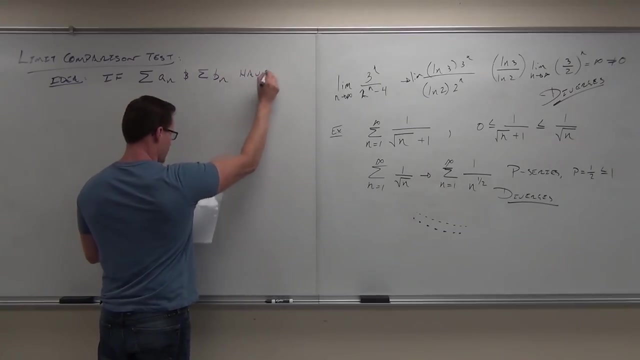 Here. I'm going to table it this way. Here's the idea for the limit comparison test. Here's the idea for the limit comparison test. If the series of a sub n and the series of b sub n have all positive terms, We have to do a series of positive terms in the order that we got it. 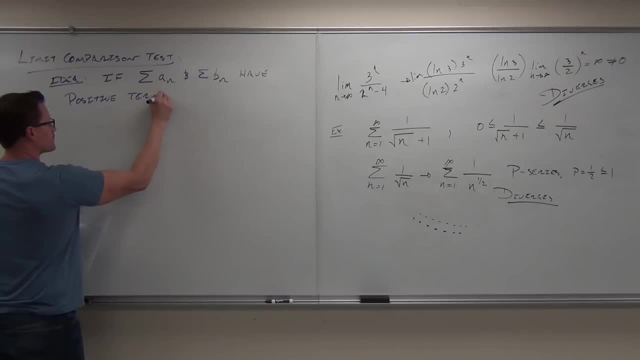 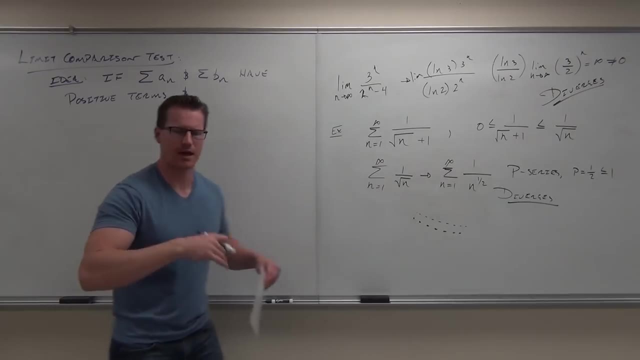 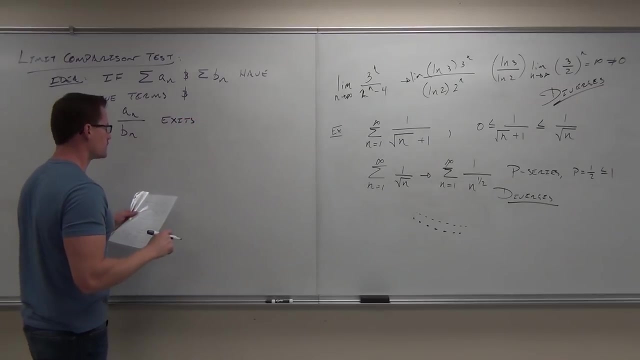 If we did, what would happen? and here's the big part. okay, so positive terms. we had that from before, right? that's for any of these comparison tests, they have to both have positive terms and the limit of a sub n over b. sub n exists not, exits. right, make this leaves. 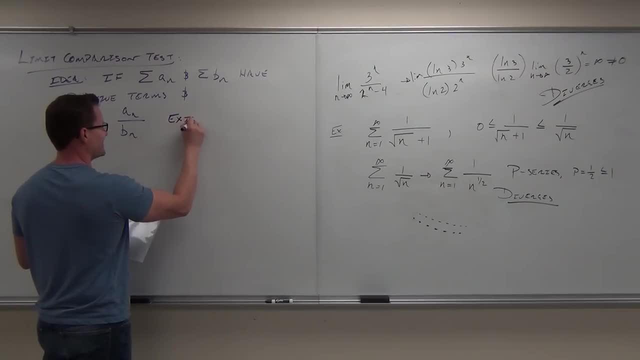 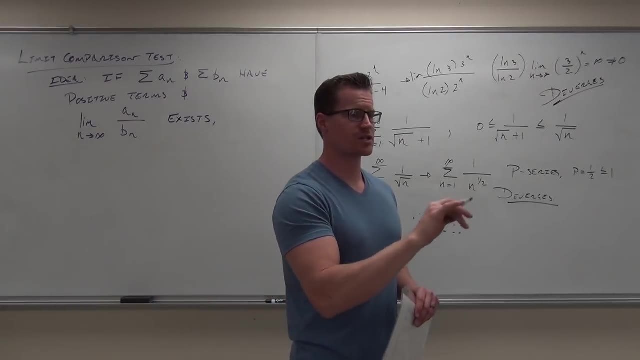 the room it just gives up exists, and here's what we know, then either both series converged or both series diverge. they're tied together so closely that one is a predictor of the other, and that's what the limit comparison test says. you could probably think of it this way, okay, well, if this exists, think about: 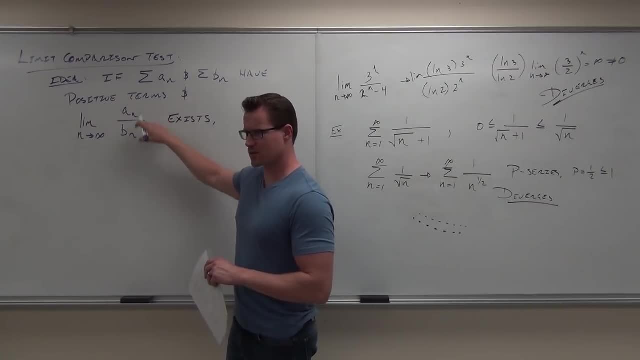 this. think of this: if this limit exists, this is a ratio right of one series of one, the terms of one series over the terms of another. If the limit exists, at some point it's n approaches infinity. that means that those terms are so close together. 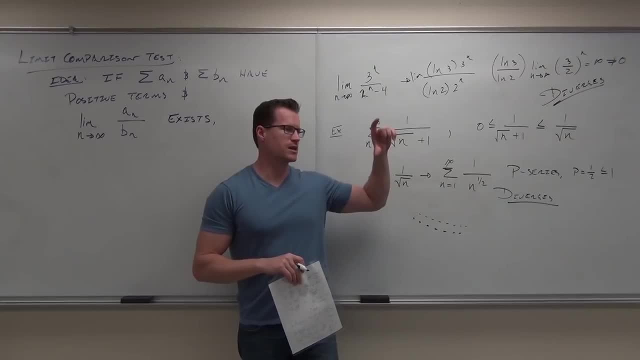 that it doesn't really matter. Does that make sense to you? If they're so different that it does matter, that thing's gonna go to infinity. Where did they get infinity? Probably infinity, because they're all positive terms, But that thing would go to infinity. 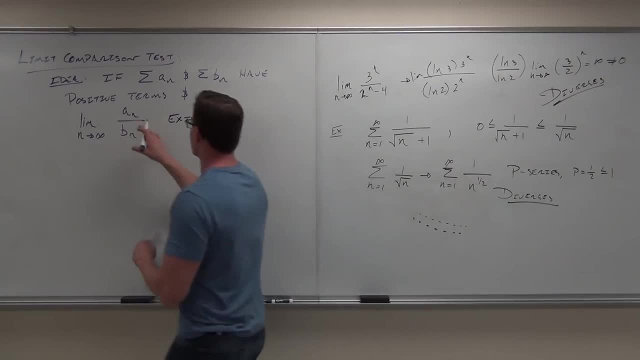 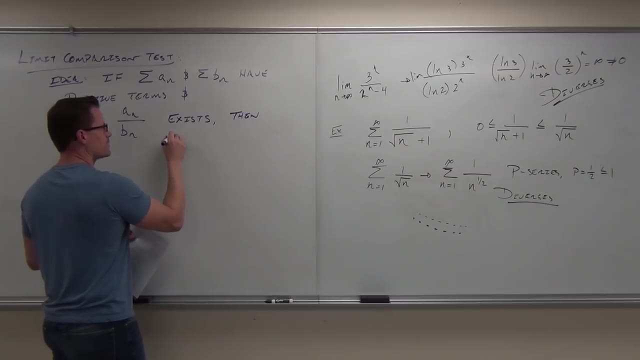 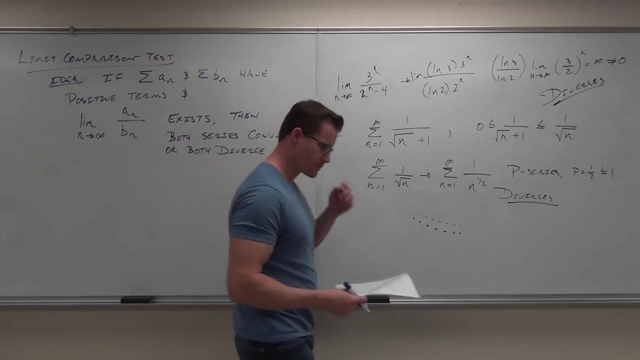 They would be so different. Does that make sense to you? So we say, okay, cool. So if this limit exists, then either both series converge or both series diverge. So again, I'm not gonna write this down, It's the same idea. 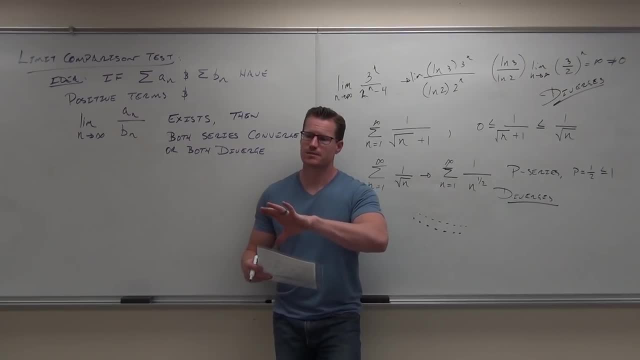 So we're gonna compare our given series to a series that we know the convergence of, and then we're gonna take a limit. That's the idea. Would you like a proof of this to prove that this is actually true? Yeah, Okay, so here's the proof. 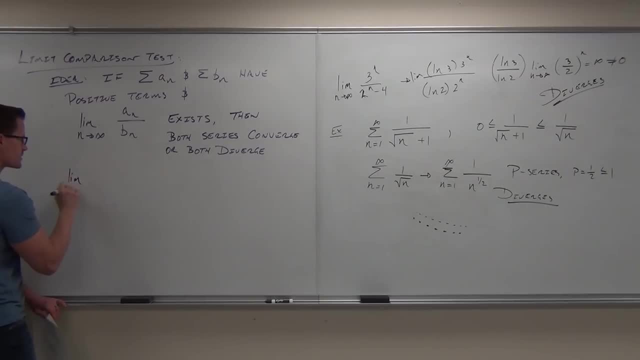 Let's suppose that this limit exists. If this limit exists, then the limit, as n approaches infinity, of a sub n over b sub n would be equal to some limit True By definition of what a limit is. what this means is that absolute value of a sub n. 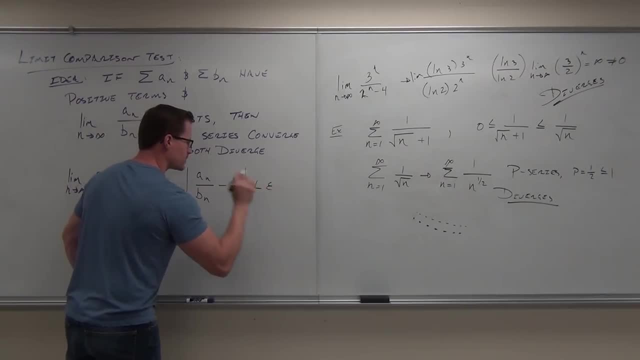 over b sub n minus l would be less than epsilon. Remember those epsilon delta proofs? You loved them right? Woo, That's what a limit. that's the definition of a limit. It means that the different. it's a very simple idea. 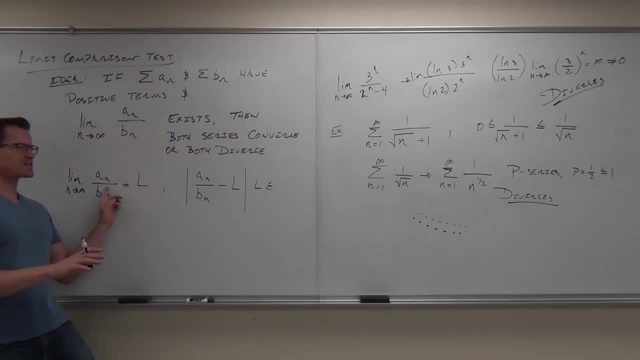 It looks really confusing. it's a very simple idea. It means that if this limit exists, then the difference between those, this fraction, well, whatever your function is, between this function and your limit, the difference between those in absolute value is less than whatever you say. it can make it smaller. 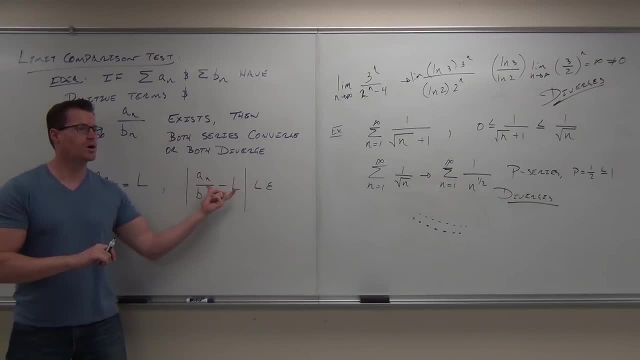 That's what it means. So you give me .0001, I can show that this difference is smaller than that. That's what the definition of a limit is. It says the difference between them is so negligible- it doesn't matter what it is. 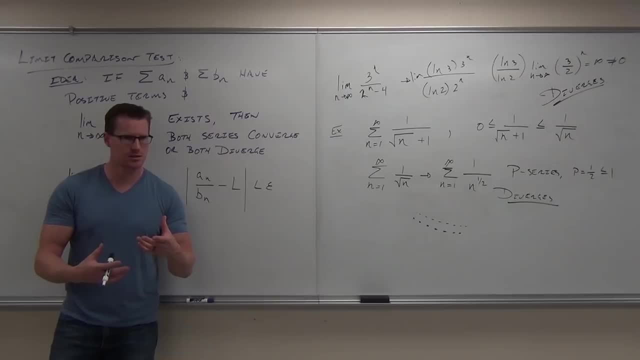 even if you give me epsilon a really little number, Okay, It's a number. Does that make sense, Are you sure? Okay, So this, by definition, is true. So if this is true, then for certain I can multiply by l, and it's still true, since l is a number. 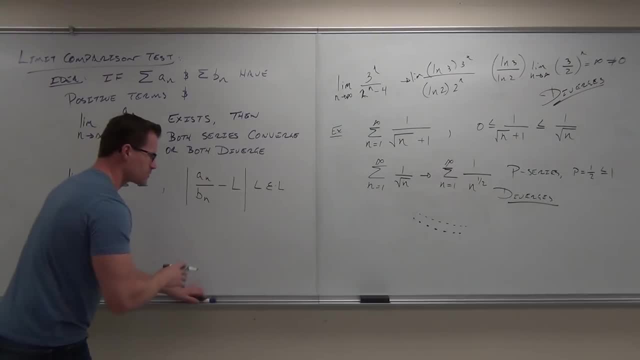 It's still true. Well, we're going to use that Because we have an absolute value: inequality. we should know that we can solve this inequality. well, we can manipulate this inequality by doing negative absolute value, negative, sorry, epsilon is the absolute value. 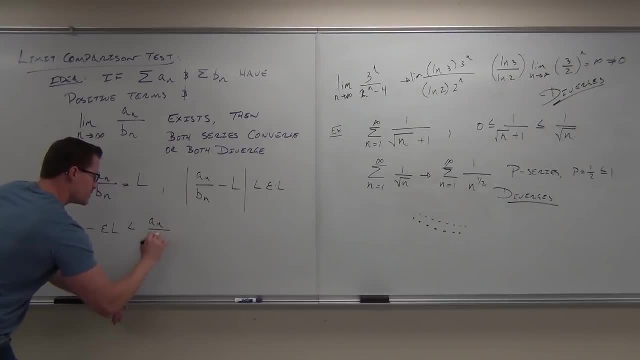 negative. epsilon l is less than, well, negative. epsilon l is less than negative. epsilon l is less than negative. epsilon l is less than n, a sub n over b, sub n minus l, which is less than epsilon l. Well, that wouldn't have to be true. 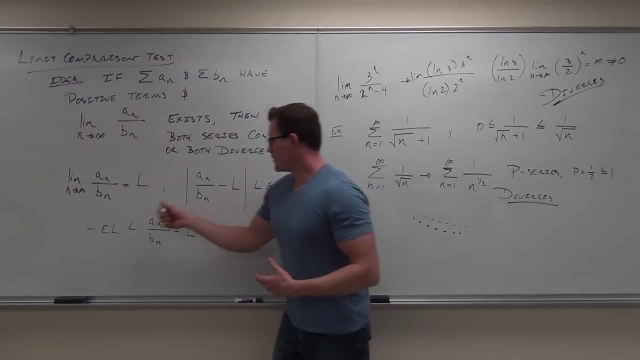 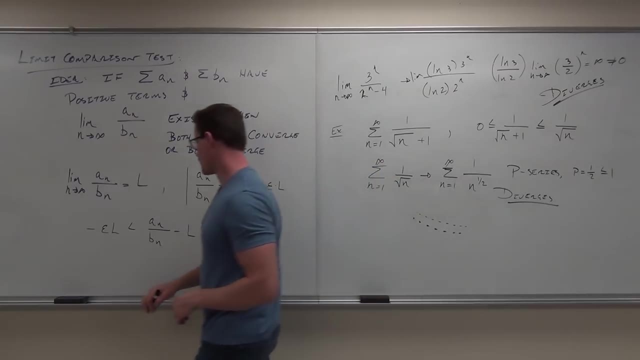 That's how absolute values work. Absolute values work this way. Okay, well, but make that negative. This is bigger than that. if I leave it positive, this is smaller than that. it's now done, when equality We're just going to solve for this. 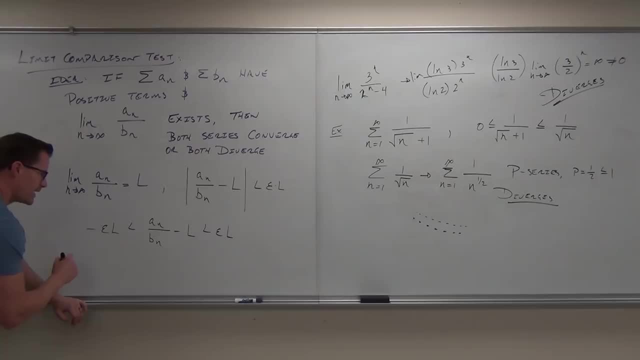 So what we're going to do is we're going to add l to both sides. If I add l to both sides, I get l minus epsilon. l is less than a sub n over b sub n, which is less than l plus epsilon l. 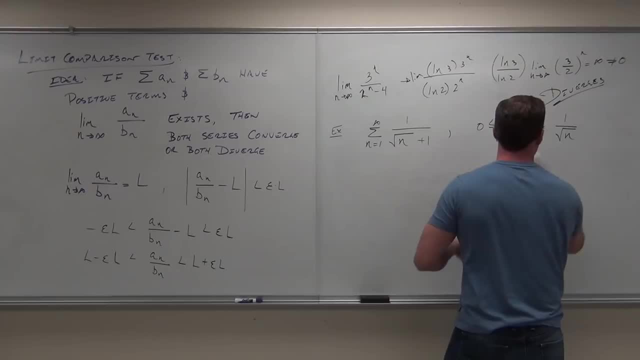 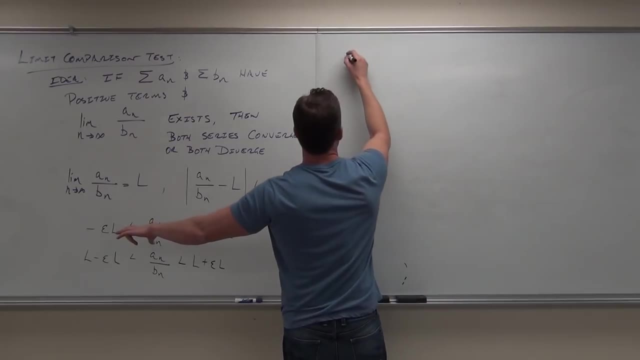 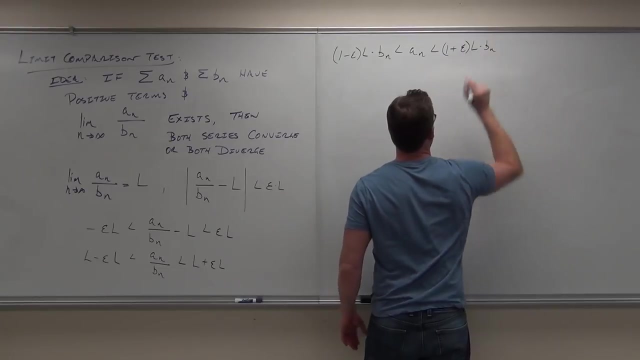 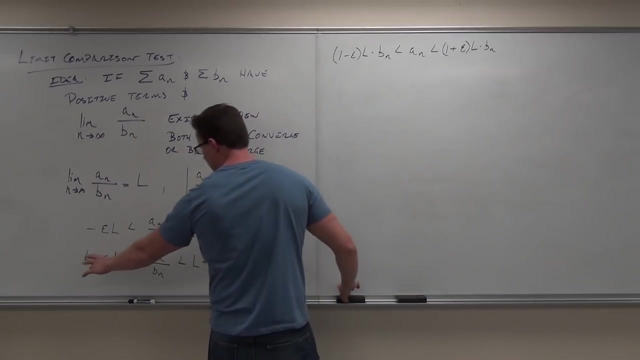 Almost done. Last thing I'm going to do is I'm going to factor and I'm going to multiply it by b sub n. So we factor out the l, no problem, it's 1 minus e, 1 minus epsilon. Factor out the l, it's 1 plus epsilon. 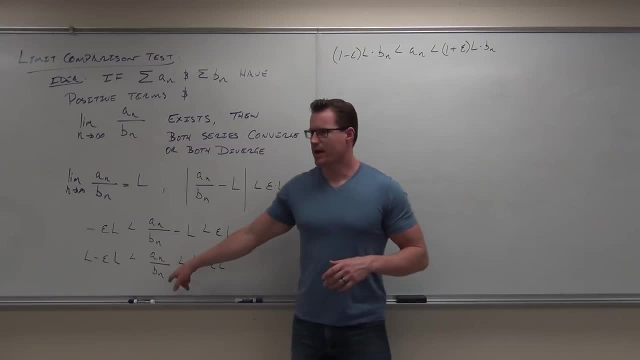 Multiply by b sub n on all three sides. By the way, we can do that because b sub n is what type of a number, what type of terms? They're positive. It's not going to change my inequality, So this is all based on. 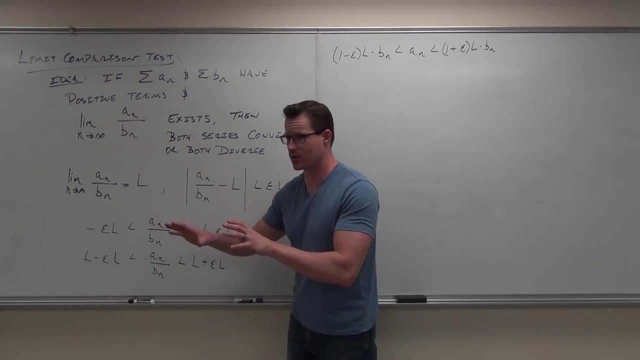 this is all based on the number of terms. So this is all based on the number of terms, So that b sub n has to be a positive term. So we can do that. It does not change the inequality. I don't know if you understand that idea. 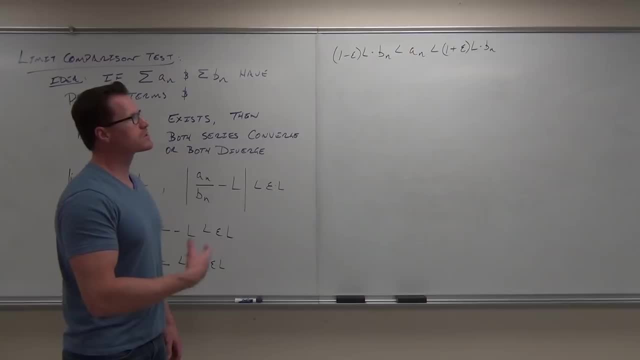 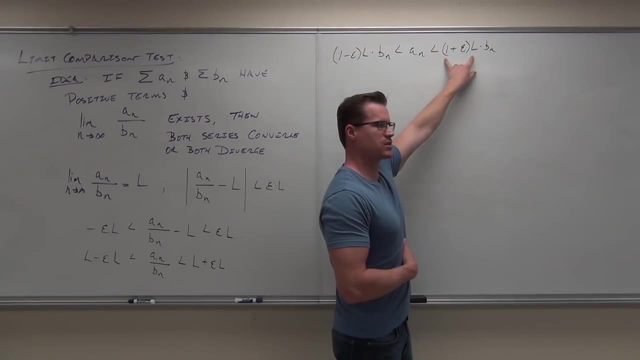 Okay, so it's positive, wrong, good. as far as inequality is concerned, Well, here's the idea. Here's where this comes in. Do you understand that? that's a constant? Epsilon is going to be some number, right. 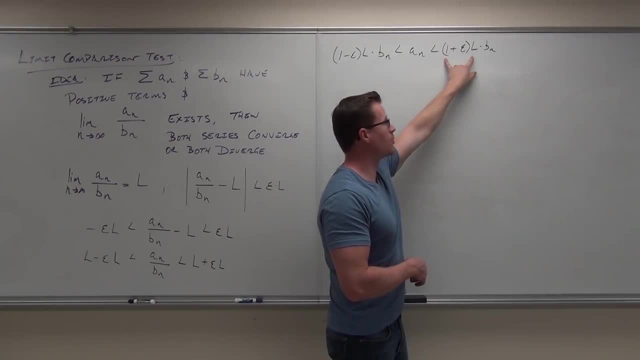 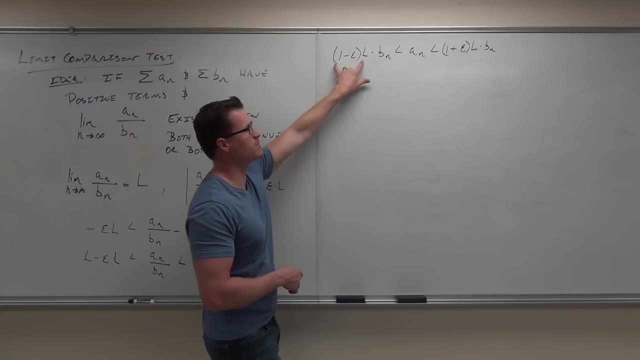 Add 1 to it: it's still some number. Multiply by l: it's still some number. So the convergence of b sub n is not affected by what this is. Likewise, the convergence of b sub n is not affected by what this is. 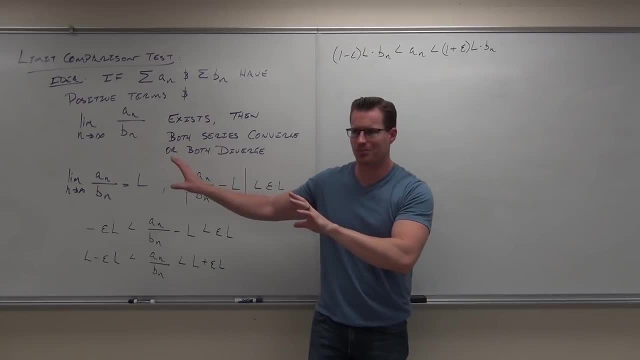 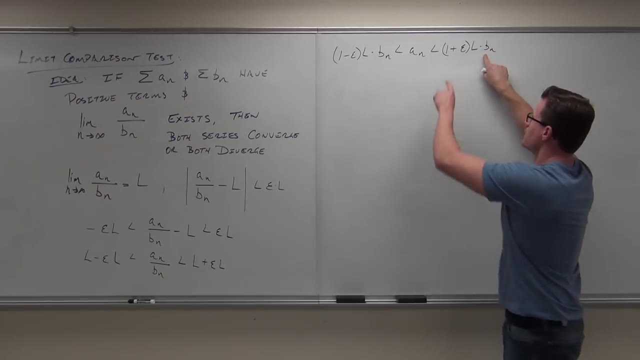 So think, Think about this, And this proves both of them. This is kind of cool. If the series b sub n converges, if the series b sub n converges, a sub n is less than that series. Do you see that? 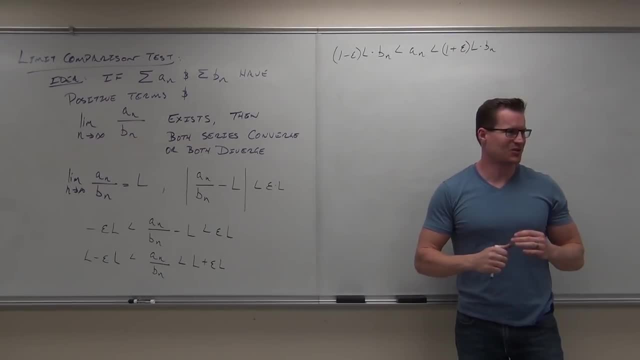 Okay, you're not really with me. huh, Are you with me? Yes, Kind of sort of, Partly. yes. Do you see the comparison test out of this right now? If b sub n converges, a sub n is less than that. 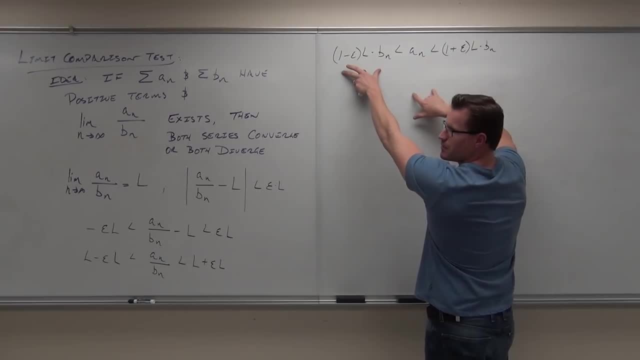 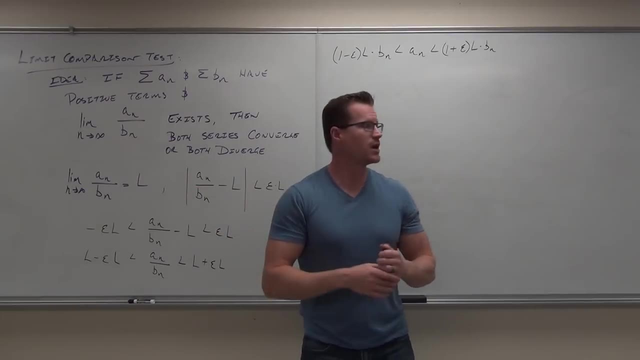 If b sub n diverges, a sub n is greater than that. So, just based on whatever we're looking at, if b sub n converges, no problem, a sub n converges. If b sub n diverges, a sub n also diverges. 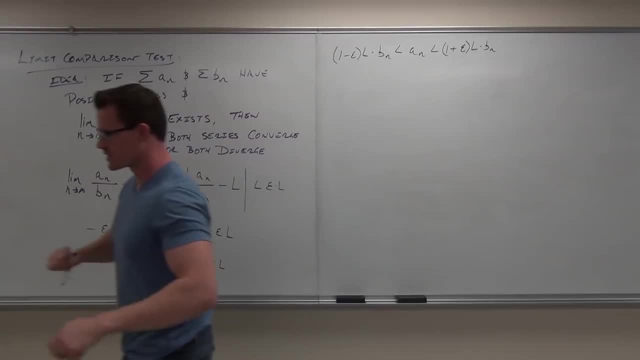 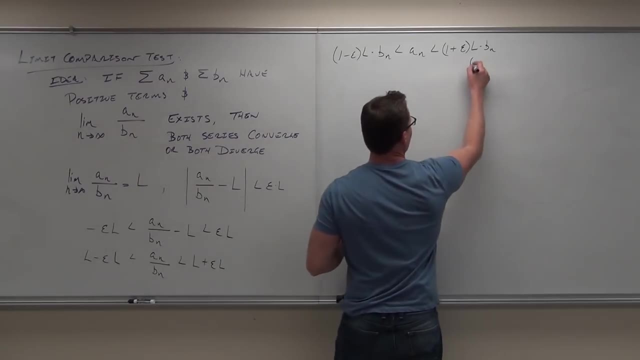 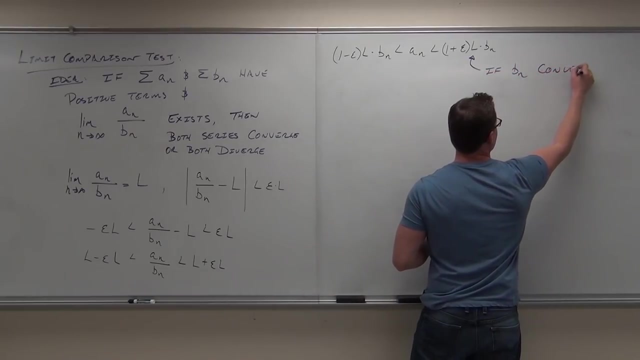 That's the idea. So I think you understand the idea. That proves this guy, That proves this, this theorem here. So I'll write that real quick and we'll be done. If b sub n converges, since a sub n is less than that and this does not. 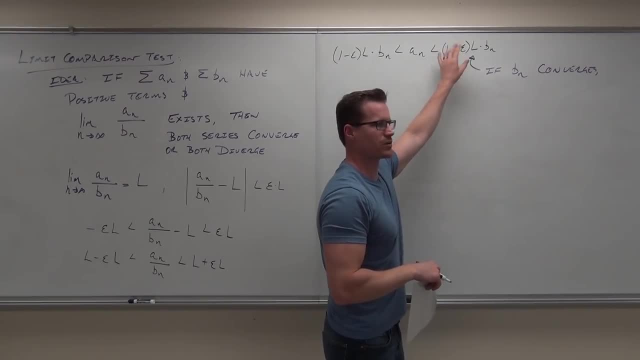 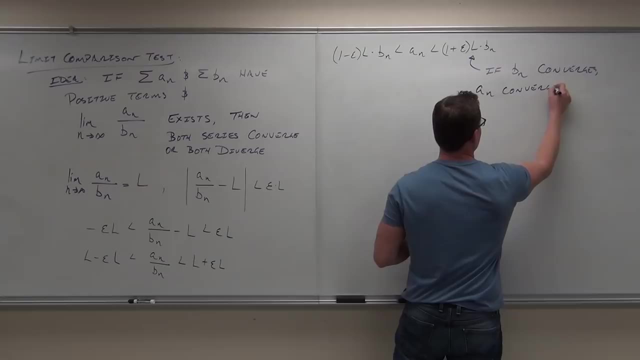 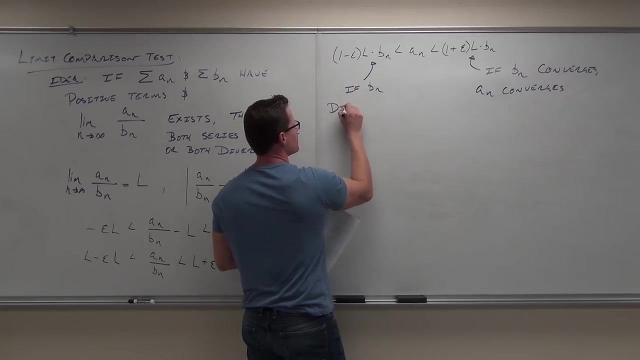 by the way, this is a constant. It's not going to affect the convergence of our series. It'd just be our series multiplied by whatever that constant is. If b sub n diverges, a sub n also diverges. Now, of course I haven't done an example with this. 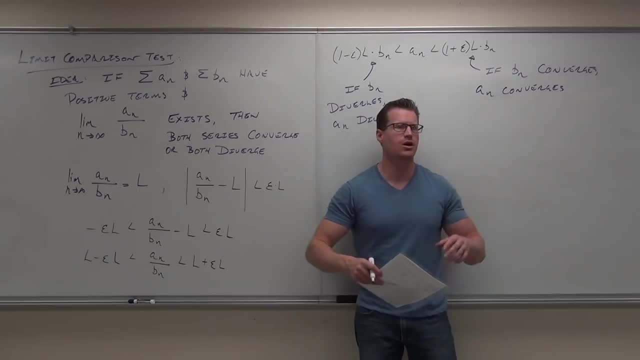 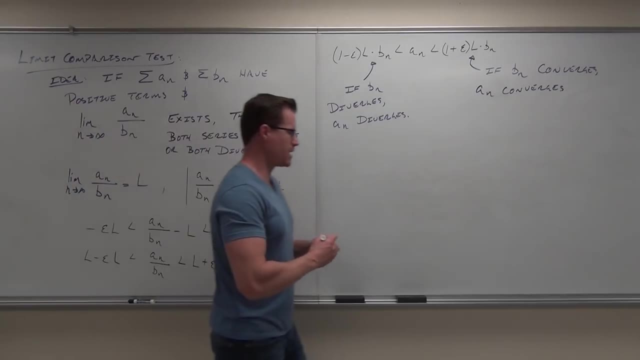 but we're going to do that last example I had with our limit comparison test. So here's the whole kind of put everything together moment for you, The first thing we start with all the time. the first thing we start with all the time is what? 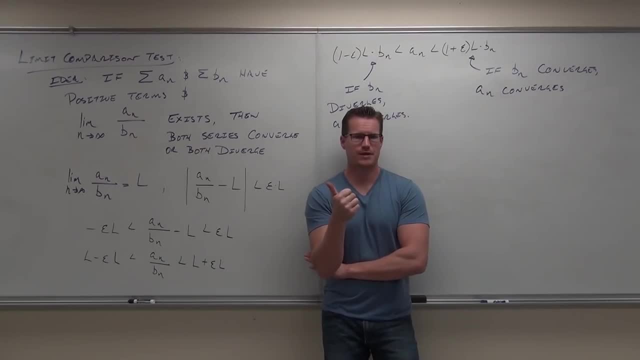 Limit Divergence. Just take a limit. If it doesn't equal zero, you're done. It diverges. After that, start thinking about easy stuff. okay, Is it a geometric? If it's geometric, do it, Goodness sakes. 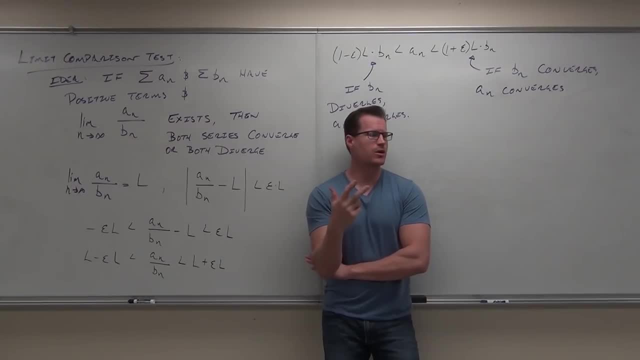 Is it a p series? Is it harmonic? If it's not one of those things, then we start talking about: okay, well, can I do an integral test with it? Maybe I can, If it's positive, continuous decreasing. 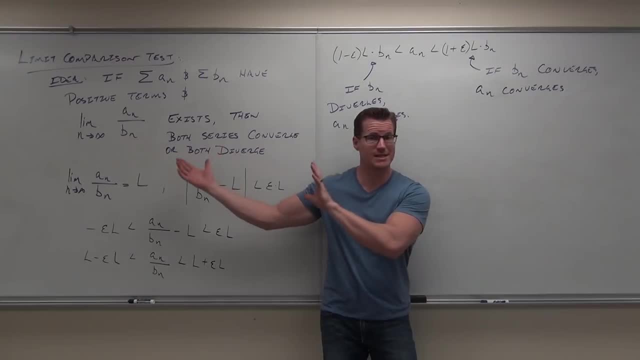 integral test works real nice. If it's not one of those things, or maybe it's easier to do this, you go okay. well at this point, I think. well now, with the comparison test, is this always smaller than a series that is convergent? 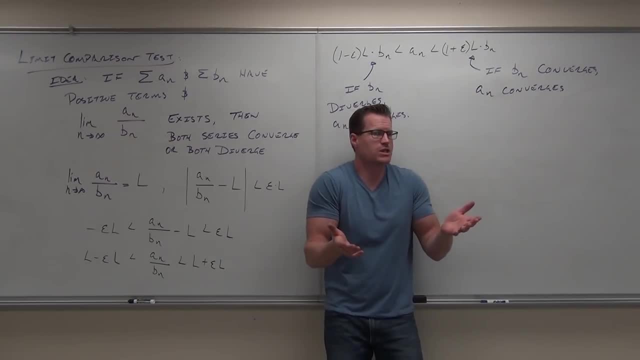 or is my given series bigger than a series that's divergent? If it is man, we're done. If that's not the case, if you go, man, and now I have something that's smaller than divergent or bigger than convergent. 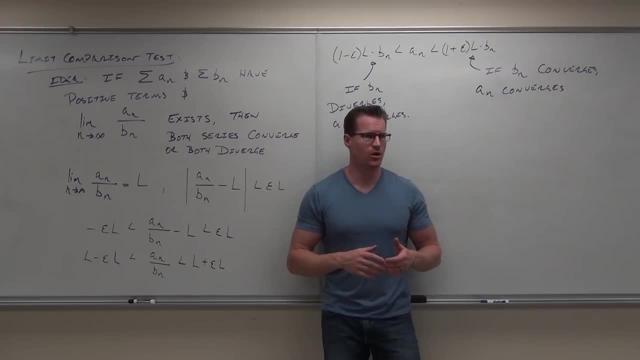 I can't really use the comparison test straight up. then what we do is we go. well, maybe a limit comparison test would work. We'll say this one's so close to the other one, so close. they'll take a limit of the ratio of them. 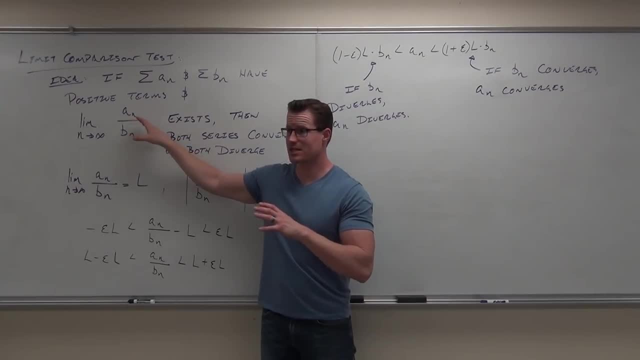 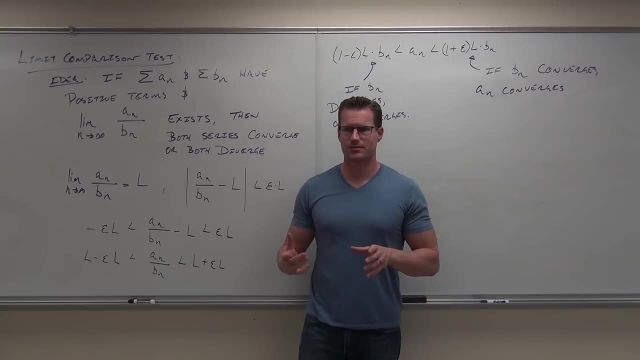 If I take the limit of the ratio of my series, then if that limit exists, my result will be the same for both my series: They will both converge or they will both diverge. Does that make sense to you? Question These tools. can we do anything? or are there some that are just? 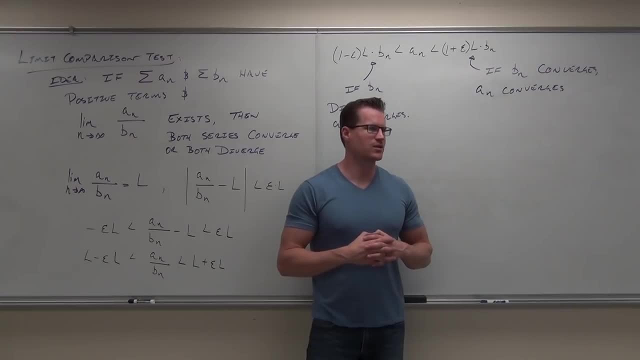 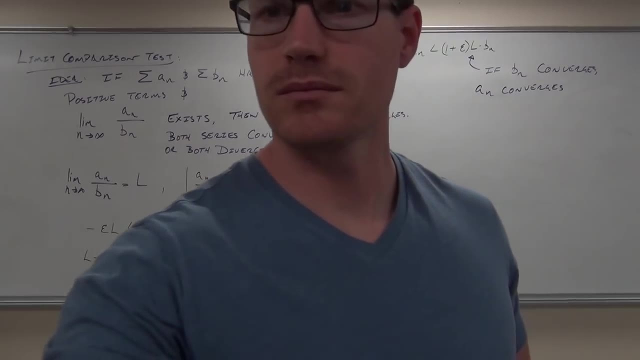 Can I do anything? No, there's other things, other techniques. I'm going to show you You can do a lot with them. I'll put it that way. Okay, All right, so let's wrap up this example. So what we learned was that oftentimes, 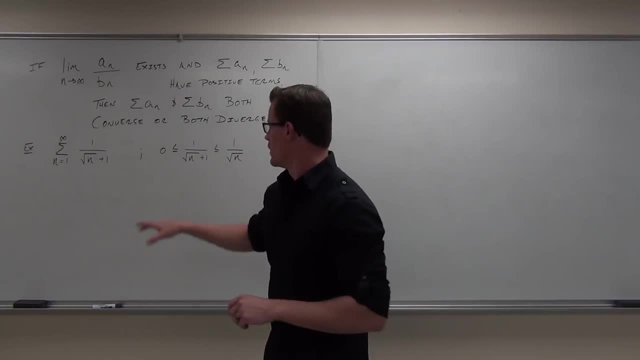 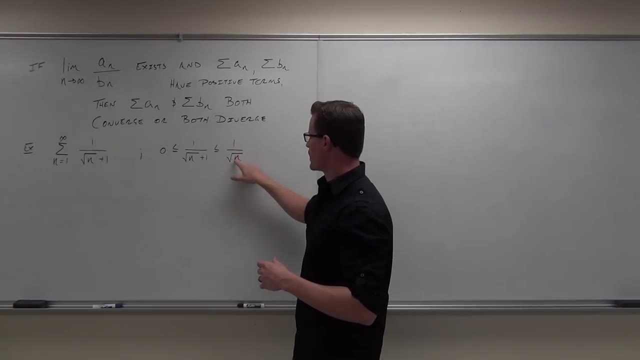 we can't use the comparison test just like it is. For instance, when we did, when we tried the comparison test with this particular series, we said: sure, the terms are positive, that's fine, sure, it's less than 1 over the square root of n. 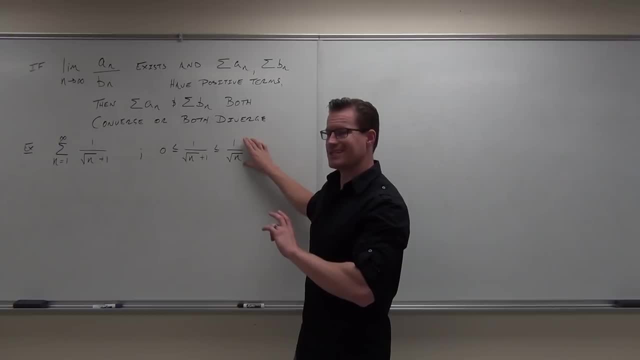 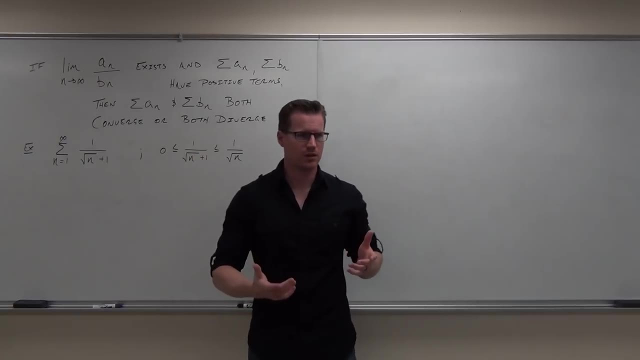 However, because 1 over the square root of n, that series diverges and it's bigger than the given series that we want to show convergence or divergence for, that doesn't do us a whole bit of good because, well, if this is bigger than the series and this diverges. 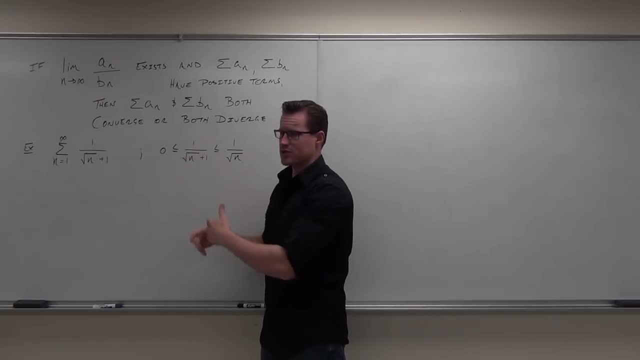 it's not forcing this one to do anything. Therefore, the comparison test by itself won't really work. We need something that, if we have our given series smaller than a series that converges, that's good, or bigger than a series that diverges, that's good. 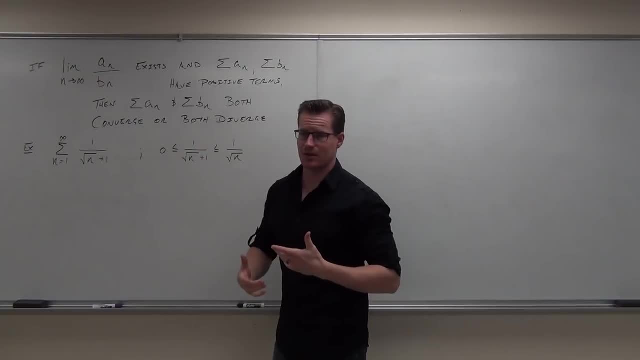 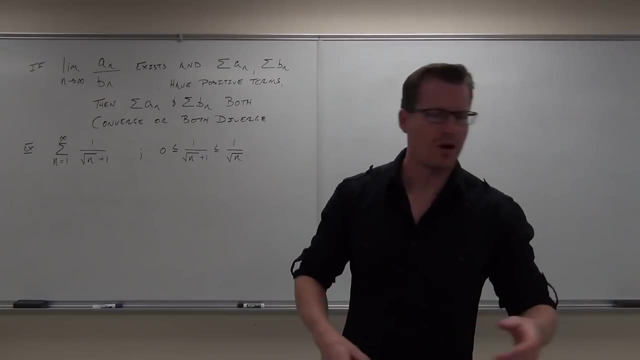 But smaller than a series that diverges doesn't do us anything. So we invented this new thing. We said all right, well, if the comparison test doesn't just straight up work, let's try the limit comparison test. So we said: all right, no problem. 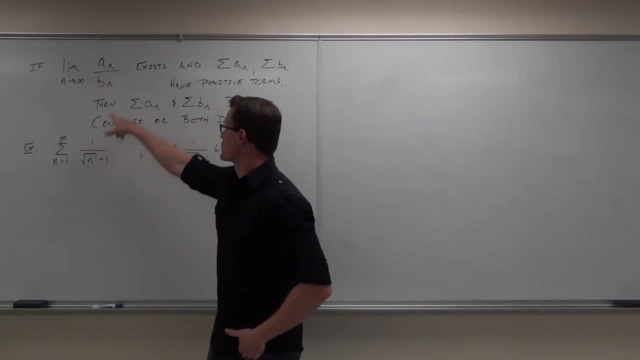 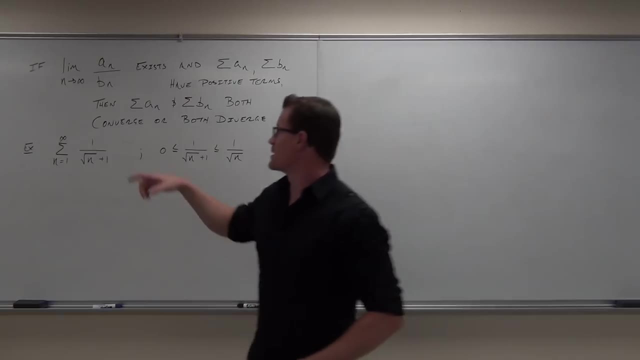 Let's compare these series in a ratio. no problem, just some sort of fraction here. and let's take the limit as n approaches infinity, If that limit exists. what that means is that these series are so close together that the ratio is 1 over the square root of n. 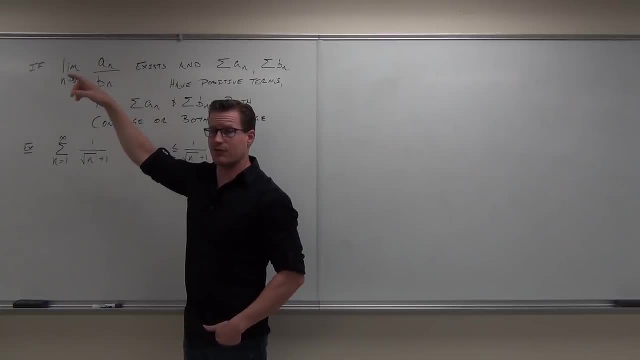 So we're going to do that. So we're going to do that. The ratio exists as some number. They're so close together that if one converges, the other one's tied to it, and if one diverges, the other one's tied to it. 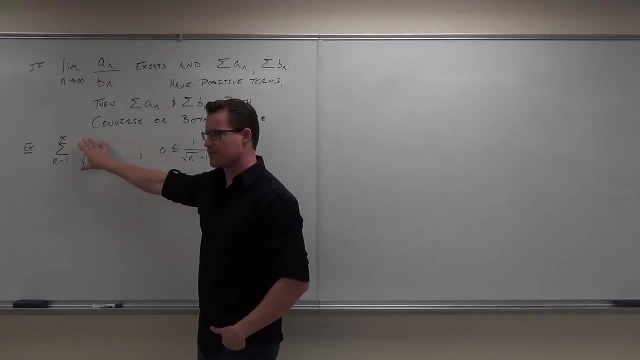 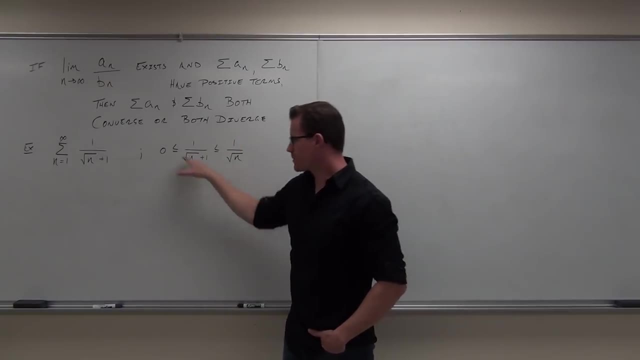 So basically, what we do is we compare our given series to one that we know the convergence or divergence for and take the limit of it. It's not a straight-up comparison test that's saying it's always less than or greater than, because that won't work in this case. 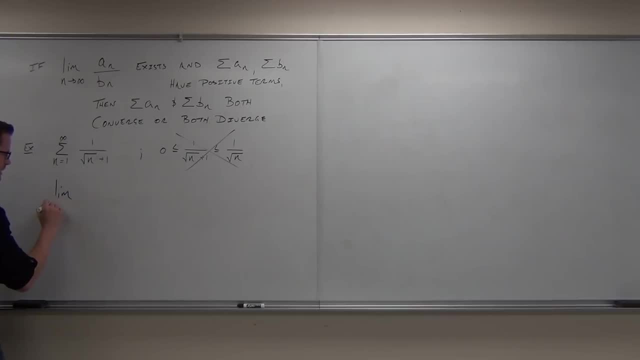 But if we take the limit and we say, all right, tell you what. By the way, a sub n is always your given series, always what you start with, b sub n is always something you're trying to base your series on. that you know the convergence or divergence for. 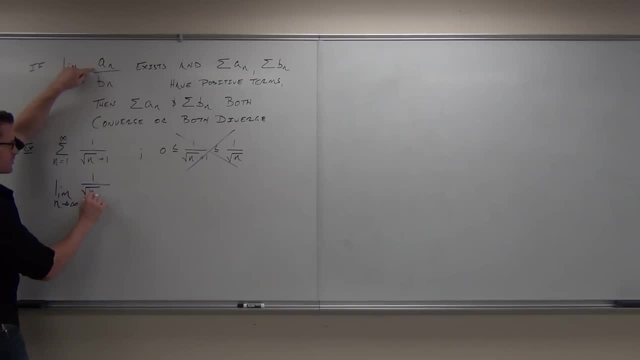 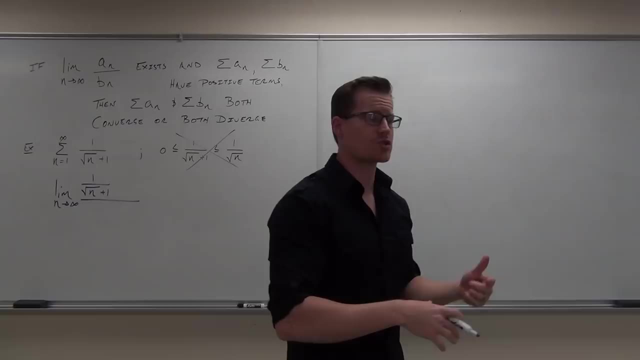 So we say, all right, our a sub n here is 1 over the square root of n, plus 1 over something that looks a whole lot like our series, that we know the convergence or divergence for. So namely, we say, all right, well, let's compare it to the 1 over the square root of n. 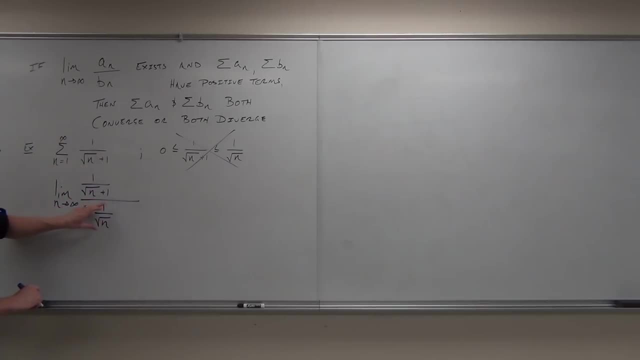 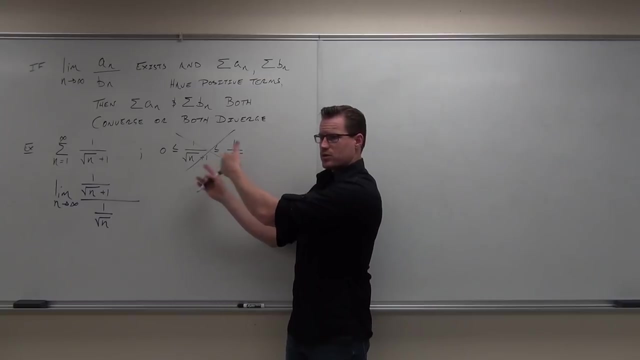 This thing's going to behave a lot like this. That's where we're getting this from. Are you guys okay with this so far? Show of hands if you are. So it's looking just like this, right? only we're not doing a comparison test. 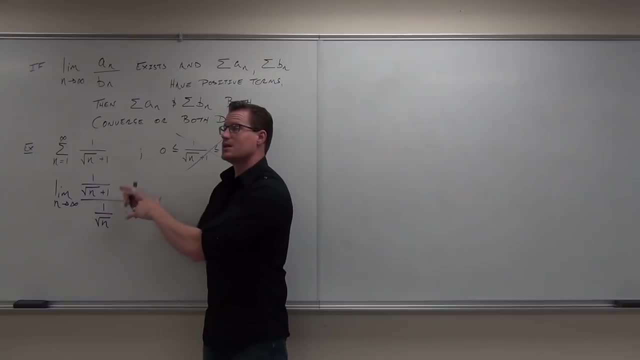 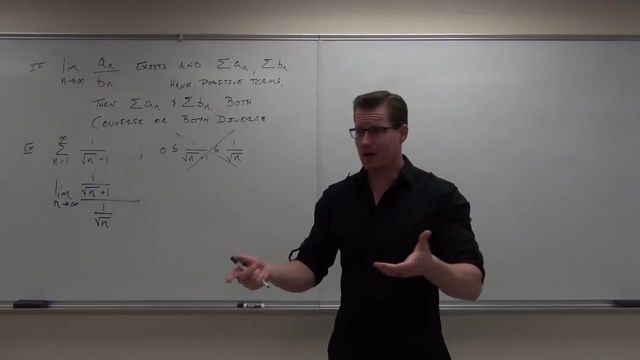 as it's always less than or greater than. We're doing a comparison test as far as the limit's concerned. That's why it's called a limit comparison test. We're taking the limit of this comparison. So far, so good. Do you know how to do limits? 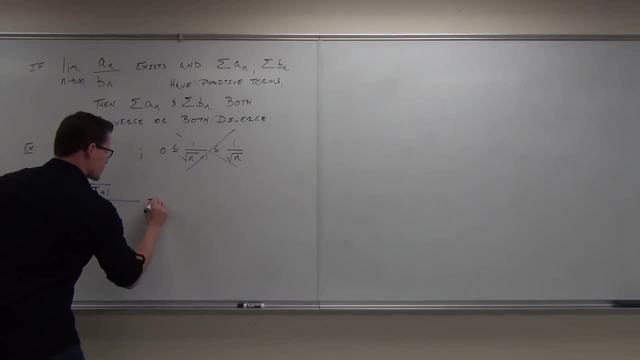 Mm-hmm, Of course you do So. we'll just make this thing simpler. Since we have a complex fraction here, let's make this: We'll reciprocate and multiply 1 over the square root of n plus 1.. 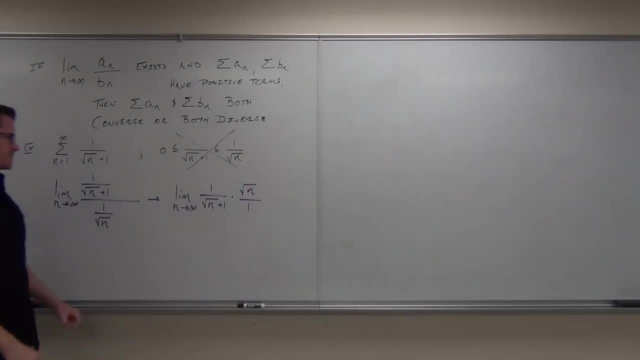 Excuse me, Bless you, Thank you. Times the square root of n over 1.. All right, well, that's going to give us a limit as n approaches infinity, of the square root of n over the square root of n plus 1.. 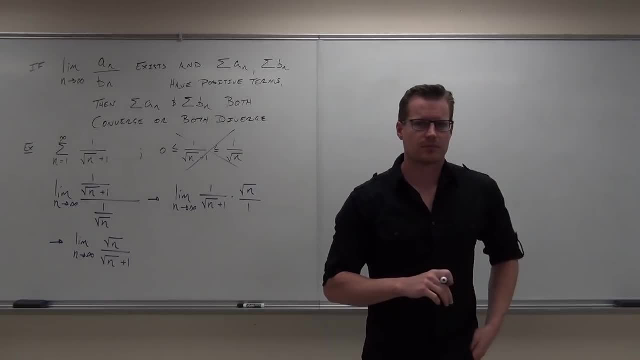 Tell me something about that. What's the limit? Infinity over infinity. Okay, tell me what you could do. What would the problem be? You could, if you wanted to, Now notice that you have the same thing over the same thing, right? 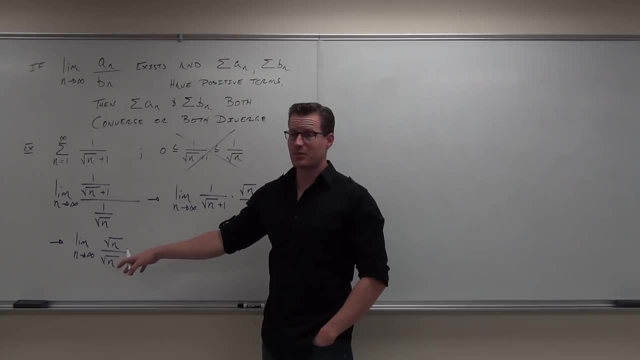 So that might be an issue for you. I don't know, Maybe something a little bit easier, something that we think about: Can't split this one up, because our denominator can't be split up. So we can't do that. What we could do is maybe just divide by the largest power of the denominator. 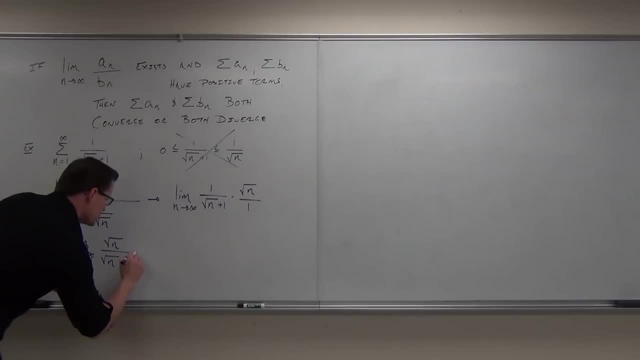 which is what we typically do with these things anyway. So if we Divide by the largest power of the denominator- I think Frank said that in the back- If we divide we're going to get the square root of n over the square root of n. 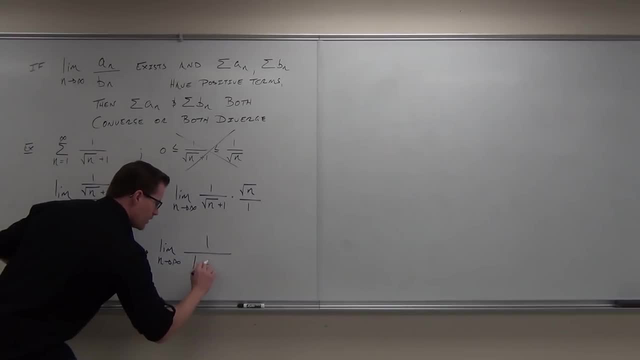 That's 1.. We're going to get the square root of n over the square root of n. That's 1.. We're going to get 1 over the square root of n, And that saves us a whole lot of time. 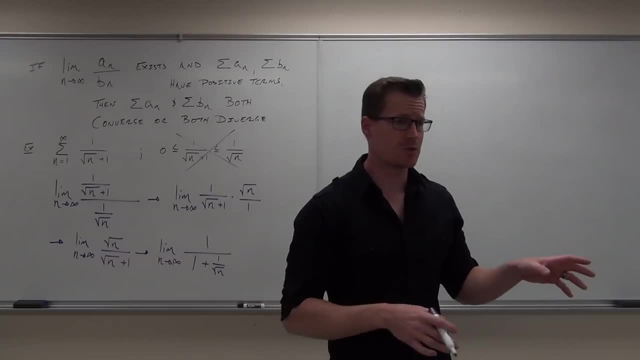 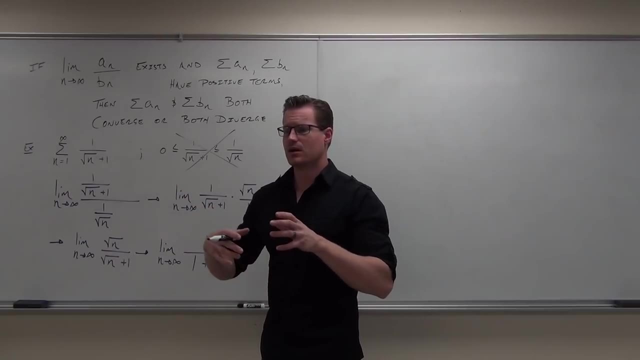 We don't have to worry about L'Hopital's rule, So don't skip some of the easy stuff when you're doing these limits. Oftentimes it's a lot easier to just divide by the largest power of the denominator if you have something that's rational, like a rational expression. 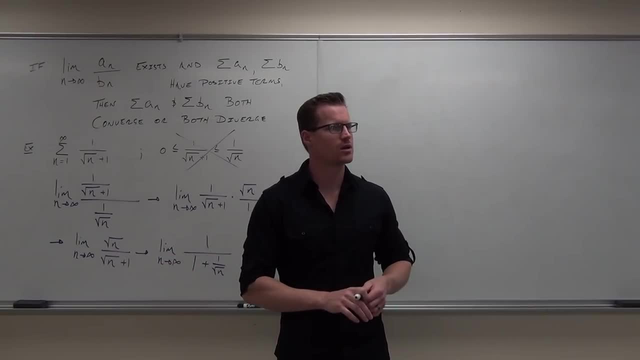 or even square roots, things like this, almost like polynomials. You guys okay with that so far, So tell me what the limit is. What's the limit of 1? 1.. What's the limit of 1? 1.. 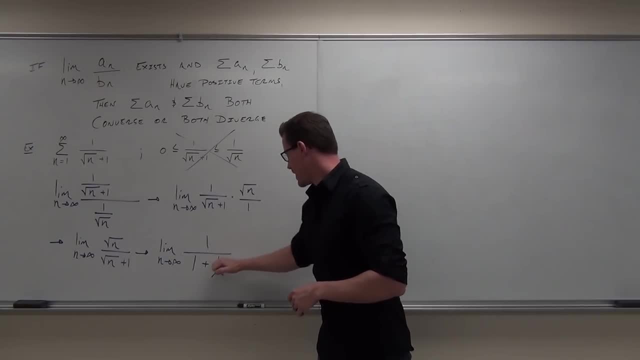 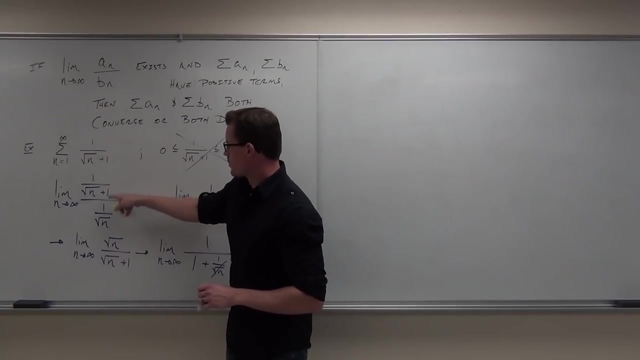 What's the limit of 1 over the square root of n as n over the square root of n? Bam, How much is this limit? 1.. Okay, Now, please listen carefully. Here's what this whole thing means. What it means is that these two things were so close together. 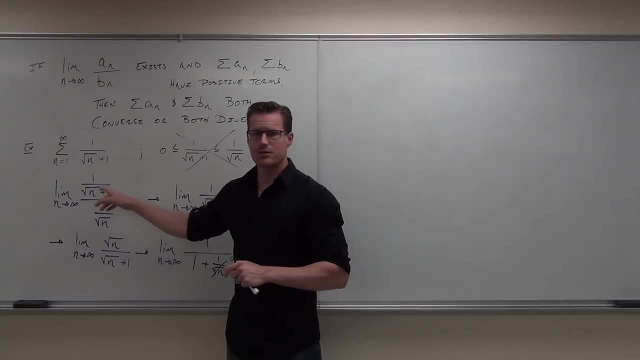 that our limit existed. It also means they're so close together that if one converges, the other one has to converge, And if one diverges, the other one has to diverge. So please do not make the mistake of doing this. 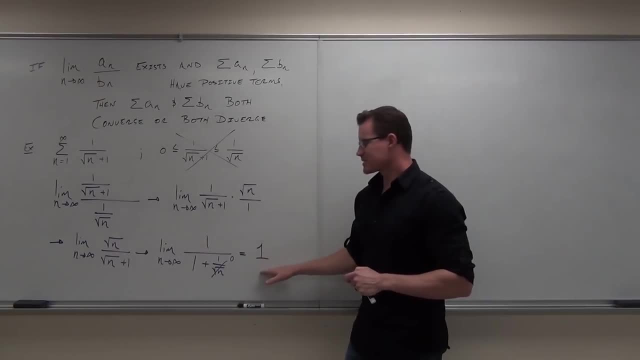 Do not make the mistake of saying, hey, the limit exists, therefore it converges. That is not what we're talking about. What we're talking about in the limit comparison test is: since the limit exists, they will both have the same result. 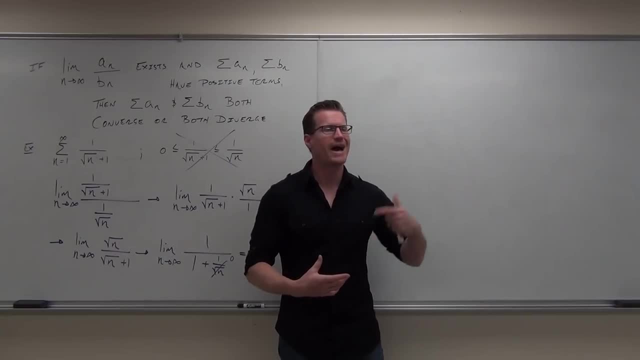 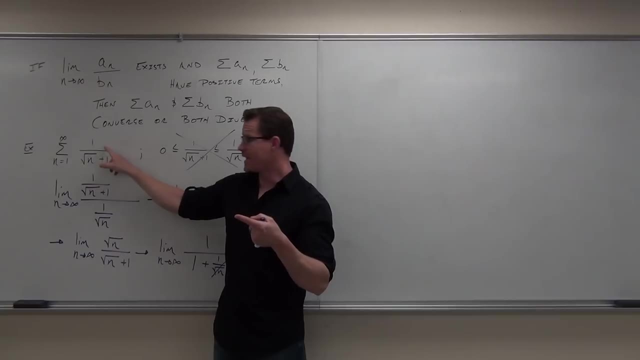 They'll both be convergent or they'll both be divergent. That is what we're talking about. That is why you compare your given series to one that you already know. the convergence or divergence for Say hey, you know what? 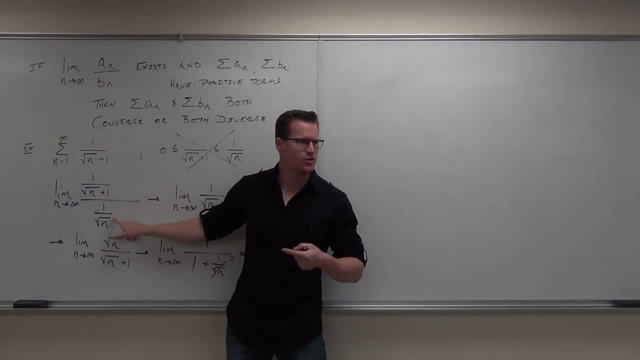 I know this one. What is that? Is that convergent or divergent? Divergent, That's divergent. Why? P series Very good And the P is So. it's a P series of P less than 1.. 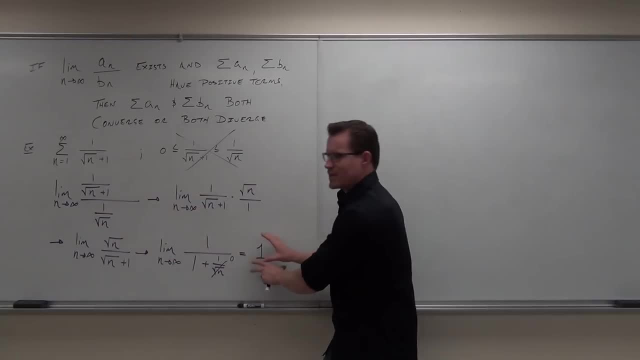 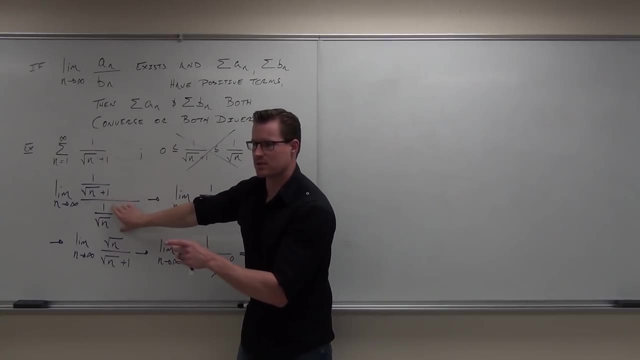 True, That's divergent. So what this says is: this doesn't mean it's convergent. This means that this thing is going to have the same result as what you're basing it on. That's what it says. So if the limit exists, we go okay. well. 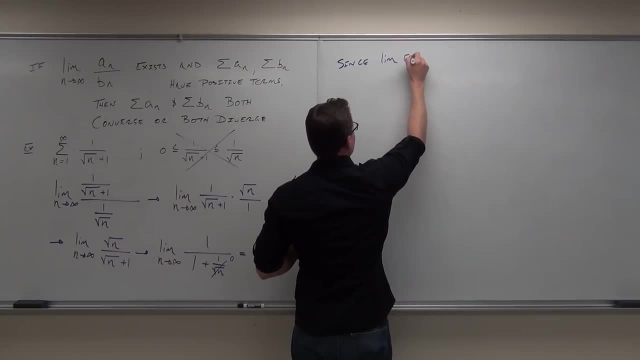 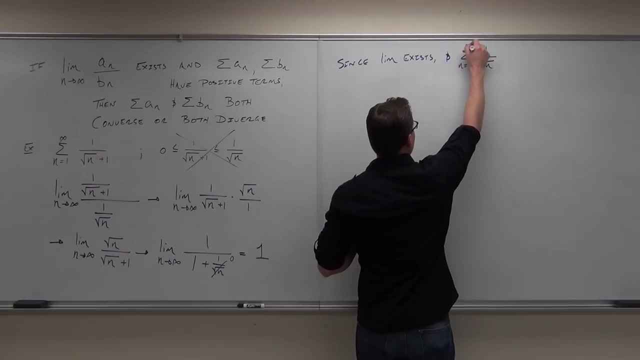 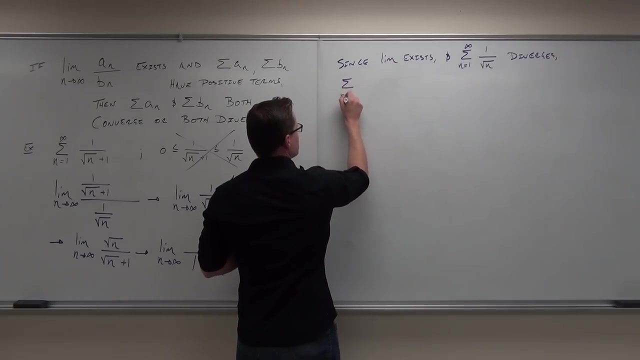 since the limit exists, since they both have positive terms, which they both do. we already checked that earlier. since the limit exists and the series of 1 over the square root of n diverges, the series of 1 over the square root of n plus 1 diverges from 1 to infinity. 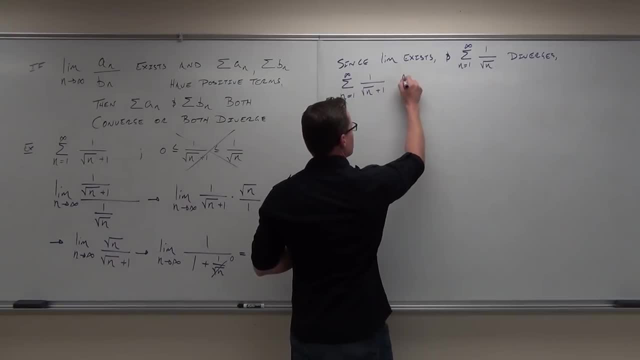 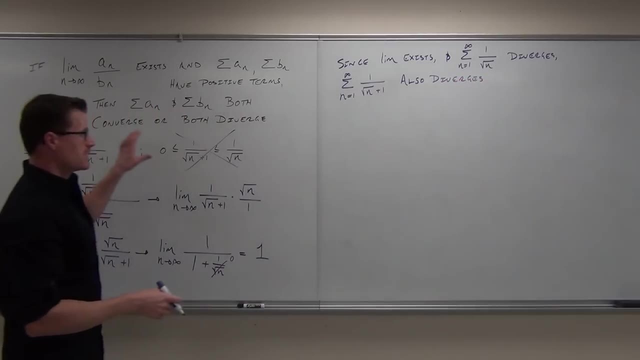 of 1 over the square root of n plus 1.. Tell me something about that one, then. Divergent Also diverges. So is that right? The limit exists. They're tied together so closely that they're going to have the same result. 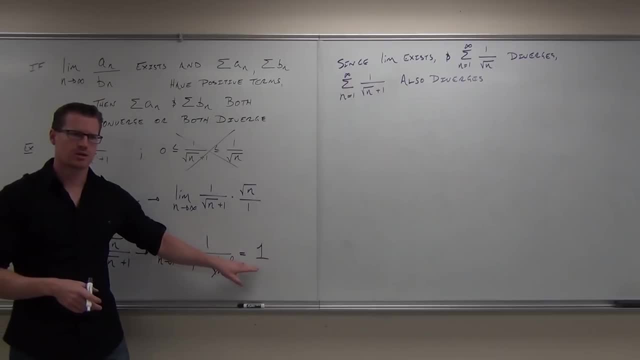 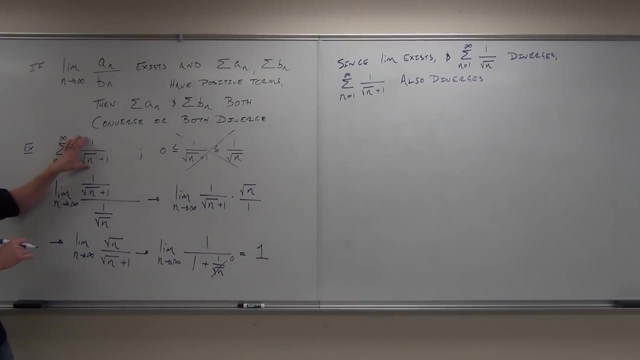 Either both converge or both diverge. A limit existing here for the limit comparison test does not automatically mean conversion. That's not what it means. What it means is that whatever your series is and whatever series you're, basing that on both converge. 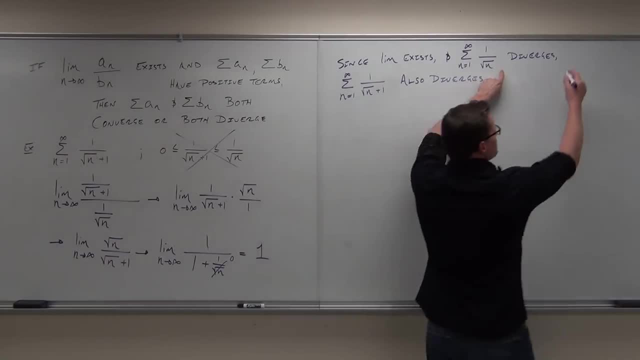 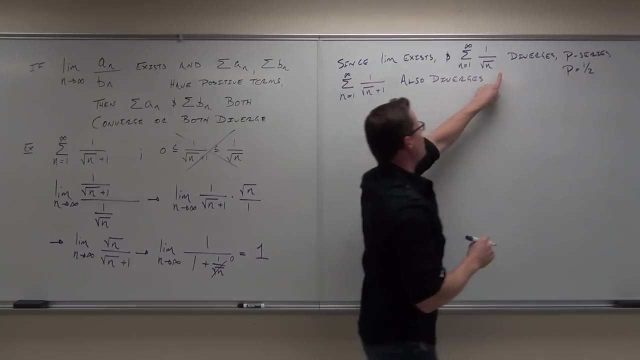 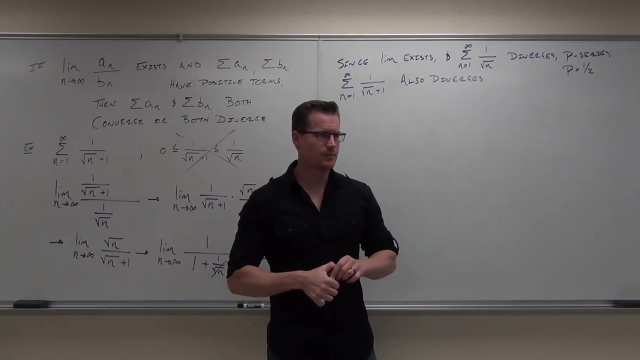 or they both diverge. If you know one of them diverges because this is a p-series with p equals 1 half, then you know this one also diverges because that limit existed. of that ratio Question. I'm kind of confused. 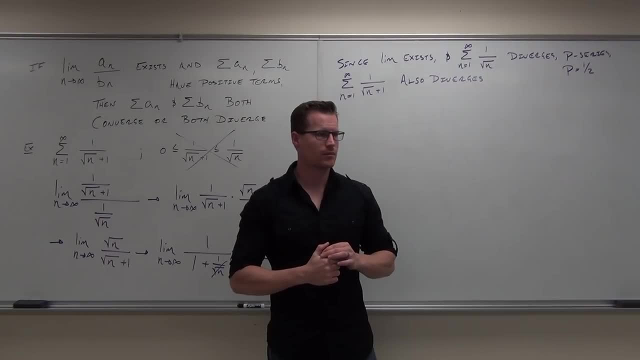 When we do limits and say we had 1 over x squared, took the limit as x over infinity, what would that mean? We say that that's 0, right, True. But then we do like series and it's like a p-series, like that. 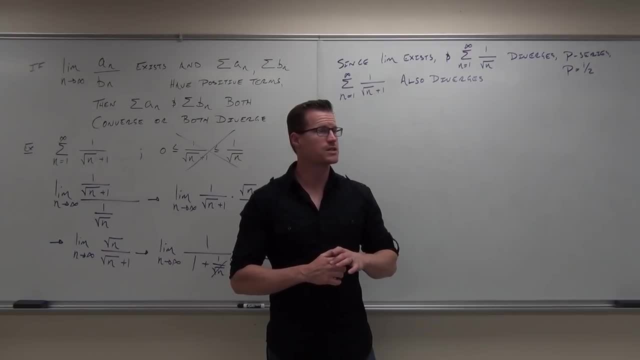 We say that it converges. The p-series does converge, But does it just converge to like 5 or something, or something like that, where it would be infinity anyways, I don't know. Well, the p-series converges, but a series is different. 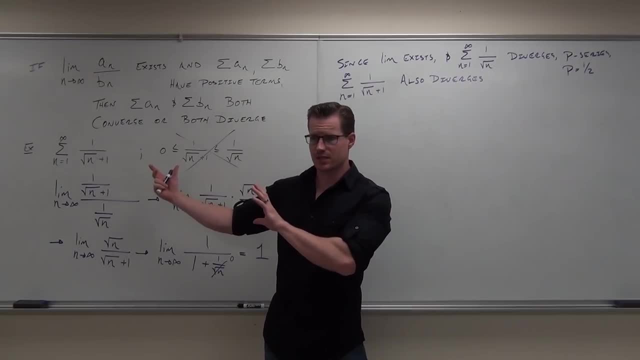 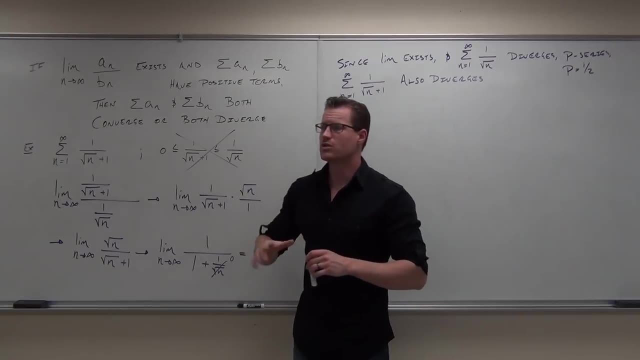 than just a straight-up limit. Now we check a straight-up limit on the series just to see that the sequence is going to converge. So try not to get confused with sequence versus series. okay, What we do immediately with the divergence test is say: hey, 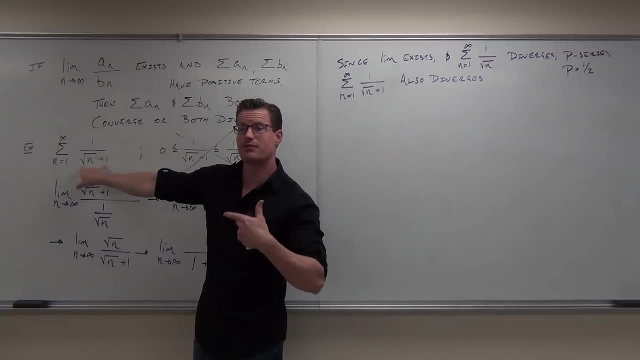 look at your sequence of numbers. This is the divergence test. Does your sequence go to 0?? Yes, it does. That means that ultimately, for our series, what we're adding up are values that are 0. Now, the series itself is not going to go to 0. 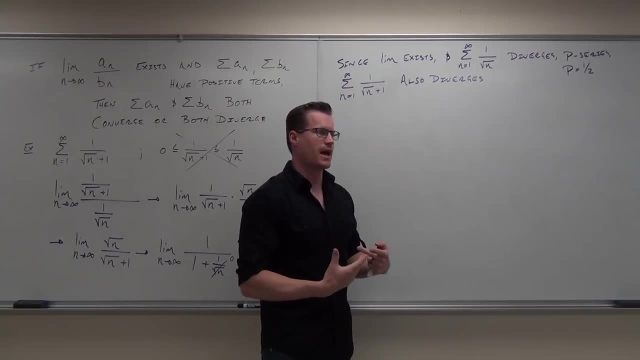 The series itself is going to add up a number of terms. I don't know what that's going to add to. in a lot of these things I do if it's geometric, because we can find the sum of that okay, But I don't know. 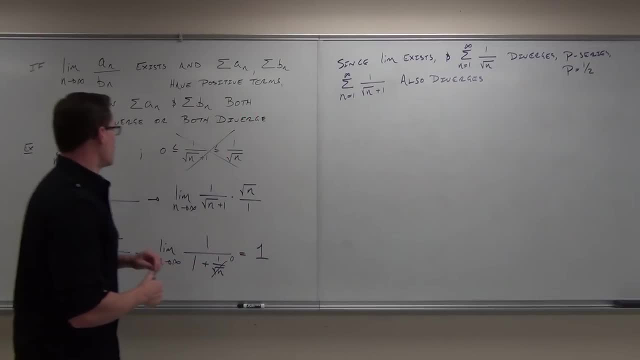 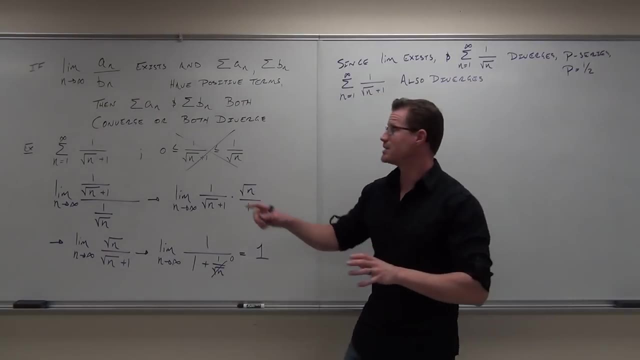 I don't know what that's going to be. So when we're taking a limit here, we're not actually finding a sum, We're not actually finding out whether it's equal to 0 or not. We're not actually finding out, basically anything besides these. 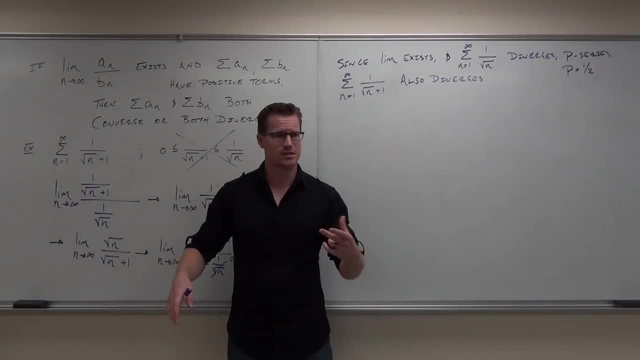 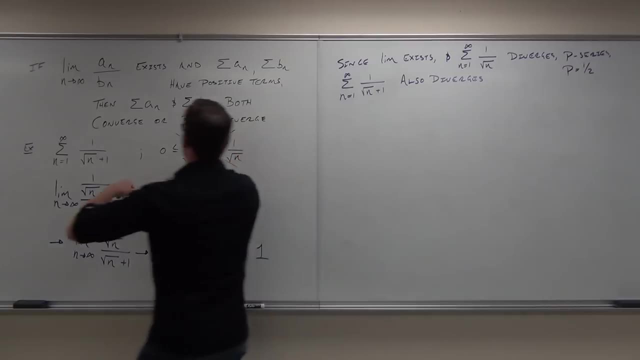 things are really closely tied together. That's what the limit comparison test does. It says these things are really closely tied together. Does the limit have to equal 0 for this to work? No, No, it just says that it has to exist. 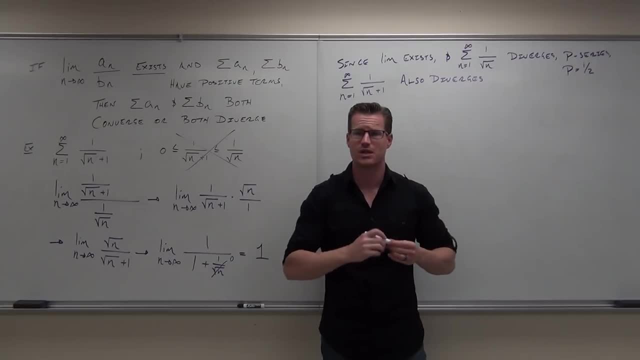 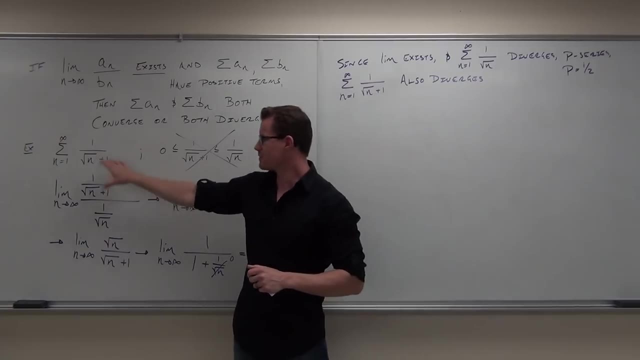 It can't be. infinity, Can't be, does not exist. okay, It's got to exist to be a number. If it's 0, cool. If it's 1, cool, I don't care what it is, As long as it's a finite number. that means these are tied together. 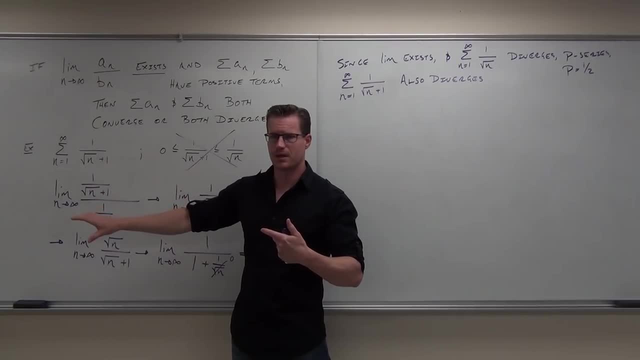 and the divergence, or convergence, will be the same between our two series. Now, when we're taking a limit of a series, like when we did the limit of this one, again, what you're just saying there is: the divergence test says the sequence from which your series is built has to go to 0 because ultimately, 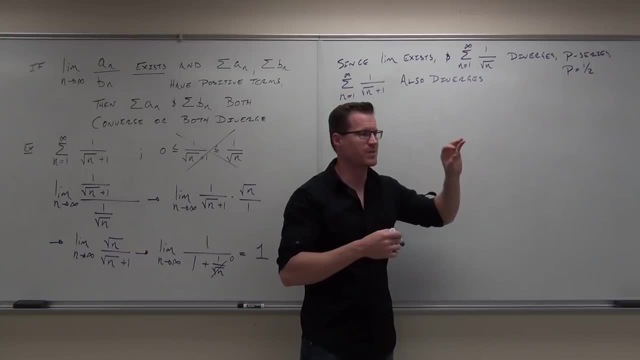 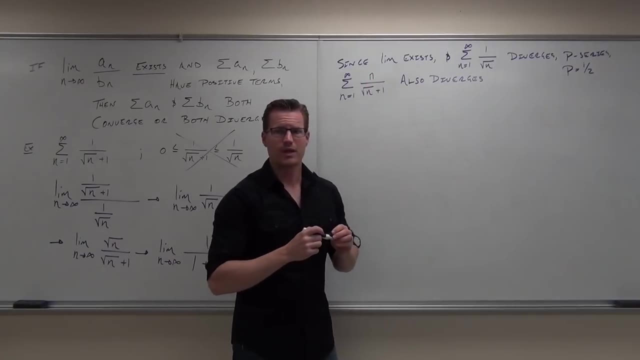 you've got to add up terms that are close to 0 for it to make sense. Does that make sense? Does that make sense If we would have had something like n over the square root of n? we add up terms that ultimately, would lead us to infinity. 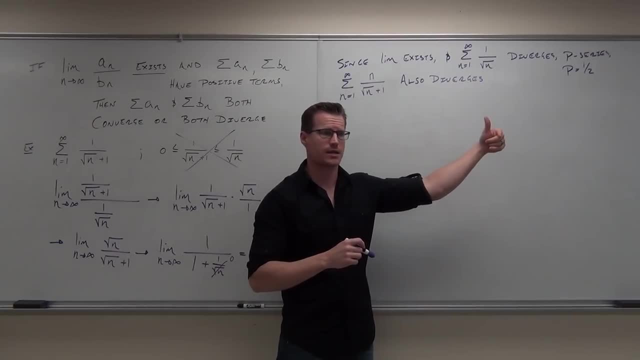 That means that our series would go towards infinity as well, and we would not be able to add that together. We would not be able to find a series that converges. So convergence for a series just means that ultimately, you're going to be adding up terms that are 0, so ultimately, 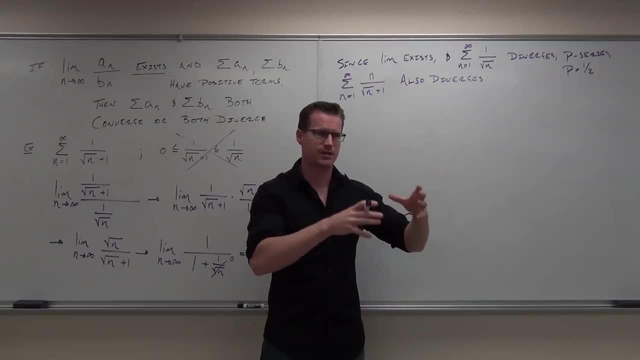 you'll come up with a sum that is not infinity, that is an actual finite number. Did that clear something up for you? Yeah, Okay, I know it's a little confusing, because we talked about sequences right, And now we're talking about sequences, kind of. 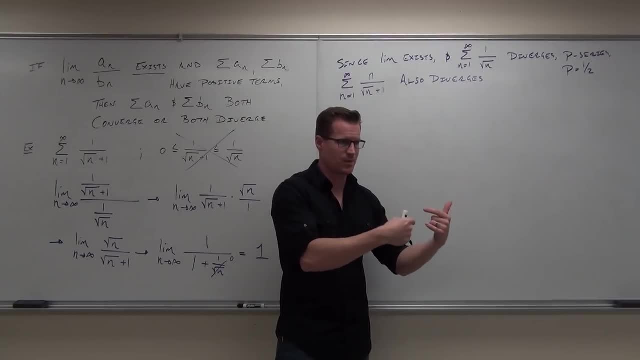 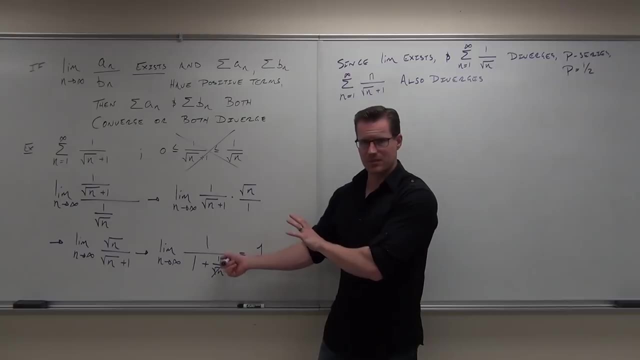 but we're adding the terms together, So some of the things are along the same line, and now I'm bringing up limits again and saying, yeah, the limit doesn't have to equal 0. It doesn't And it doesn't mean that if a limit exists, we're getting convergence. 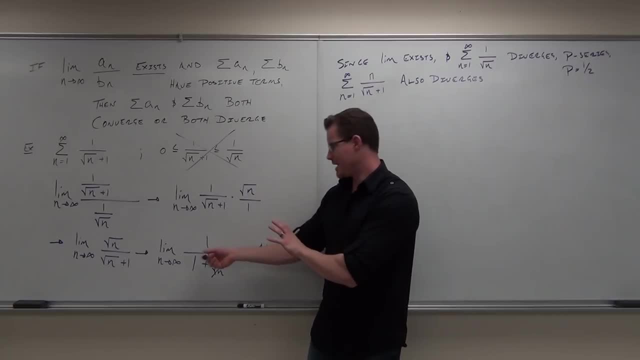 It doesn't mean that if a limit exists, we're getting divergence. You have to read the problem. You have to say, hey, this thing, if it exists, these two series will have the same output. So you're going to have a series that's going to have the same output. 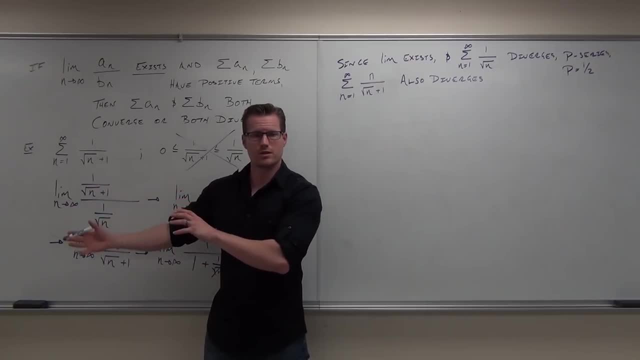 So you're going to have a series that's going to have the same output. So you're going to have a series that's going to have the same output, whether one's divergent, the other's divergent, where one's convergent the other's convergent. 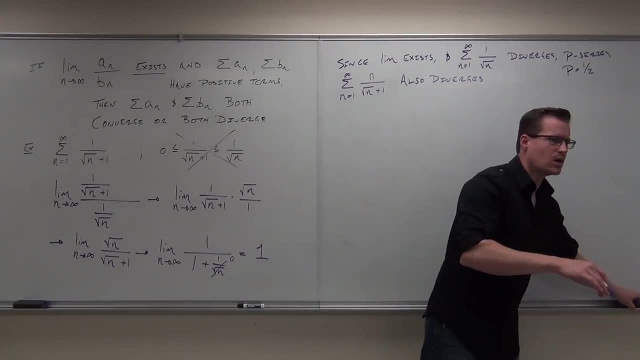 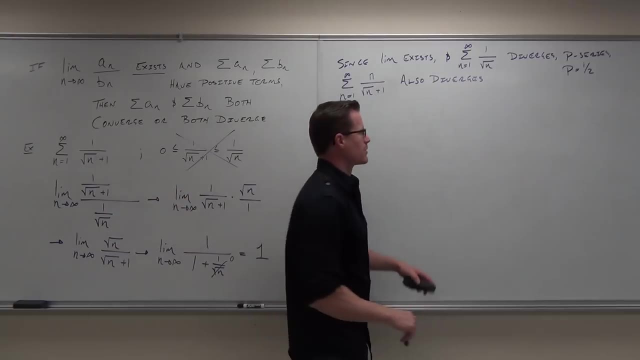 So it's a little different idea. We're using a limit here not to show convergence or divergence. We're using a limit here to show that they have the same convergence or divergence, And I proved that theorem last time. Okay, Anyway, I'm going to move on here a little bit. 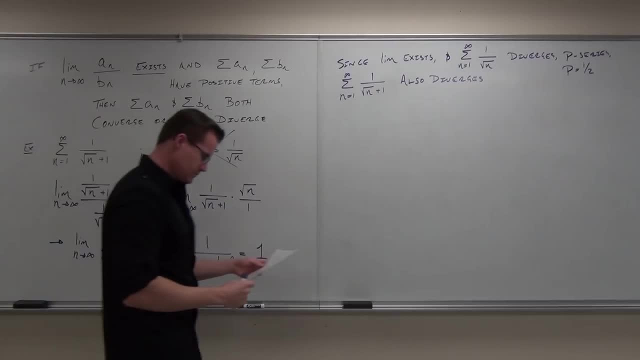 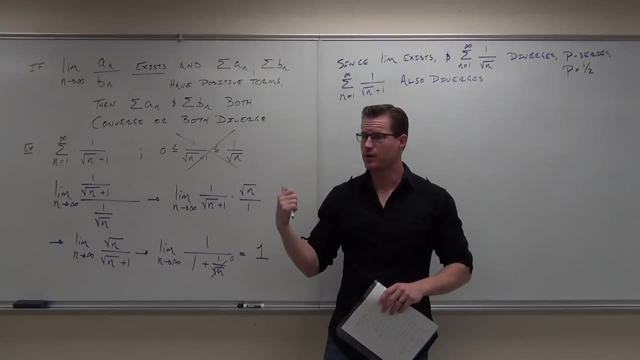 I'd like to get a couple more examples out of you. Let's see if we can do this one. Are there any other questions? Are there any further questions? That was a good question. Thank you for that one. Any other questions before we move on? 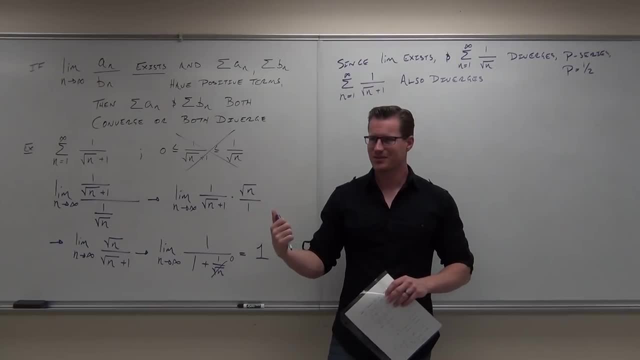 Did this make sense to most of you? Did this make sense to all of you? How many people did it make sense for Feel okay with that one Ify, Are we okay? Question? So just to further clarify: if this limit were to approach infinity or some abstract number like that, then what would happen? 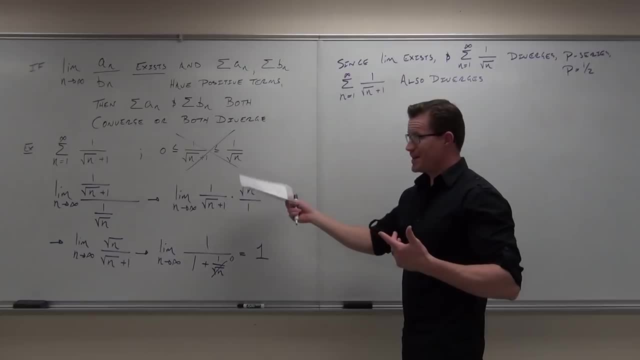 Then you can't say a thing about it. Then you might try maybe a different series. Now for us, usually we're going to pick them so that they're really close. I'm going to show you how to do that right now. 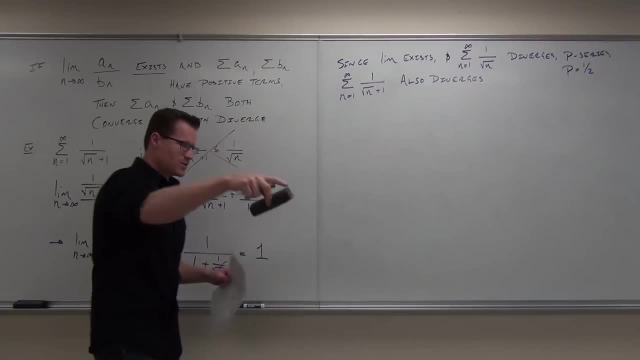 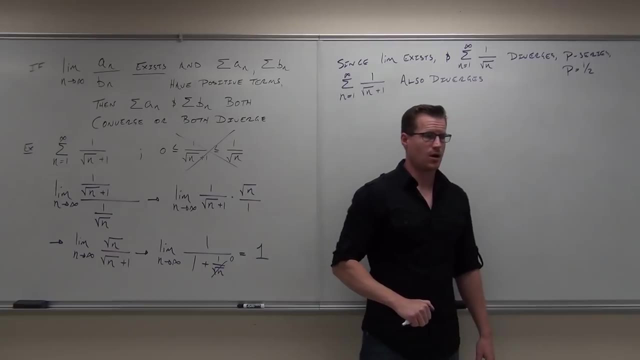 So maybe this will clear up your question. Question: Okay One and then two. So a sub n is the one that's given and b sub n is the one that you're using. right, Always Okay Question. Do you want us to answer it like that, with the sentence? 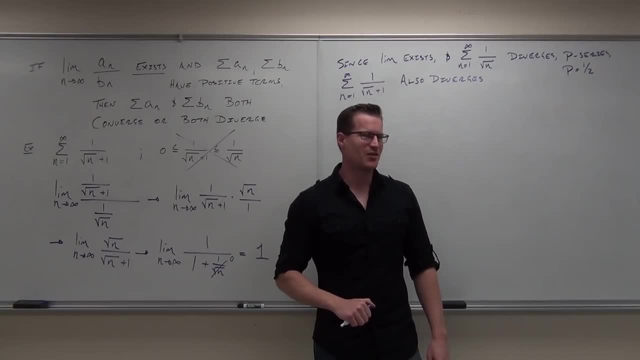 I would love it if you guys would answer it like that. I'm guessing some of you won't, But I would love it if you would answer it just like that, because that is literally what the answer is. It's saying because of the 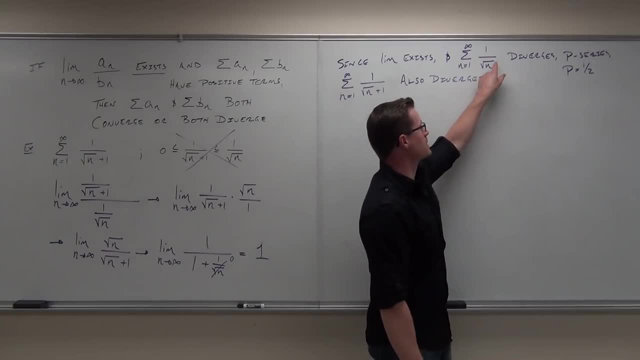 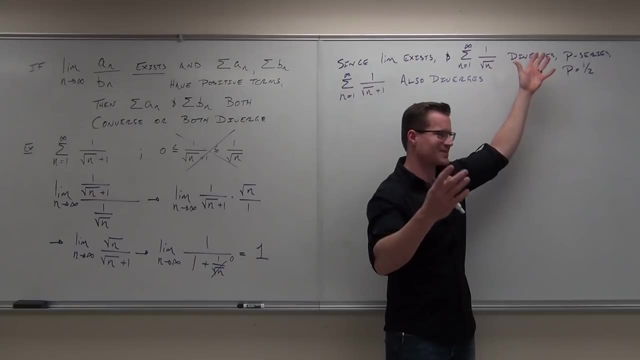 Because the limit exists, Because the series here diverges, because it's a p-series, You have to state things like this: Okay, You can't just say, eh, it diverges. You've got to state why. You've got to show me your thinking here. 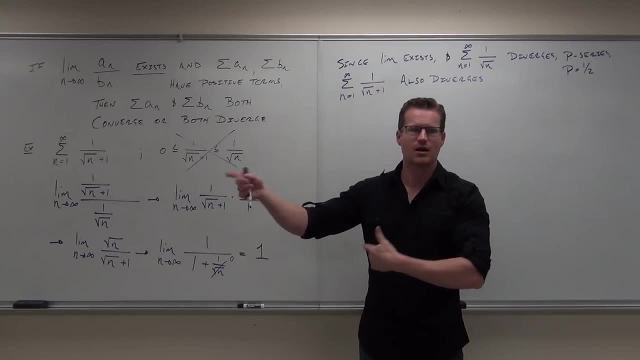 Much of this is not going to be just math work. Much of it is thinking reasoning Like: well, this is a divergent series because it's a p-series, because p equals one-half- Okay, Cool, How does that relate to what we're doing? 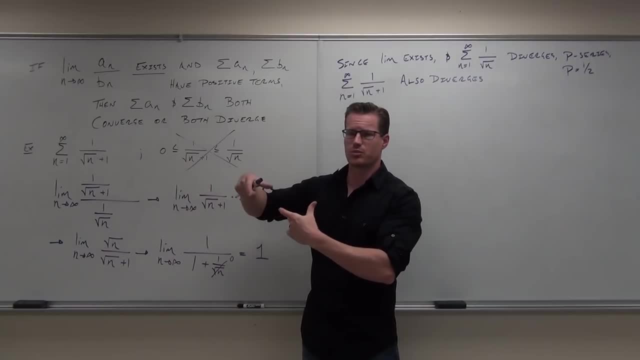 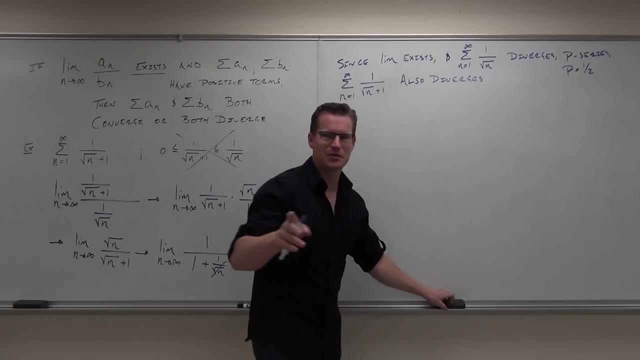 Well, because the limit exists. it says that they're going to have the same result. They're both going to be convergent or divergent. Since one was divergent, The other has to be. That's the idea. Any other questions? 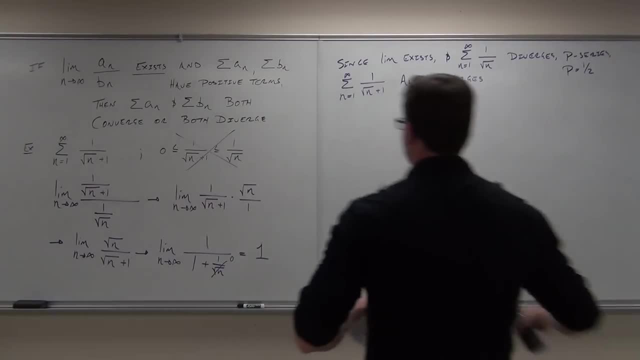 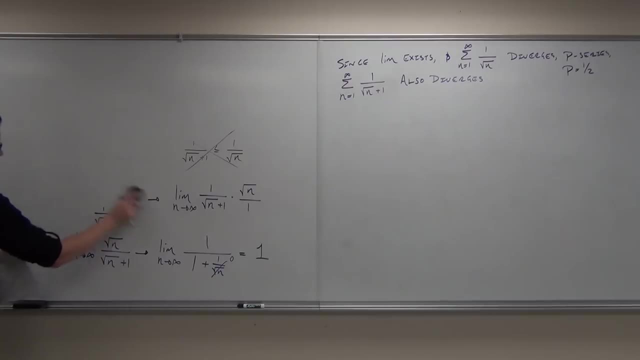 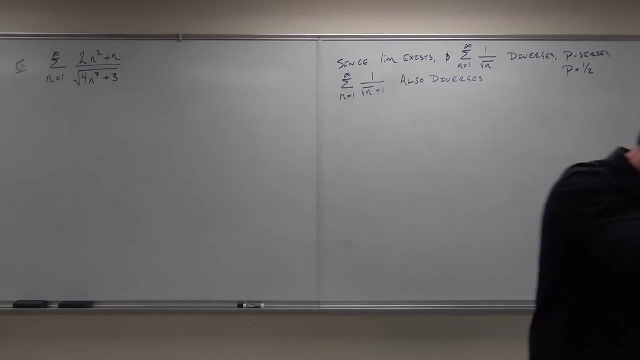 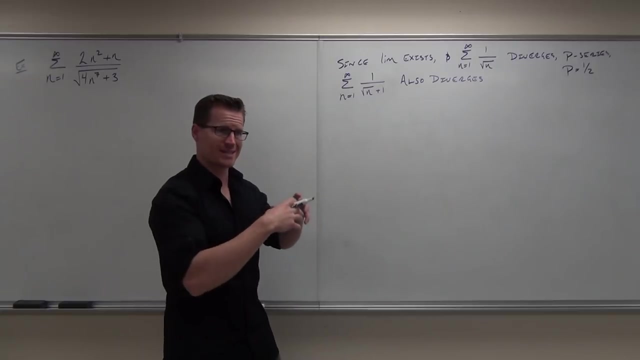 Those are all good. Let me show you another one, Last chance. I waited this time. I was nice And you go. ah man, what are we going to do here? Well, listen, we don't have to have a series. that's exactly the same. 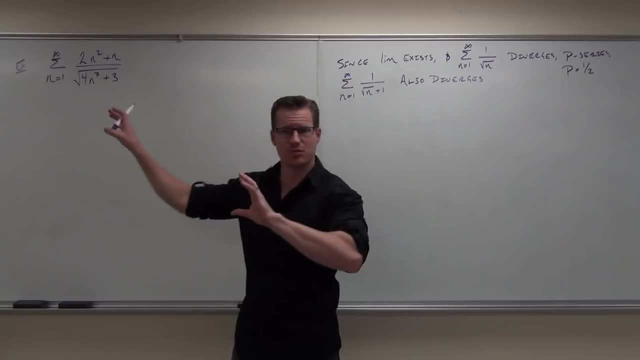 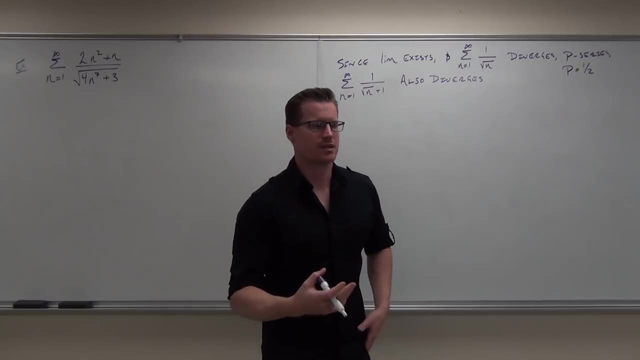 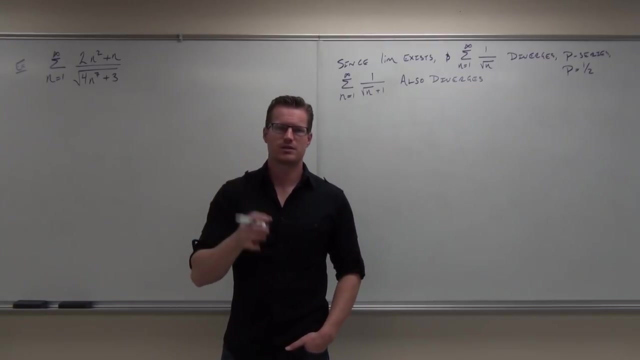 That's not the idea here. We have to have a series that behaves kind of like this one that we know the convergence for. So here's what we do When we're coming up with these, especially when you have something that's rational or kind of semi-rational, where you have almost polynomials or square roots of polynomials. listen, do you guys know anything about limits as n approaches infinity? 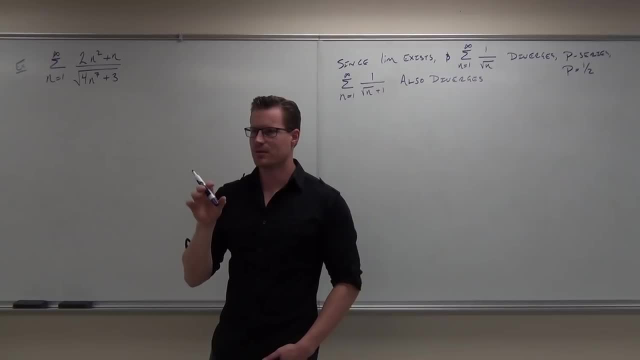 Do you know that with polynomials, the limit is dictated by the behavior of your very first, your leading coefficient, your leading term, I'm sorry, your leading term. Did you know that? Yeah, So think of the end behaviors of these functions. 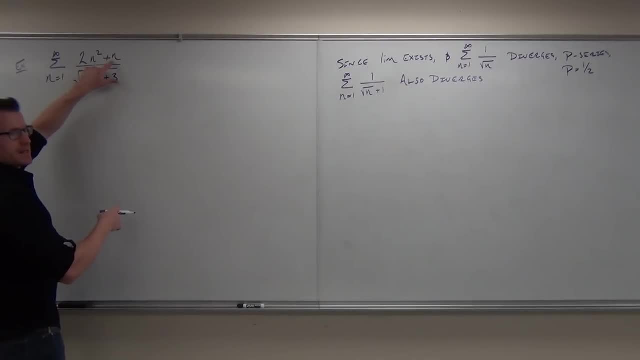 So the end behavior of this function? I don't even care what that is. Okay, The end behavior is going to look a lot like 2 over n squared. Does that make sense? The end behavior of this? does that 3 really matter as far as the end behavior goes? 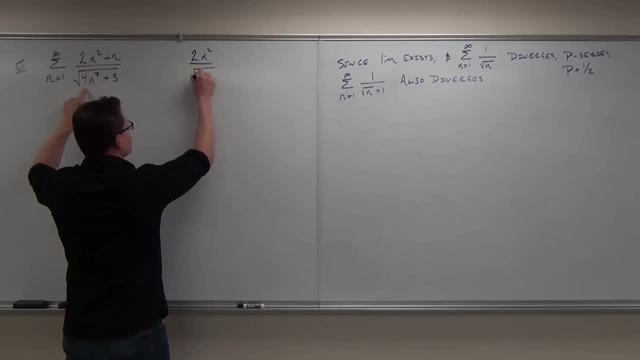 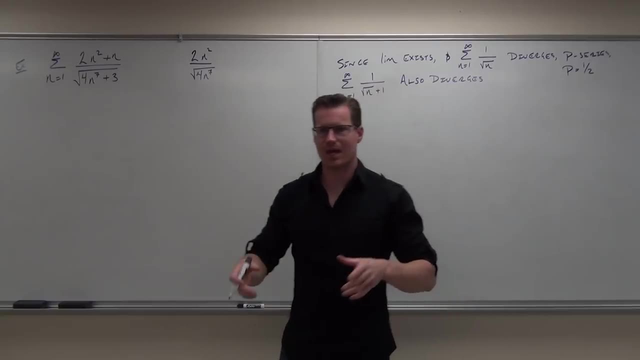 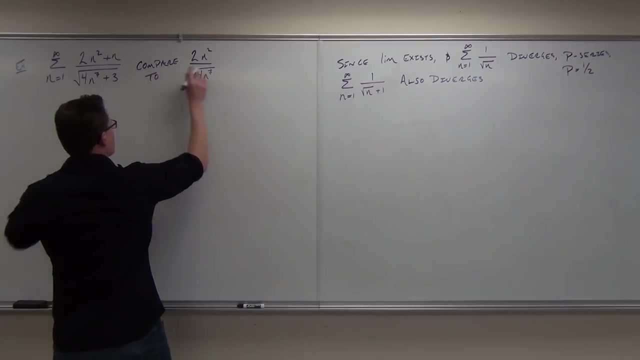 No, This is a whole lot like the square root of 4 n to the 7th. That's really what we have there. That's the end behavior. So when we're doing these, we're going to compare this to this one. 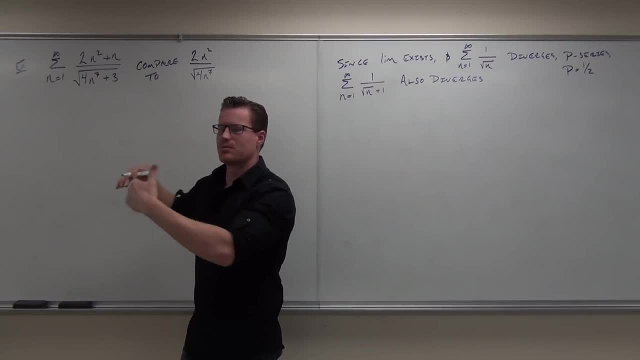 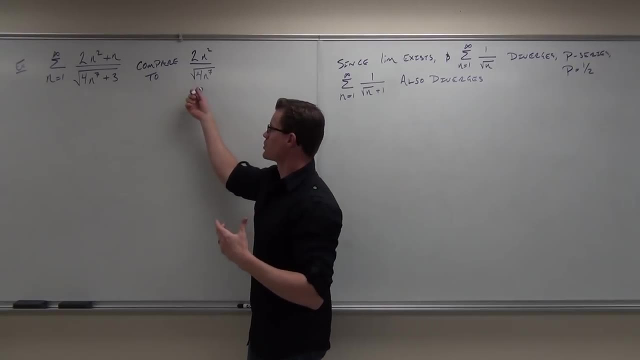 Why, Well, this is going to act really similar as n approaches infinity. Now are all the terms going to be the same. No, No. but as we get towards infinity, these terms are going to be really close to that one. 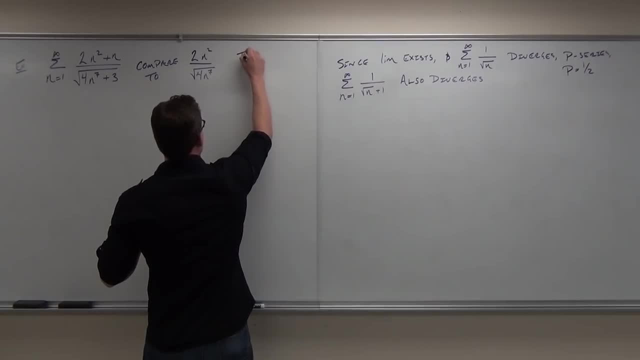 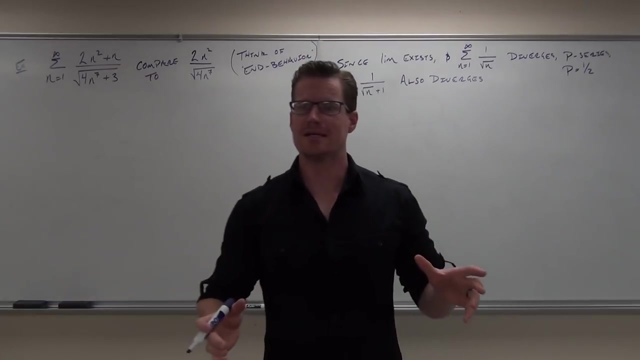 So the end behaviors will be very close. So what I want you to do is think of end behaviors Basically with polynomials. that's really easy Because it's a very simple process, Because that's just the leading term. 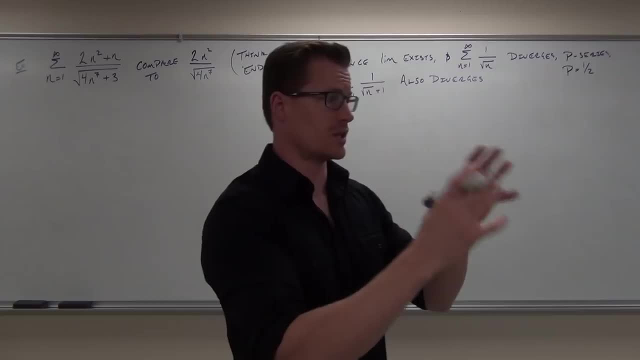 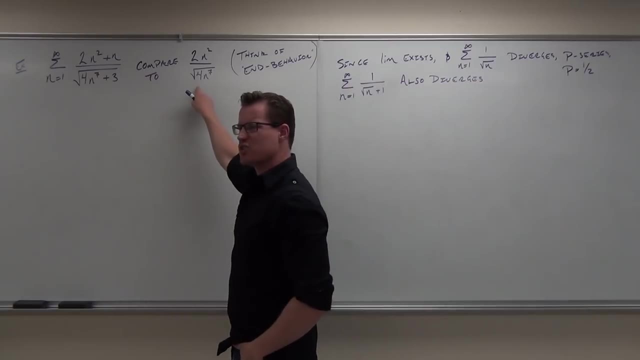 That's what a limit is. is n approaches infinity or x approaches infinity? It's just the leading term. It's the term with the largest power. That was it. So let's be kind of nice about this. Can you simplify that? 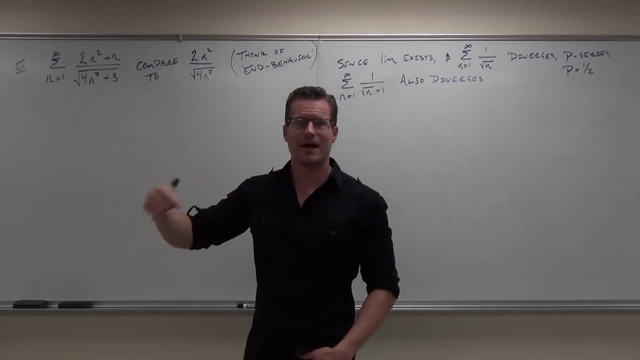 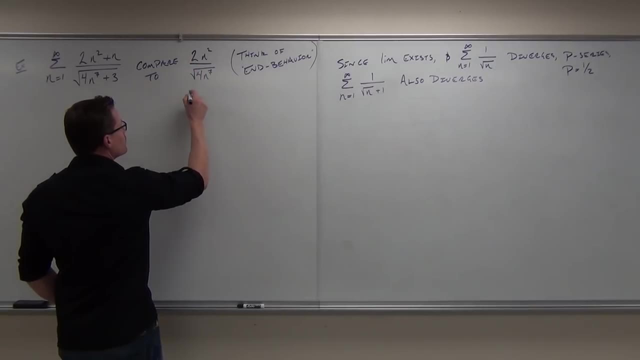 Hey, that's why this thing's going to be nice, Because if we simplify this, we will find out what the convergence or divergence is of it. So let's do it. How do I simplify it? Square root of n, squared n to the 7th. 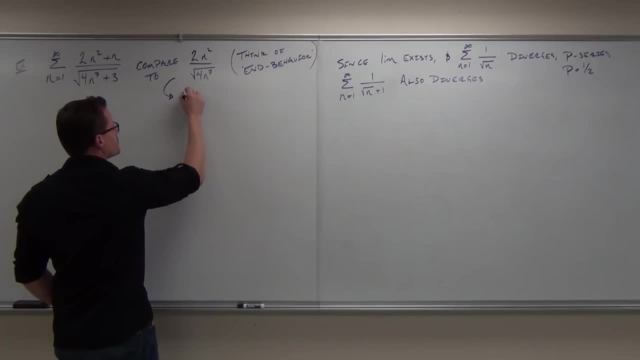 Say what? Pull the 4 out and then Pull the 4.. Okay, So 2n squared over, 2n to the 7 halves, We can do that. Yeah, Can I keep going? Yes, How much is it? 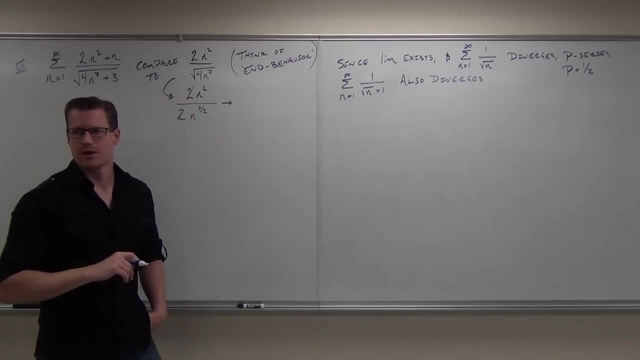 2 is gone. 2 is gone. Yeah, Okay, That's good news. What about n squared over n to the 7 halves? Can you do that? 1 over n to the 7?? Oh wait, Un-pull it. 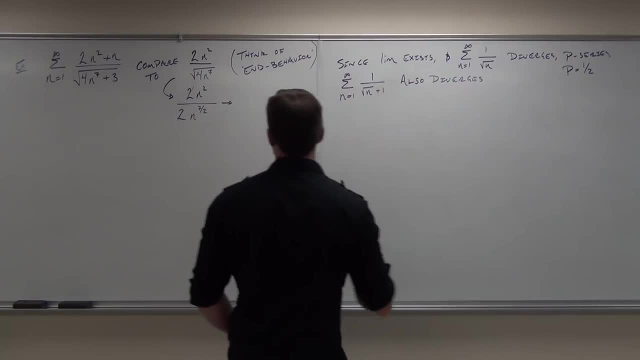 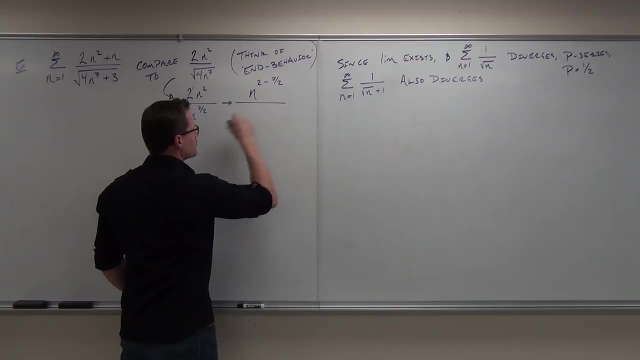 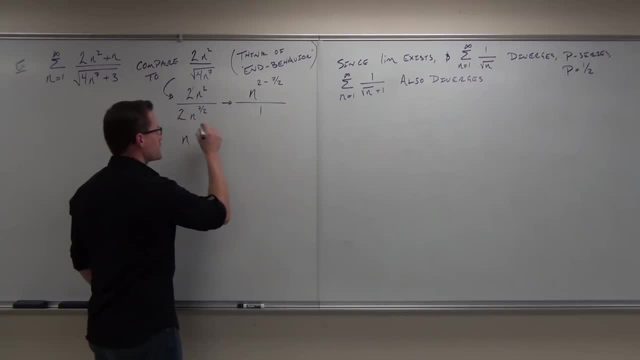 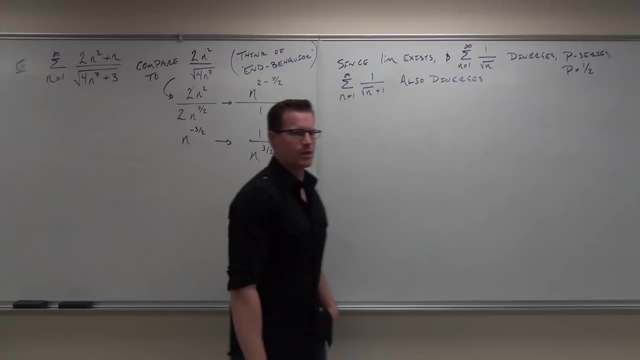 This would be 4 halves minus 7 halves, That's n to the negative 3 halves, or we get 1 over n to the 3 halves. We get 1 over n to the 3 halves. You guys okay with this so far. 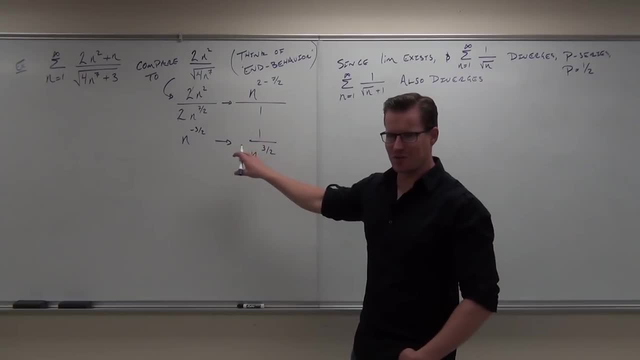 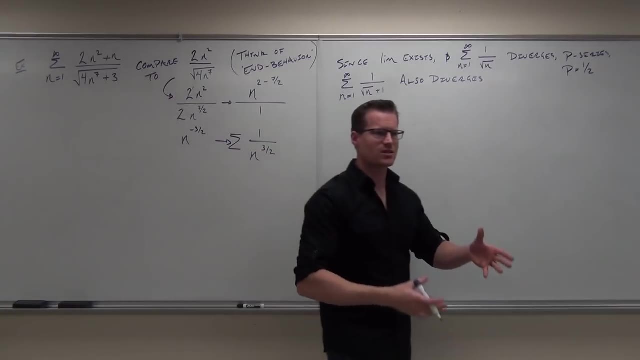 Yes, Are you sure You should be, because that's freaking. just some algebra, and you should be okay with it. Now tell me something about this series. Tell me something about that series. It's a p series. Ah, it's a p series. 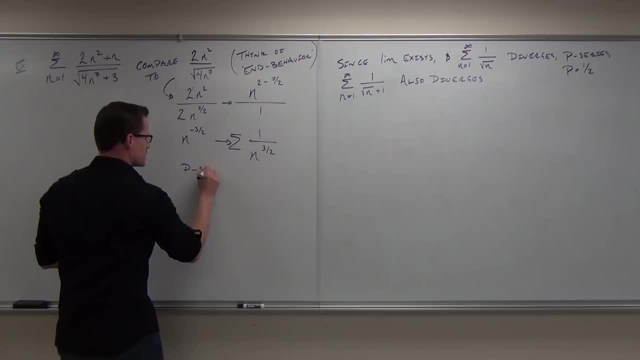 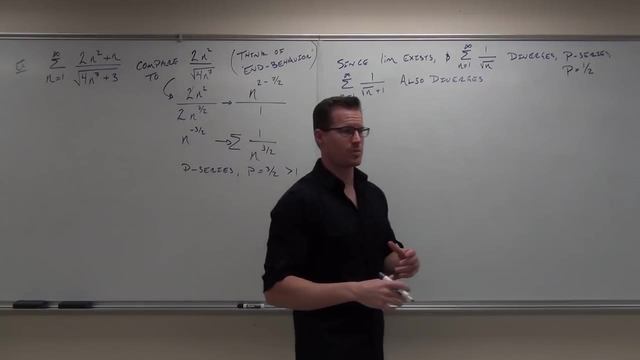 What's the p? Three halves. So this is p series with a p equals to three halves greater than. tell me something about a p series with a p equals three halves greater than one. What do you know? Convergence, That's convergent p series. 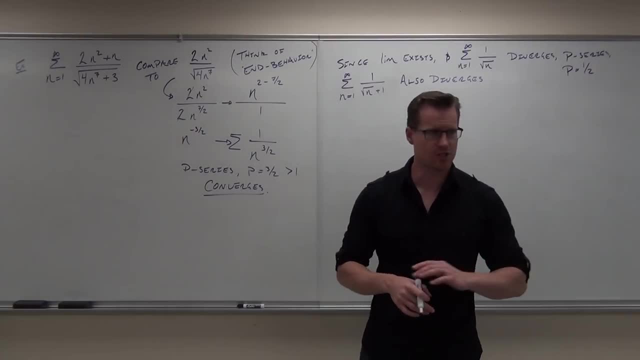 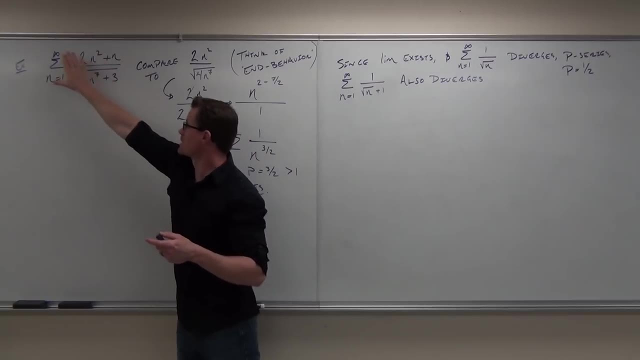 Now let's think about what the limit comparison test is gonna do for us here. So we probably already would have done the divergence test. Hopefully you would have done that. Now the limit of the sequence here: without the series, the limit would be zero. we're good to go. 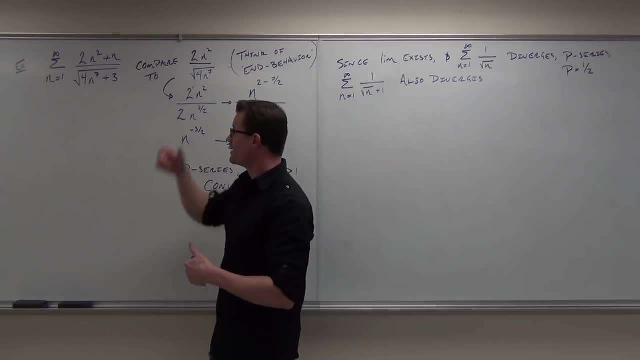 It says we might not be divergent. Then we go ahead and we think: well, is it a straight up p series? Is it geometric? Is it any of these things that we can do? Is it integral test? Is it a comparison test? 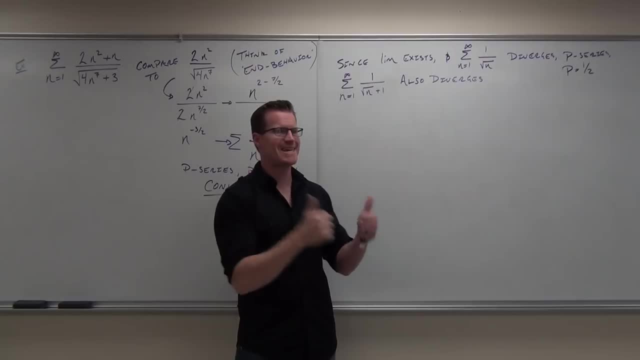 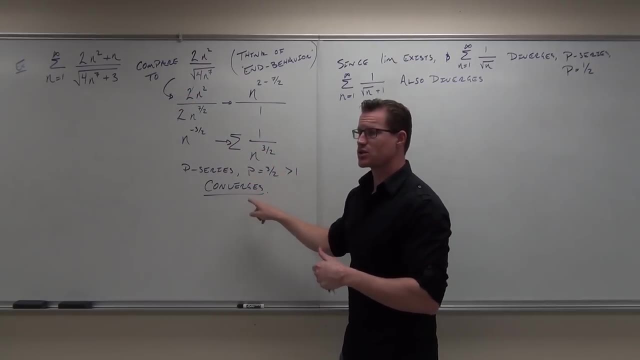 I don't know. it looks pretty hard for a comparison test. Can I do a limit comparison test? Yeah, Yeah, think of the end behaviors. End behavior would look like this guy. This guy is a convergent p series. So what we're gonna do now? 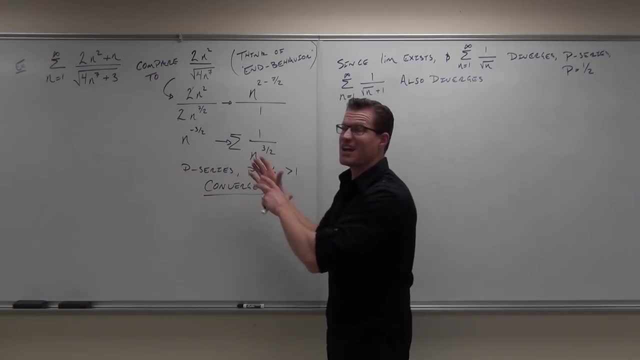 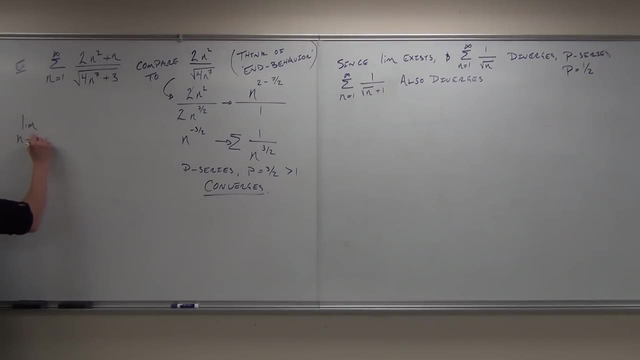 now that we've determined this is a convergent p series, or even if it was a divergent p series, we compare this as a limit. as n approaches infinity, What's gonna go on the numerator of this ratio? The original one? The original one? very good, we'll put it. 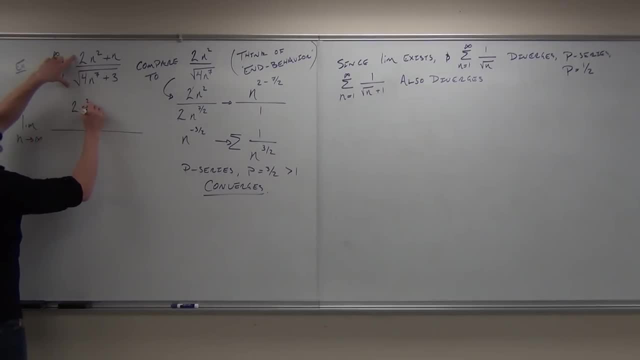 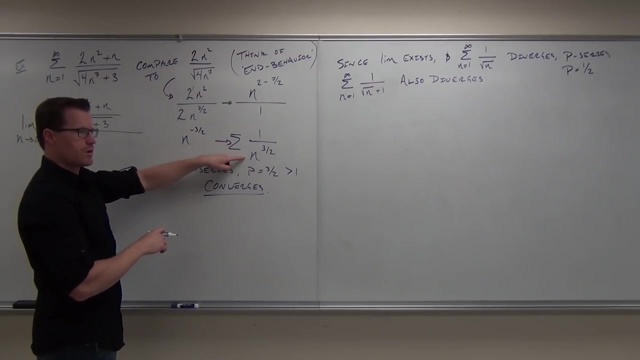 So the original series, that's our, a sub. n Over what? Over what? The nth, Say what now? 1 over the nth, nth, The nth one. so this one, You could even use this one, whatever you want. 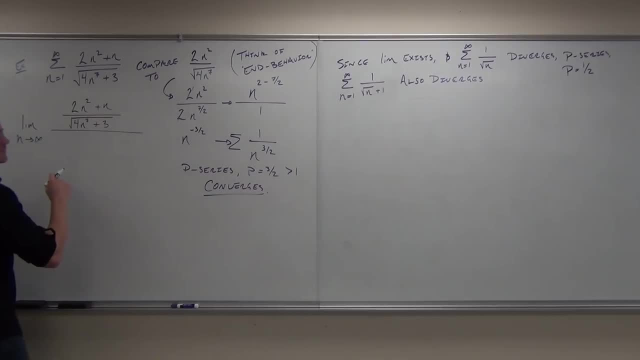 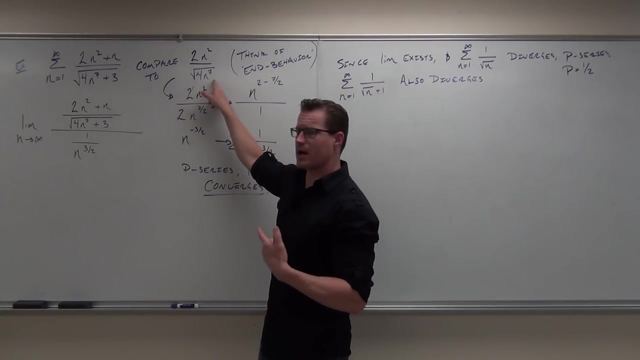 Now it's fine. I don't think it really matters which one you use. We do them. basically I'd use that one because it's nicer Basically and you can do these a couple of ways. okay, Basically what I like to do, I like to find out what I'm going to compare my original. 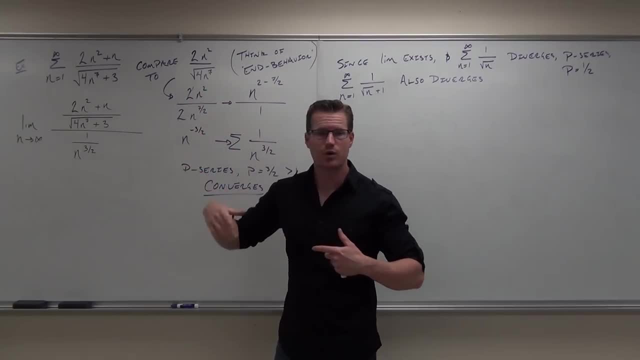 series to. I like to simplify that as much as I can, because they all should be simplified, because, basically, you're getting rid of everything but the leading terms. Did that sink in? That means they're all going to simplify. Hello, You're getting rid of everything but leading terms. 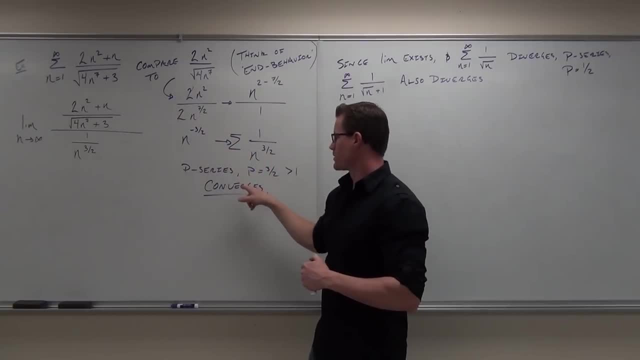 Should be just one term over one term. you can simplify that. I like to find out whether it's going to converge or diverge first. I like to have that in the back of my mind. then I like to compare it with the simplest. 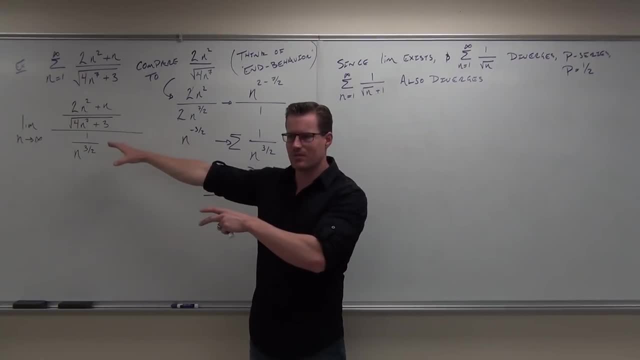 form. That should make sense, right? That way, I don't have to re-simplify in my problem. Well, this is a whole lot easier to deal with than that one is, isn't it? So why would I put that back in? 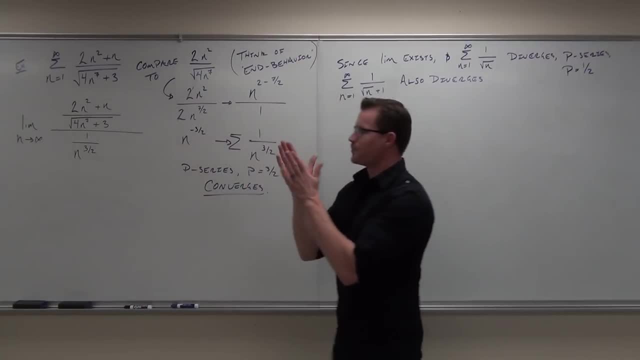 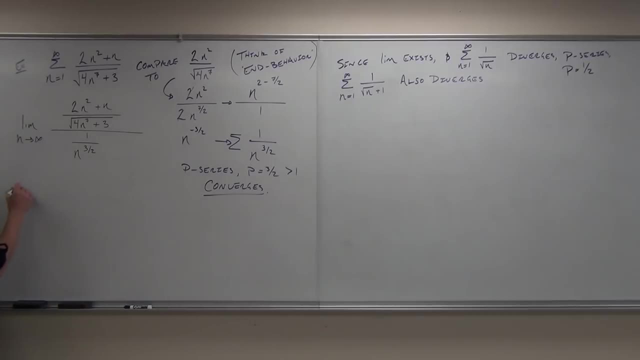 I'm going to use my simplifying. Tell me the next step. What would you do? Multiply by reciprocal. Multiply by reciprocal. We could do that. Are you starting to notice all the algebra you're going to do So we'll have. 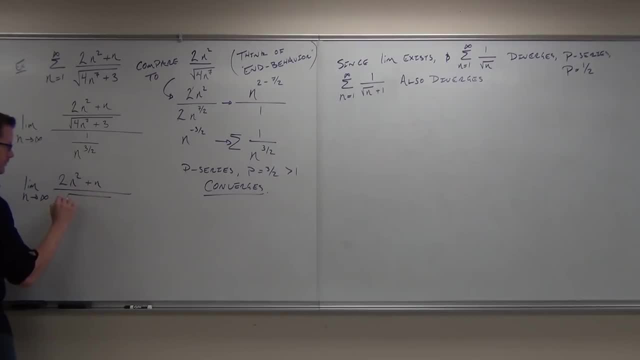 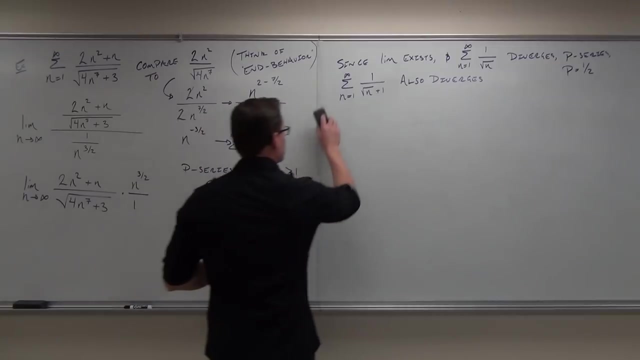 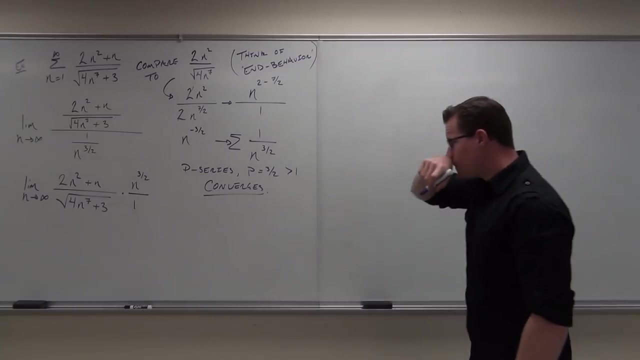 2n squared plus n over the square root of 4n to the 7th, plus 3 times n to the 3 halves over 1.. Now I'm going to move over here. What now? Distribute the n over the 3 halves? 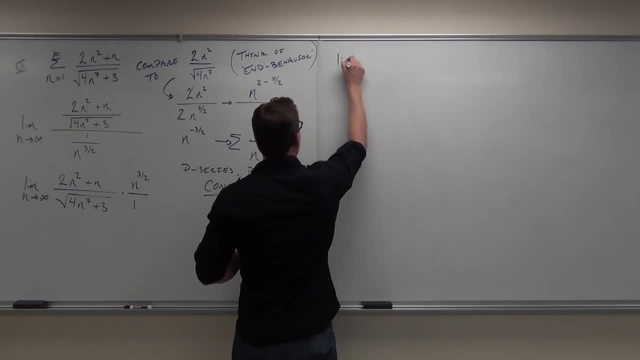 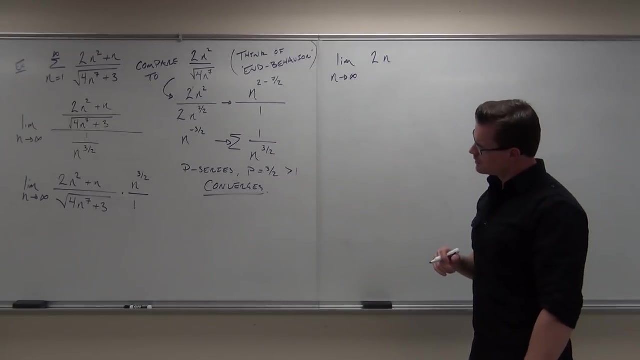 Yeah, OK, We can do that: 2n to the 3rd plus n, plus n to the 5th, to the 7th, 2n to the what now? 2.. Oh wait, No, never mind. 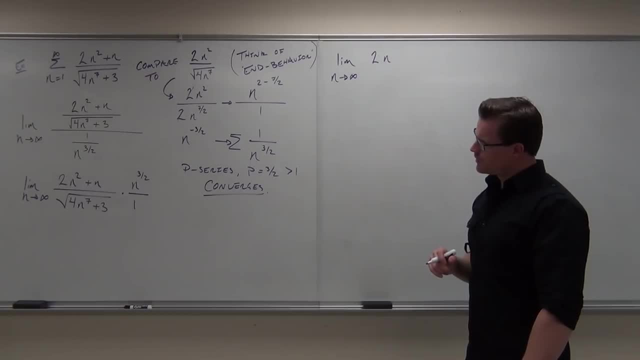 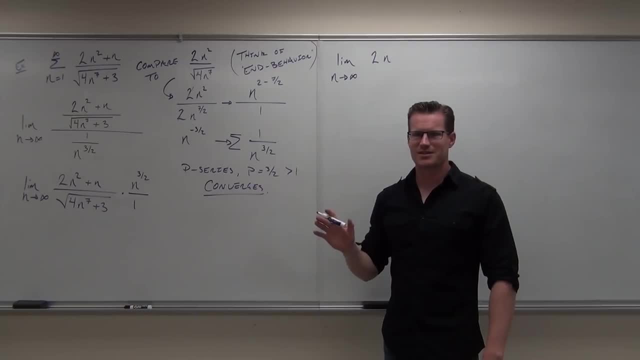 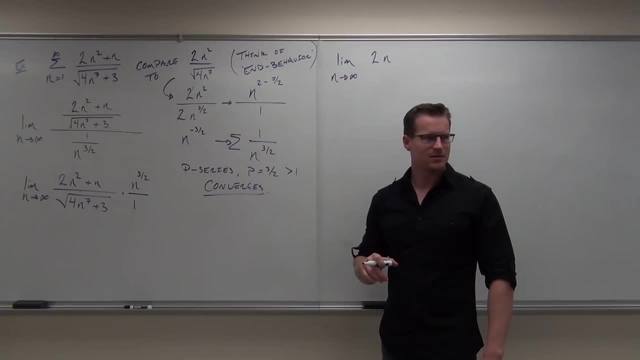 It was so hot over here, I'm going to punch more papers. Can we just pull more n's out, Because I think that's what we've been doing anyway. So it's going to be a 5. If we add 7 halves. 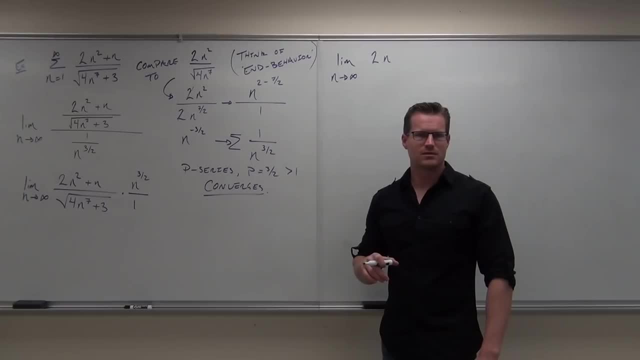 7 halves. Yeah, 7 halves. It's the 7 halves, 2n raised to the 7th. You guys figured it out What Well it would be: 2 over 2 plus 3 over 2.. 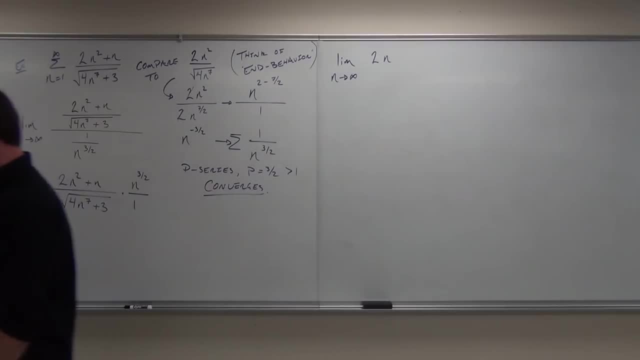 I figured it out. You better be able to figure it out. So 3,, 4,, 5 over 2.. OK, Last time I checked I didn't know how to do it, I figured it out. Yeah, Last time I checked it was 7 halves. 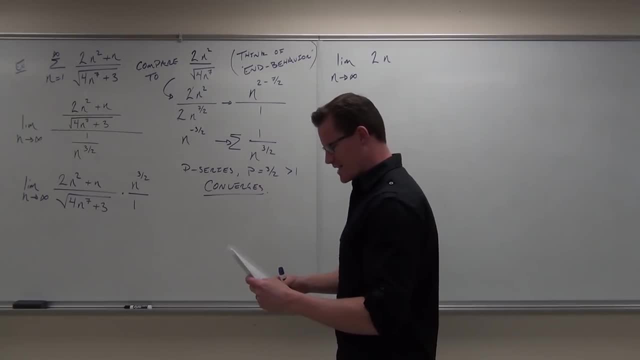 Damn. Do you know what you do when you multiply common bases? You add exponents. You add exponents Plus how much? 5 over 5 over 2.. Over your nasty square root, Don't do a L'Hopital's rule. 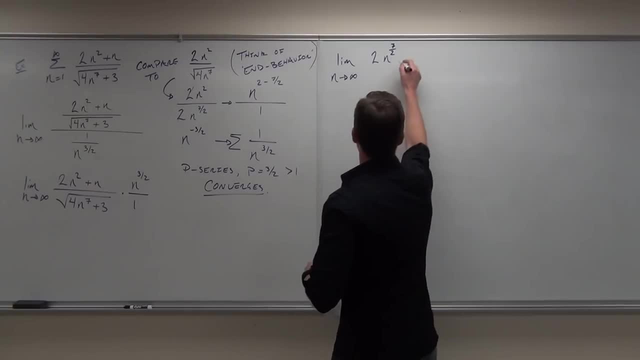 You have to do a L'Hopital's rule. You don't do a L'Hopital's rule. I'm going to do it. I'm going to do it, OK, So the sum of the common bases has to be 3 over 2.. 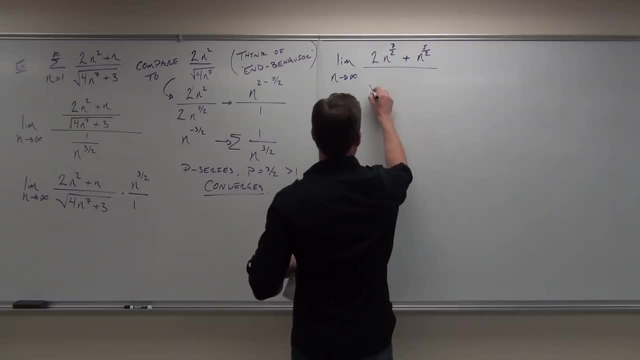 So what do you do? Well, I'm going to do it. So the sum of the common bases has to be 3 over 2.. See, that's what you do. You take the total And then you multiply it. I'm going to do it. 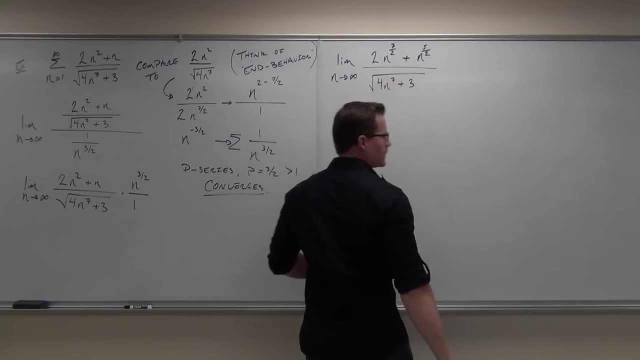 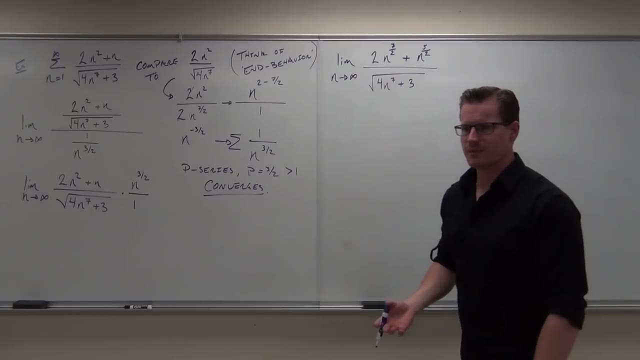 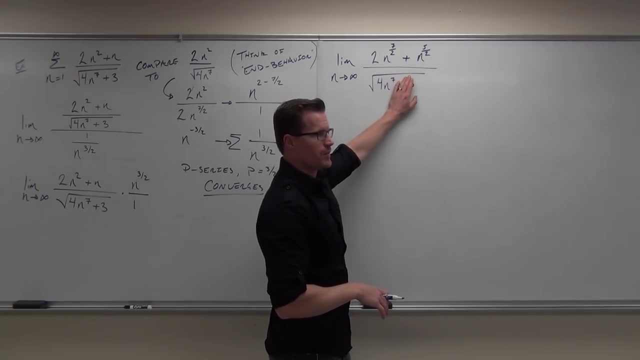 Don't do a L'Hopital's rule, don't do that, Just divide by the largest power in the denominator. So if you divide by the largest power in the denominator, here's how you figure that out. You cover up all but the leading term, that would be the largest power. 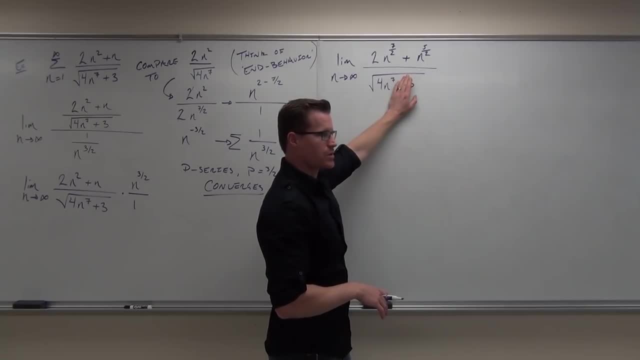 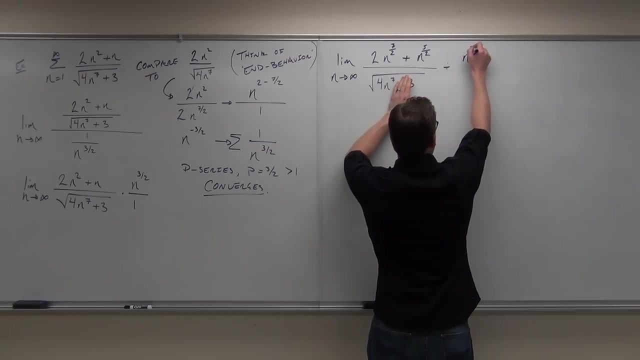 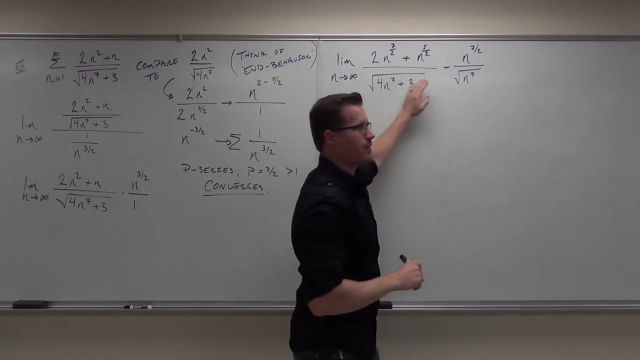 So cover up all but that thing and write that as a power. So we're going to divide by N to the 7 halves. So we're going to divide by N to the 7 halves over N to the 7 halves. I want you to understand that these are equivalent. 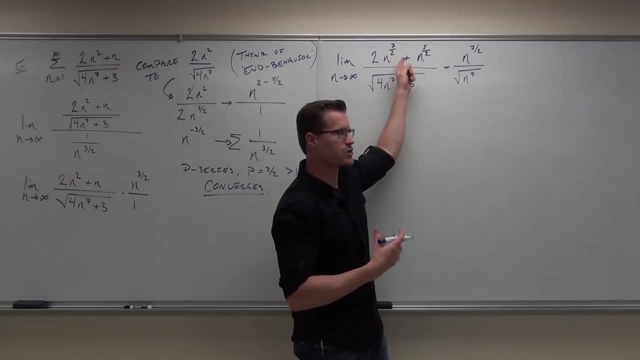 Do you understand that they're equivalent: One we've written as rational exponents, one we have as radicals. Now please listen carefully. Okay, You don't always get to do this just like it is. You have to verify that the radicand, the inside part, is actually positive. 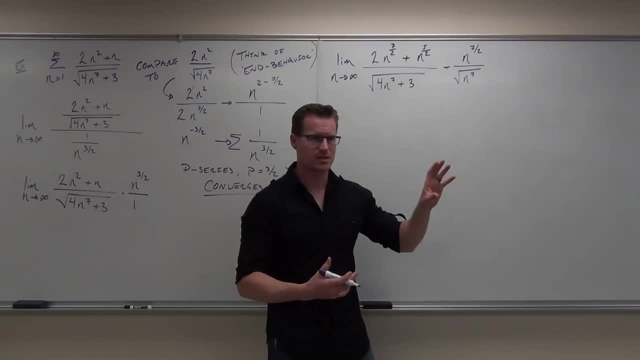 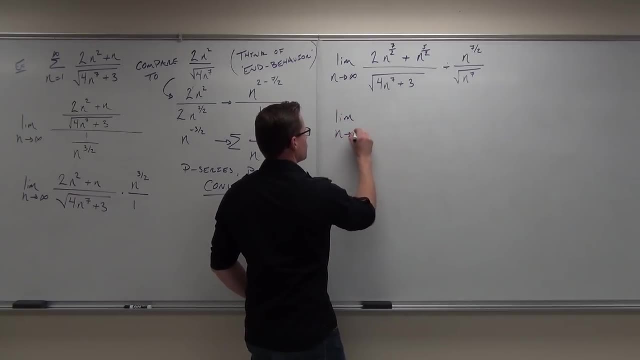 Because this is positive, we can make that straight up move. Does that make sense to you, So that we're good to go? So if we divide this, we're going to have a limit, as N approaches infinity, of 2N to the 7 halves. 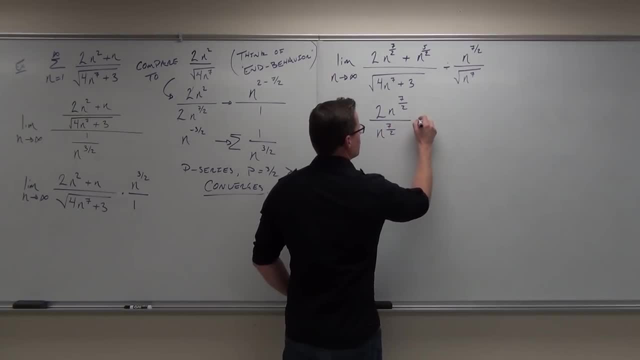 over N to the 7 halves. I'm going to show you every step here. Okay, So we're going to divide by N to the 7 halves plus N to the 5 halves, over N to the 7 halves, All over big square root, because that has a square root, that has a square root. 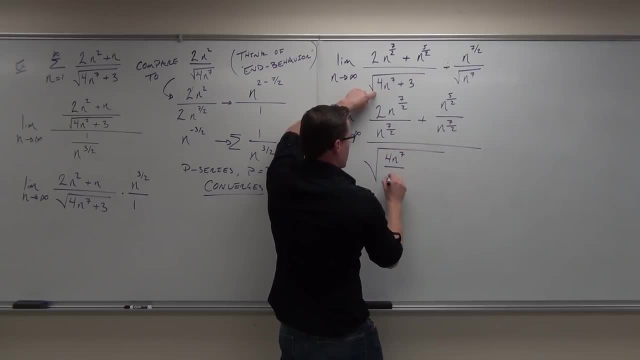 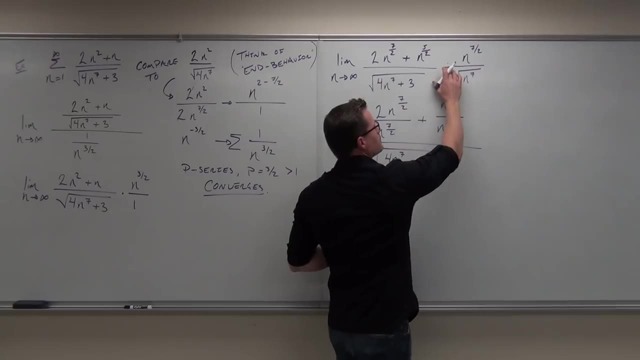 We'd have 4N to the 7th over N to the 7th, plus 3 over N to the 7th. I want to make sure that you guys understand that we are not multiplying here, We're dividing. we're dividing by each of these terms. 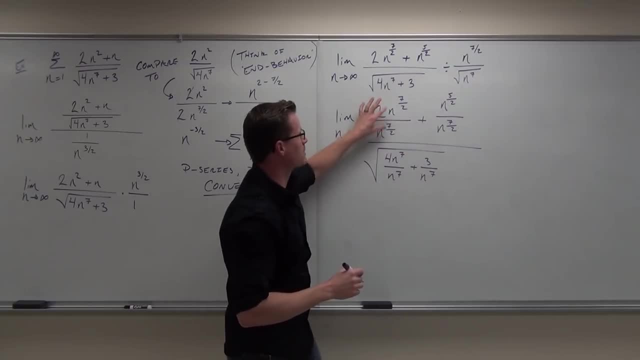 Okay, So it's getting divided. it's getting divided. That's why we have this over N to the 7 halves and over N to the 7 halves, Because we have two square roots here. we can make that one large square root over N to the 7th. 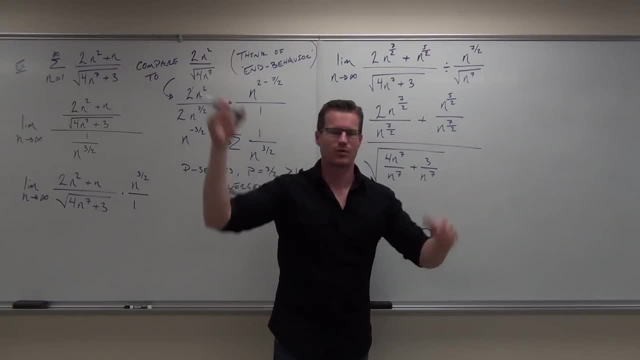 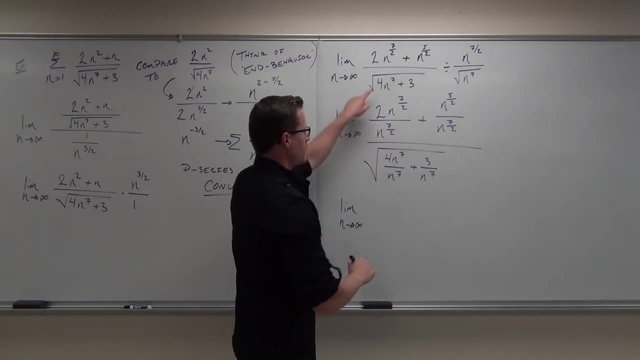 and over N to the 7th. So if you don't mind, I'll give you the algebra there. Let's simplify it. So we have a limit. N approaches infinity. How much does this give you? 2. Plus 1, over what? 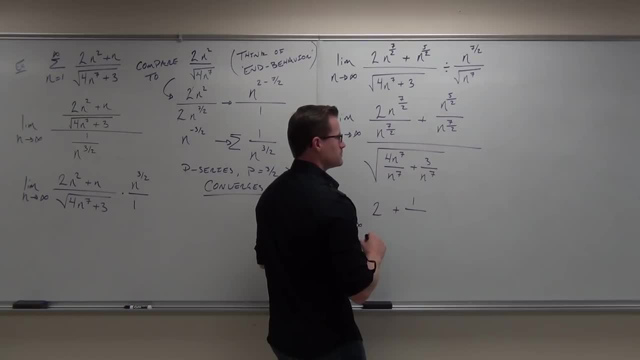 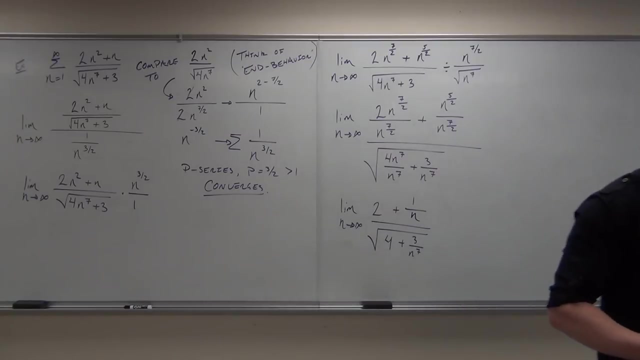 2. 4 minus 1. 2. N Over. This would be square root, Square root of 4 plus 3 over N to the 7th. Can we take the limit now, now that we got rid of all that stuff? 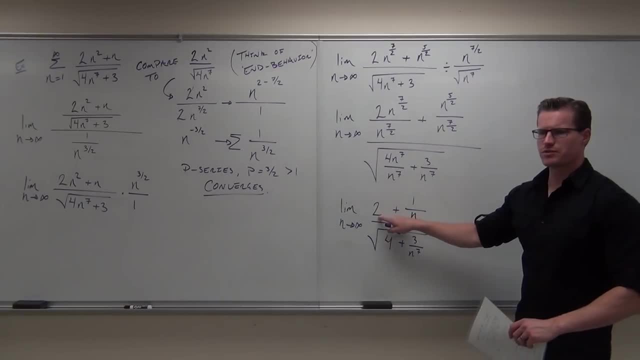 What would you get? What's the limit of 2 as N approaches infinity? What's the limit of this? as N approaches infinity, It goes to 0.. How about the limit of this one? 0.. How about the limit of this one? 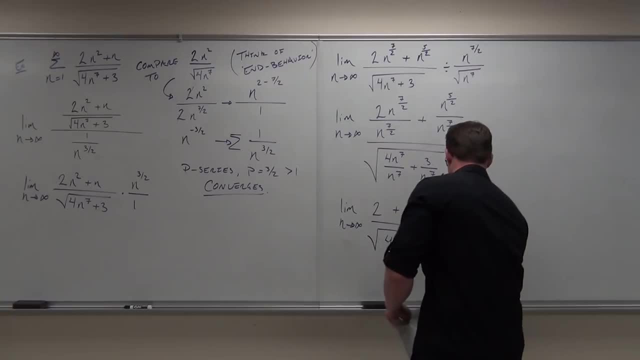 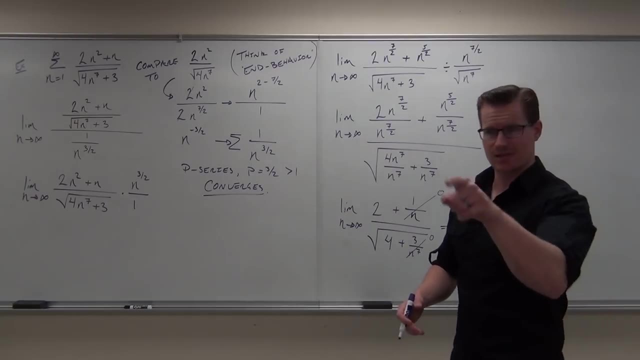 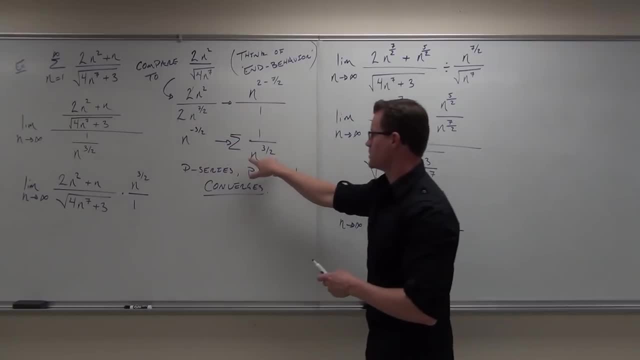 1. 1. 1.. What does that tell you? The limit exists. The limit exists. That's what it tells you. It says the limit exists, Which means that, going back here, it says that what we have and what we compared it. 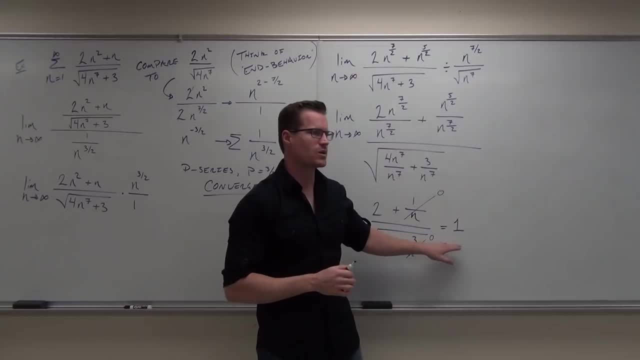 to will have the same result. If this one is convergent, the one we're given is convergent. If this one is divergent, the one we're given is divergent. Does this always tell you convergent or divergent? No, 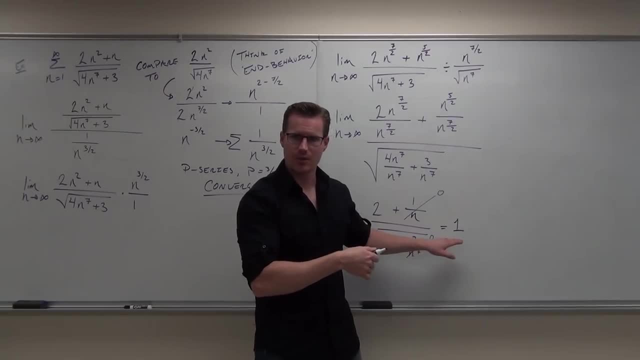 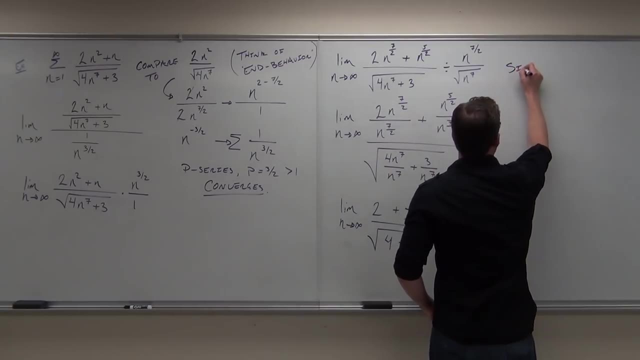 No. The first example: we had it existed, yet it gave us divergent. Now we have a limit that existed, yet it's going to give us divergent, No, No. So the way we write this is: since the limit exists and the series of 1 over n to the 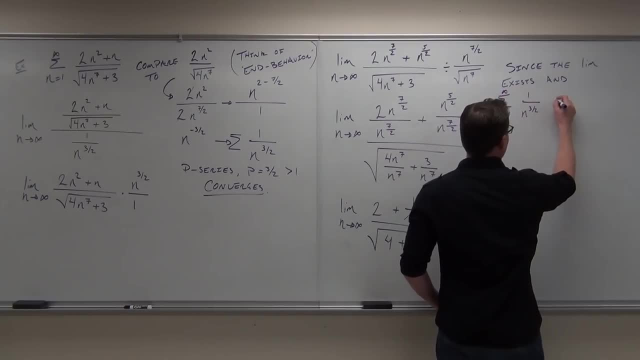 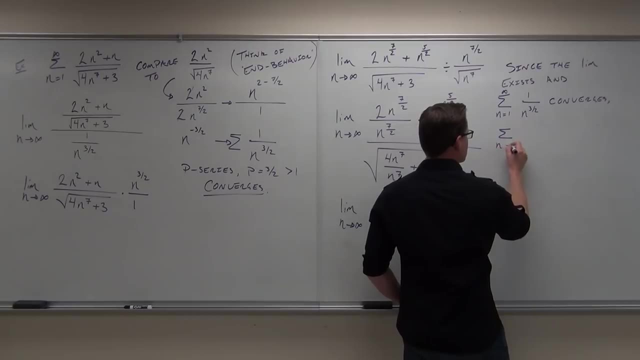 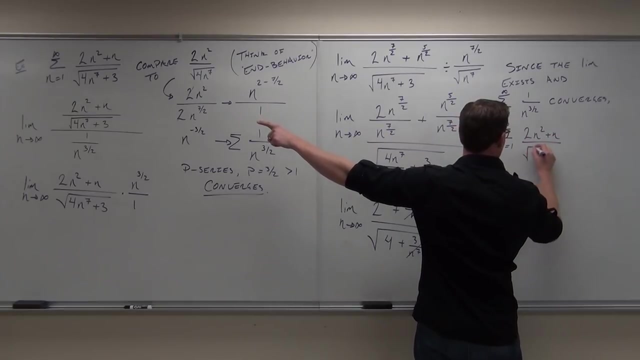 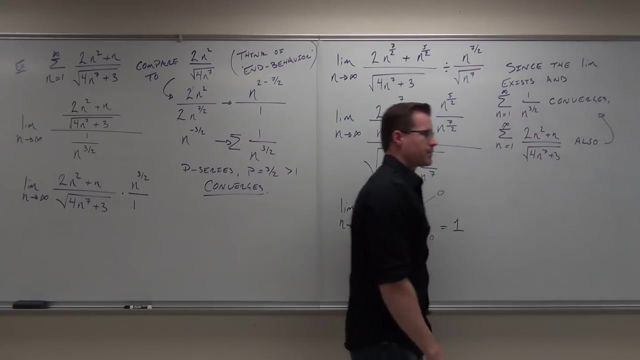 3 halves. as n equals 1 to infinity converges, then we have the series from 1 to infinity of our nasty junk also converges. That's the idea. Do you understand the idea? Show of hands. if you do, Do you feel okay with this stuff? 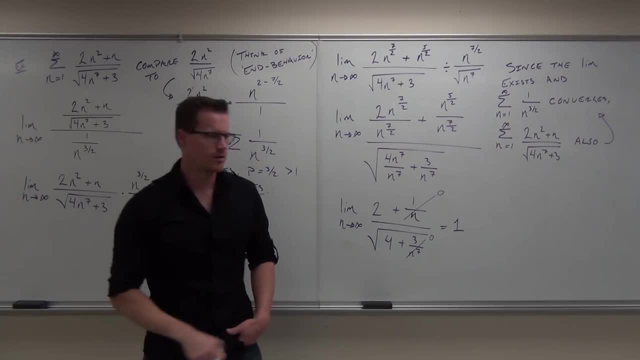 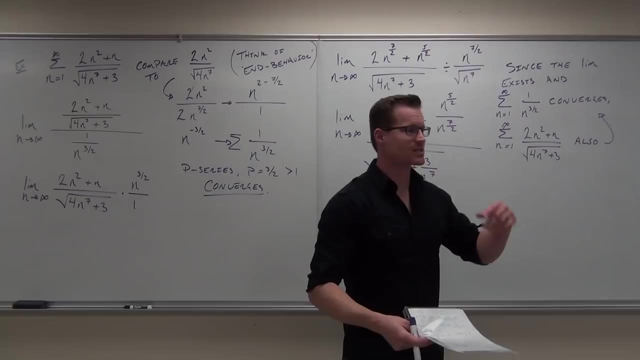 Easy, Medium, Hard, Different, A little different, It'll get easier. The problem with all this stuff is that there's so much stuff. That's the problem with this. It's because some of this will get confused in your heads and some of you will think: 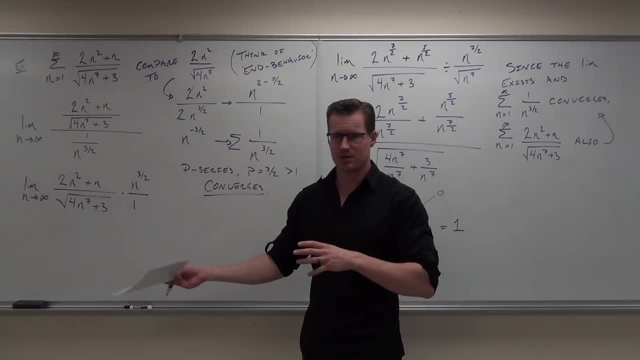 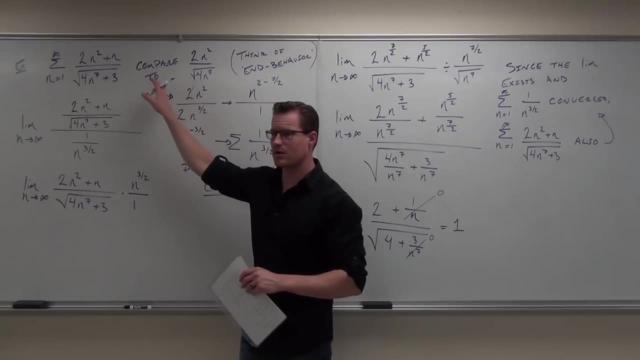 back to the comparison test for sequences. forget about the limit comparison test here. Some of you will get confused with the divergence test. taking a limit of a sequence here, saying equal to 0, and automatically think it converges. Some of you will think, well, since this doesn't work, I'm going to do this. 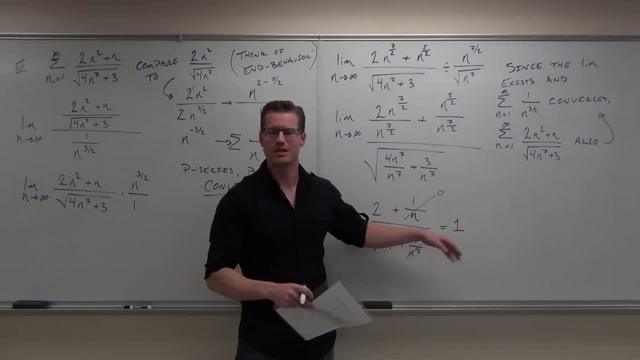 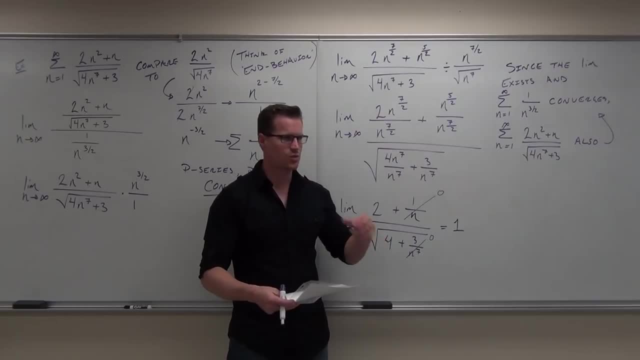 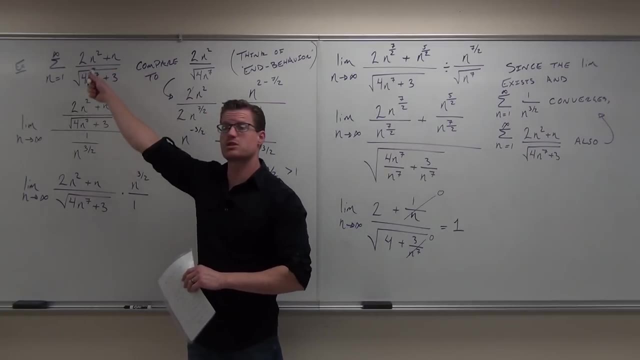 There's a lot of stuff that we're doing, So I'm going to try my best to reinforce the ideas here. The ideas are: you start with the divergence test and you take a limit of this sequence from which your series is built. If it does not equal 0, you stop right there. 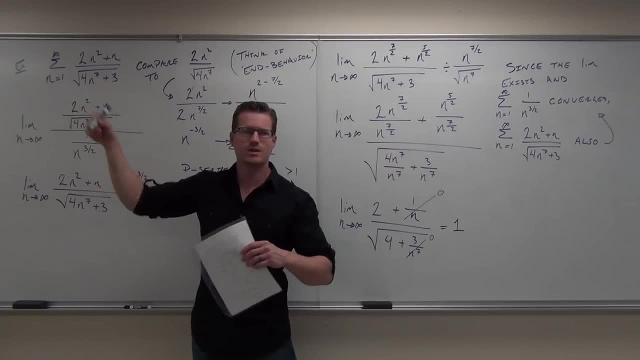 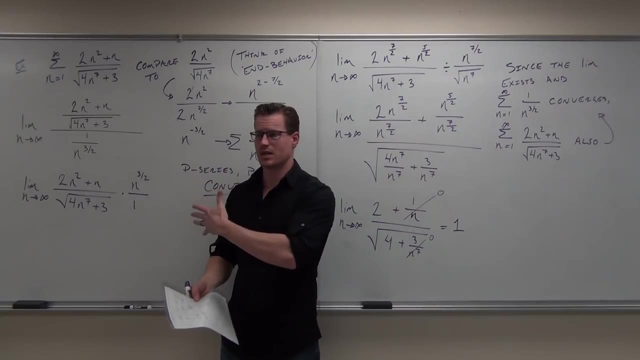 Your series is divergent. Does that make sense? After that, you keep going with one of the methods that I've used so far: geometric series integral test, comparison test, limit comparison test. there's several now. We do a limit comparison test, but you understand. 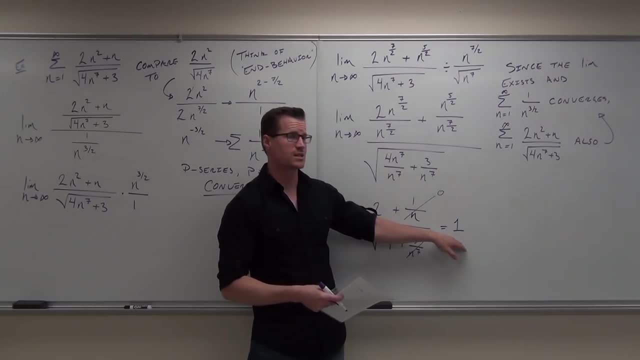 with a limit comparison test that if you equal any number besides infinity or does not exist, that means the results are tied together. Both converge or both diverge, not necessarily one or the other. Okey dokey, Would you like to try one more? 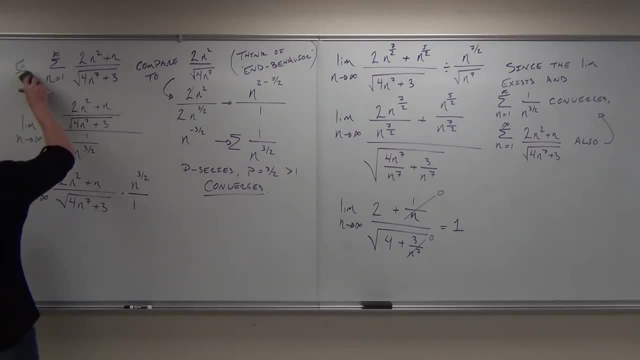 One more? okay, one more. Any questions before I raise it. Are they kind of fun though? They're kind of fun, right, I enjoy them. It's totally different than doing all those integral stuff, isn't it Kind of like a puzzle? 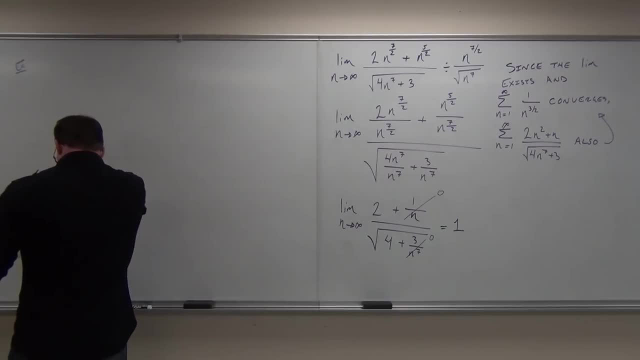 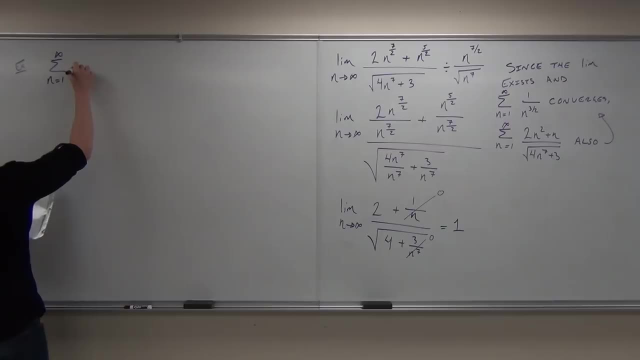 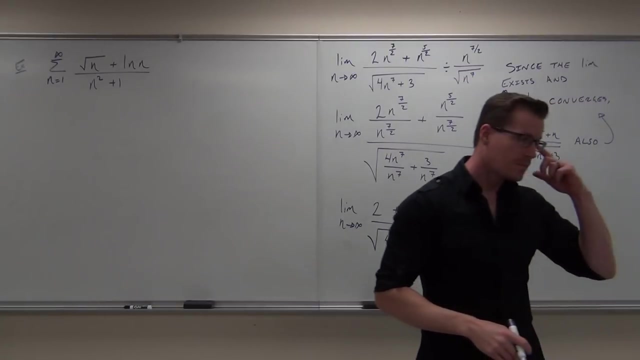 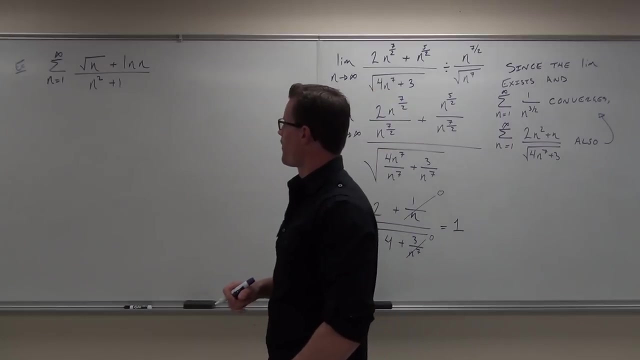 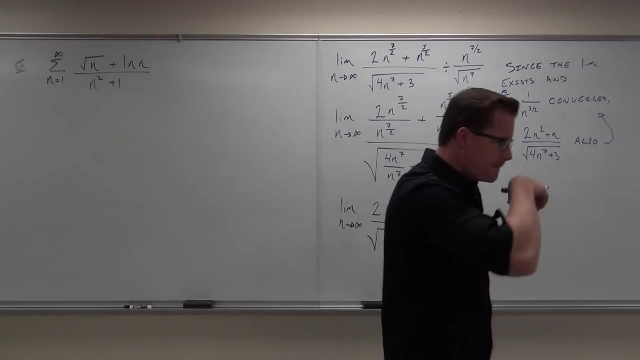 You just got to get creative with picking a new piece of them. That's why it's kind of like a puzzle. It can be puzzling, Especially with this one. Let's start from the beginning. First thing: What would you do first? 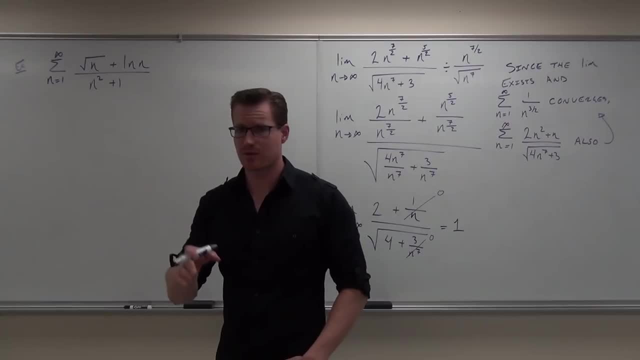 Divergence test: You would do it. Let's pretend that we did it. But you want to start there. Let's pretend we did it. Divergence test: It equals zero. What should you do? Go in or stop? 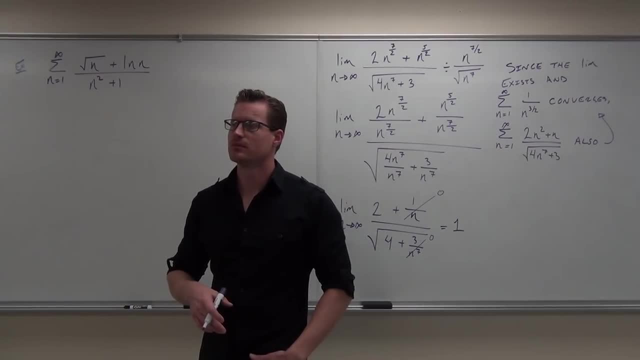 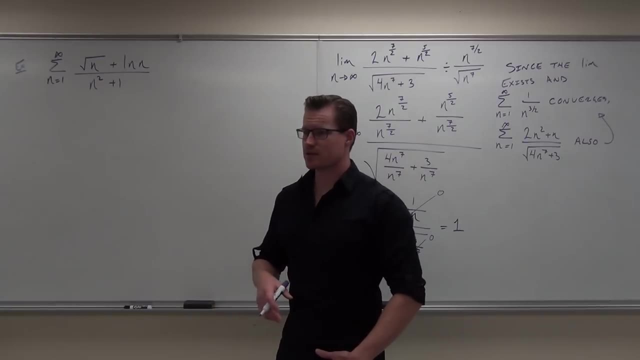 Divergence. go in, It equals zero. Let's pretend that we did it. Keep going, Keep going- Equal zero. What would you do? Stop, No, Keep going. Okay. What would you check here? Would you want to do integral test? 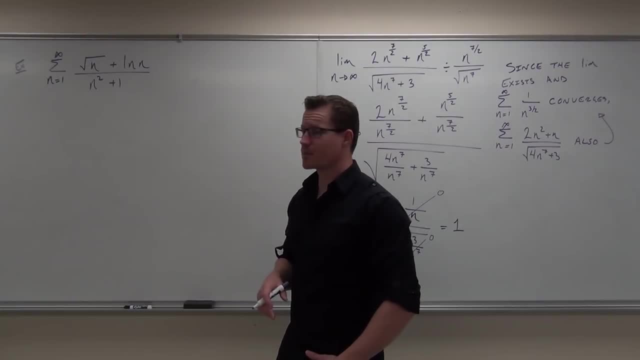 No. Can you do the integral of that thing? No, Probably not a good idea. Does it look like a piece of paper? No. Look like a geometric series: No, No. Look like something we could compare it to: Yes. 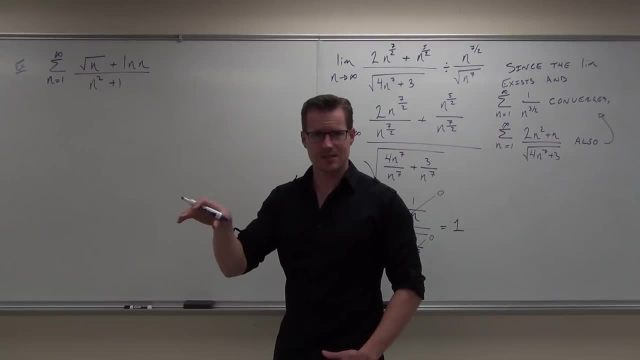 Yes, Yeah, but not a real easy one, huh, Because I don't know that that's always less than something or always greater than something. So if it's not something easy like that, like we had a couple of them that were nice, we. 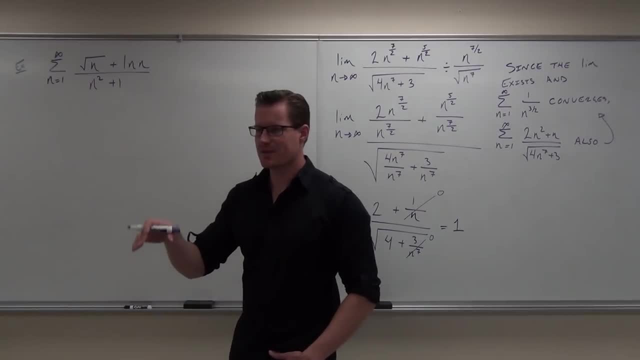 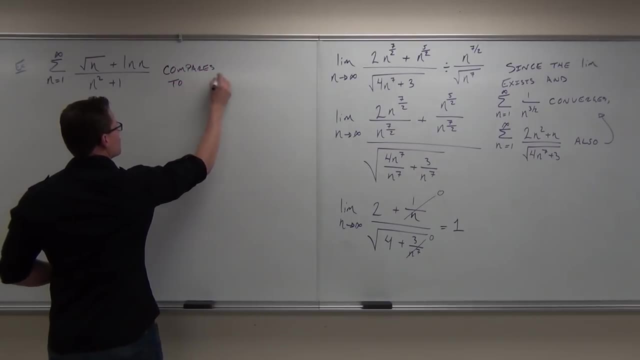 go, well, maybe we want to try the limit comparison test. So let's try to see if this compares to something. So this compares to what? Oh boy, Let me just get rid of the now and then. Well, here's the thing. 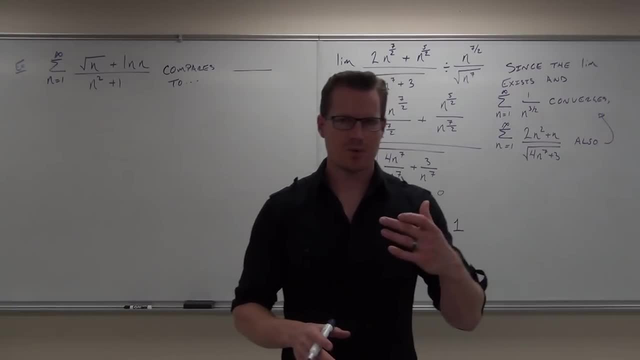 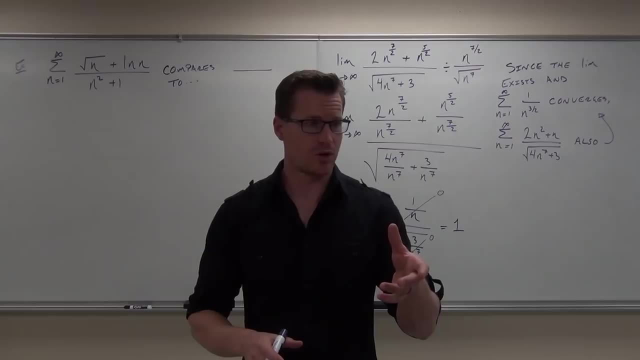 You're going to get rid of part of it, right, But you need to keep the fastest growing part. First of all- you know I've been skipping a couple of things- You do need to make sure that this has positive, This has positive terms. 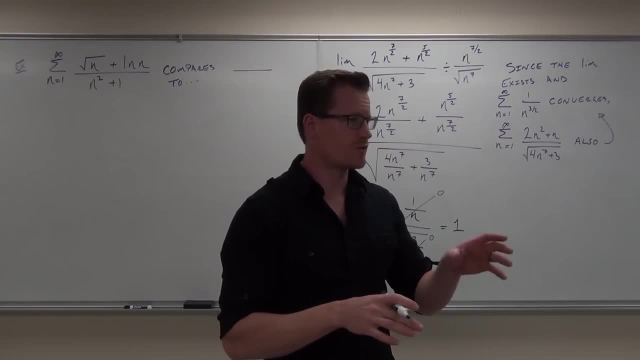 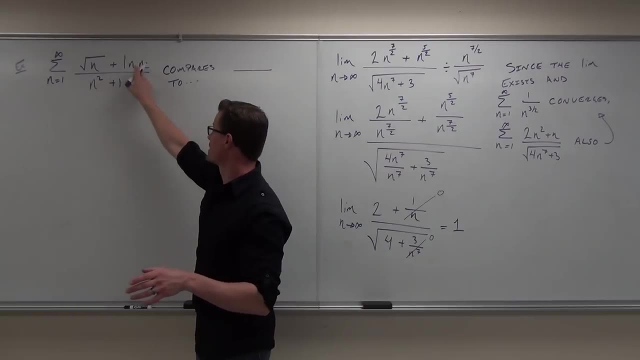 And I'm kind of taking that for granted. That's not a trivial point. You do have to make sure that it has positive terms. Does this have positive terms? Yes, Yes, As long as n is greater than 1, yes, it does. 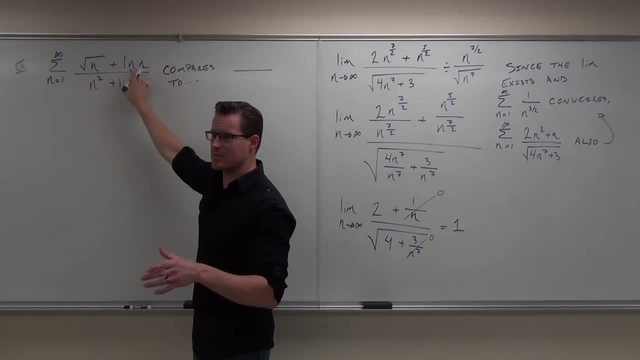 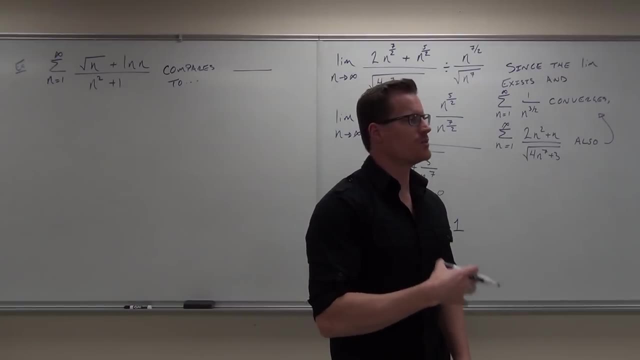 Because n between 0 and 1, there would be negative terms Maybe. Well, actually I would for here. So we do have positive terms and we need to check it. Now, if you're going to talk about n behaviors, that's what I told you, right? n behaviors. 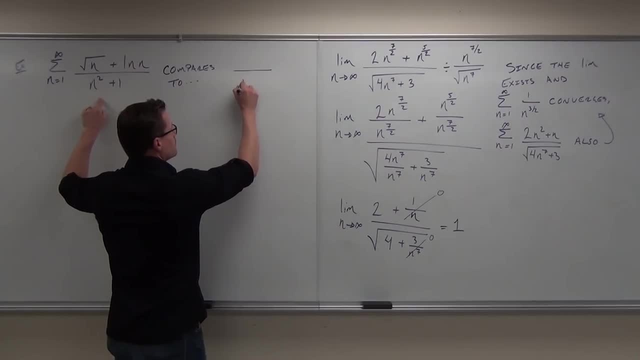 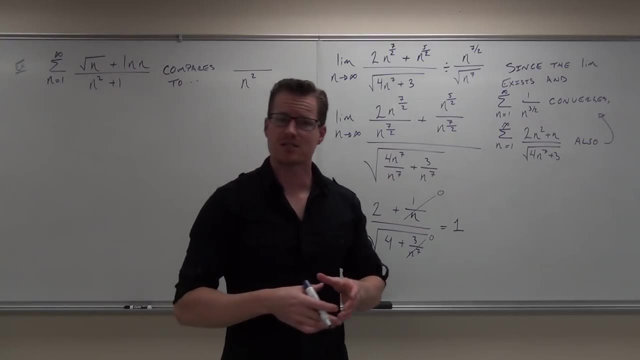 are this one? That's going to be pretty easy. What goes on our denominator 1.. Yeah, That's a piece of cake. N behaviors- are this one? It can get a little tricky. What you want to do? you want to keep the fastest growing part. 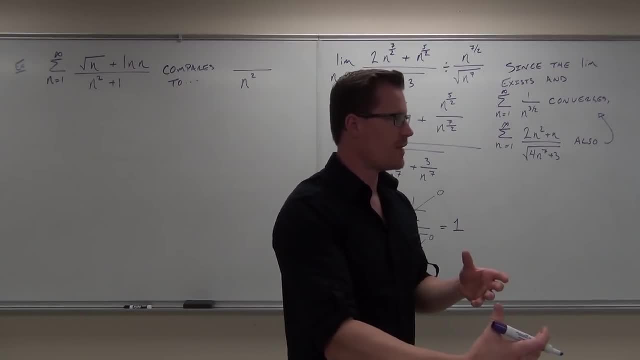 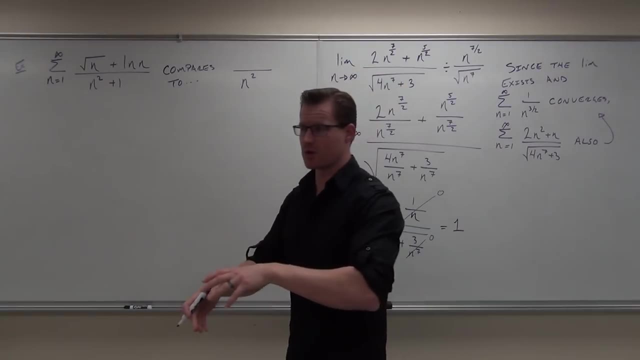 The fastest growing part will give you the n behavior. Does that make sense to you? That's why we keep the largest power, that leading term, because that's given us our n behaviors, the fastest growing or fastest falling apart. Well, in our case, what grows faster? square root of n or ln. 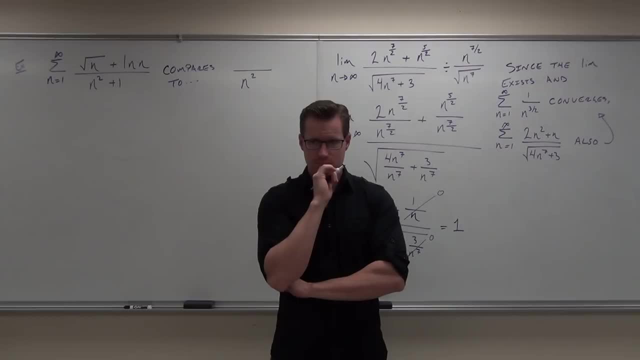 Ln Square root of n. Better, I don't know Ln. You're going to have to think about that a little bit later, But maybe you are guessing right now. Could you punch it into a calculator and look at the graph. 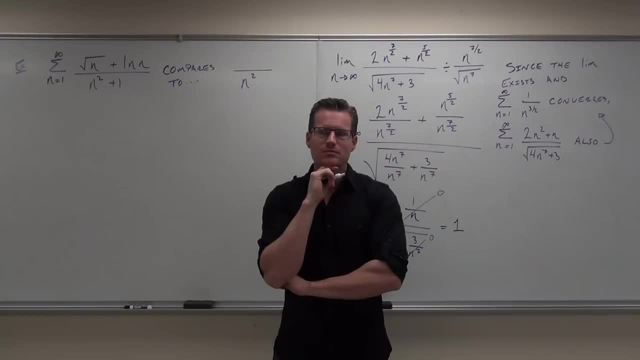 They are very similar. Square root of n is decreasing as it gets larger. The l of n gets bigger, Untrue- They both increase. They both increase. Put some high number in both. Put some huge number in both of them. That will prove everything. 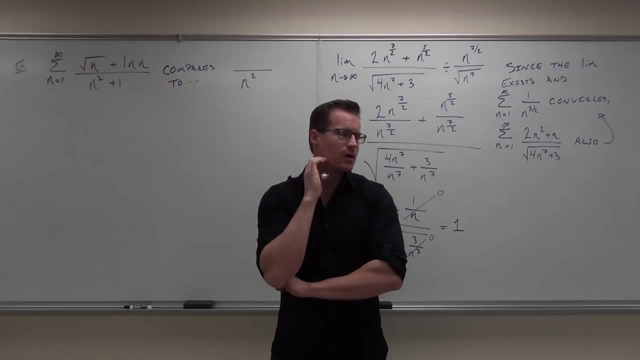 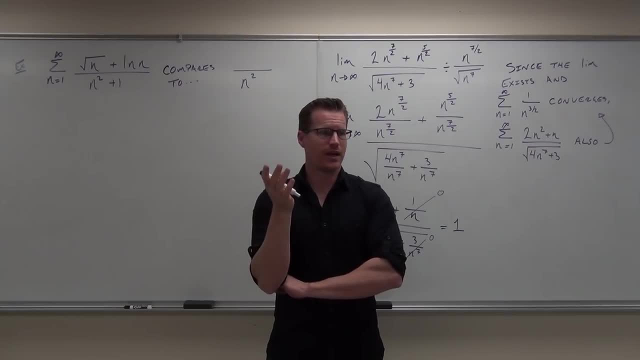 That's a great idea. Well, you can think of it as ln of n is an inverse of e to the x, correct? So if e to the x starts climbing real fast, ln's gonna climb, but slower and slower and slower. 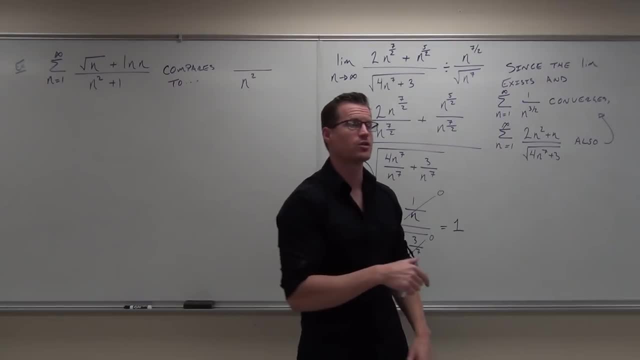 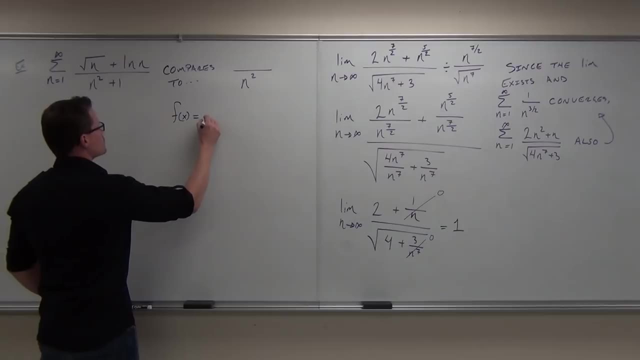 less of a pace than square root of n. Square root of n is the faster increasing one. Now how do you show that? Here's how you show it. Maybe you consider f of x equals square root of x and f of x. sorry, maybe g of x. 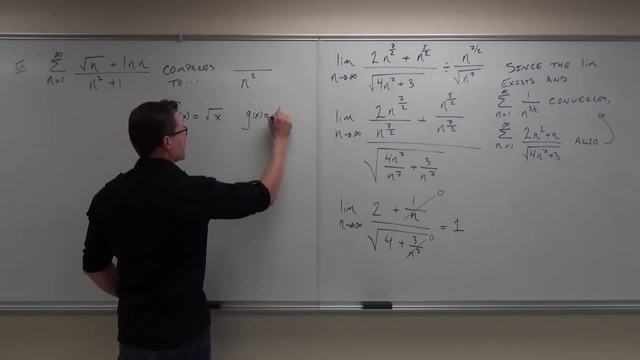 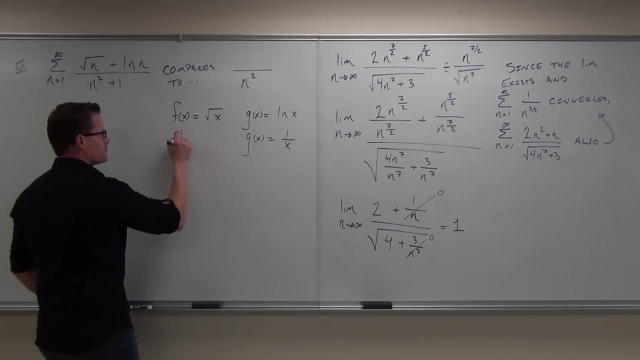 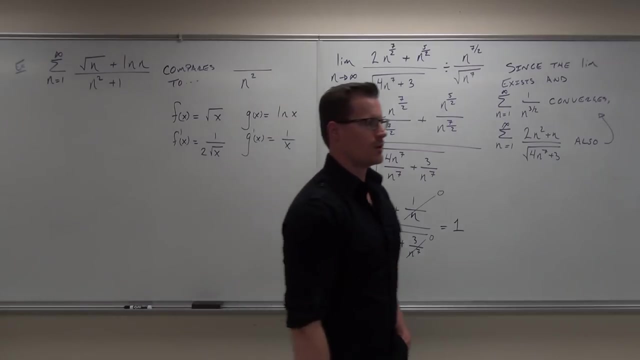 I don't want you to get confused on that. g of x equals ln x. The derivative is one over x. The derivative is one over two square root of x. You can verify that later if you want. Now here's the whole point. 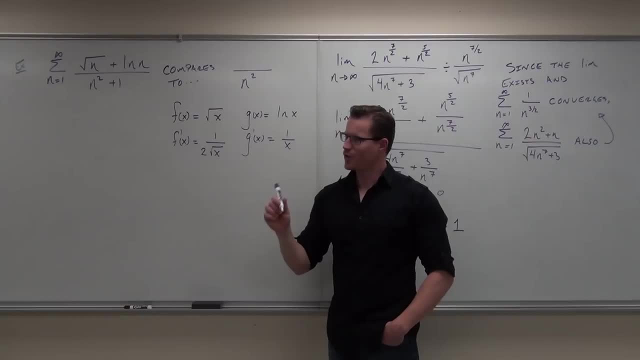 This is kind of interesting to think about. Hopefully, I hope you're with me on this one, You guys. okay, on the derivatives, right Derivatives? tell how you're increasing. in this case, they're both increasing. They're both increasing graphs. 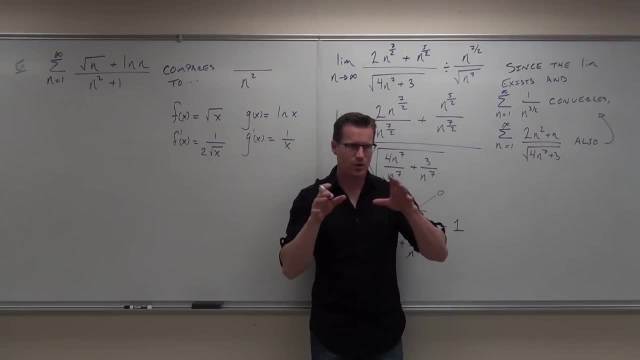 Tell us how you're increasing. So whichever one goes to zero, whichever derivative goes to zero faster, that's the one that stops increasing sooner. I'll say that one more time, so it makes sense. okay, This is how your functions are increasing. 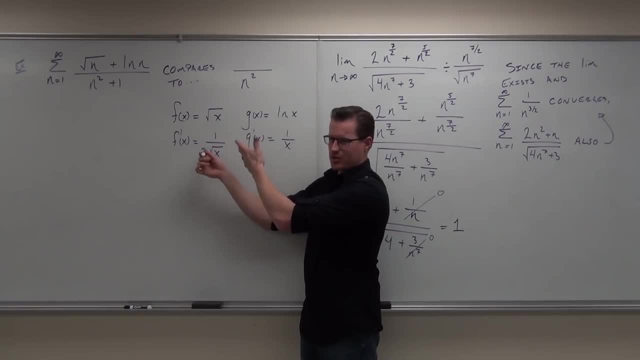 Are you with me? They're both positive, with x greater than one. So this is how they're increasing. Whichever- since this shows how your graphs are increasing or your functions are increasing, whichever one goes to zero faster is the one that stops increasing sooner. 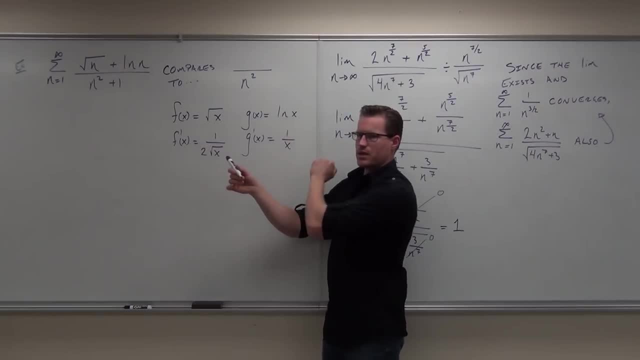 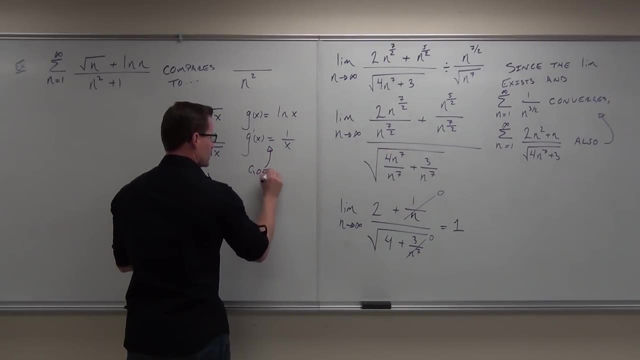 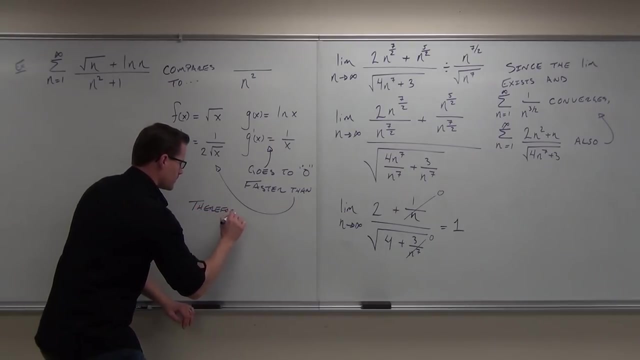 Did that sink in Which one goes to zero faster, This one does That goes to zero faster. So this goes to zero faster than this. Therefore, Okay, And what does it say? F of x increases faster than g of x. at the end. 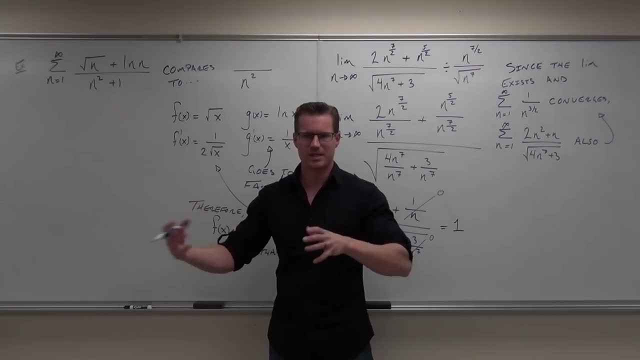 You can think of it as increasing longer, increasing faster. This is the basic idea. Does that make a little bit of sense to you? It's kind of weird, right? You're using a derivative to say, well, which one goes to zero faster? 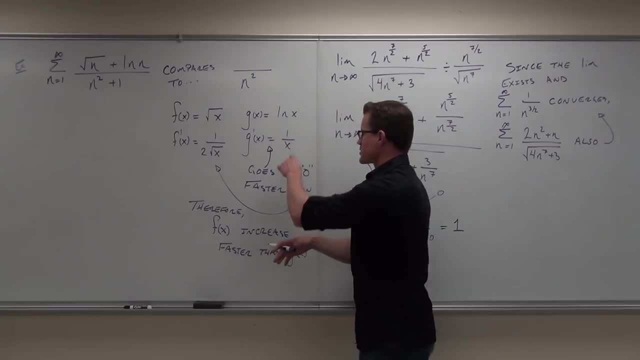 which one slows its increasing behavior faster, Since this goes to zero faster. this slows its increasing behavior faster than this one does. That's the idea. This will always be increasing at a faster rate than this one. Does that make sense to you? 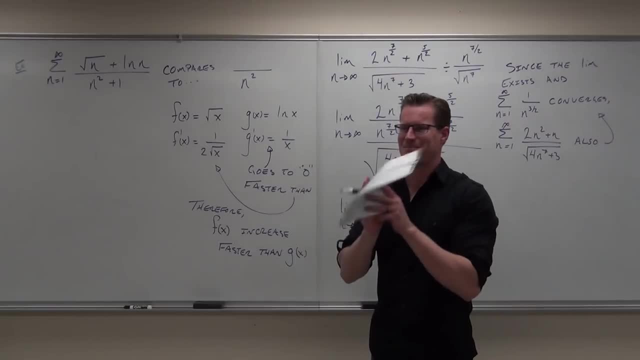 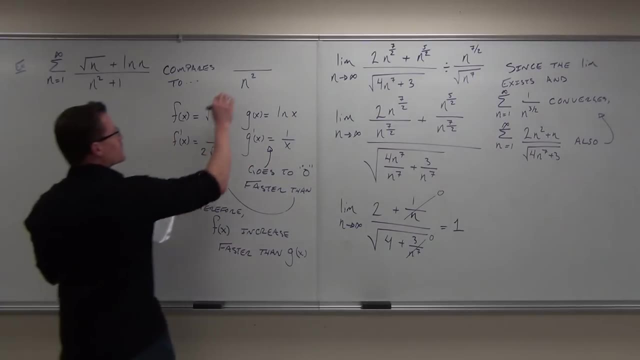 Okay, Don't just plug in numbers, Please, I'm begging- Plug in 7.. I don't know. No, don't do that. okay, Actually, go through the math here. So what are we going to pick for this one again? 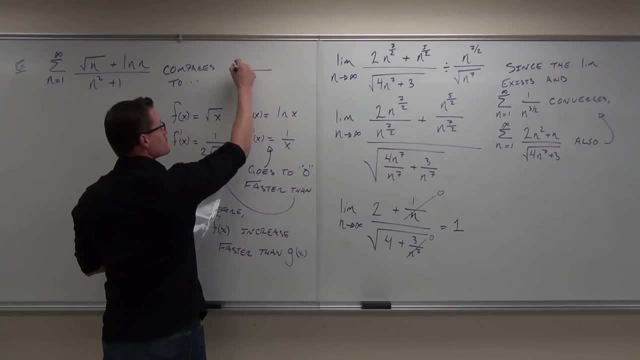 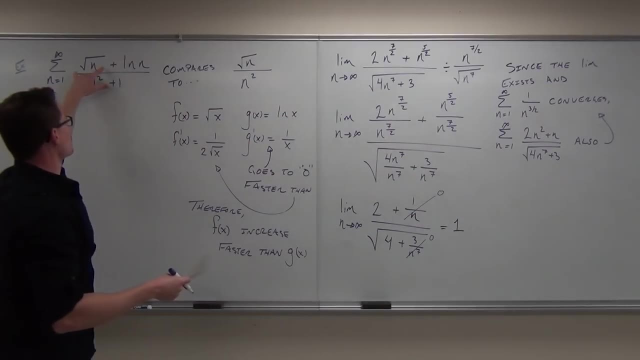 Is it going to be ln of n or square root of n? Square root of n? Yeah, it's going to be square root of n, because this one is going to be the model for n behavior, Since this increases faster than this one at n behavior. 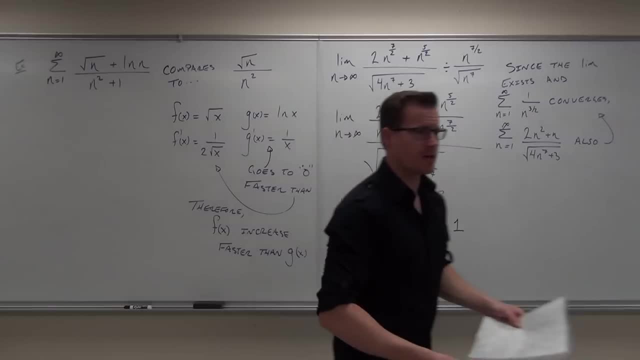 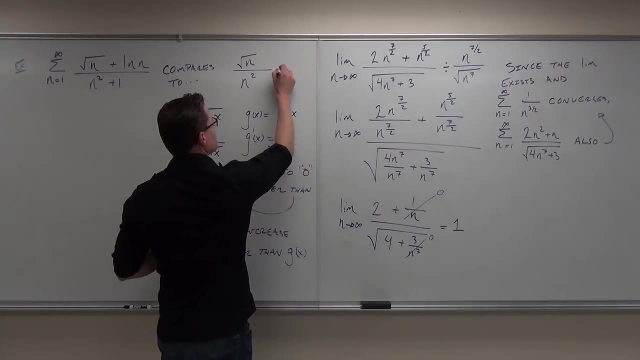 we use that Now. can you simplify it? Definitely, If you have only one term over one term, you better be able to simplify these things. Let's simplify it. What is it? n to the 1 half minus 2.. 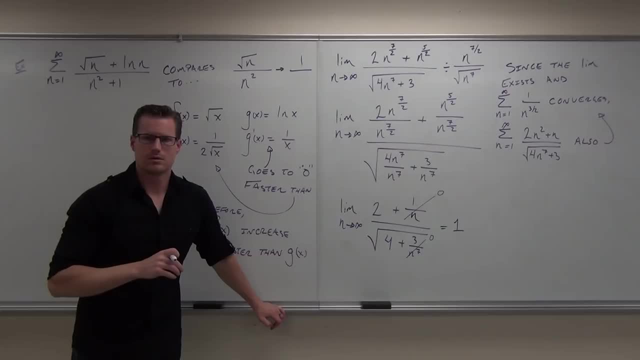 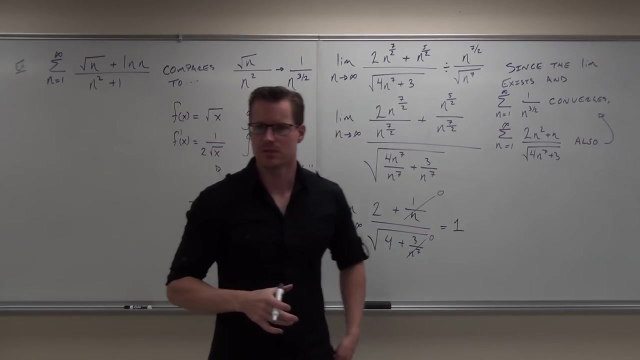 So 1 over? Don't leave me hanging. Huh, Is it 3 halves? Yes, it is 1 over 2?? 1 over 3 halves. 1 over n to the 3 halves- Exactly what that is. 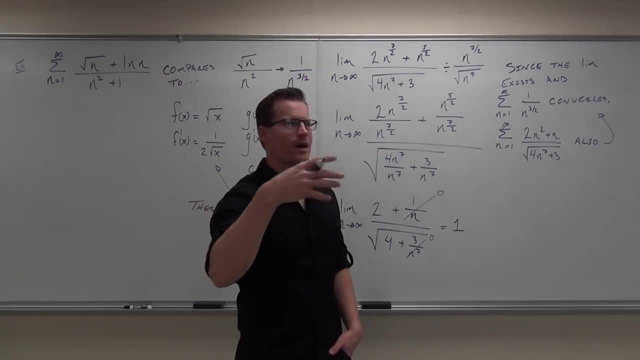 Does that make sense to you? We have square root of n, That's n to the 1 half. 1 half minus 2 is negative 3 halves. We'd have 1 over n to the 3 halves. Tell me something about that series. 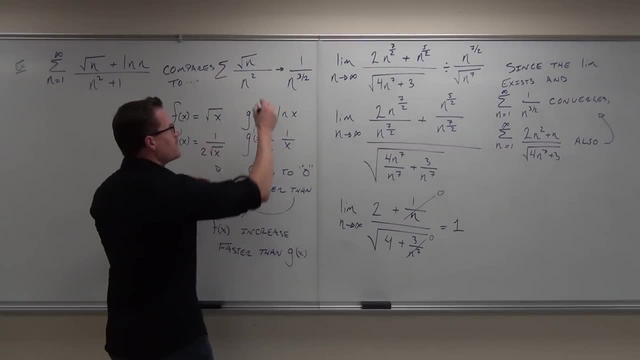 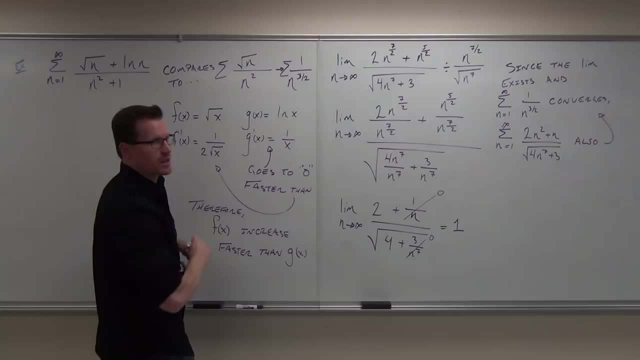 This is what now: P series. It's the same as last time. It's the exact same thing. It's a P series. I love P series, Me too. I really do. They're so easy. P series- P equals 3 halves greater than 1.. 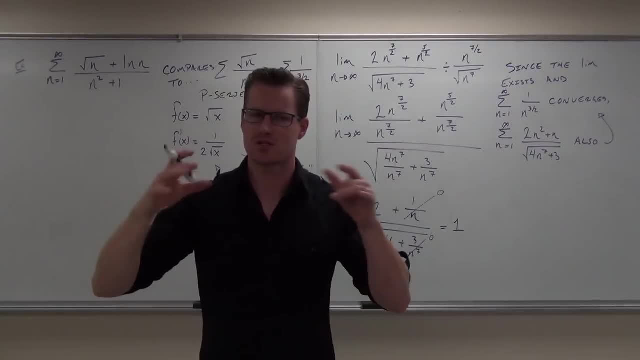 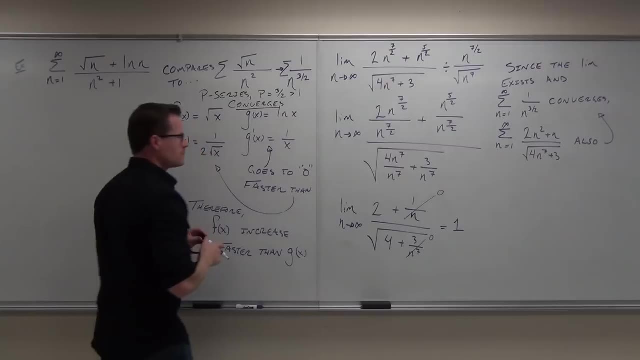 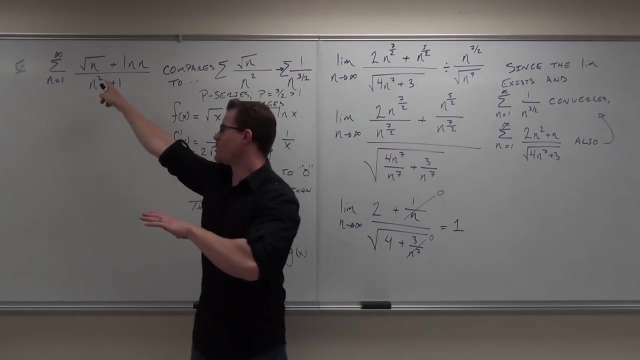 Tell me something about this particular P series, which we are comparing our given series to, Convergence Brilliant. So tell me this: If we compare this to this and the left, if the limit exists, what do we know about that? 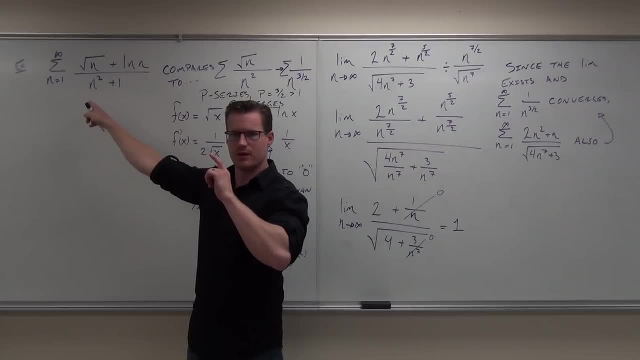 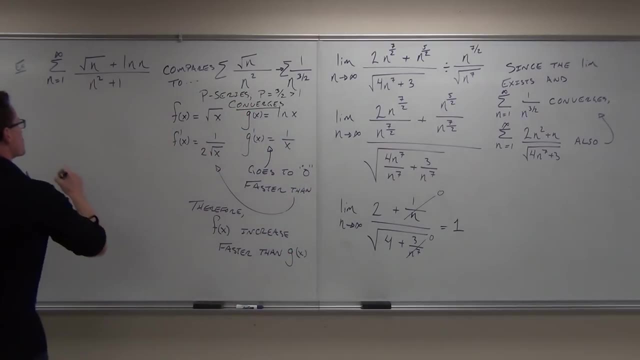 That it also converges. It also converges, Very good. What if the limit doesn't exist? Can't do it. No, no, no, no, Done, Can't do it. So let's do our limit comparison test. 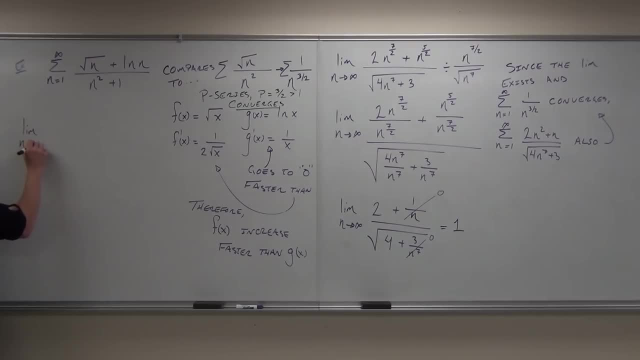 So we start off with a limit. as n approaches infinity, What goes on our numerator, please? N squared n plus ln n- Oh, that's going to be nasty. N squared plus 1, all over what? Over what N squared. 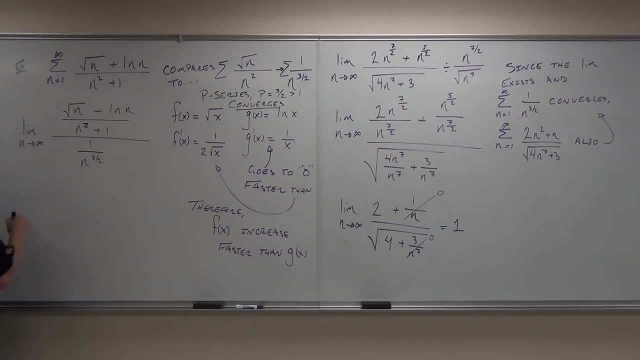 Over n to the 3 halves. Yeah, that's right, And then we start working with it. This is a limit as n approaches infinity, of square root of n plus ln, of n over n squared plus 1.. That's a lot of n. 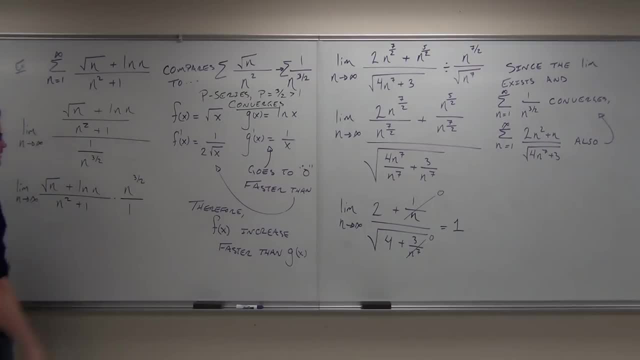 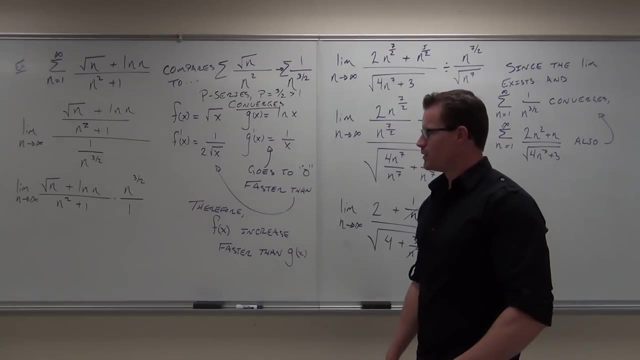 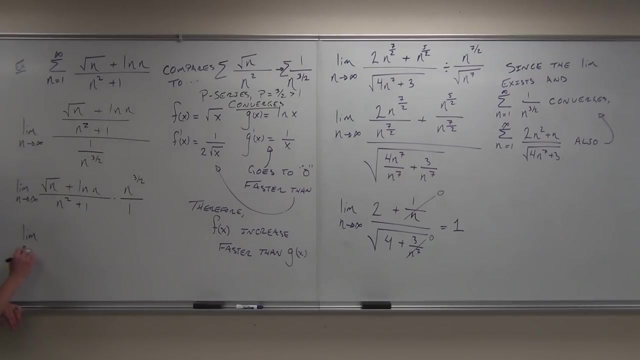 Dang N to the 3 halves over 1.. That is a lot. That is a lot. From there, what would we do? Let's distribute, Let's distribute. So if we distribute this, we get a limit as n approaches infinity of n squared. 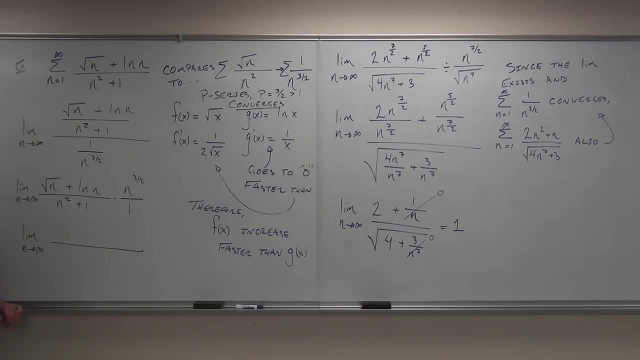 n to the 5 halves. Excuse me, n squared, Wouldn't it be n to the 5 halves? Yeah, If this is a 1 power, you'd have 2 halves plus 3 halves. It would be 5 halves. 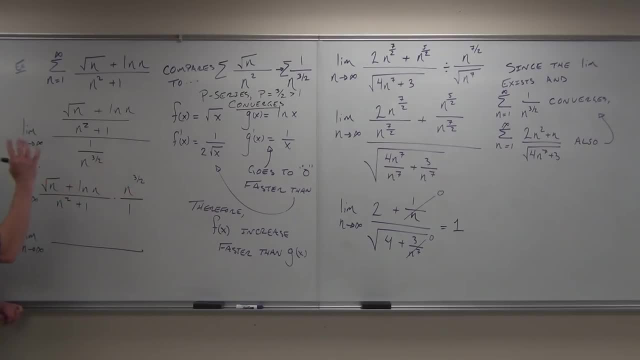 But this is a 1 half power. 1 half plus 3 halves is 1 over 2.. That's n squared 2. Plus n to the 3 halves. ln, I didn't know, it was right n. 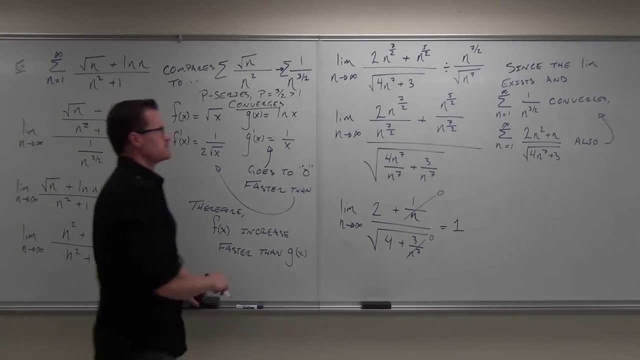 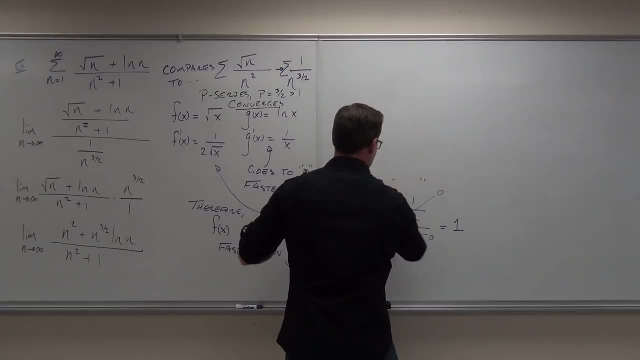 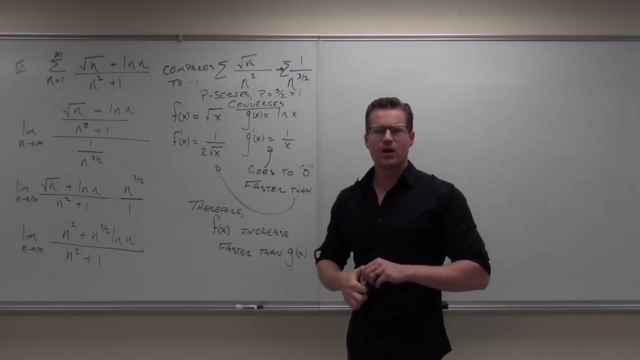 Over n squared plus 1.. Goodness gracious me, That's a lot of stuff going on. What's the next thing that you might want to consider doing? Would you try like a L'Hopital's right now or something? Is that a good idea? 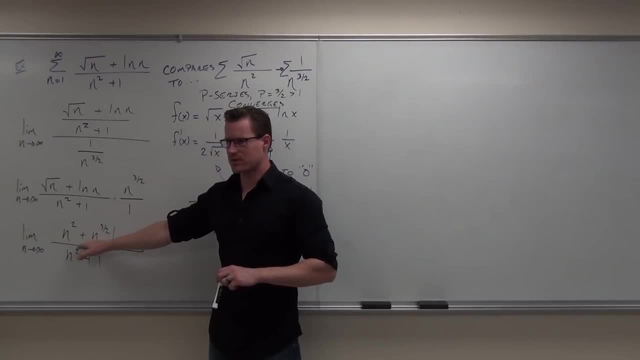 No, No, You get that plus right there. That's not a good idea, because this would be infinity plus infinity. We don't know what that is. Okay, That's not a good idea. Let's do the L'Hopital's. 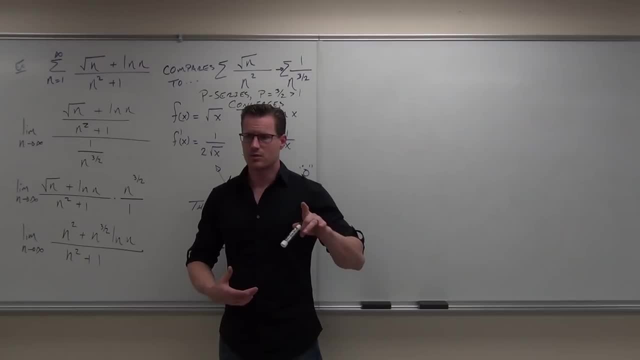 That's not a good idea. You can't do L'Hopital's out of the indeterminant form for you to do a L'Hopital's Now. I'll give you a caveat to that. You can do L'Hopital's on individual portions of this, because you could split up parts of. 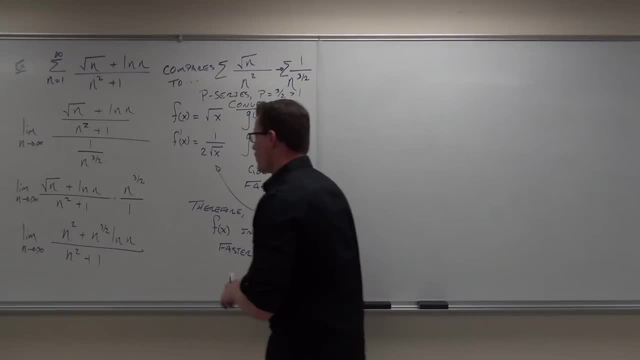 your limit. You could do that. I'll do that in a minute. So what would you do? Divide by n power? So let's divide by n squared Everywhere. So this is a limit, as n approaches infinity of n squared. divided by n squared. 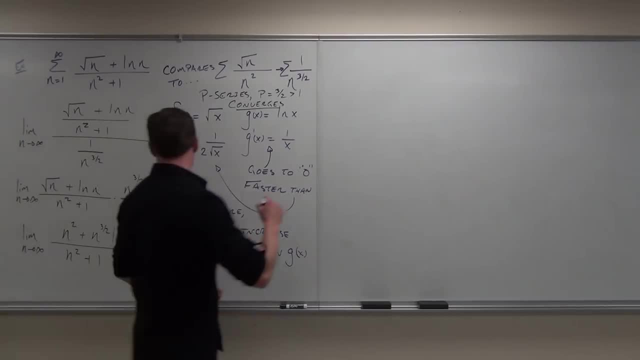 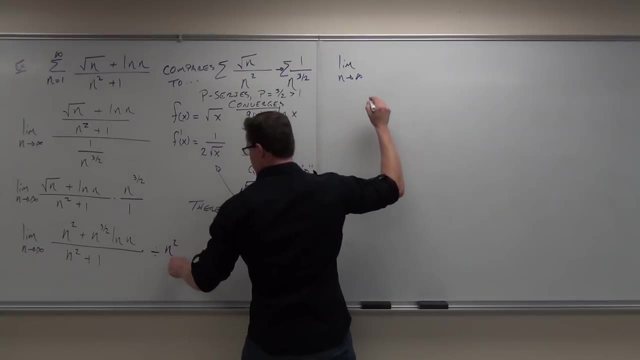 So the limit is n squared divided by n squared. So what's the limit? The limit is n squared divided by n squared, So it's 1 over 2.. 2. The limit, as n approaches infinity, of n squared divided by n squared. 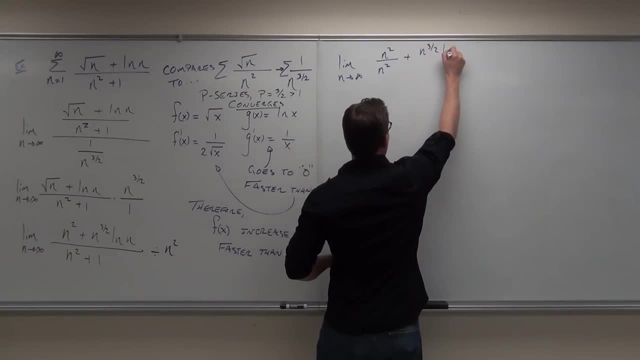 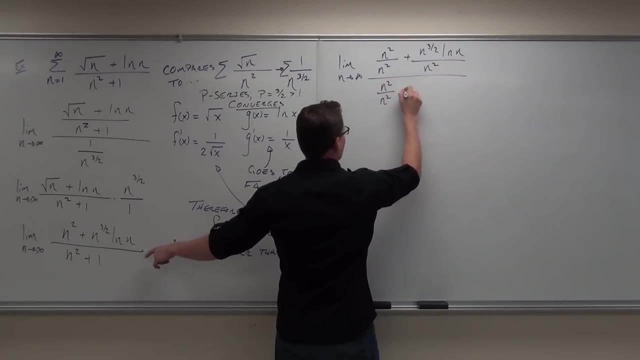 Yeah, I'm gonna write it out Plus n to the three halves ln: n over n squared, all over n squared over n? squared, plus one over n? squared, just so we see where everything's coming from. Limit as n approaches infinity. 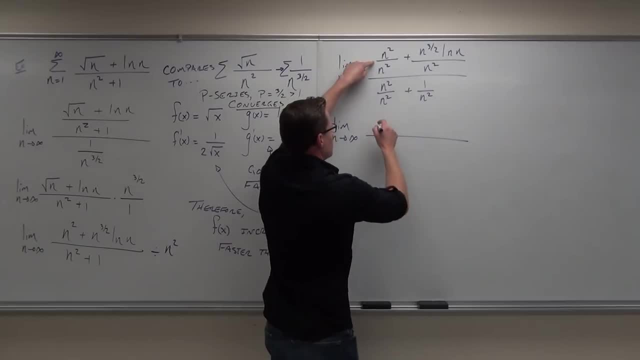 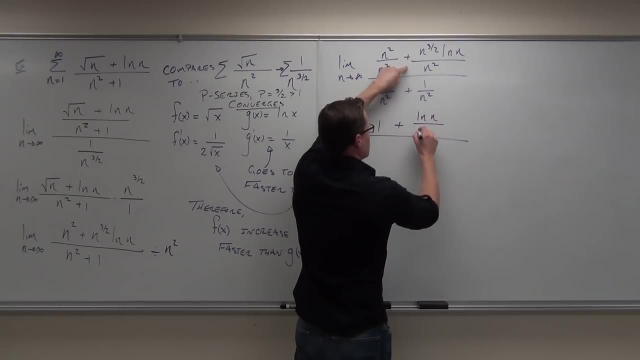 Oh goodness. So what's this? One Plus ln over n to the one half, ln of n over n to the one half. exactly, This is one. this is one over n to the second. Can I have a show of hands if you feel? okay? 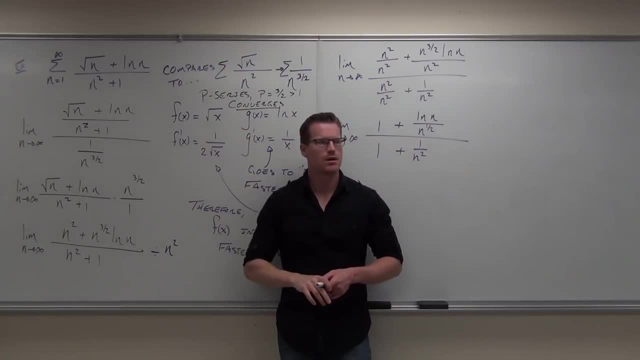 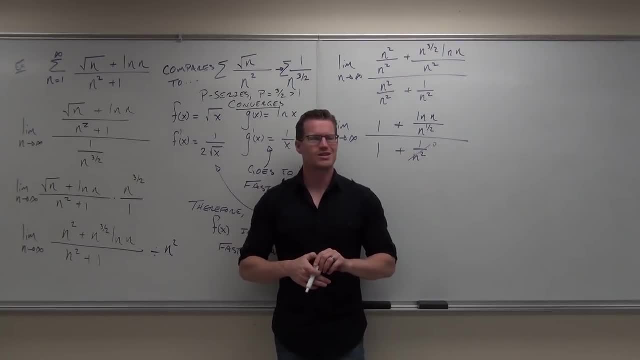 Zero. So this is going to zero. What about that one Indeterminate? It's an indeterminate form. Why is it an indeterminate form To infinity, over infinity. Brilliant, exactly right. So off to the side. Now you can do this, it's okay. 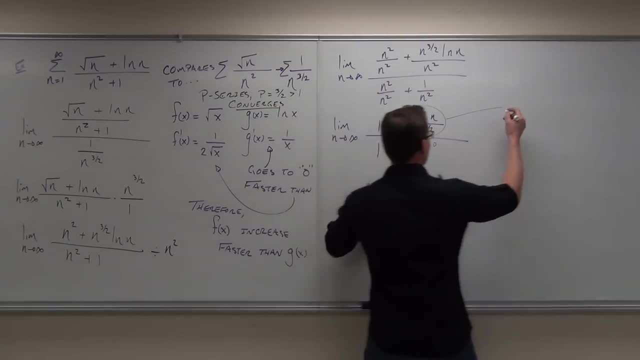 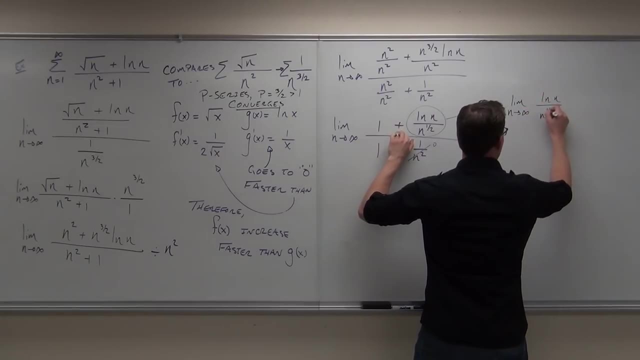 Here's why you can do it. You can separate this limit by addition. We can do a limit as n approaches infinity of ln, n over n to the one half. This thing equals infinity over infinity. so we'll do. Oh, what are you going to do with infinity over infinity again? 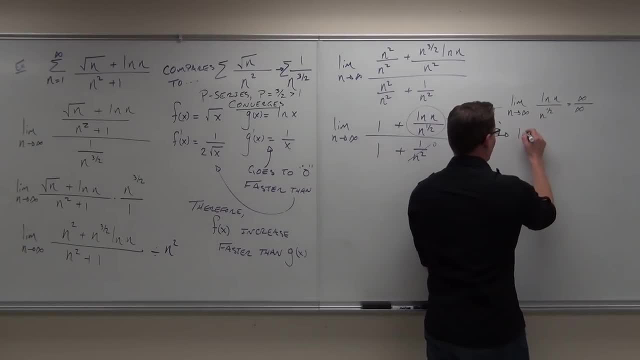 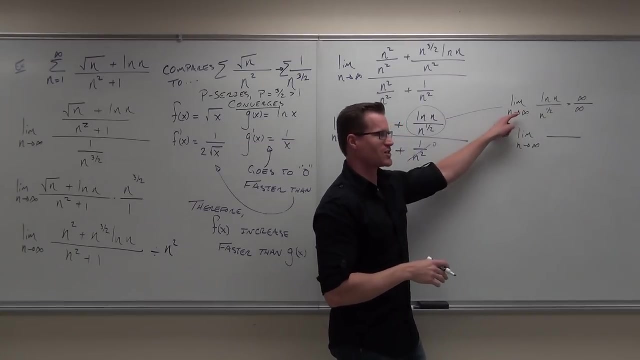 Love Lopey Tall. Love Lopey Tall. He's much better than Lopey Short Joking. That was a horrible joke. I get my sense of humor from my dad. Love you dad. I don't know if he watches these. 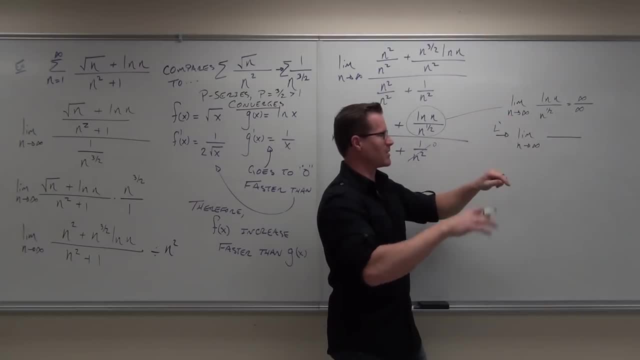 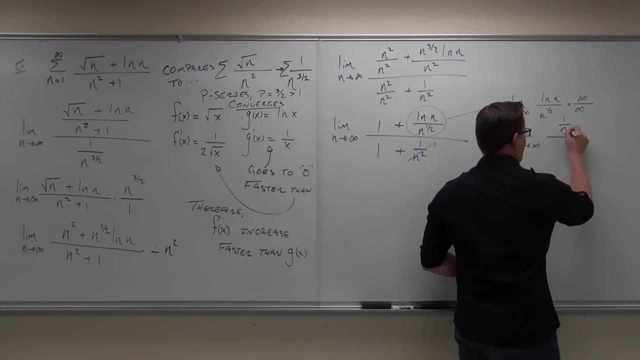 He should. He really should Give him something to do. He said he worked on this, but never mind, Don't watch that dad. So what's the derivative of L and N? One over N? Derivative of N. that looks sloppy, doesn't it? 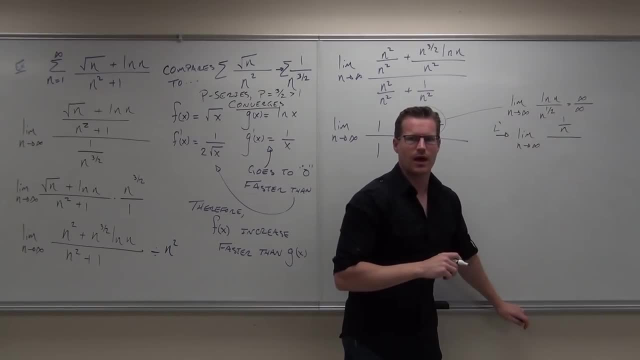 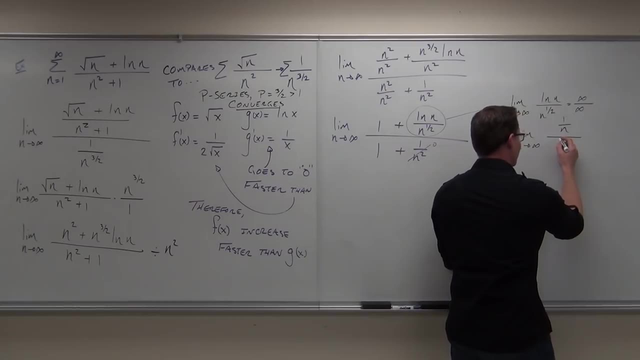 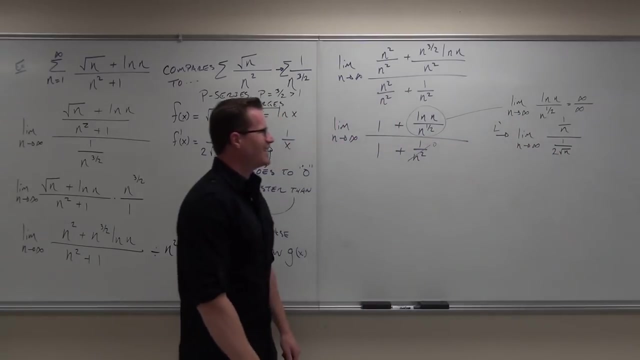 N to the one half. What's the derivative of N to the one half, N to the one half? No one half. N to the negative, one half. Okay, One over two. Okay, let's do that, It's easier. 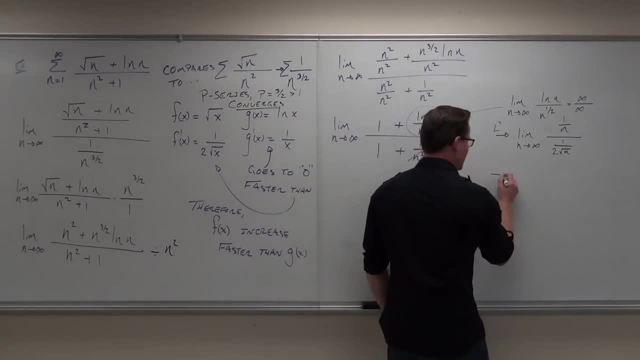 Yeah, one over two square root of N. My Math serves me correctly. I don't think so. Is it a negative? No, no, it's not. I don't think so. because you bring in the one half, You take one away from the exponent. 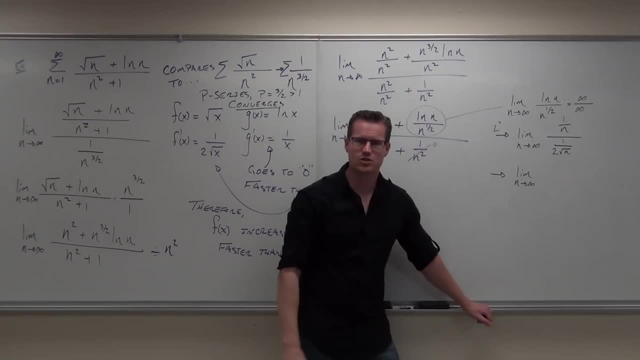 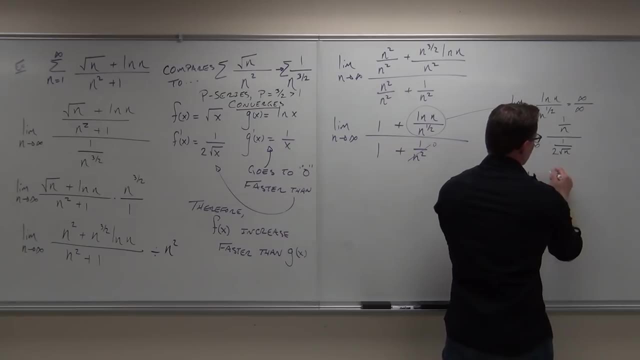 It becomes negative. That's a negative exponent that goes to the denominator. So two square root of N, Let's go ahead and let's reciprocate and multiply. So we have. If we reciprocate and we multiply, we're going to have. 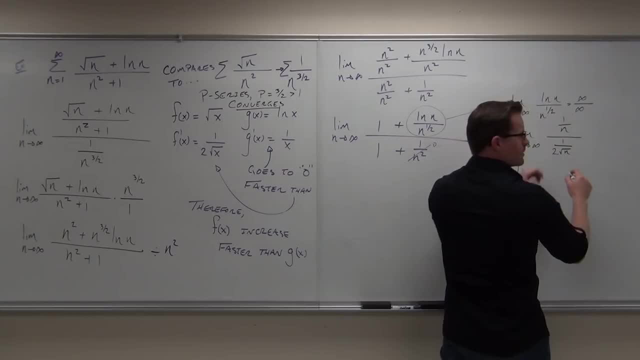 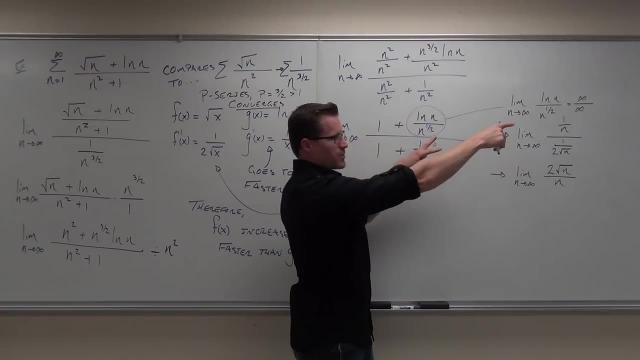 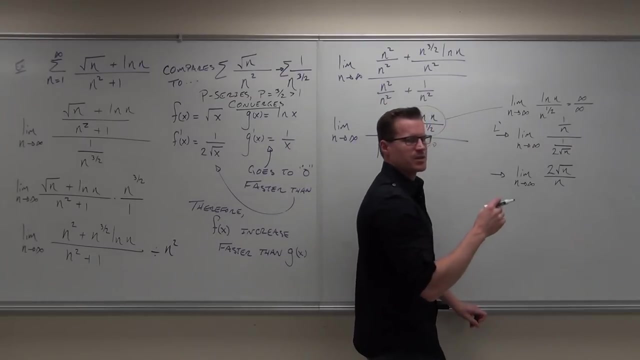 What is that? Any time now, One over N times two, root N, Reciprocate and multiply. So far, so good. Yeah, Okay, Well, yes, but be smarter about this. okay, I should have taught you something. 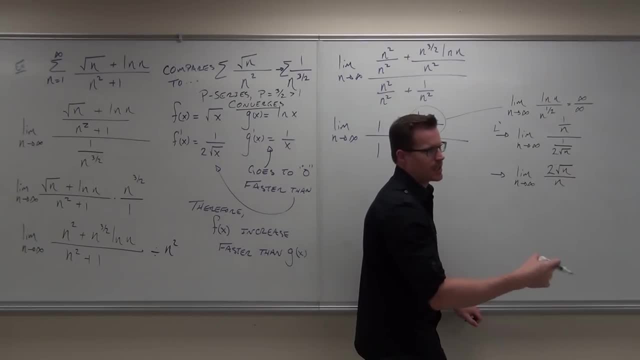 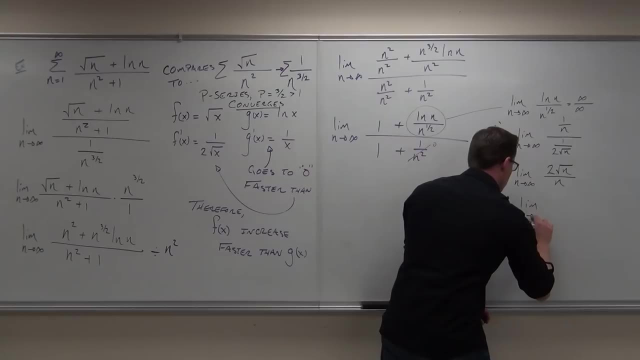 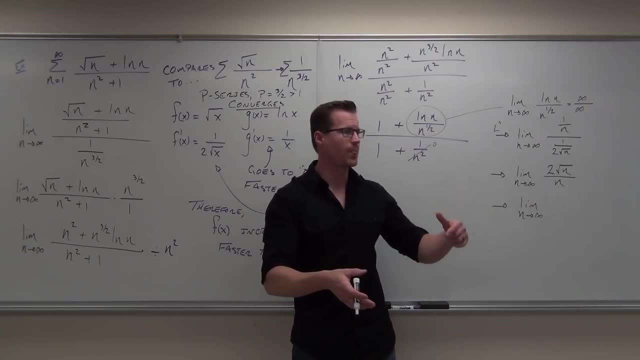 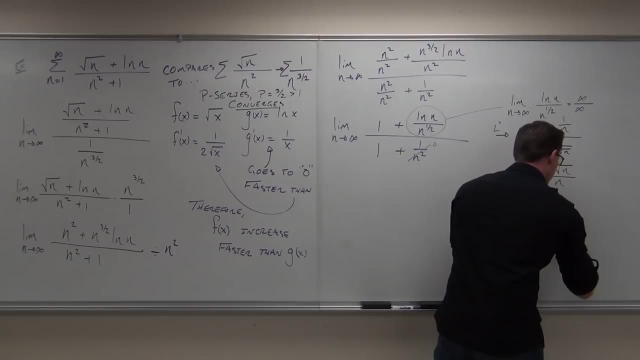 We should have learned that a long time ago when I said with L'Hopital's rule, before you do it again, you must simplify the fraction, And that goes without saying, hopefully for you. So with us, this is going to be two over the square root of N. 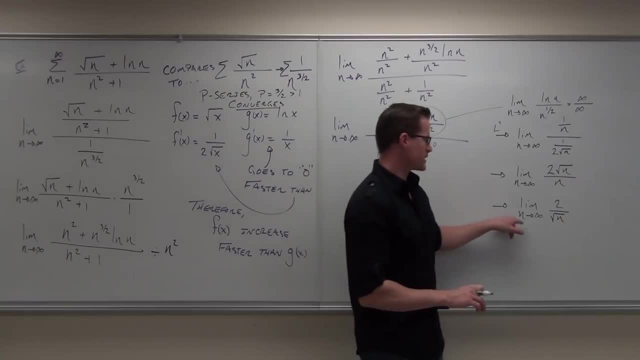 Yes, no, Tell me something about the limit, as n approaches infinity, of two over the square root of N. What is it? Zero, Okay, So now we know this thing is zero, So we have a limit as n approaches infinity. 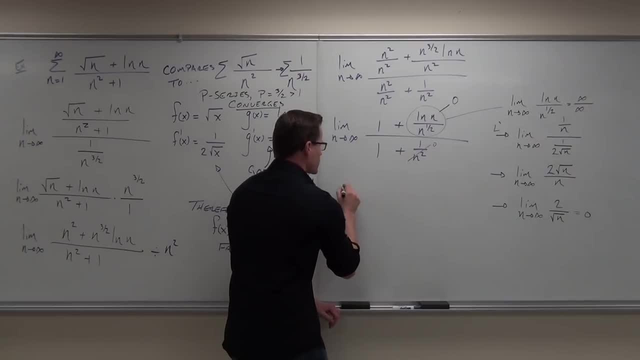 Actually we let it, I'm sorry, we let it approach infinity. What's this limit going to equal? We have one plus zero over one plus zero. How much is that One? So our limit equals one. Do most of them come out to one? 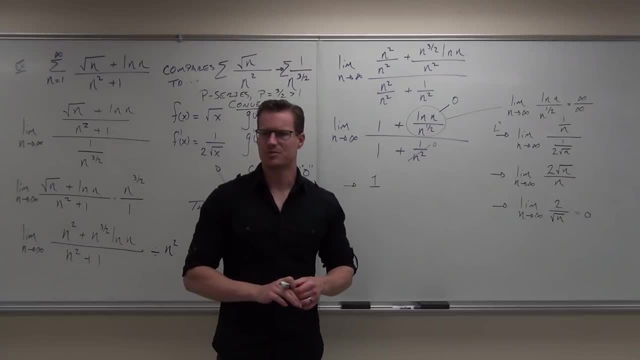 I can't say that. No, I don't know, It just depends, Just coincidence. So it's one over one, right Yeah? So what? So the limit of that is one over one, because that, in the term of one, approaches infinity. 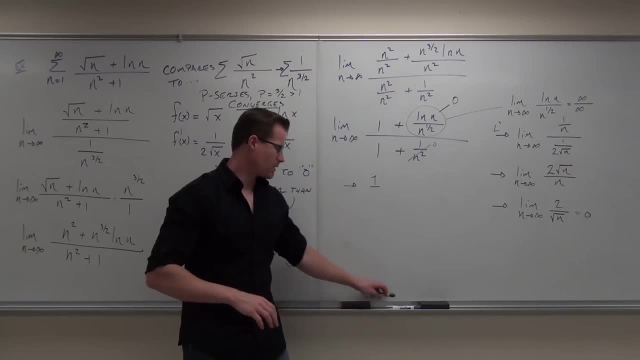 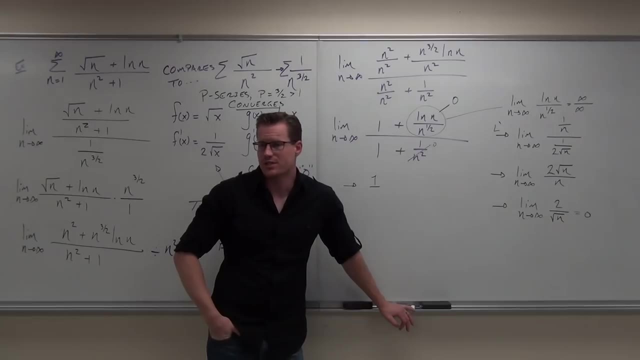 Right, You know I'm going to go out there on a limb and say, yeah, they probably do, because if you're talking about n behaviors and you're saying they're very close, you have basically something over the same thing, So a lot of them should work out to one. 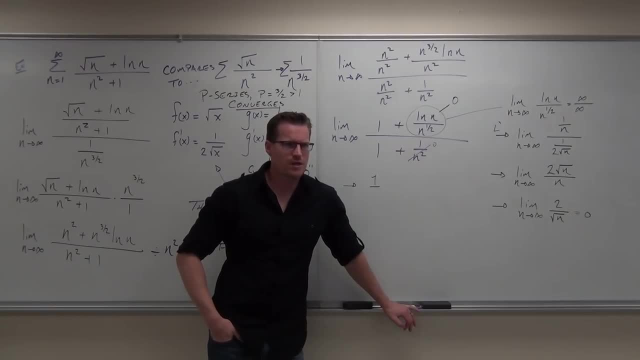 What's the next statement that you're going to make? Do you know the next statement that you're going to make? Yes, Since the limit exists. Since the limit exists, So write that down. Since the limit exists, Series And. 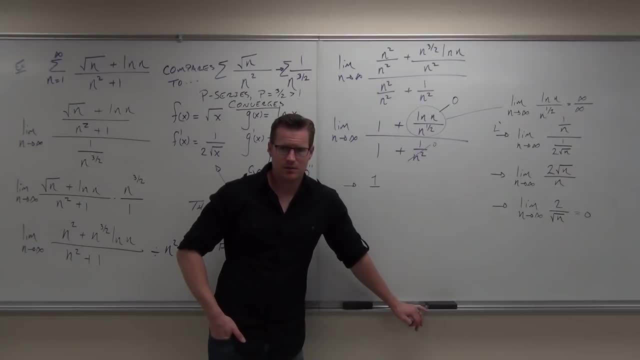 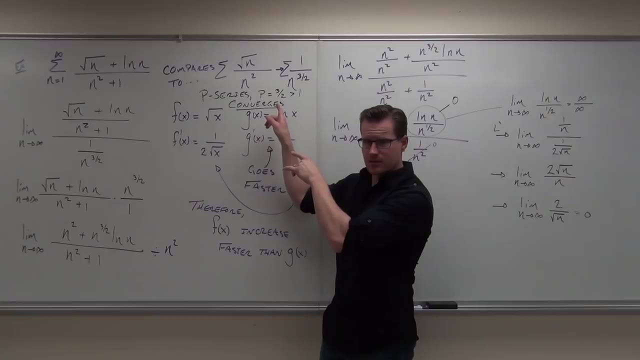 And the series of one over N to the three-half of infinity. Okay, And the series of one over N to the three-half is convergent Because, Because it's greater than one. Very good, Then, what do you know about our given series? 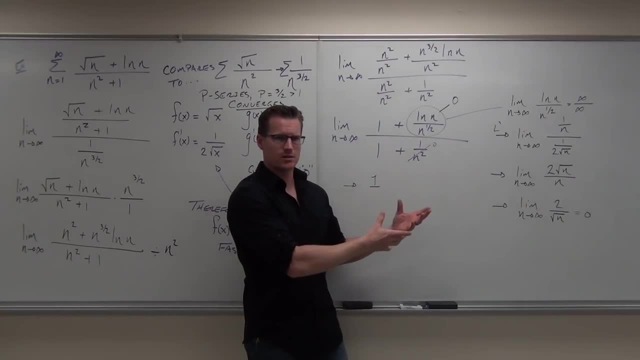 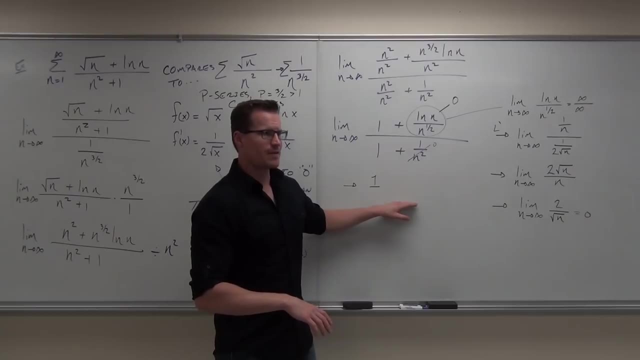 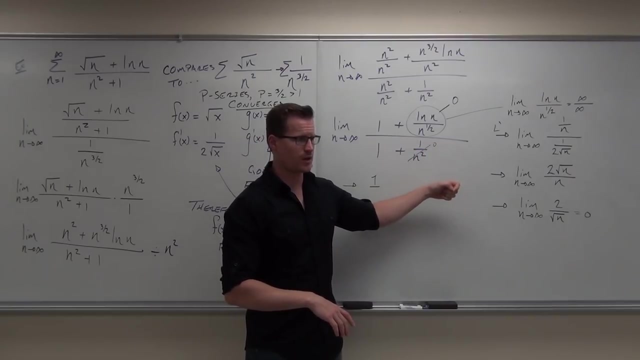 It also converges. That's exactly what you should write. So word for word: since the limit exists and the series of one over N to the three-halves is convergent by P series, P is three-halves greater than one, then, and this is the only. 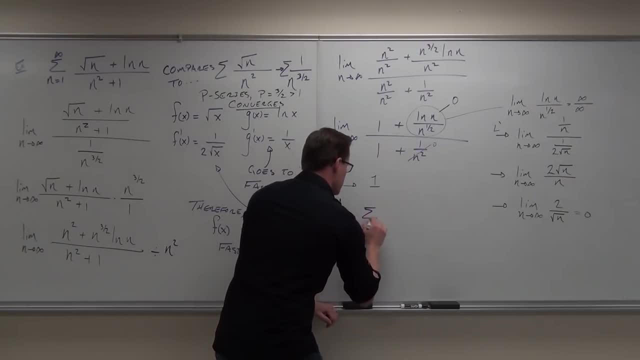 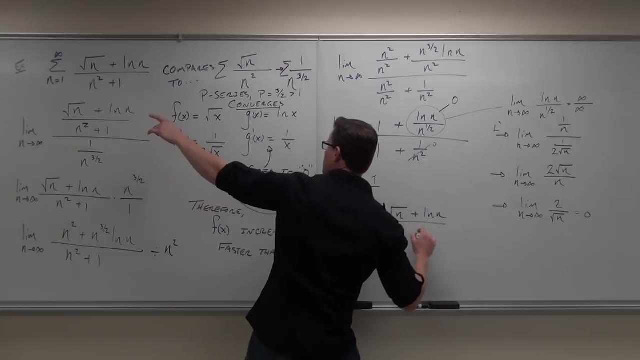 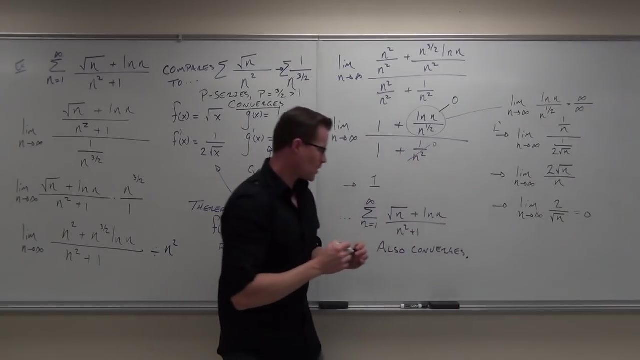 part I'm going to write because I ran out of room. then the series of one over N to the three-halves that we were given also converges, Also converges. Here's what I'm wondering – does a limit comparison test make sense to you? 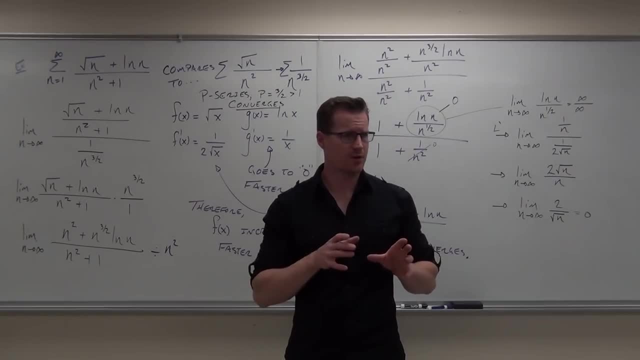 It does. It's kind of a cool thing, isn't it? It's saying: use the N behavior, end behavior, make a limit out of it. it's just a ratio saying: if the end behaviors are very similar, make a ratio. if that limit exists, then sure enough. 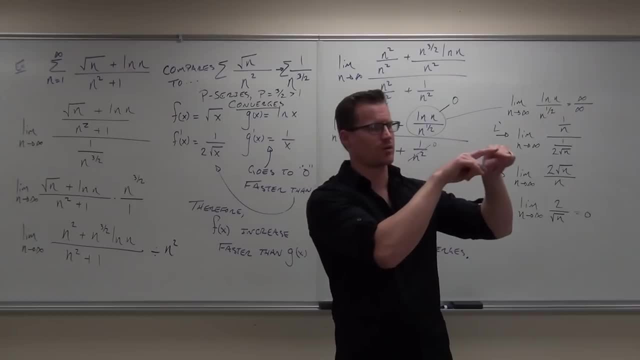 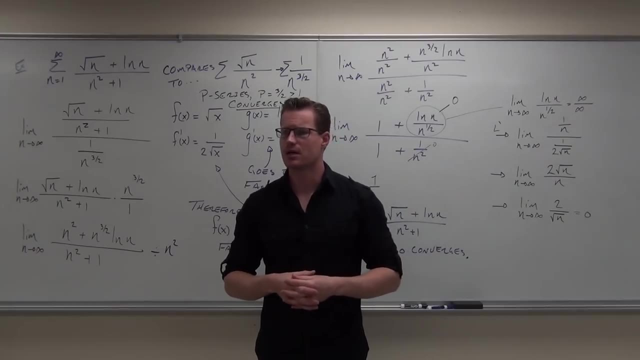 they're both gonna be convergent or both divergent, because they model after the same curves, basically, at the end, behavior. that's the idea. So we have a number of things now, and here's the wrap up, the number of things. 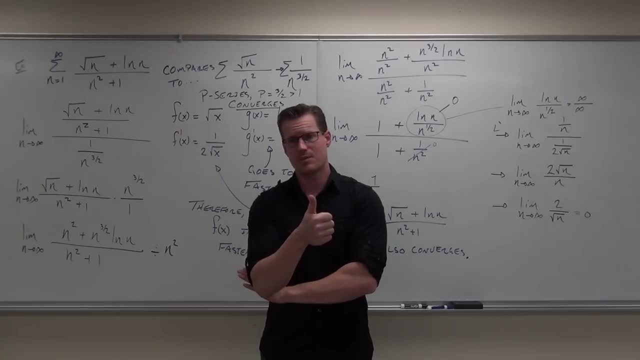 First thing you always check for is: yeah, always take a limit of the sequence from which your series is stemming. okay, Just the terms. If it equals zero, you must keep going. If it doesn't equal zero, you're done, because that whole thing is divergent, okay. 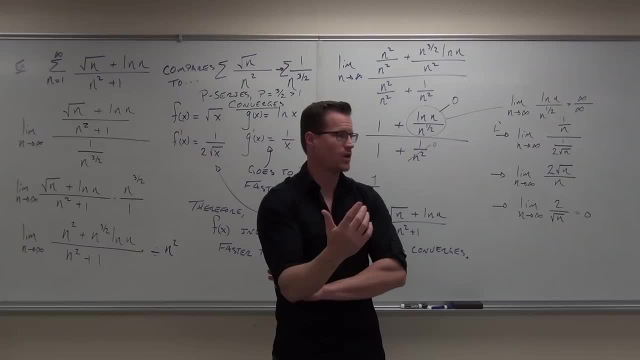 After that, check for the easy ones. Don't make this stuff harder than it is. I would automatically check for a geometric. maybe I can make it. I would automatically check for a piece series. I mean, that'd be a piece of cake. that'd be kinda nice. 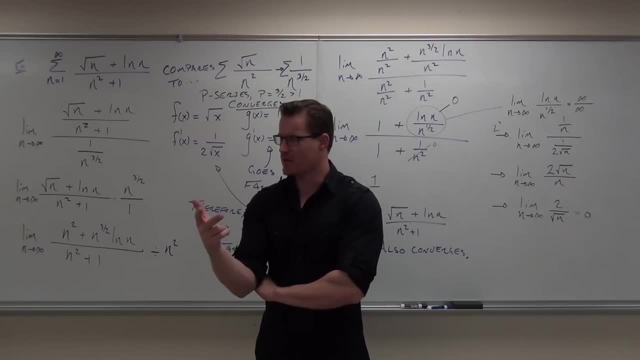 After that I'd check for if it's an easy integral, I'd do integral test if I can do that. or we could do now a comparison test, like an easy comparison test would be kinda cool to do because there's less than something. 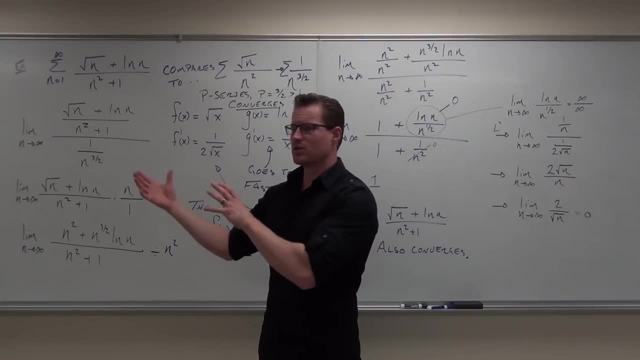 that's sometimes really easy to do. If that's not the case, we gotta do a limit comparison test. So for some of these nasty looking ones, the limit comparison test is the way to go, if you can show what the n behaviors are appropriately. 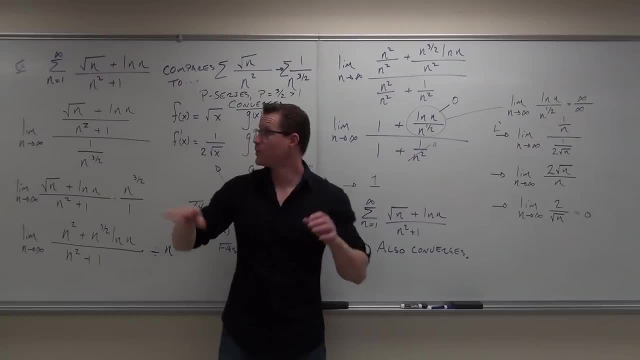 So for us remember, that was this whole piece right here saying: well, we wanna stick with the square root of n and not the ln of n, because that is really the n behavior of that function. Does that make sense? That's the numerator of our sequence, as it were.